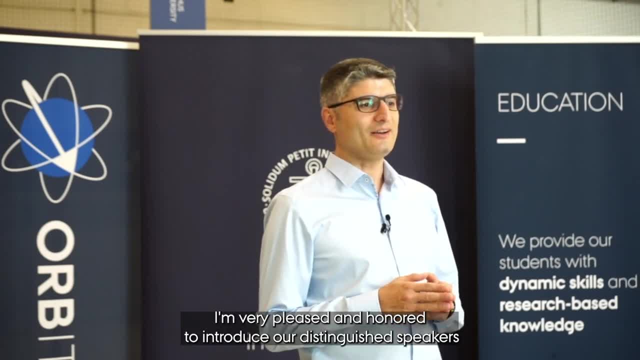 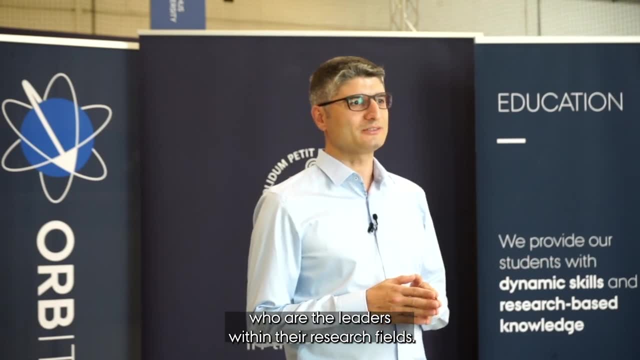 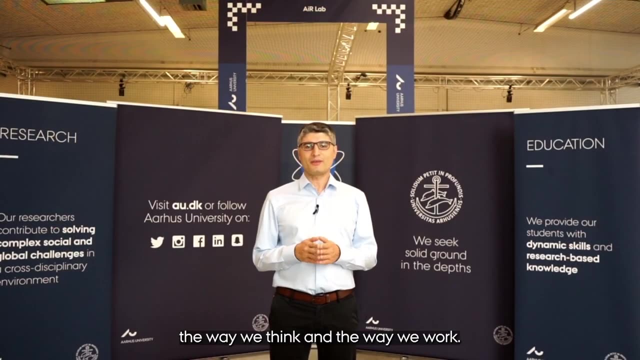 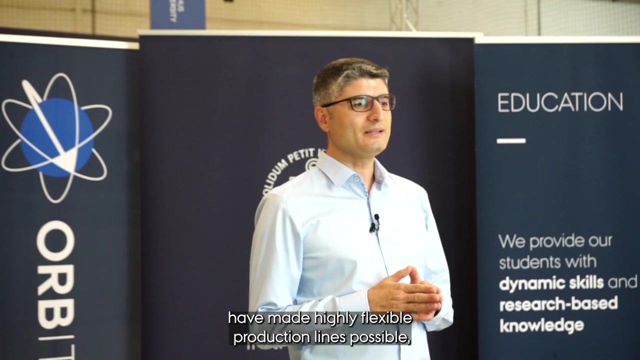 University. I'm very pleased and honored to introduce our distinguished speakers, who are the leaders within their research fields. Robotics and AI have been changing our world, the way we think and the way we work. Digitalization and Industry 4.0 have made highly flexible production lines possible. 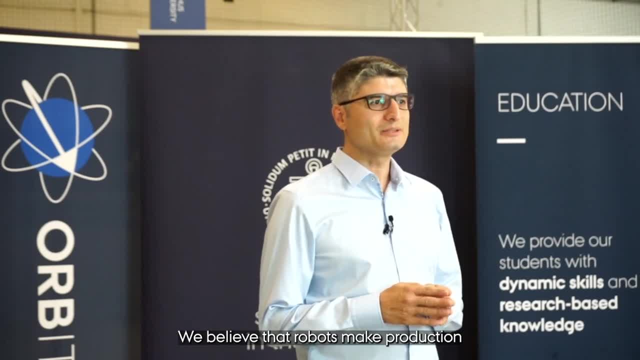 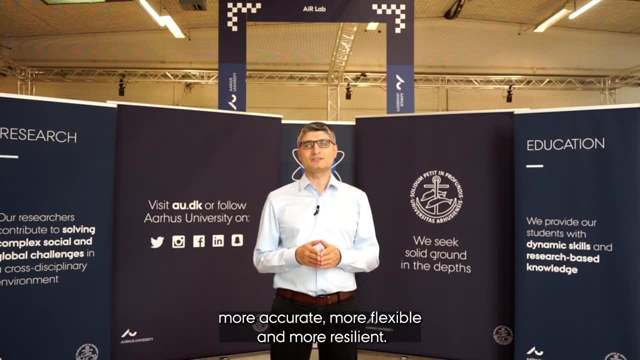 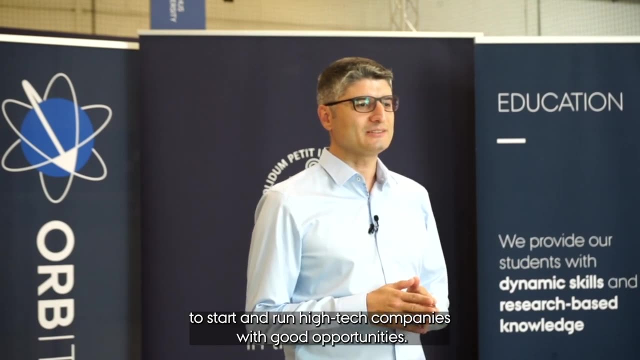 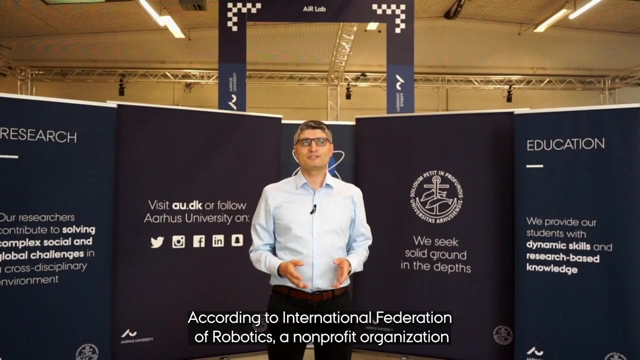 that was not possible before. We believe that robots make production more accurate, more flexible and more resilient. Aarhus University and Aarhus in general is a fantastic place to start and run high-tech companies with good opportunities. According to the International Federation of Robotics, a non-profit organization in Germany, the annual global robotics turnover 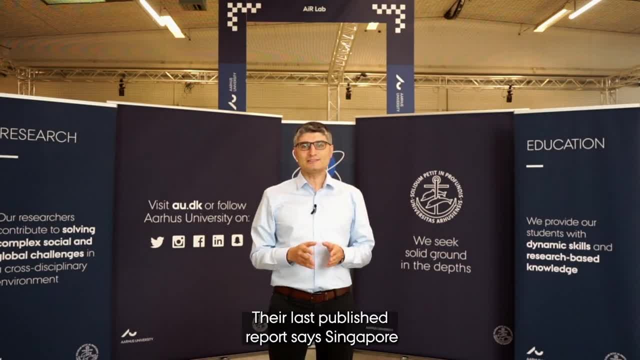 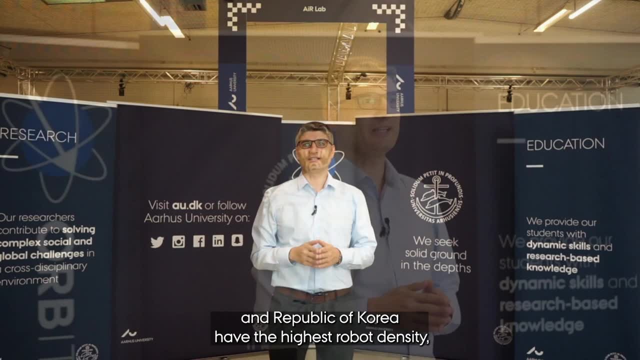 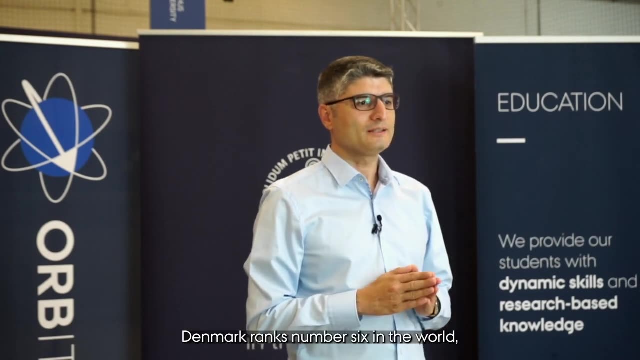 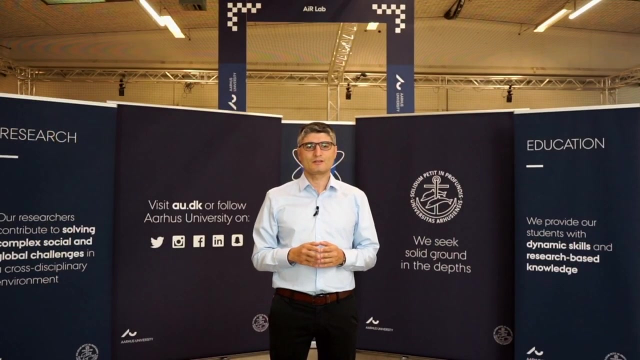 is 50 billion dollars. Their last published report says Singapore and Republic of Korea have the highest robot density, which is defined as robots installed per employees in a country. Denmark ranks number six in the world according to this criterion, which is amazing. COVID-19 was unfortunate for the whole world in 2020.. 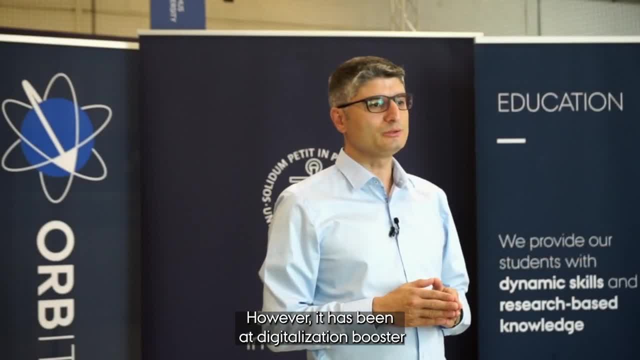 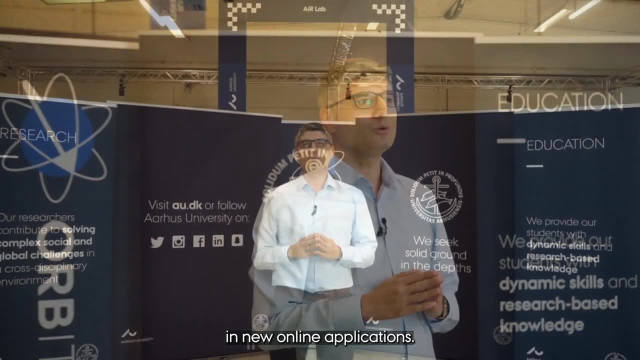 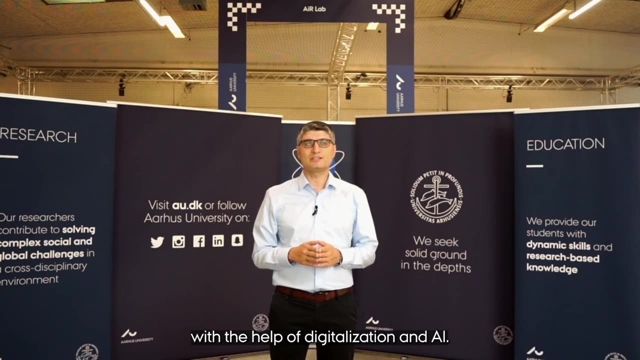 However, it has been a digitalization booster because we have been aware of the importance of increased demand in new online applications. Adaptation is the new normal, with the help of digitalization and AI. According to a recently published report by the Danish Academy of Technical Sciences, Denmark's high-tech companies employ more than 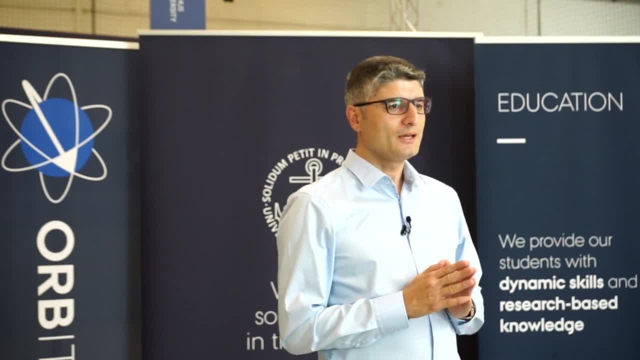 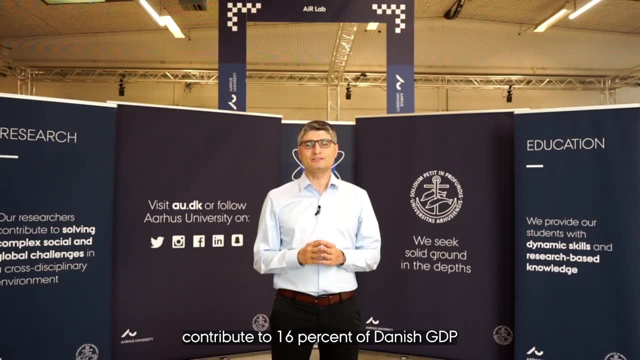 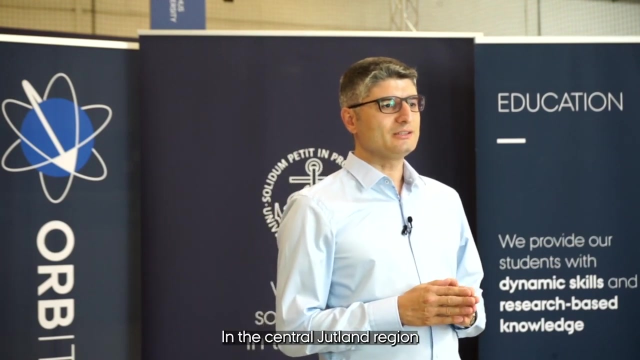 300,000 full-time employees. In total, 2,363 high-tech companies contribute to 16% of Danish GDP and 40% of Denmark's total exports. I believe this data shows Denmark is a knowledge-based innovative economy. In the central Jutland region, there are 456 high-tech companies. 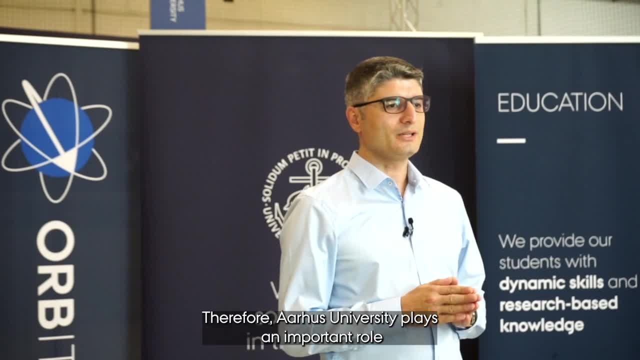 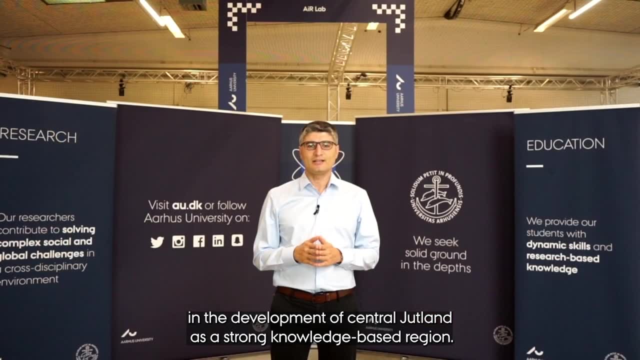 that employ 61,000 people. Therefore, Aarhus University plays an important role in the development of central Jutland as a strong, knowledge-based region. As you might have noticed, AI surrounds us. AI is everywhere, such as in our mobile phones. 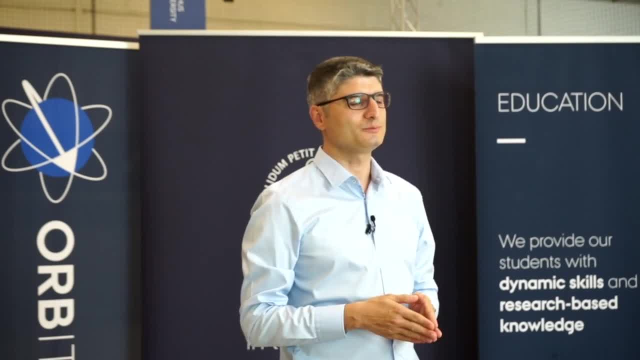 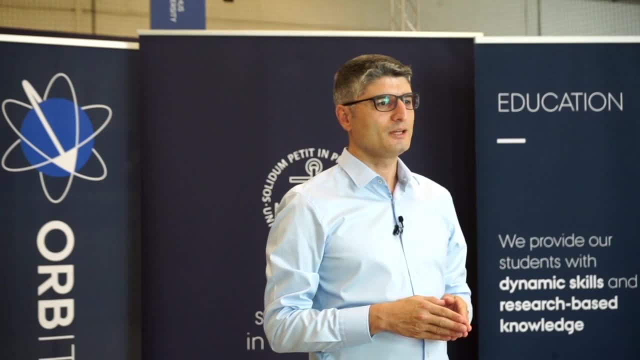 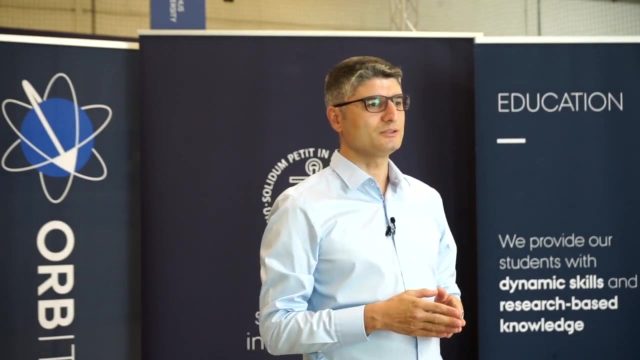 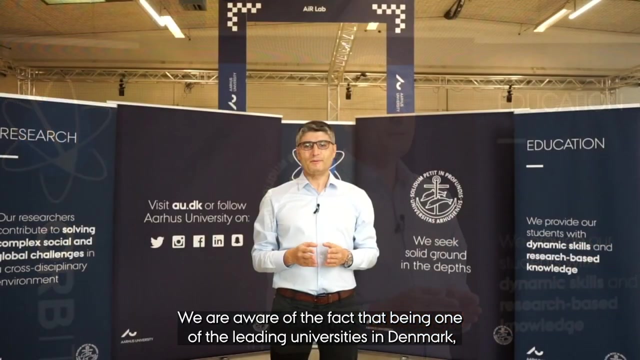 social media channels, financial markets and so on. We are pushing the boundaries of AI and creativity In today's fast-moving world. there is a fascinating scientific and technological revolution in the robotics and AI area. We are aware of the fact that, being one of the leading universities 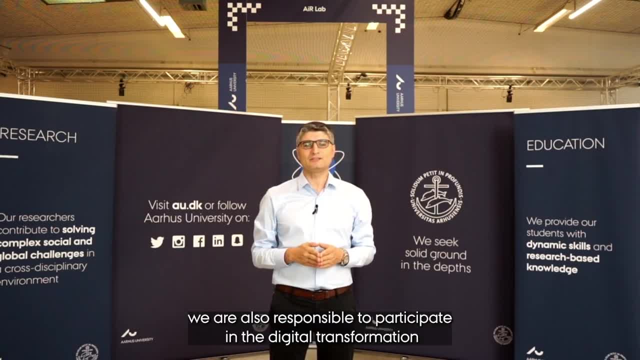 in Denmark, we are also responsible to participate in the digital transformation of the Danish industry by offering them new knowledge and innovation. Before we start our amazing presentations now, it's my pleasure to give the floor to our wise dean, Brian Winter, who will share his view about robotics and AI at Aarhus University. 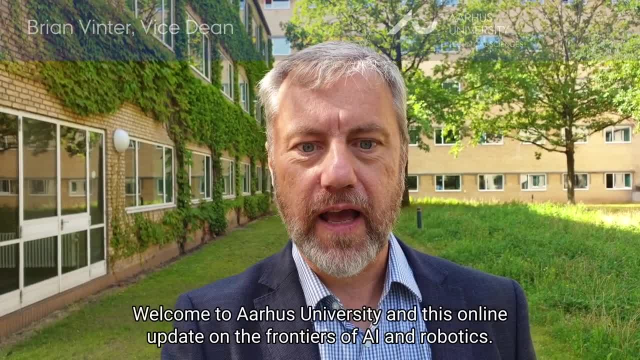 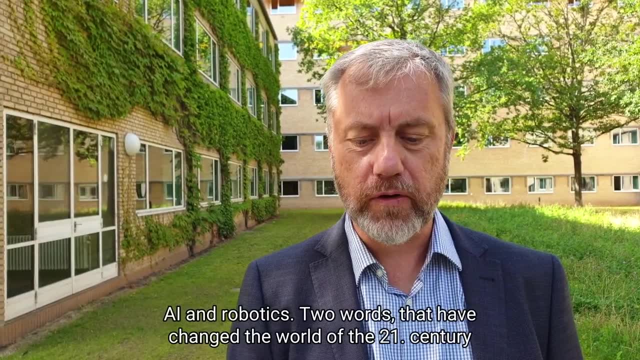 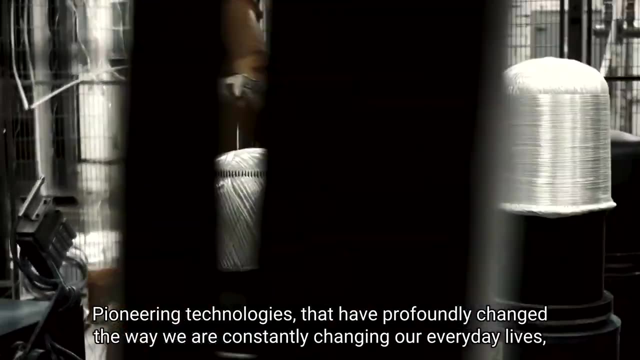 Welcome to Aarhus University and this online update on the frontiers of AI and robotics. AI and robotics are two words that have been together for more than 25 years, two words that have changed the world of the 21st century. pioneering technologies that have profoundly changed the way we are constantly changing our everyday. 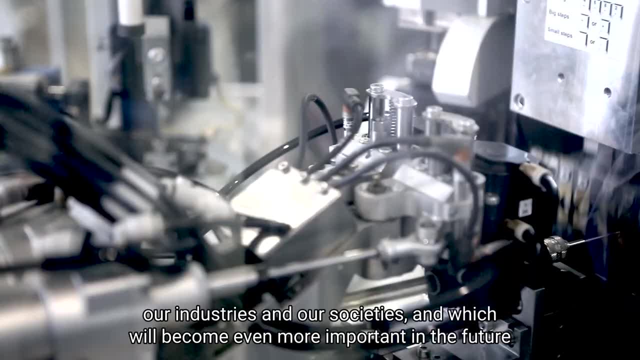 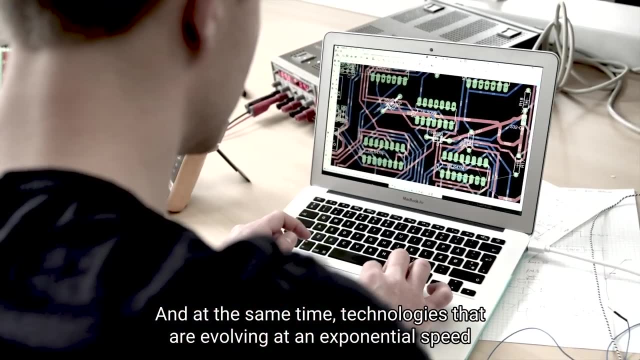 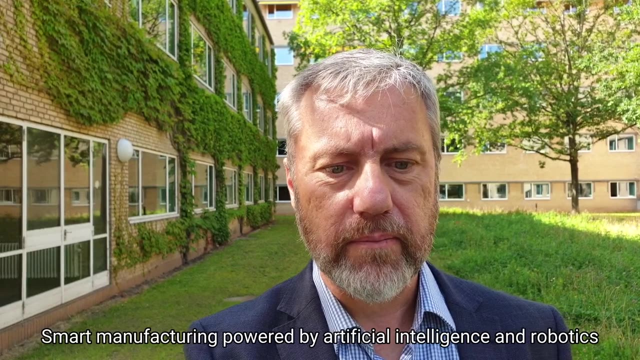 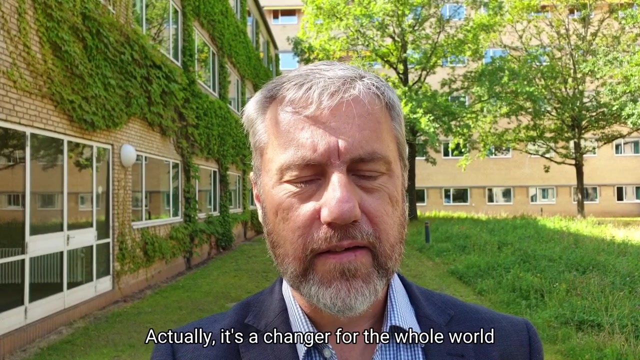 lives, our industries and our societies, and which will become even more important in the future, and, at the same time, technologies that are evolving at an exponential speed and where today's state-of-the-art is tomorrow standard. smart manufacturing powered by artificial intelligence and robotics is a game changer for academia and industry. indeed, actually, it's a changer for the 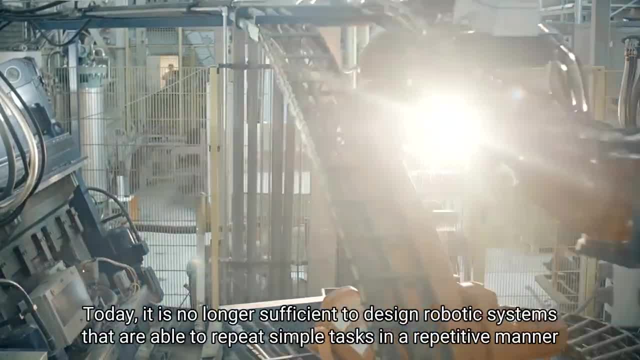 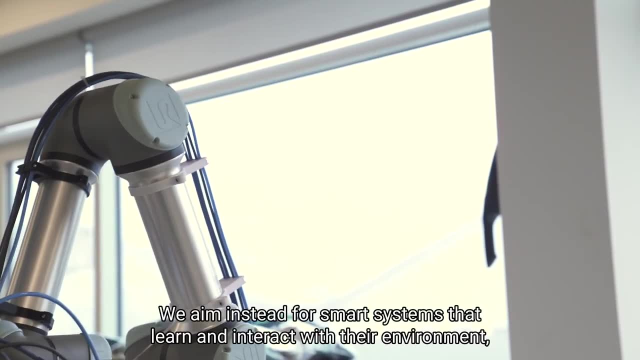 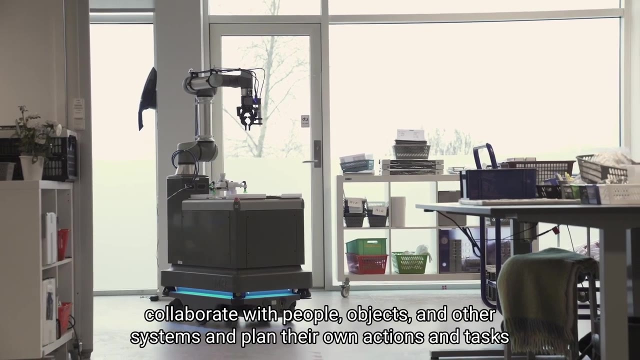 whole world. today is no longer sufficient to design robotic systems that are able to repeat simple tasks in a repetitive manner. we aim instead for smart systems that learn and interact with the environment, collaborate with people, objects and other systems, and plan their own actions and tasks accurately and efficiently. 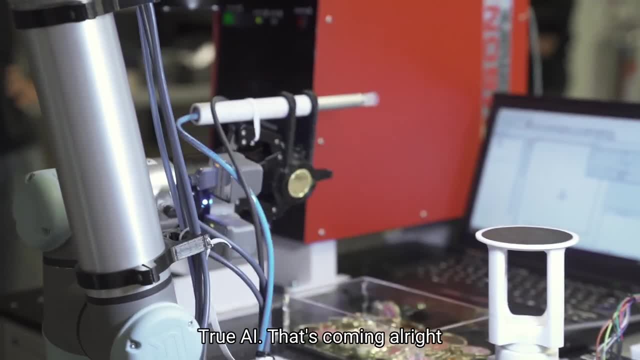 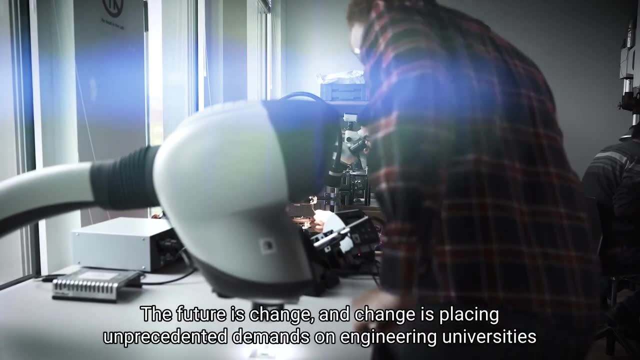 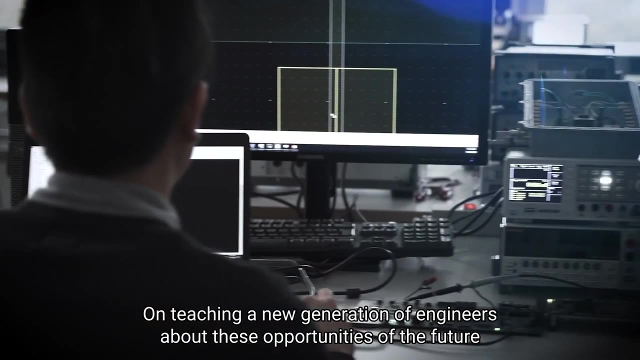 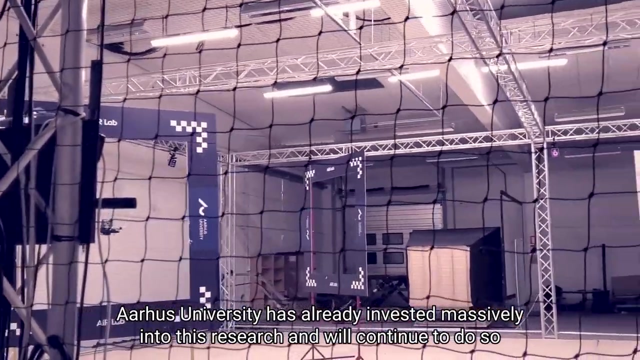 and completely autonomously through AI. that's coming all right. the future is change, and change is placing unprecedented demands on engineering universities, on research and development of these breakthrough technologies, on teaching a new generation of engineers about these opportunities of the future. Aarhus University has already invested massively into this research and will 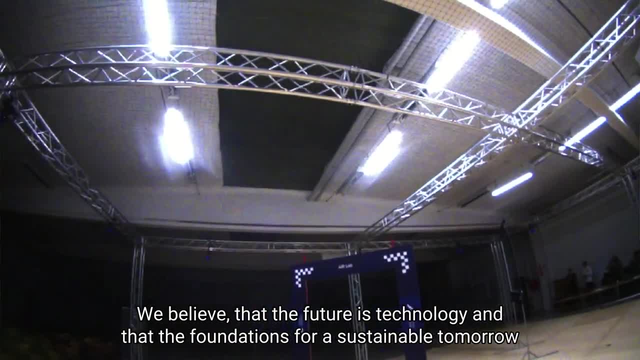 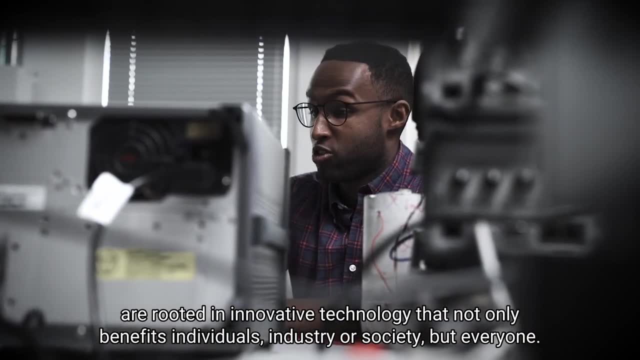 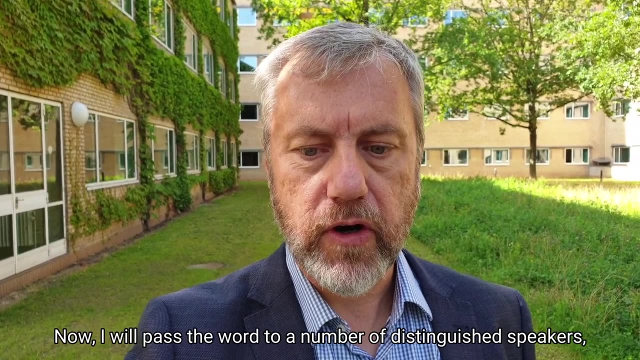 continue to do so. we believe that the future is technology and that the foundations for a sustainable tomorrow are rooted in innovative technology that not only benefits individuals, industry or society, but everyone. now I will pass the word to a number of distinguished speakers, all world-leading researchers in their 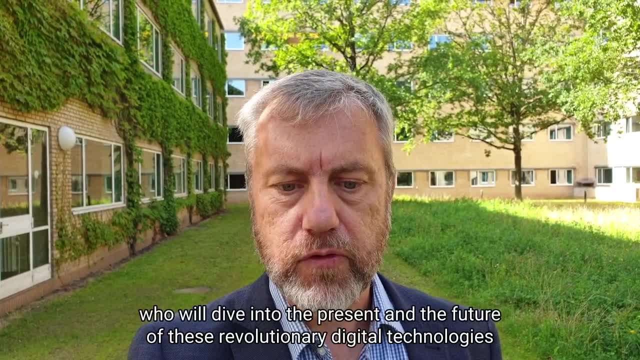 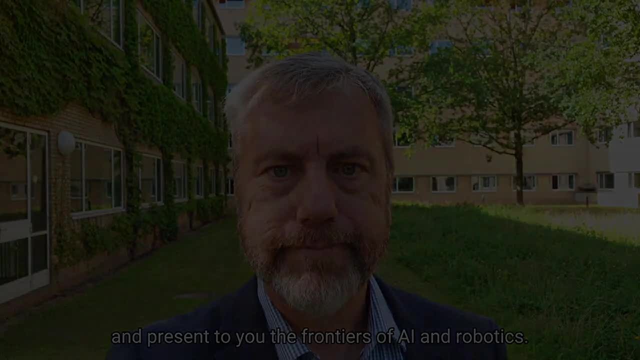 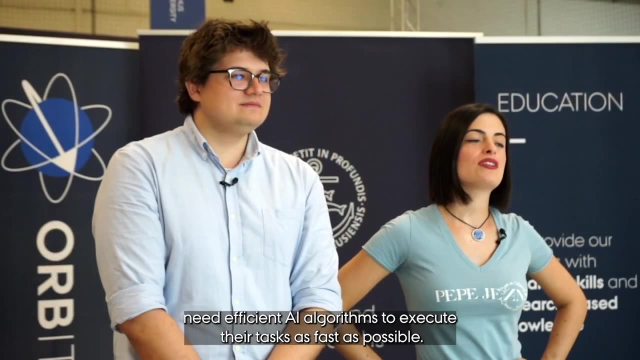 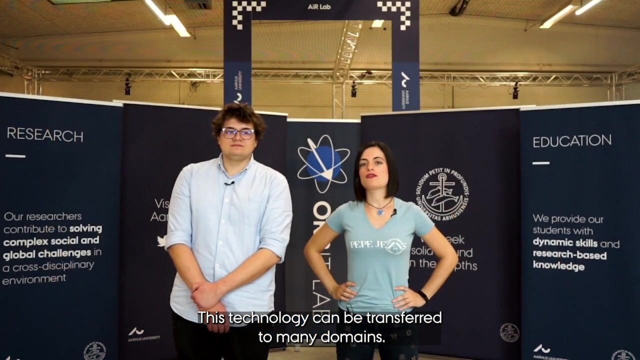 specific field who will dive into the present and future of these revolutionary digital technologies and present to you the frontiers of AI and robotics? do you know that quadrotors can now match the speed of racing cars? drones need efficient AI algorithms to execute their tasks as fast as possible. this technology can be transferred to. 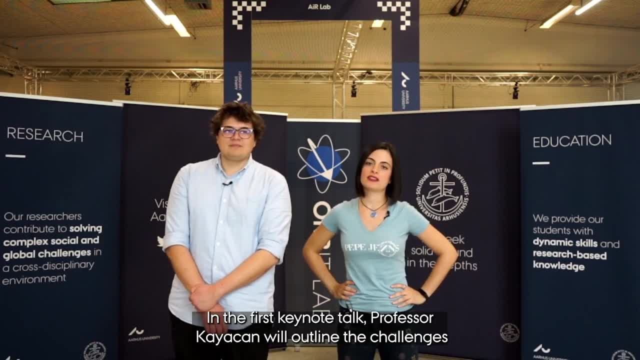 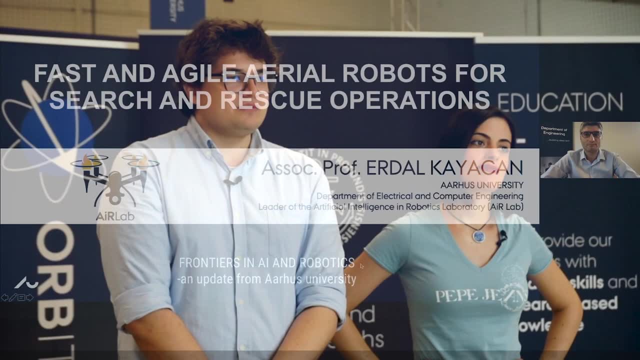 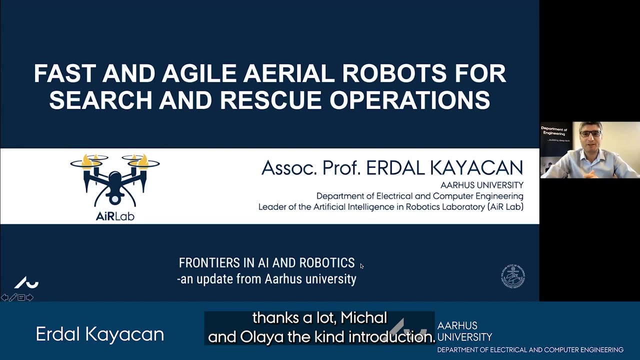 many domains. one of those is search and rescue operations. in the first keynote talk, Professor kaya Jan will outline the challenges and opportunities of fast and agile flights for drones. hi, I'm Erdal kayajan. thanks a lot Mihail and Olaya for the kind introduction. today I will talk about fast and agile aerial robots for 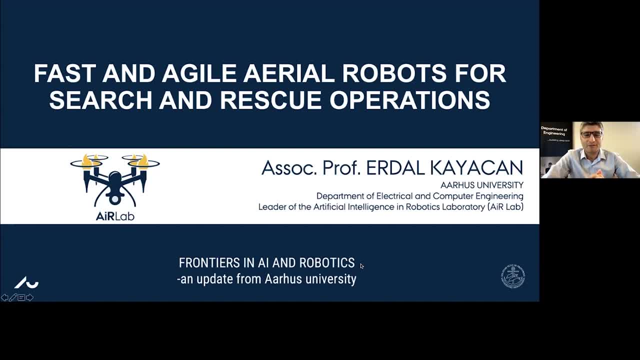 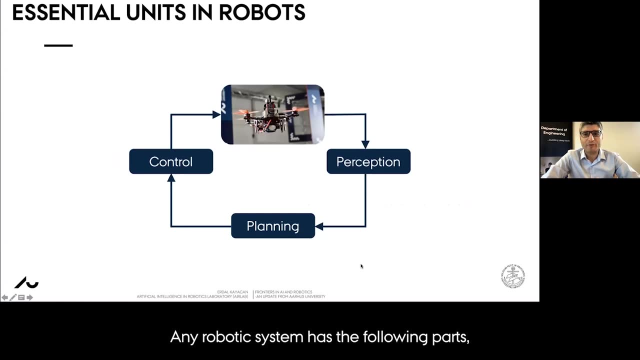 search and rescue operations, and this research is the outcome of our research activities at air lab at Aarhus University. any robotic system has the following parts, which are control, perception and planning. human beings move with the similar blocks as well. for instance, when we go into a dark room, the first thing we have to do is to switch on the lights. this is for our perception. 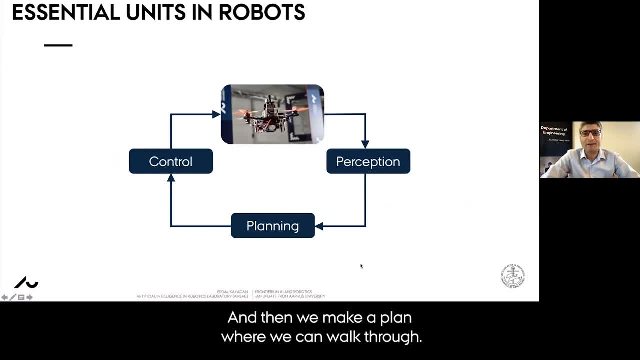 system, because we have our own eyes, and then we make a plan where we can walk through. we want to avoid obstacles. this is the planning part, and this is done by our brain, and the last is execute the task, which is done with our muscles, and this is also controlled by. 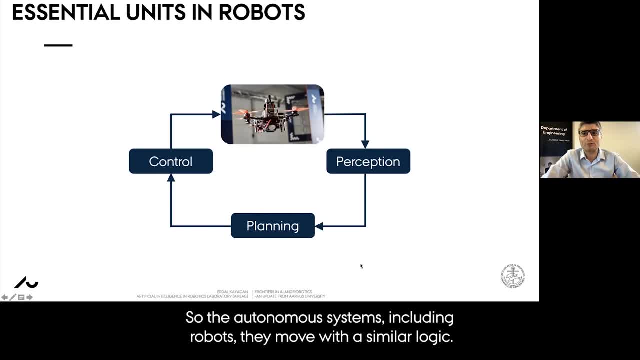 our brain, so the autonomous systems, including robots. they move with a similar logic, but in the recent years there is the advancements of artificial intelligence and computation power for the robots outer loop. in our outer loop there is one block which is called learn. so we want our robots to. 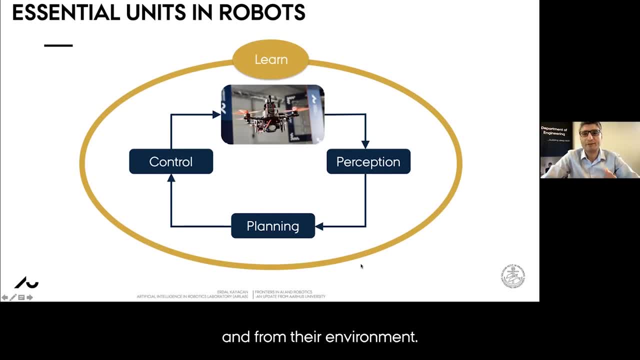 learn from their background and from their environment. and there is the second block, which is understand, so we want them to understand their environment. the third block is interact: we want them to interact with their environment. and the last is to adapt, so we want our robots to adapt to their environment and recent AI methods, including deep neural, 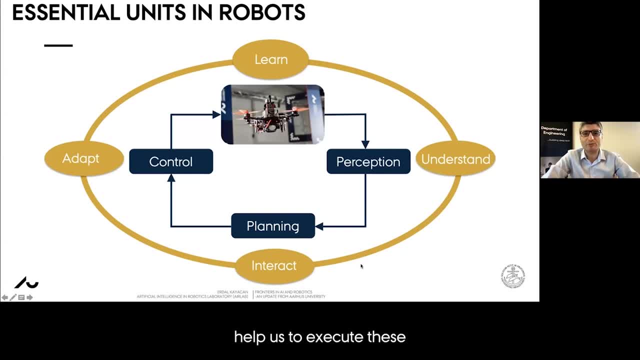 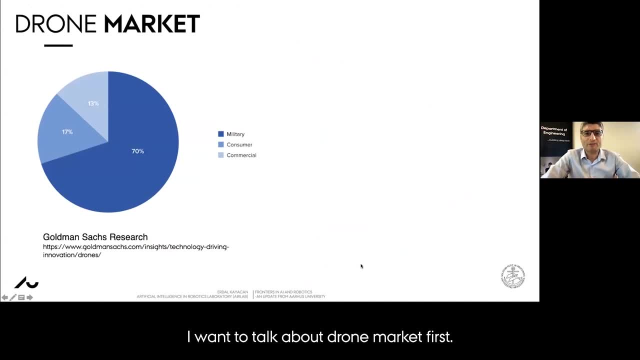 networks help us to to execute these tasks in the in the outer loop. I want to talk about drone market first. so far, most of the funding was spent for military drone market but but changing so day by day we are seeing more and more consumer and commercial drone applications. 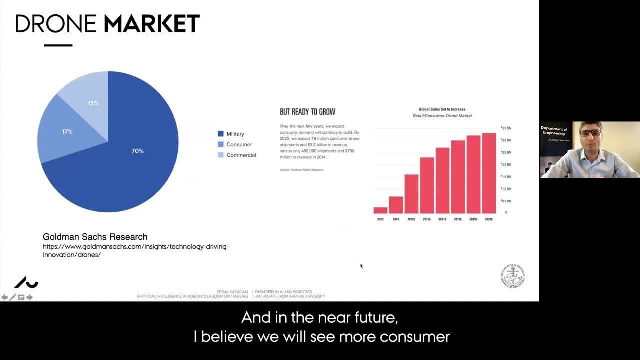 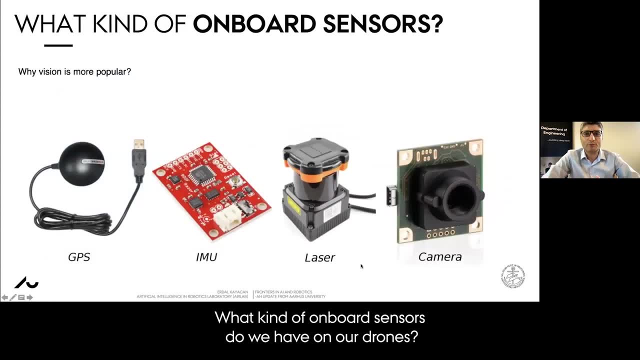 and in the near future, I believe we will see more consumer and commercial drones in the markets. what kind of onboard sensors do we have on our drones? first of all, we have the GPS global positioning system and we have IMU, we have laser and we have camera. 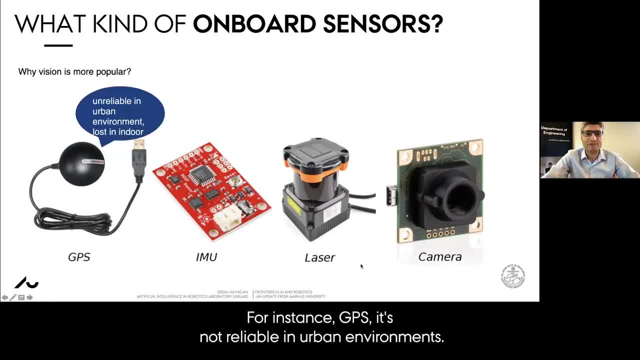 some of them have some drawbacks, for instance, GPS. it's not reliable in Urban environment, what we call is a shadow effect. when you have tall buildings, there is a shadow effect and the accuracy of GPS is going down. and in indoor environment we don't have GPS at all. we have 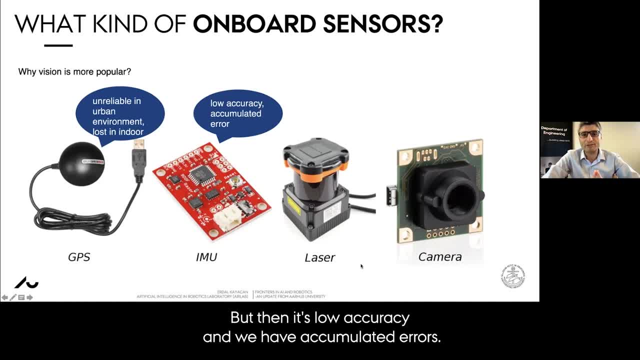 the IMU, but then it's a low accuracy and we have accumulated errors. so when we use IMU for for positioning um to to measure the position of the robot, it is subject to accumulated errors. we have 2D and 3D laser scanners, but they are heavy and they are expensive. so the rest of the sensors. 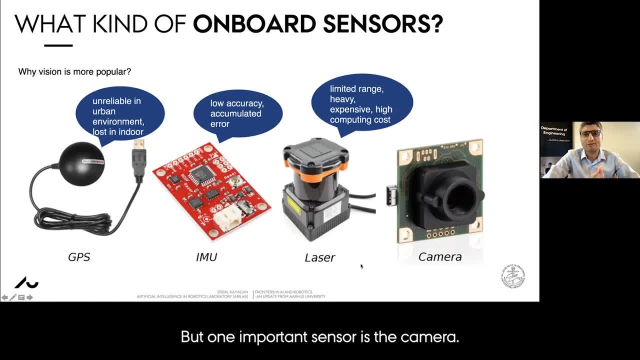 I'm not mentioning them, but one important sensor is the camera. so the cameras don't have these uh drawbacks. they are reliable in indoor and outdoor environment, They don't consume lots of energy, They are accurate enough and they are cost effective. So all these positive properties of cameras make them really advantageous for our applications. 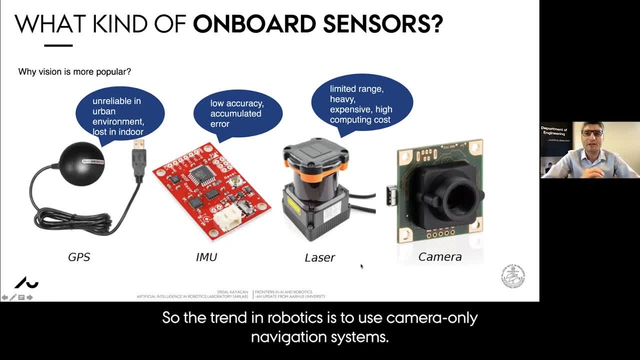 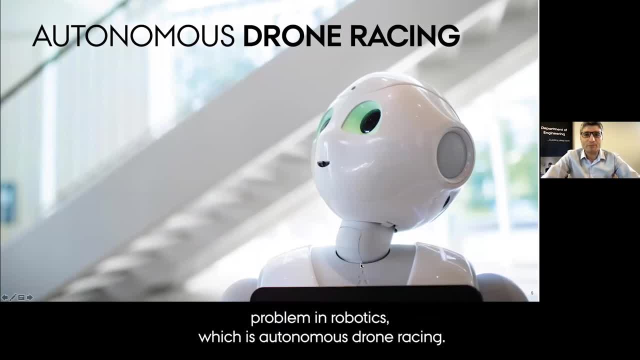 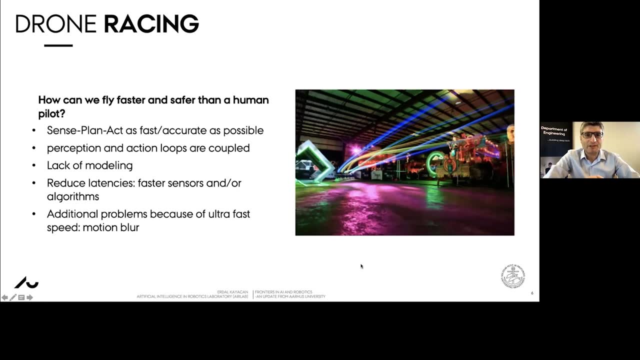 So the trend in robotics is to use camera only navigation systems. I want to talk about a very interesting research problem in robotics, which is autonomous drone racing. So the question in this problem is whether we can fly faster and and safer than a human pilot. 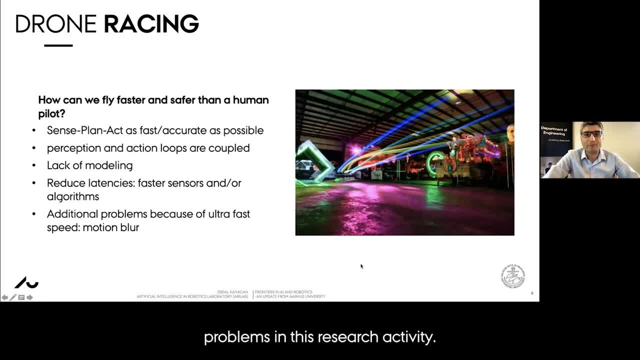 There are some serious problems in this research activity. For instance, we have lack of modeling. So when the drones move really fast, their dynamic models are subject to some internal and external noises and uncertainty And there is lack of modeling. The second problem is, since they are flying so fast, we have to reduce the latencies. 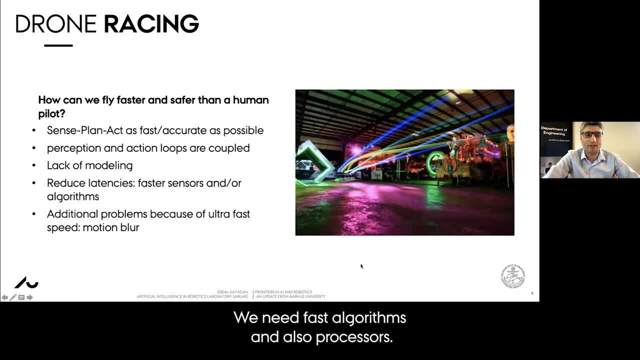 So we need fast sensors, We need fast algorithms and also processors. And one interesting additional problem is the motion blur. So when the drone moves so fast, there is motion blur on the camera And the features coming from the camera are disturbed. 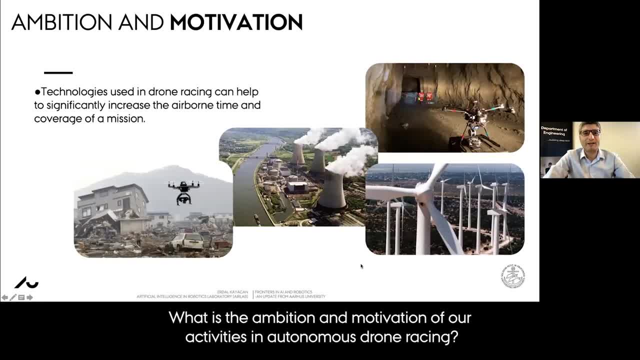 What is the ambition and motivation of our activities in autonomous drone racing? Is it just a game? Of course it's not just a game. We assume that the technologies used in autonomous drone racing can help to significantly increase the airborne time and coverage of a mission. 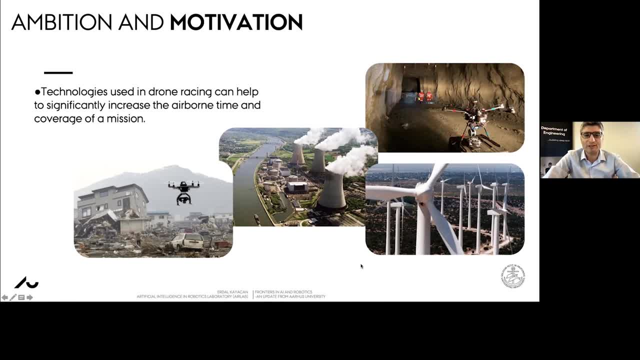 And this. these technologies can be used in Underground mining operations, help people after an earthquake or maybe even a nuclear power plant accident. In all these applications, the environment, the map of the environment, is either inaccessible or corrupted. So the drone has to map its environment very fast and then it has to plan very fast and execute very fast. 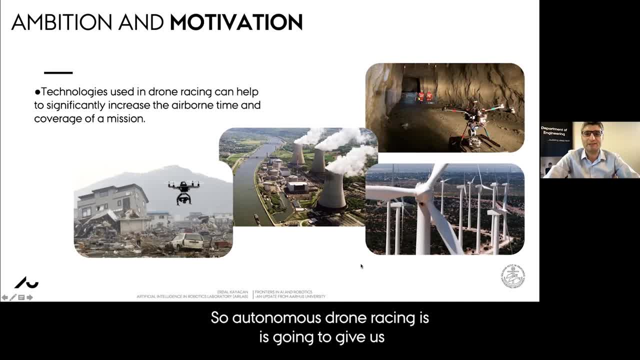 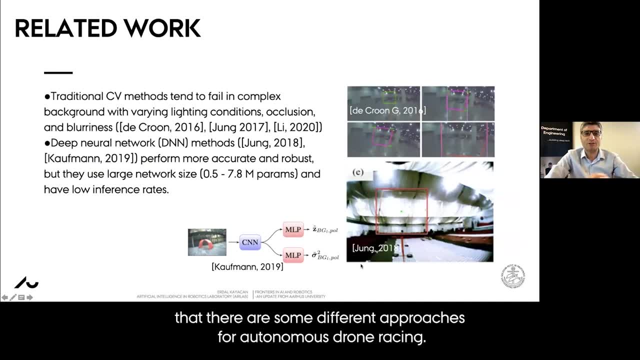 So autonomous drone racing is going to give us this opportunity to develop these technologies. We have checked the literature that there are some different approaches for autonomous drone racing. There are some traditional computer vision methods But when we change the background or the gate geometry these methods tend to fail. 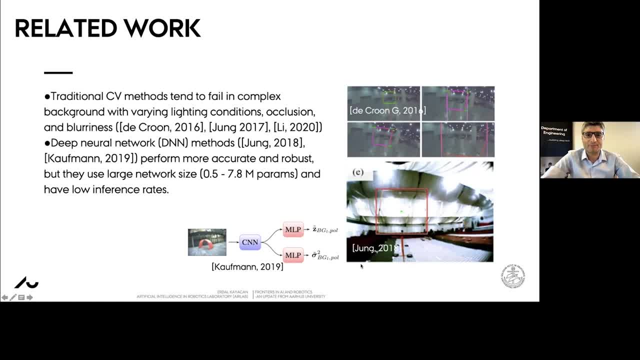 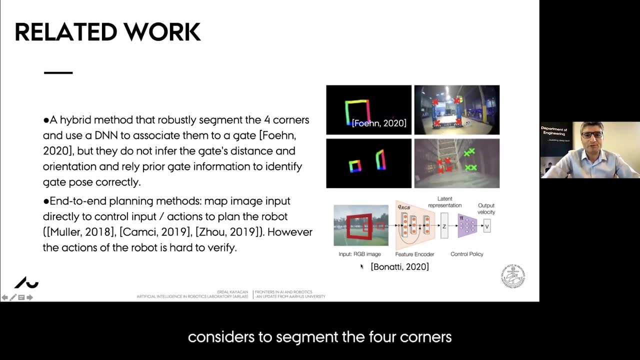 There are some deep learning based approaches And they are really big size and they have a couple of million parameters to tune. There are some hybrid methods. For instance, one paper considers to segment the four corners and then use a deep neural network to associate them to a gate. 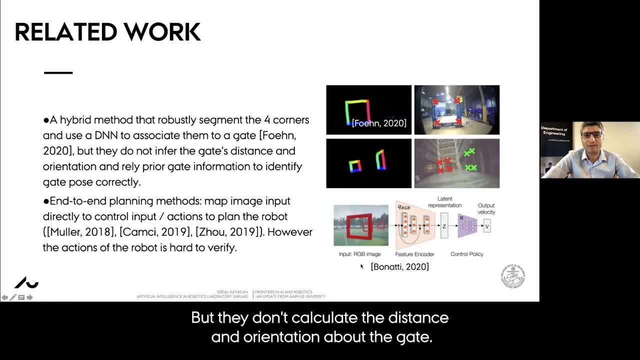 But they don't calculate the distance and orientation about the gate. There are some end to end planning methods where the input is the raw sensor input and the output is the robot action. When they work, nice, Yes, they are really nice methods. But when the method fails, it's really difficult to find where the error is. 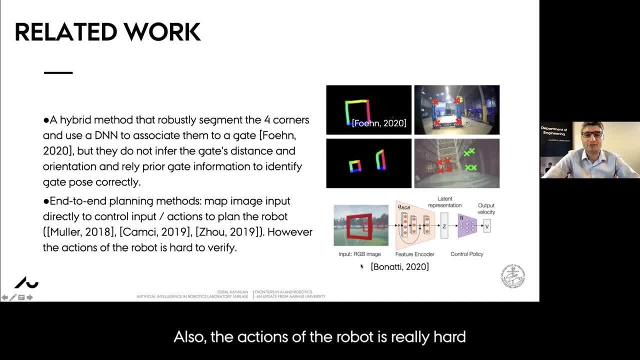 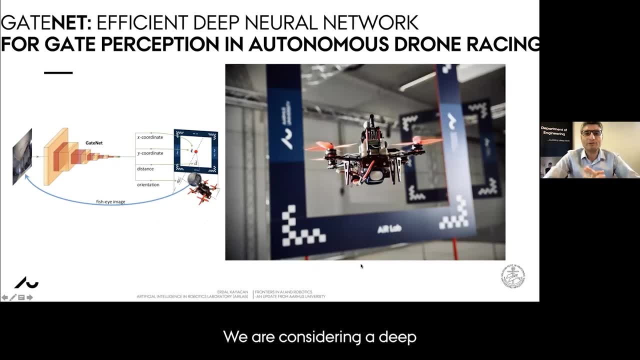 So also the actions of the robot is really hard to modify, verify. We are considering A deep neural network based approach for the perception problem. We are estimating the X and Y coordinate of the gate, distance to the gate and orientation to the gate. 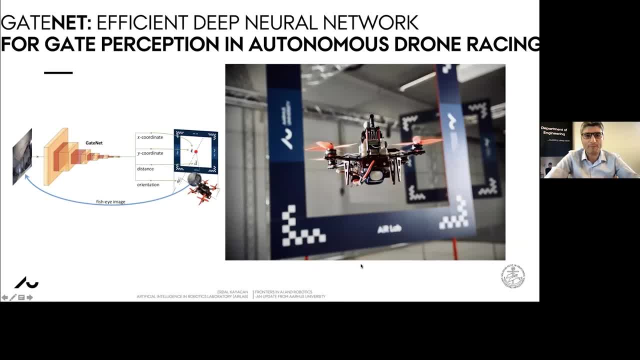 Of course, distance and orientation are relative to the drone. One interesting approach from our group is the use of fisheye image. I want to explain why we want to use fisheye images, fisheye lens. This is because in real life, the obstacles are pretty close to each other. 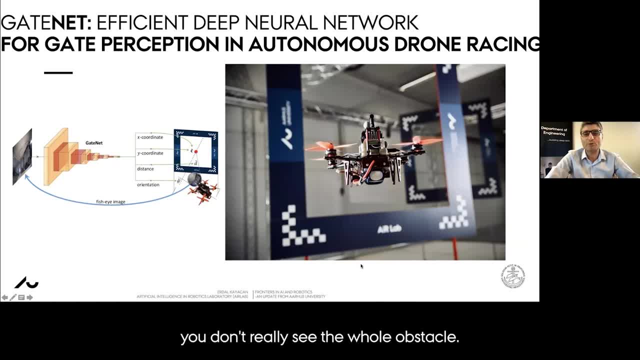 And when you use a standard lens, most of the time you don't really see the whole obstacle. For instance, for our gate In our lab we have placed the gates which is closer to each other And then when we use fisheye lens we have a better field of view and then we can see them. 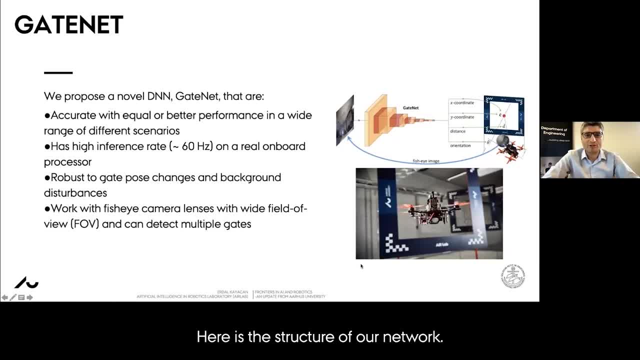 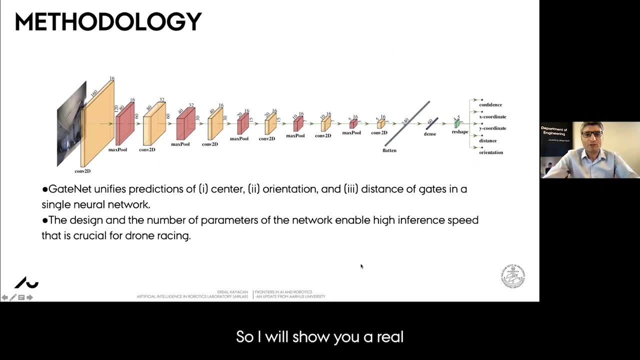 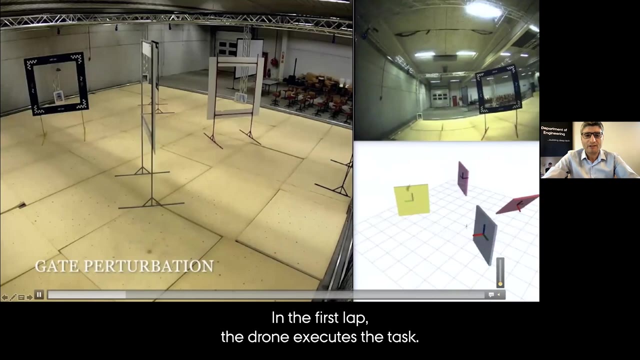 Here is the structure of our network. And our network is able to run on onboard computer with almost 60 hertz inference rate. So this is the methodology. So I will show you a real world results. In the first lab the drone executes the task. 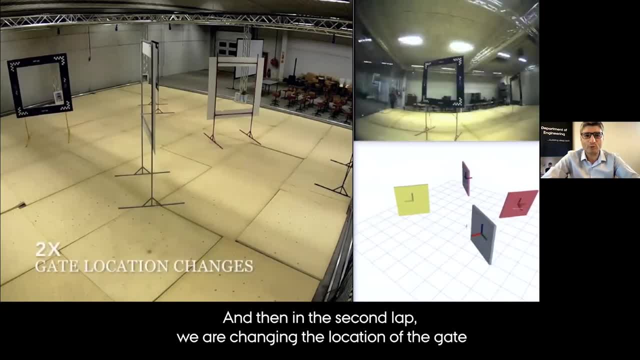 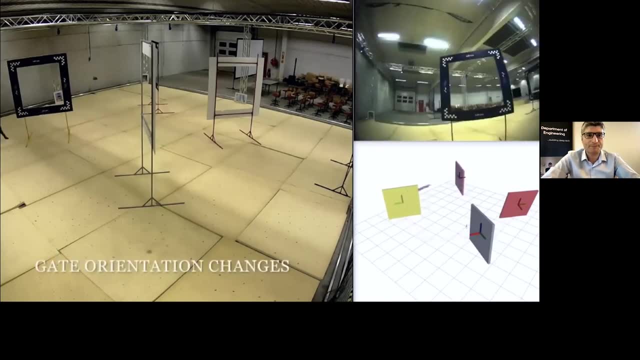 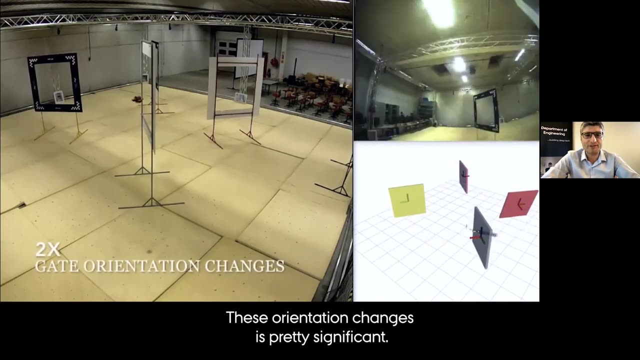 And then in the second lab we are changing the location of the gate. That we show our method is robust to background changes. Once we are successful, then we change the orientation of the gate. This orientation changes is pretty significant. It's almost 35 degrees. 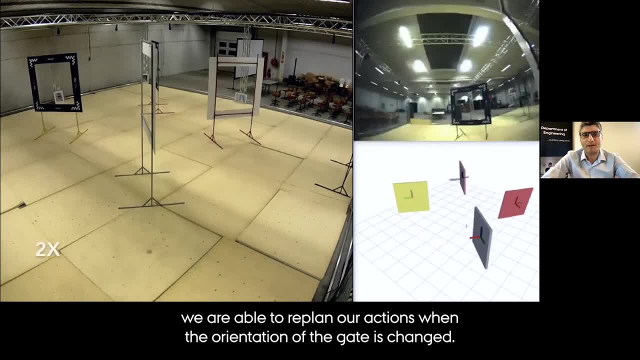 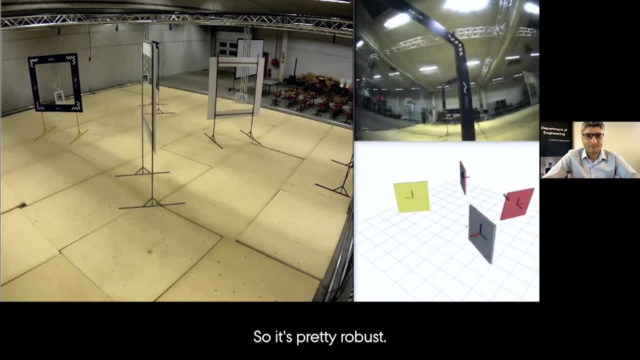 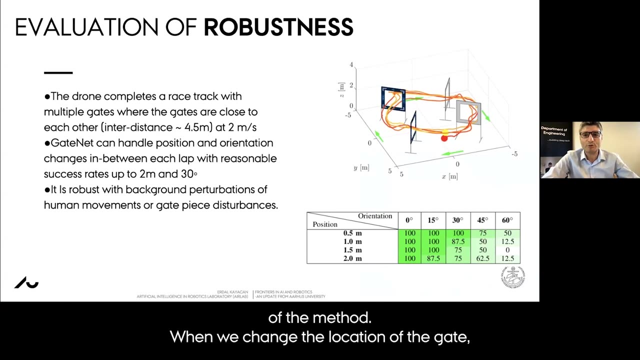 So we also change that. we are able to replan our actions when the orientation of the gate is changed. So it's pretty robust. We have also evaluated the robustness of the gate. When we change the location of the gate, the accuracy is not disturbed at all. 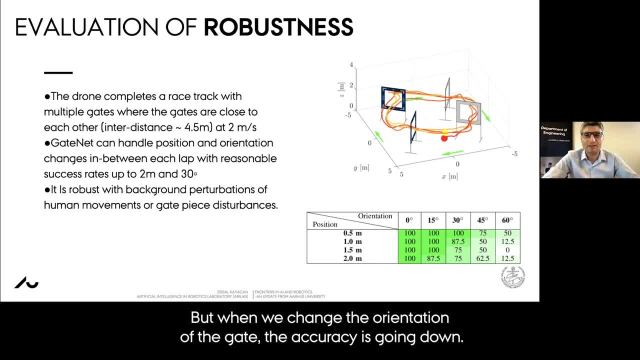 But when we change the orientation of the gate, the accuracy is going down. This is pretty expected, I think, Because when we change the orientation of the gate to 90 degrees, nothing is visible on the gate, And when you make it, let's say, 45 degrees, you can see only half of the pixels on the screen. 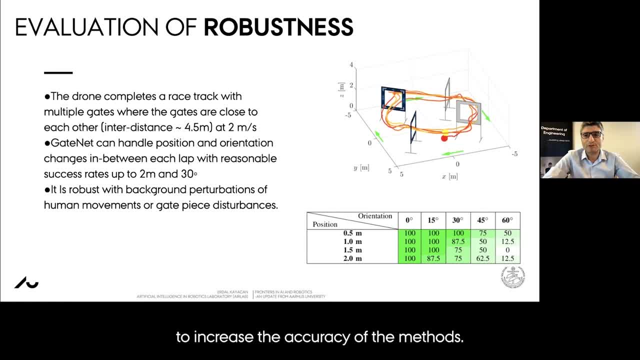 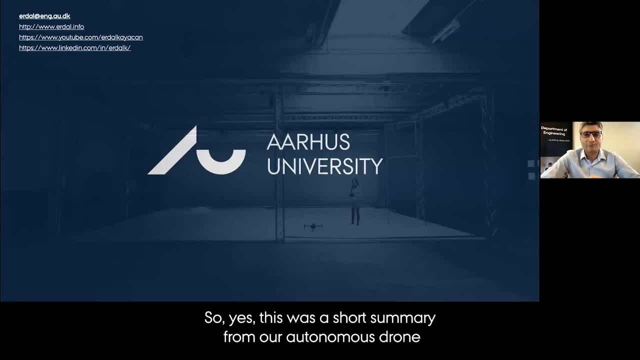 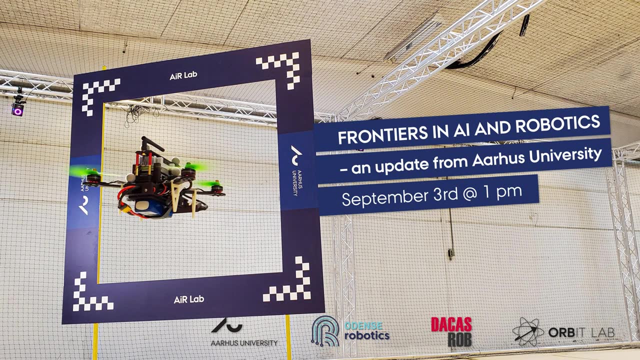 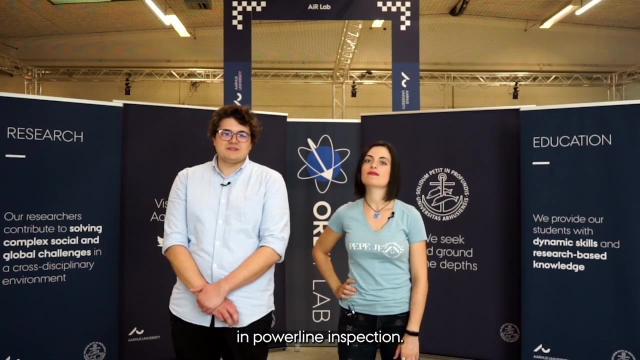 Of course, there are some methods to increase the accuracy of the method. So, yes, this was a short summary from our autonomous drone racing research activities And thanks a lot for your time. Powerline inspection is dangerous for human workers. Drones can be a cost-effective solution to reduce the accident risk in powerline inspection. 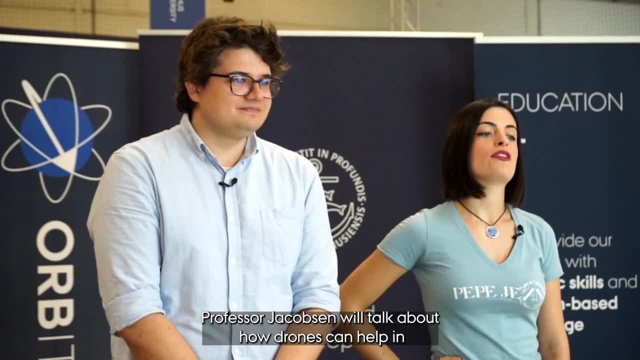 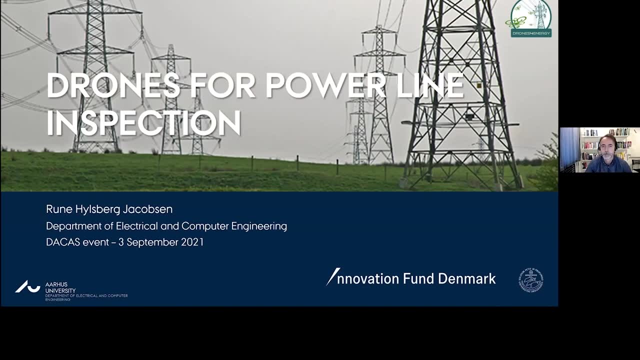 We believe that they will play a vital role in the future. Professor Jacobsen will talk about how drones can help in powerline inspection tasks. Hello, my name is Rune Hulsberg Jacobsen. I'm associate professor at Aarhus University in Denmark. 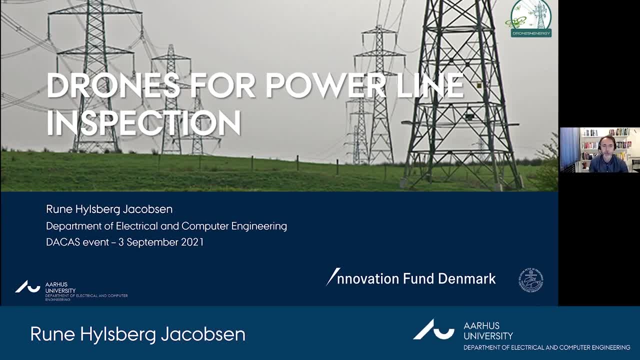 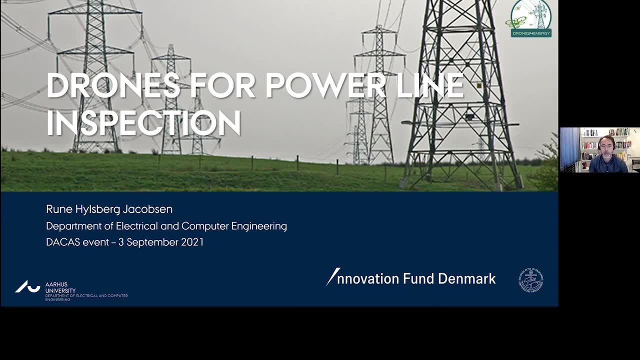 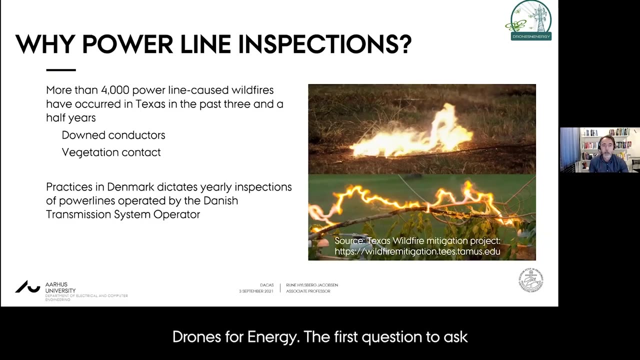 I work with the Department of Electrical and Computer Engineering. I would like to give you a brief insight into an appealing application of autonomous swarming drones for powerline inspection. We work with this use case in the Innovation Fund project Drones for Energy. The first question to ask is: why are powerline inspections of interest for drones? 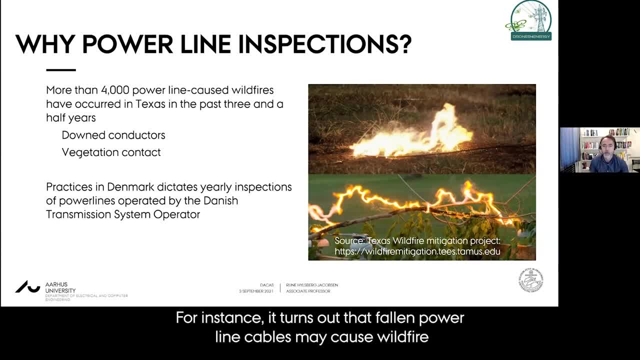 For instance, it turns out the fallen powerline cables may cause wildfire from downed conductors or conductors in contact with vegetation. In Texas alone, more than 4,000 incidences of fire have been caused by broken powerlines during the past three and a half years. 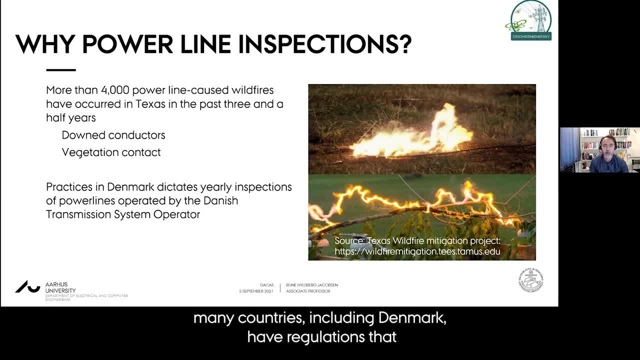 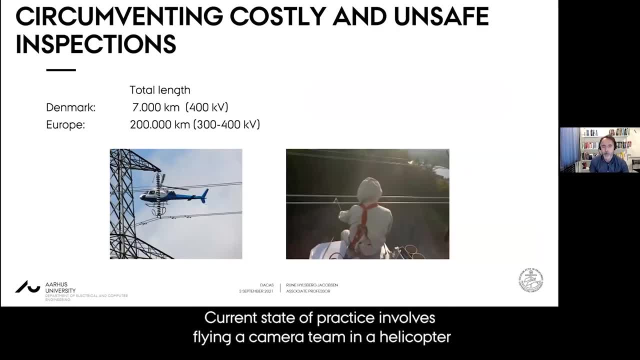 Because of the safety concerns, many countries, including Denmark, have adopted regulations that demand continuous inspection of powerline infrastructure. Current state of practice involves flying a camera team in a helicopter alongside with the powerlines or manually climbing on the cables. These operations are costly and pose high risk to the inspection team. 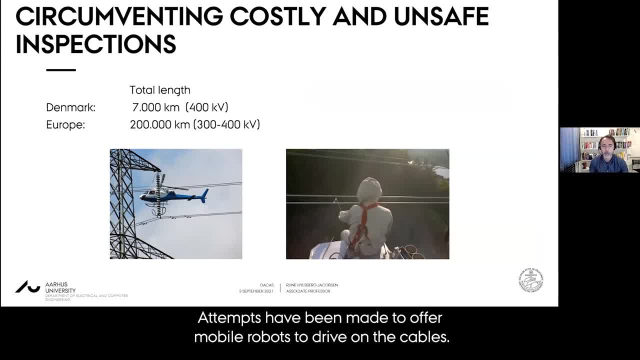 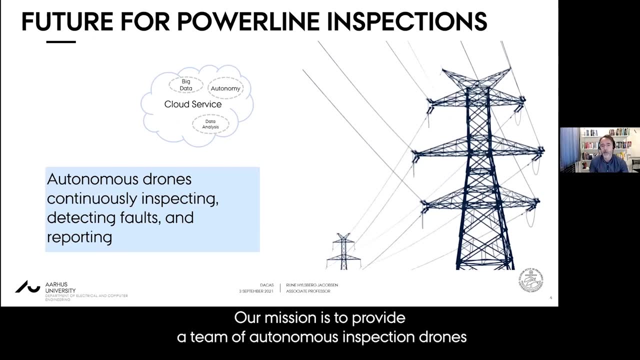 Attempts have been made to offer mobile robots to drive on the cables. Such robot needs to be attached to the powerlines and manually shifted from one segment of line between two pylons to the next. Our vision is to provide a team of autonomous inspection drones that would live on the cables, continuously inspecting, detecting faults and reporting to the operating organization. 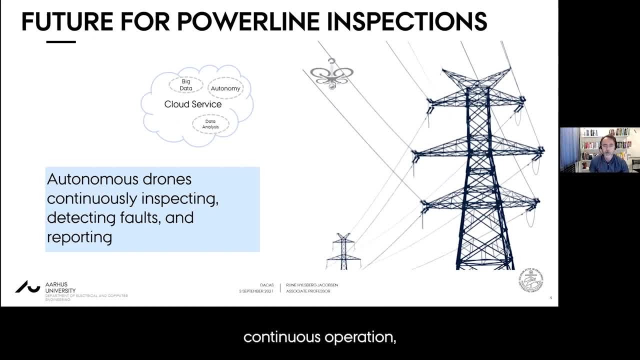 To enable this continuous operation, drones will harvest energy from the powerlines using inductive coupling. We implement a gripping mechanism where the drone can climb on the cables And then grab onto the cable and harvest. We deploy a team of autonomous collaborating drones for the inspection. 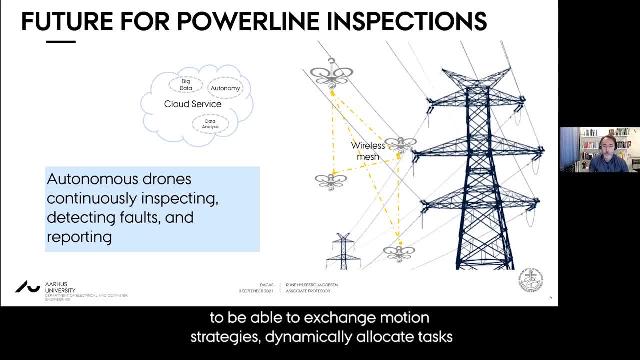 Drones form a wireless mesh network to be able to exchange motion strategies, dynamically allocate tasks and share data. To monitor the inspection mission continuously, we use long-range radio communication for control and telemetry of individual drones. Cloud services are provided. They provide information services to the team and act also as a repository for the inspection images. 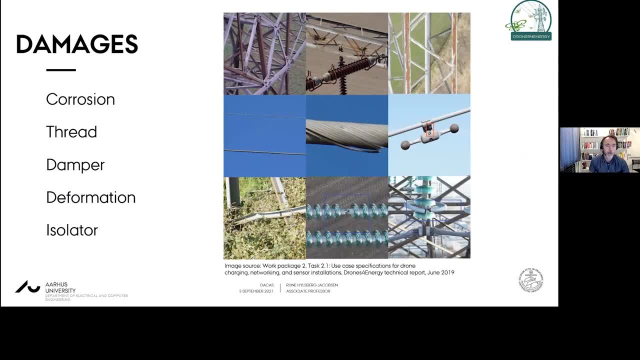 Examples of the faults that we are looking for are corrosion, loose threads, broken dampers, deformation in the infrastructure, such as the pylons. This may be a farming machine that has crashed into the pylon, for instance. Or we look for broken insulators. 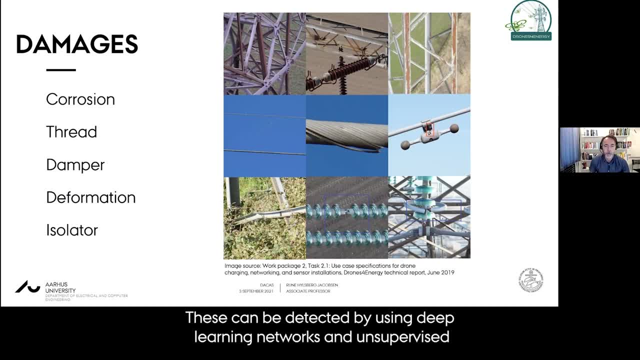 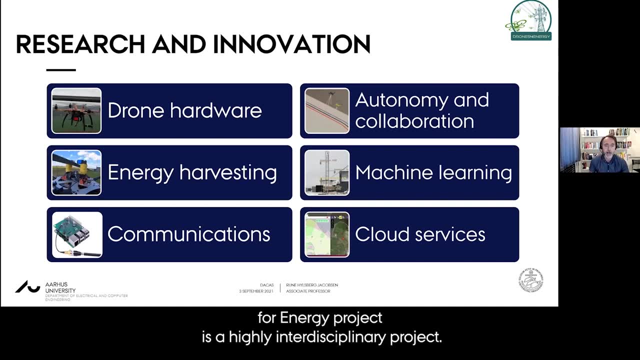 These can be detected by using deep learning networks And unsupervised learnings. The Drones for Energy project is a highly interdisciplinary project. It involves drone hardware development, Energy harvesting technology, Wireless communication and networking Algorithms for autonomous operations and collaboration. 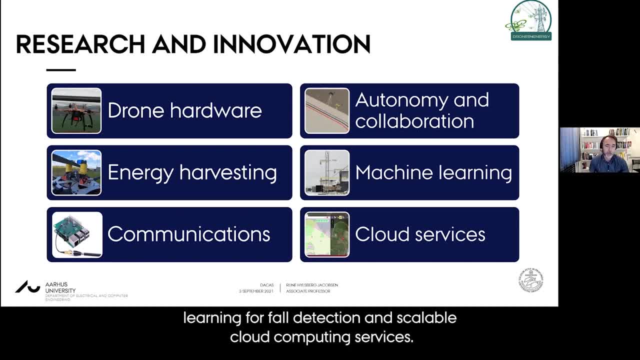 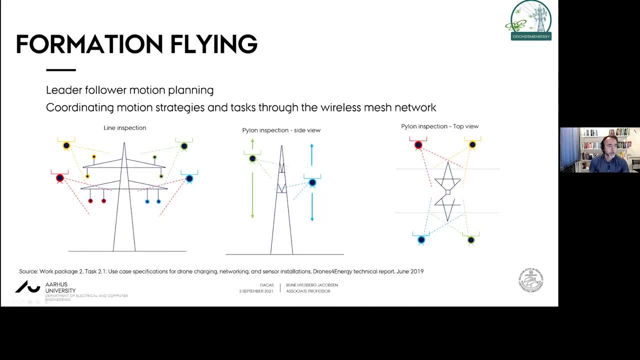 Machine learning for fault detection And scalable cloud computing services. With this innovation, We can significantly decrease the cost of an inspection operation, while providing also better safety for the operators involved. To give some examples: For instance, by flying in a formation, this could lead to an increased efficiency of the mission operation during the inspection time. 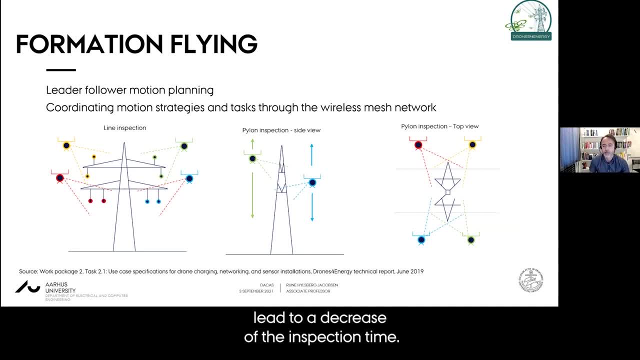 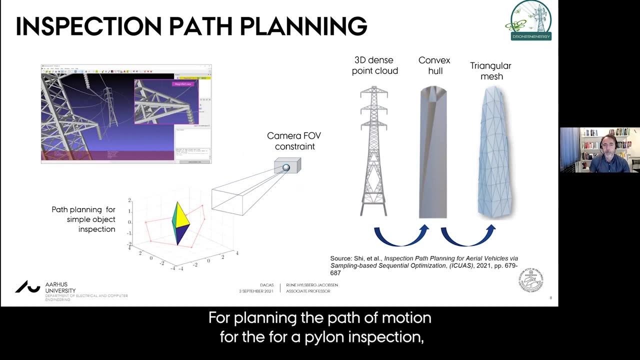 And it will lead to a decrease of the inspection time. Formation flying would also mitigate the problem of the need of flying under the cable, which is not permitted today. For planning the path of motion for a pylon inspection, for instance, We take a 3D model to calculate the optimal inspection path for the drones. 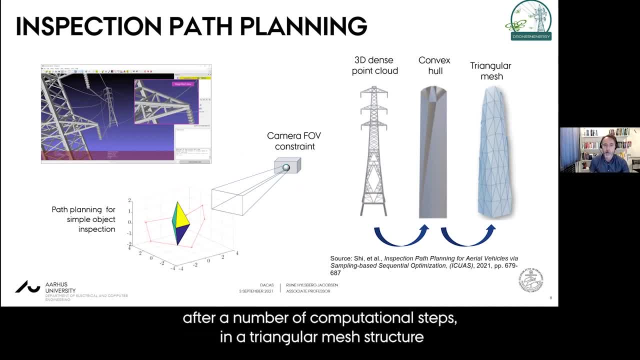 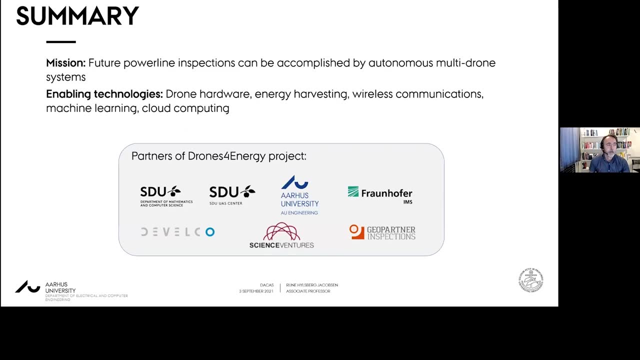 The 3D model is created from a point cloud And results, after a number of computational steps, in a triangular mesh structure From which the optimal viewpoints can be calculated, Taking into account the camera and the safety constraints. The drones for energy project is carried out by a strong consortium of partners. 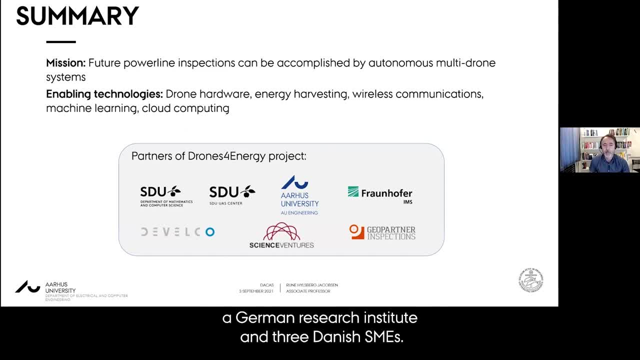 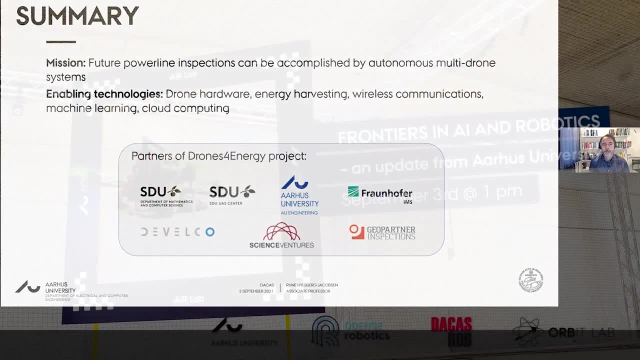 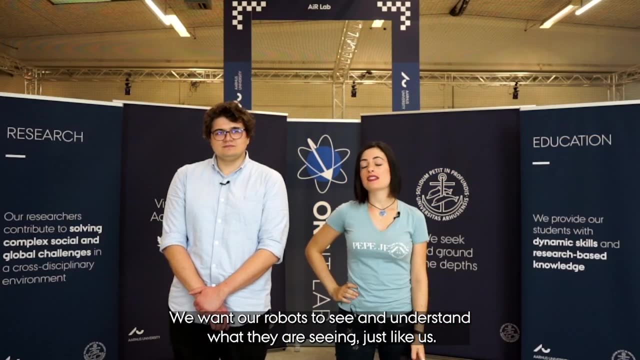 Including two Danish universities, A German research institute And three Danish SMEs. Thank you for listening. We want our robots to see And understand what they are seeing, Just like us. Thanks to computer vision, Our robots can now perceive the world. 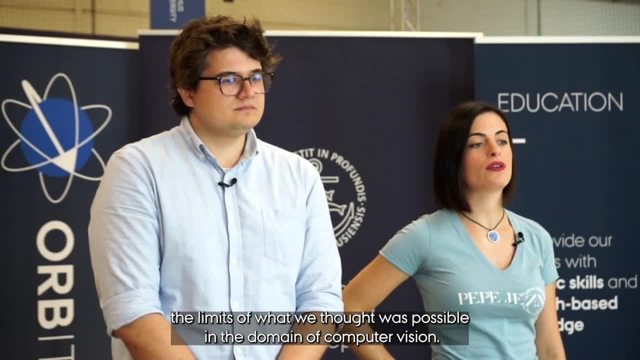 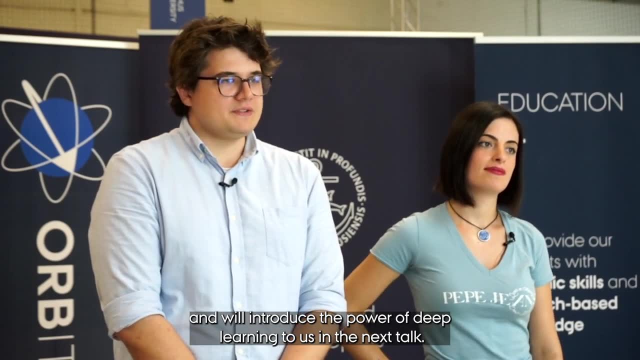 Deep learning has pushed the limits of what we thought was possible in the domain of computer vision. Professor Iosifidis is an expert in the field And will introduce the power of deep learning to us in the next talk. Hello, my name is Alexandros Iosifidis. 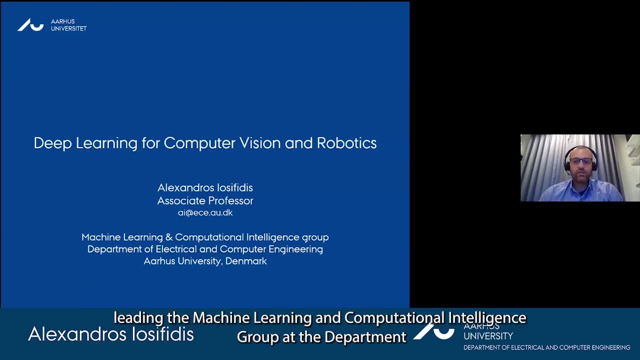 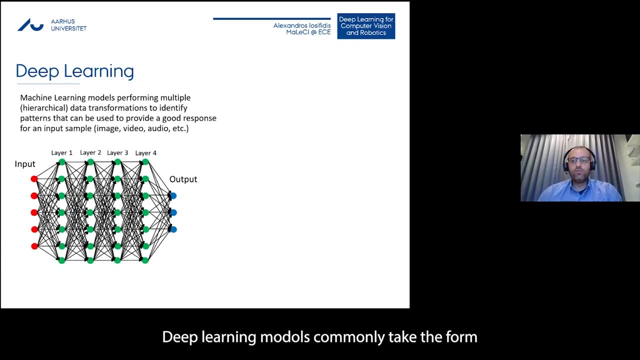 And I am an associate professor leading the machine learning and computational intelligence group At the department of electrical and computer engineering at Aarhus University. Deep learning models commonly take the form of artificial neural networks Which can receive as input data And perform successive data transformations. 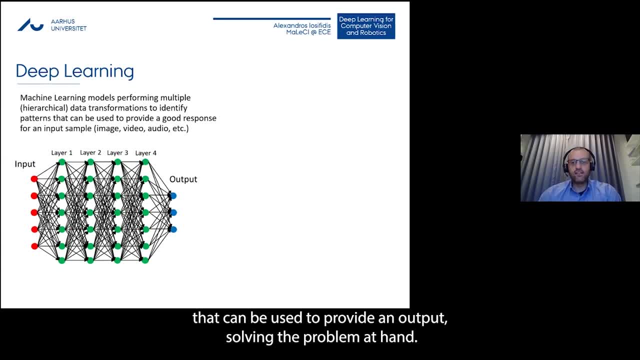 In order to identify patterns in the data That can be used to provide an output solving the problem at hand. In this figure, each of the cycles corresponds to a processing unit called neuron, Which receives as input an input Processes it to detect a pattern. 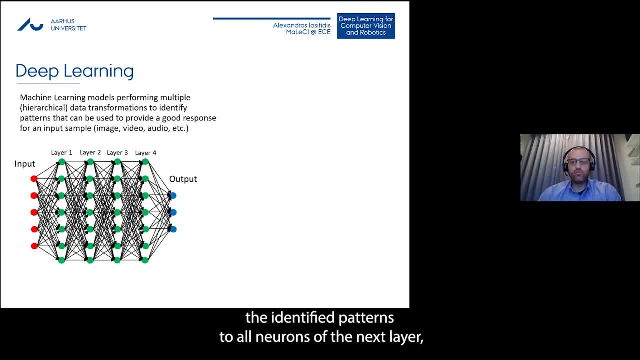 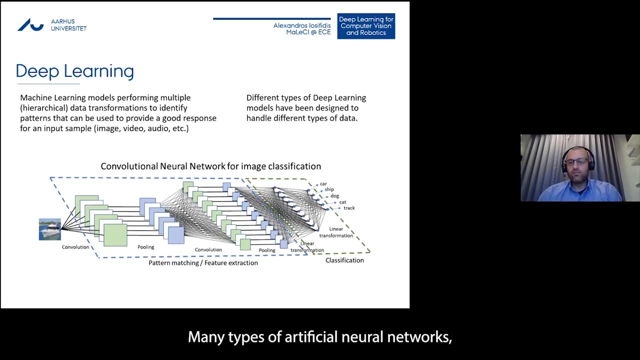 And forwards the identified patterns To all neurons of the next layer Which are connected to it. By optimizing all these hierarchical data transformations jointly, Deep learning models can achieve impressive performance in a wide range of applications. Many types of artificial neural networks formed by different types of neurons. 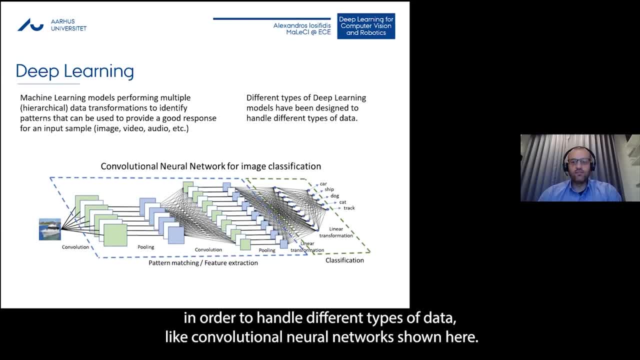 Have been designed in order to handle different types of data. Like convolutional neural networks shown here, This neural network can receive as input an image And transform it to multiple images In a hierarchical process, Each of which can be seen as a detector of a specific pattern or feature. 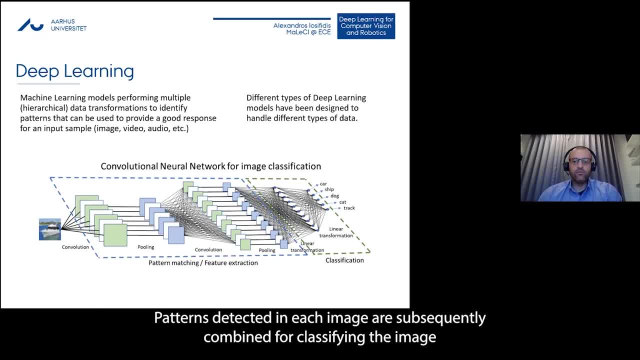 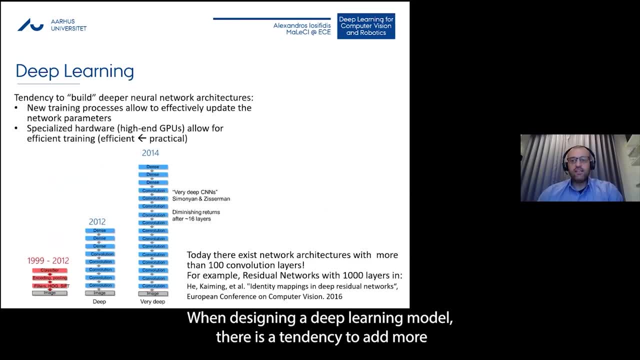 Patterns detected in each image are subsequently combined For classifying the image in one of the specified categories. When designing a deep learning model, There is a tendency to add more and more layers, Leading to a very deep neural network architecture Nowadays, due to recently proposed effective training methods. 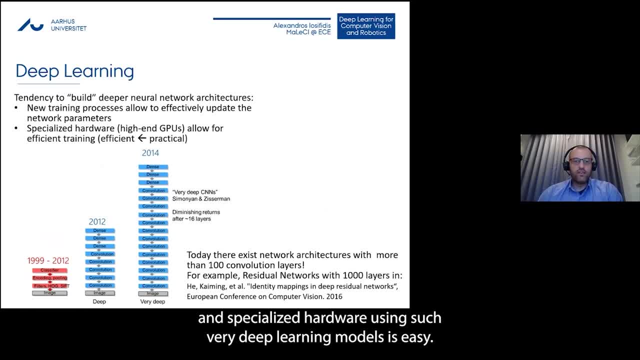 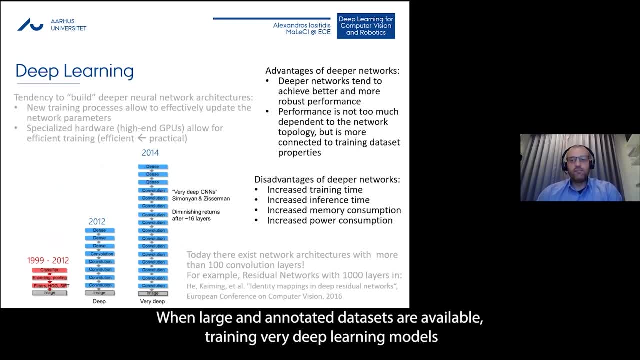 And specialized hardware. Using such very deep learning models is easy When large and annotated data sets are available. Training very deep learning models is usually sufficient to achieve high performance. However, the use of such very deep learning models Leads to long training and inference time. 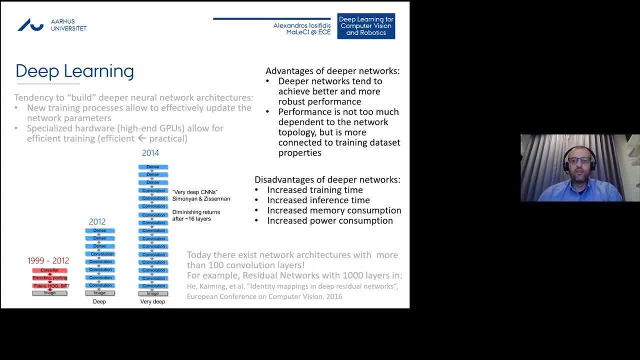 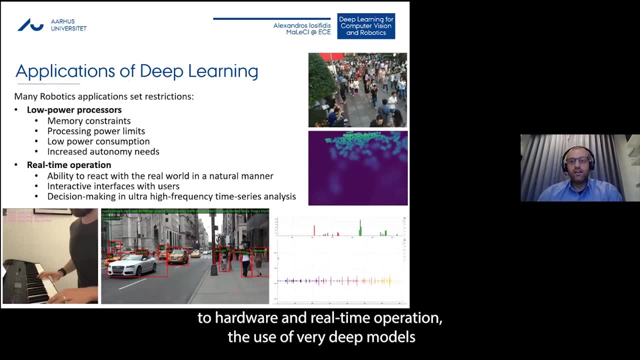 And high memory and power consumption In robotic applications, Setting restrictions with respect to hardware and real-time operation. The use of very deep learning models is not practical. This is due to the low memory and processing power of the adopted processors And the increased need for autonomy for a long period. 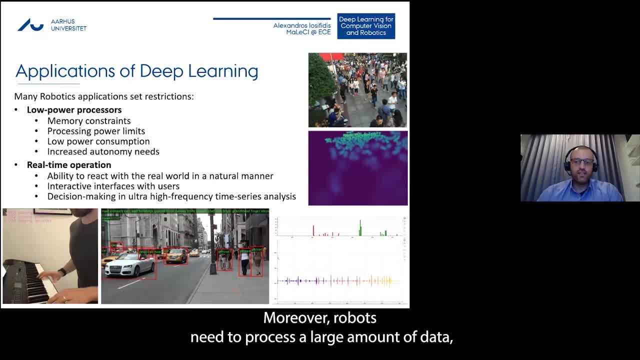 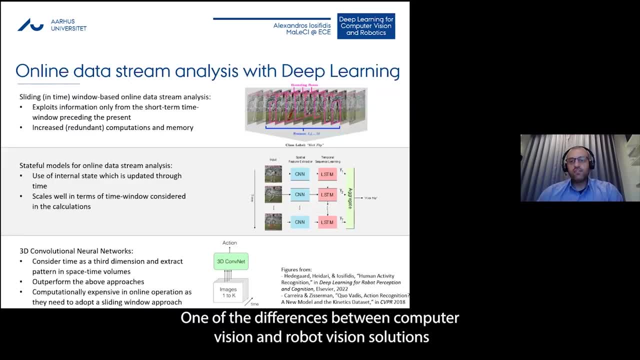 Moreover, robots need to process a large amount of data, Make decisions and react within their environment in real time. One of the differences between computer vision and robot vision solutions Is that the latter needs to process the incoming visual stream in an online manner And lead to actions in real time. 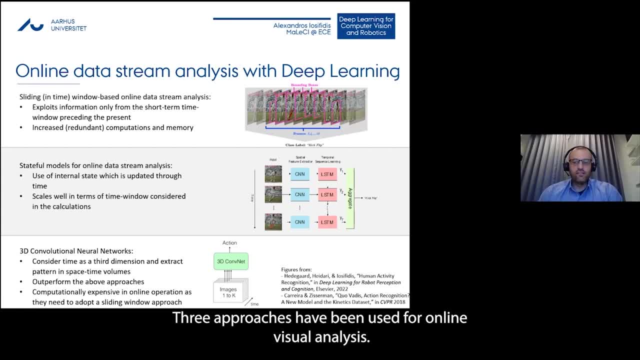 Three approaches have been used for online visual analysis. The use of sliding window or video frames Allows exploiting information from the short-term time window preceding the present, But it leads to high computations. This issue is addressed by using deep learning models Which can update their state over time. 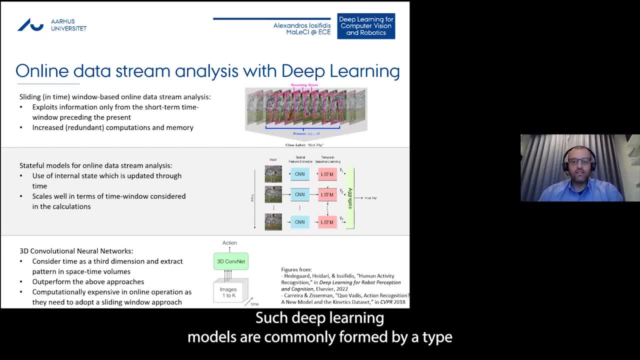 Such deep learning models are commonly formed by a type of recurrent neural networks And can lead to real-time operation, But they cannot reach the performance levels achieved by 3D CNNs, Which consider the time as a third dimension And process multiple video frames jointly. 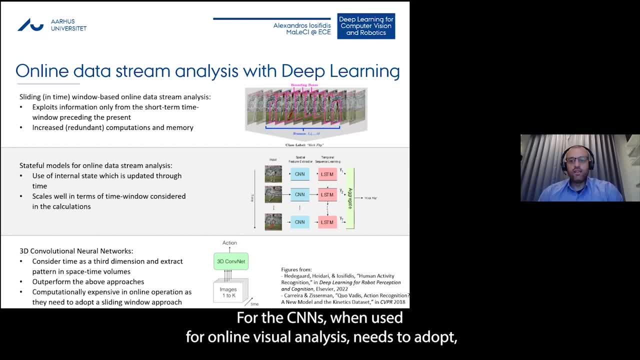 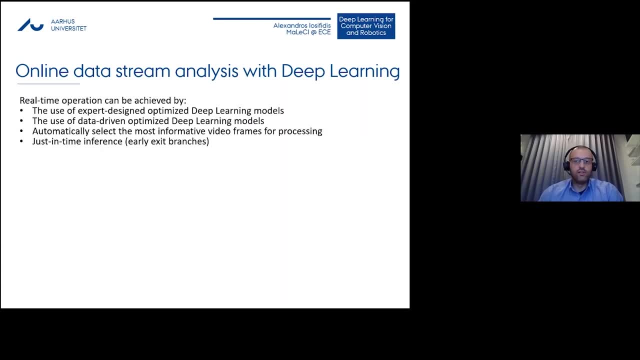 3D CNNs, when used for online visual analysis, Need to adopt the sliding window approach, Leading to a high computational cost. To achieve real-time in online data analysis problems, One can try to design efficient deep learning models. These models can be designed by a human expert. 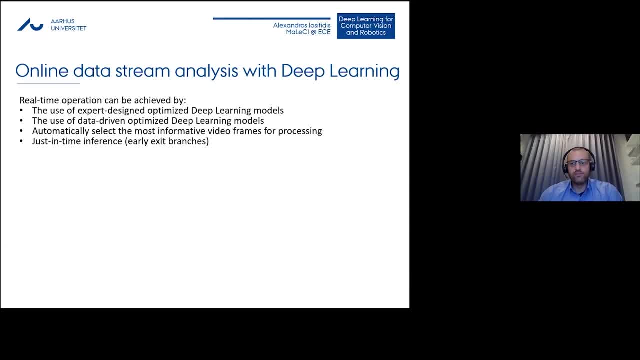 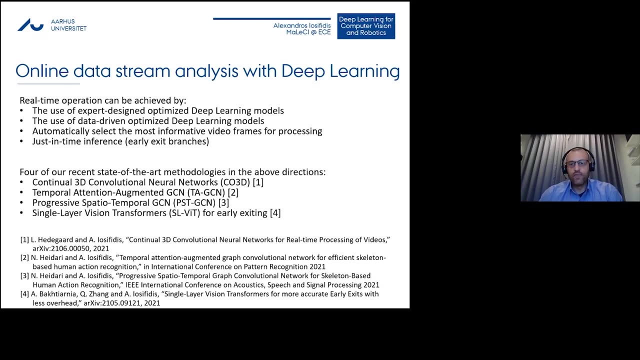 Or by following a data-driven optimization process. One can also automatically select a subset of the most informative video frames to process, Or to perform calculations on each video frame, Depending on time constraints. We have proposed methodologies that follow each of these directions In achieving real-time operation. 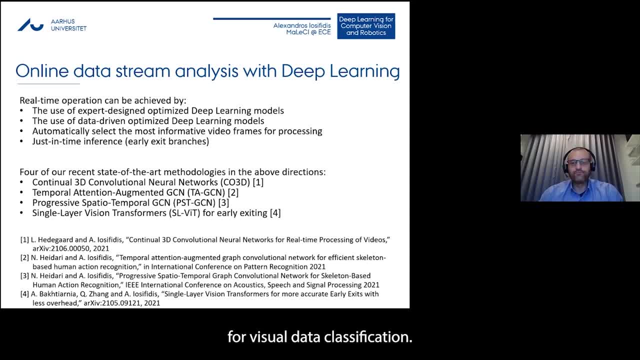 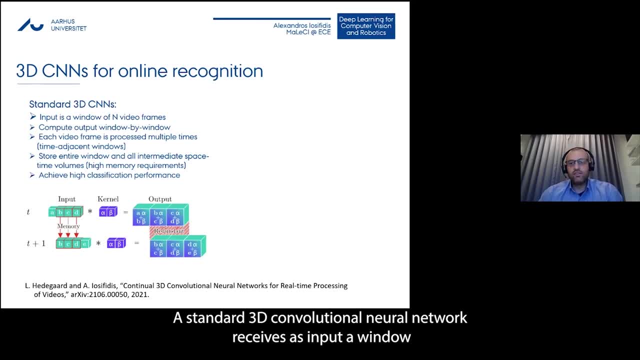 Based on deep learning models for visual data classification. Our first methodology redefines the operation of 3D convolution. A standard 3D convolutional neural network receives as input a window formed by multiple video frames. When it is applied in online visual analysis, 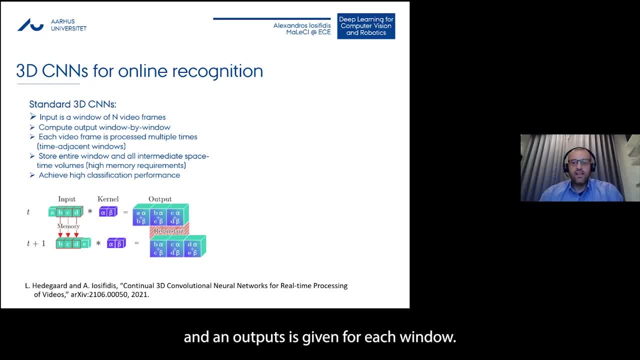 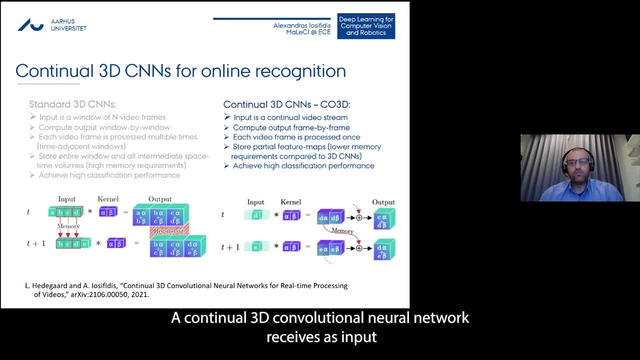 Multiple overlapping windows or video frames are processed And an output is given for each window. A continuous 3D convolutional neural network receives as input A continuous video stream And computes an output for each video frame. This means that each video frame is computed once. 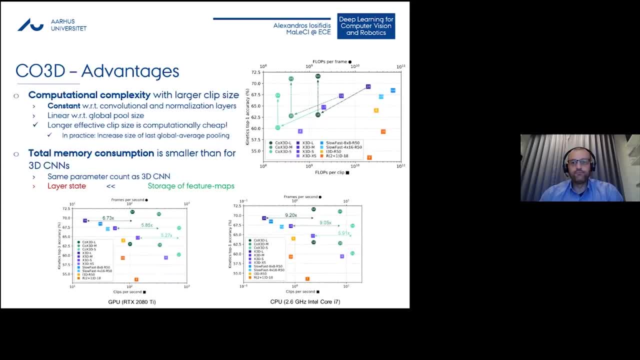 Which speeds up the processing considerably. The gains achieved by using our continuous 3D CNNs Reached a reduction in the number of computations of one order of magnitude, Leading to a speed up of up to 6.7 times when using CPU. 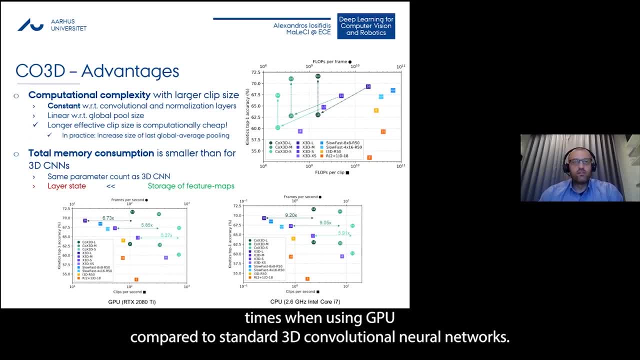 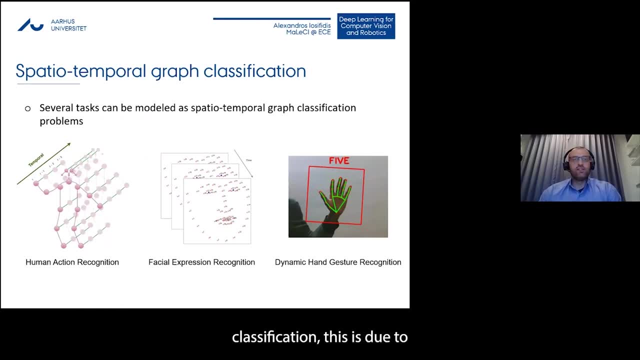 Or 9.2 times when using CPU, Compared to standard 3D CNNs. A problem of particular interest is that of spatiotemporal graph classification. This is due to that several tasks can be modeled by using graph structures, For example, by applying a human body skeleton detection method. 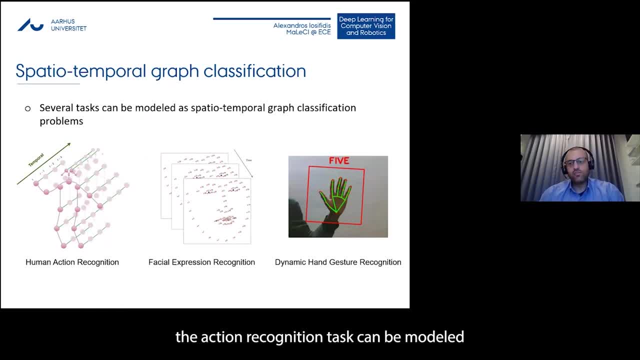 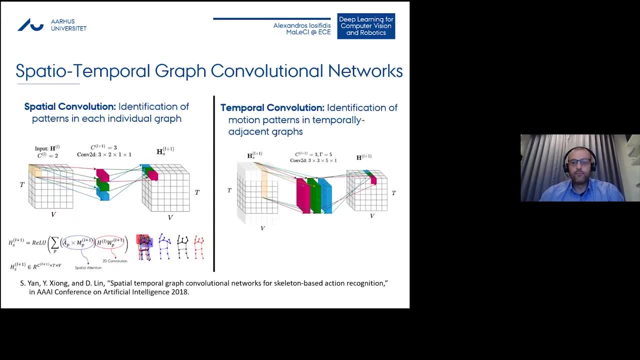 And calculating the human body poses. The action recognition task can be modeled as the classification of human body poses evolving over time. A type of deep learning model that is suitable for handling spatiotemporal neural networks Is the spatiotemporal graph- convolutional neural network. 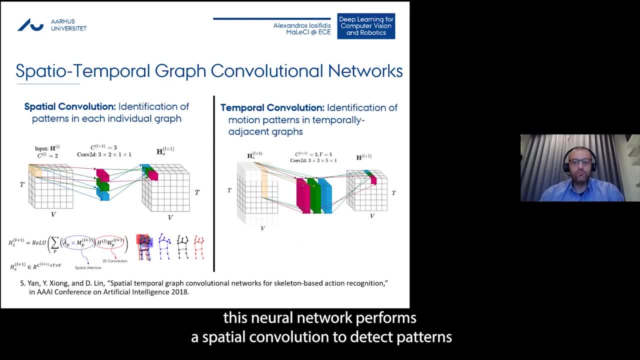 At each of its layers, This neural network performs spatial convolution To detect patterns in the human body poses And the temporal convolution for detecting patterns In the movement of the joints of the human body over time. In order to achieve high performance, These networks need to be formed by a high number of layers. 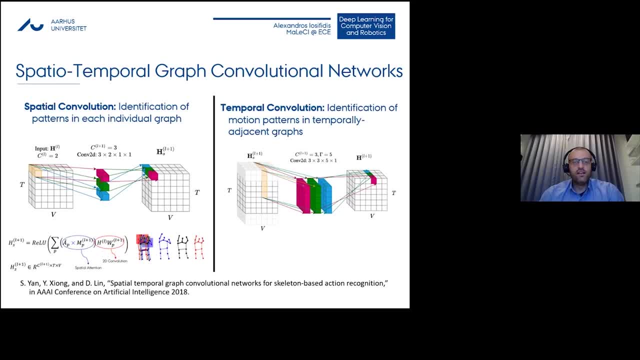 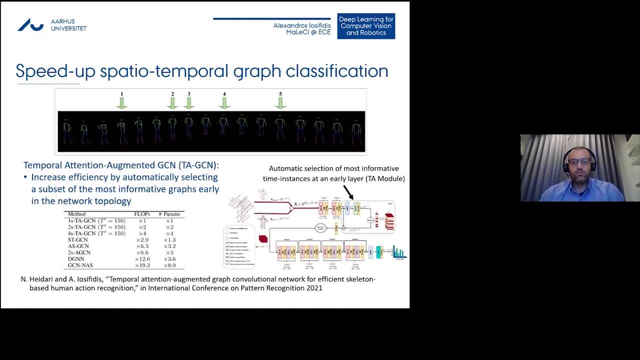 And to receive as input a high number of human body poses. This leads to slow evolution And slow operation. To speed up the calculations, We proposed a method for automatically selecting the most formative body skeletons, Based on a new temporal rotation mechanism. 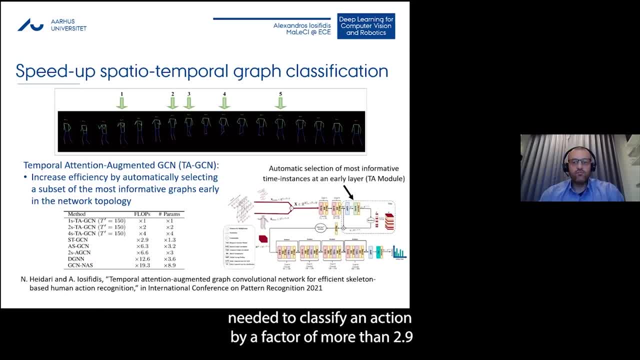 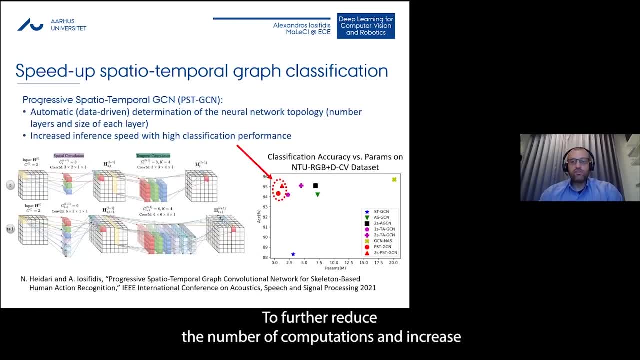 This leads to a reduction of the computations needed to classify an action By a factor of more than 2.9.. While achieving very similar performance. To further reduce the number of computations And decrease the processing speed, We proposed a method which automatically determines. 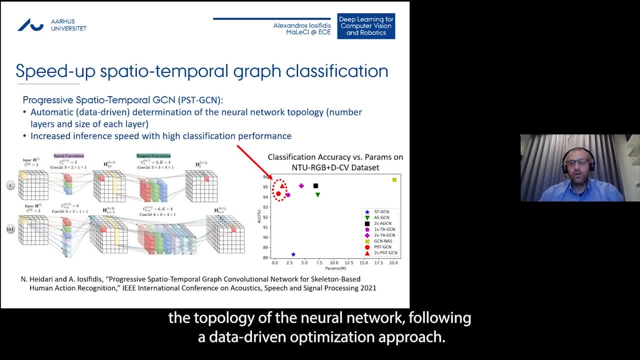 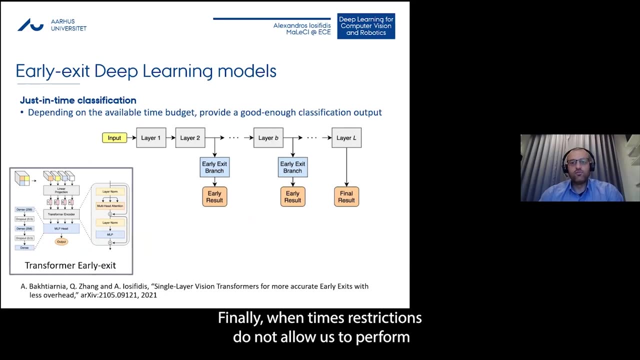 The topology of the neural network To perform a data driven optimization approach Using our method. Compact neural networks are designed Which lead to high performance, Low number of computations And increased classification speed. Finally, When time restrictions do not allow us to perform, 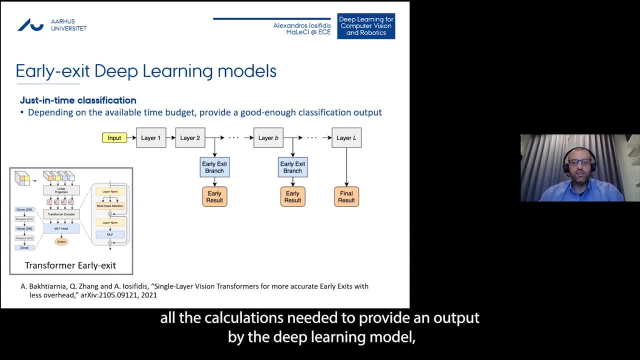 All the calculations needed to provide an output. By the debugging model, One can add early exit branches In the intermediate layers of the neural network topology. The performance achieved by using such early exits Depends on the type of exit used And the way it is trained. 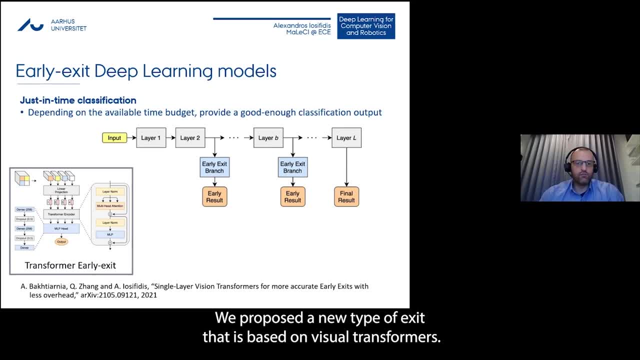 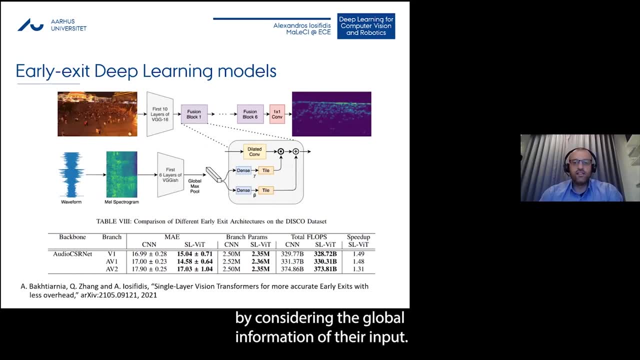 We proposed a new type of exit That is based on visual transformers. One of the properties of transformer layers Is that their outputs are computed By considering the global formation of their input. This makes them suitable for achieving high performance When they are used earlier in the neural network topology. 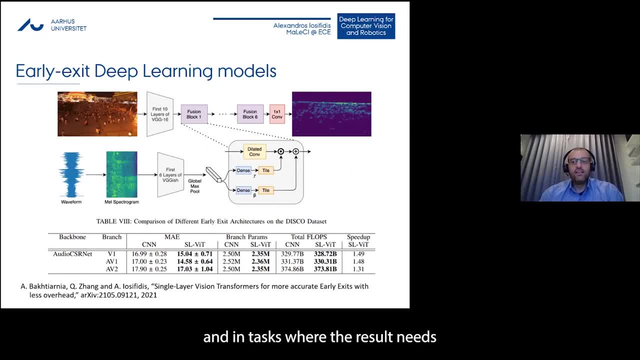 And in tasks where the result Needs to consider the entire Input image. Such a task is a task of audiovisual crowd counting, In which the network is asked to provide An estimate of the number of people appearing In a video frame. 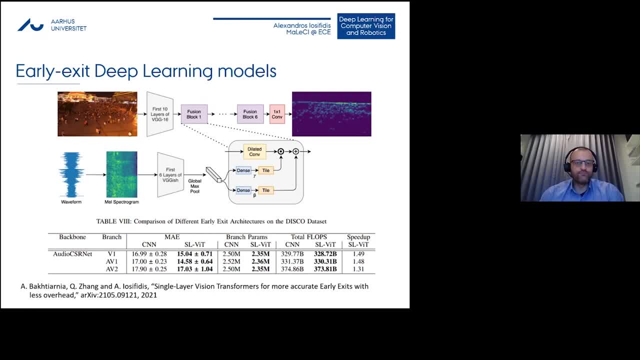 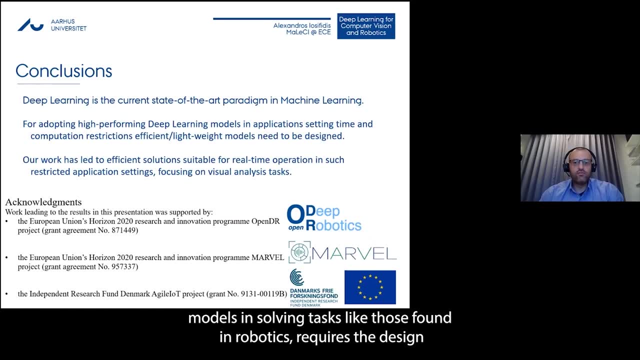 Considering also the ambient audio information. As a conclusion, We can say that The adoption of high performing Models in solving tasks, Like those found in robotics, Requires the design And effective training Of efficient deep learning models. We have been working in this direction. 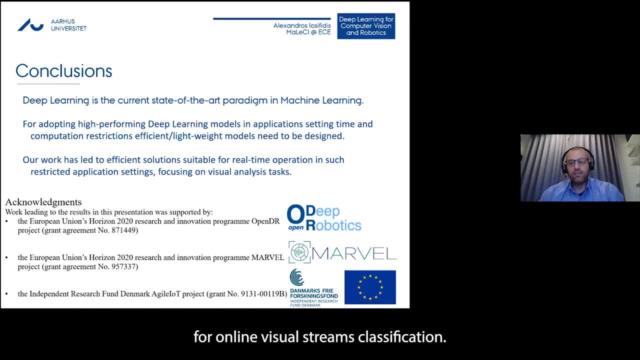 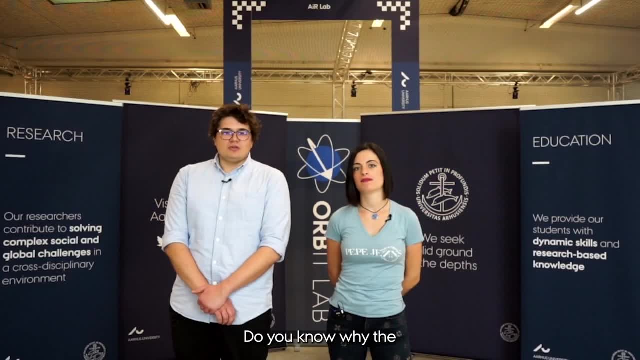 And proposed efficient solutions For online visual stream specification. Thank you very much for your attention. Do you know Why the world seems blurry Out the window of a high speed train? This is due to motion blur in our eyes. Cameras experience similar challenges as well. 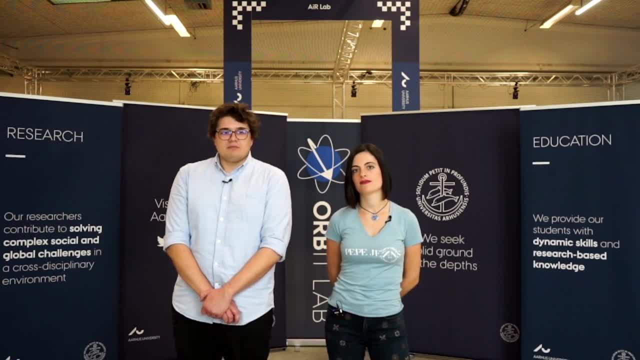 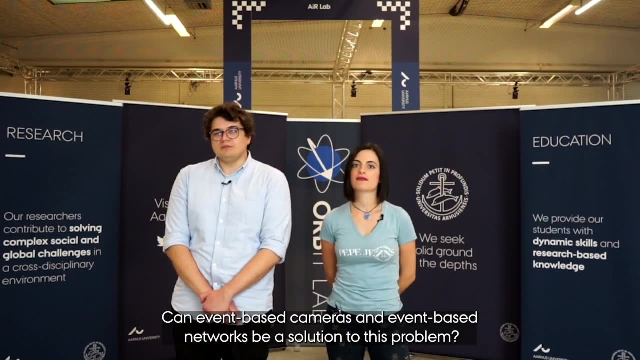 When we fly too fast with a drone, Motion blur can cause Our algorithms to fail. Can event based cameras And event based networks Be a solution to this problem? Professor Moradi will talk about Neuromorphic technology. Hello everyone. 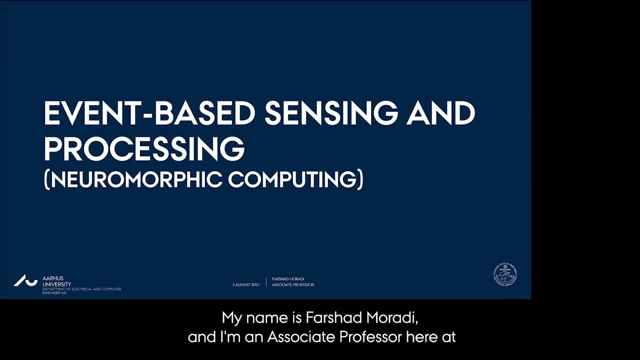 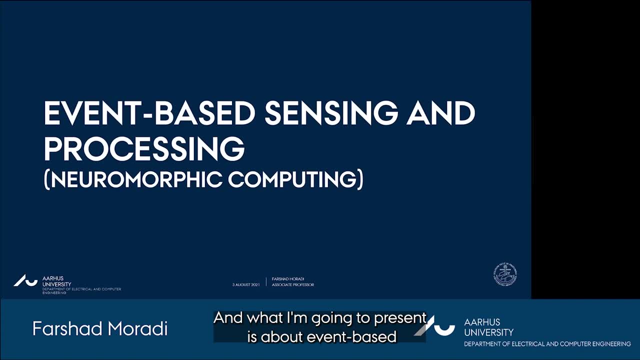 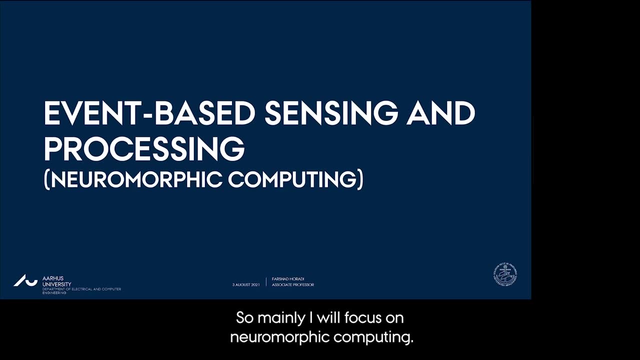 My name is Farshad Moradi And I'm an associate professor Here at Orbitz University Department of electrical and computer engineering, And what I'm going to present Is about events based Sensing and processing, So mainly I will focus on 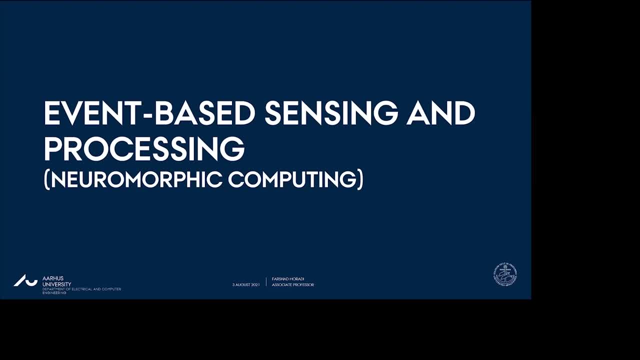 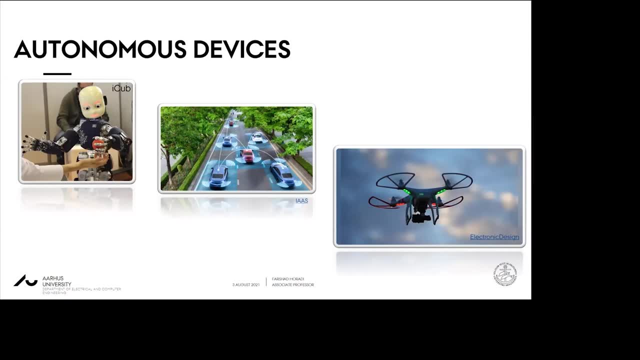 Neuromorphic computing. So today we See a lot of Autonomous device around us, So you can see some examples, As we are talking about Smart robots, You're talking about Automation or self-driving cars And also self-driving. 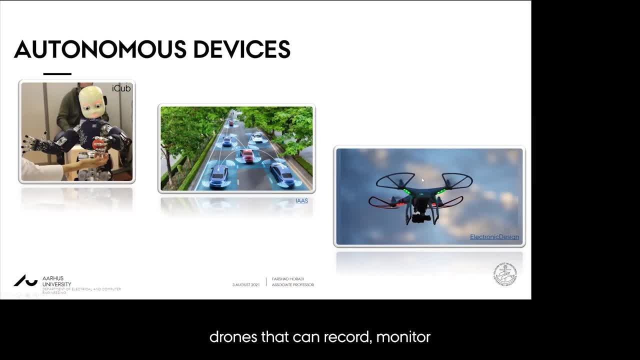 Or Drones That Can Record, Monitor And then Process The data. What is important here For all these devices That we see around ourselves Is To Have a high performance To be able to do. 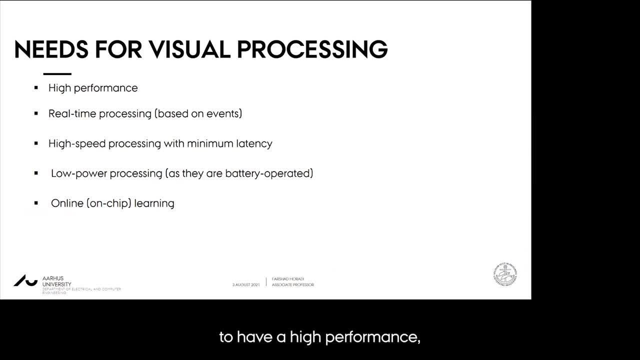 Real time processing. When they're receiving data, They process at the same time, Without Probably Even sending it Data to cloud Or Not being able To do A real time processing. When they're receiving data, They process at the same time. 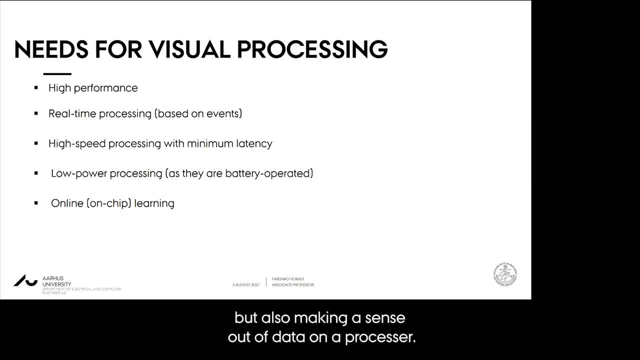 Without, Or Not only For, data collection, But also Making a sense Out of data. On Processor, They need to Have a high speed With Minimum latency, And What is important here Also Is 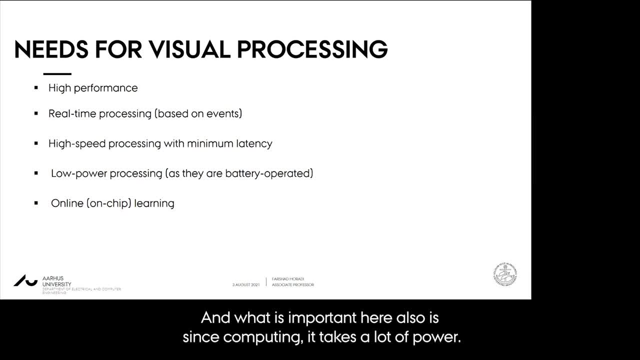 Since computing It takes A lot Of power, So it's quite important To have a low power Processing, Because Mainly These Devices Are Battery operated And Have a Long Battery lifetime. Another: 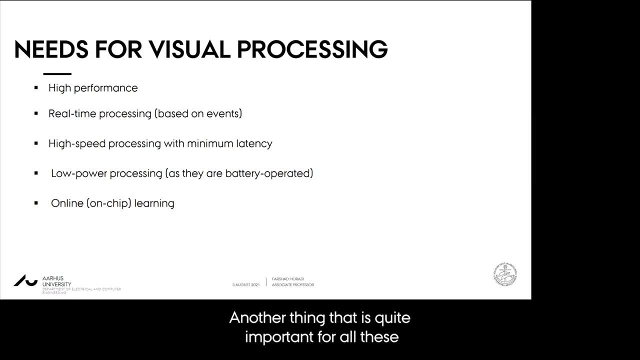 Thing That is Quite important For All These Processors, Or All These Device That Are Able To Adapt Themselves To Environment. They Learn Things And 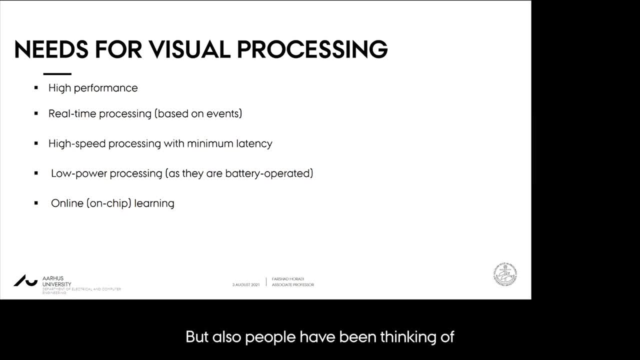 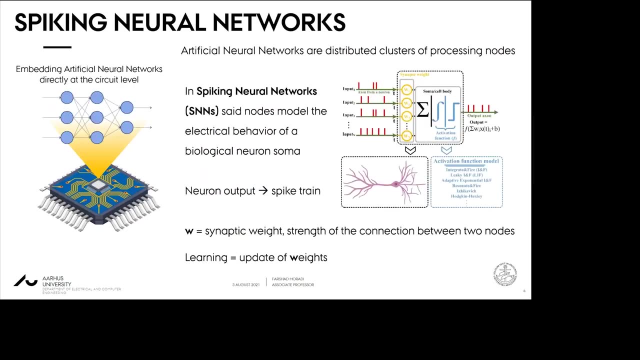 They Can Adjust In Thinking Of Machine Learning, Where They Get The Digital Data And Then They Process This Digital Data, But In Reality They Are. 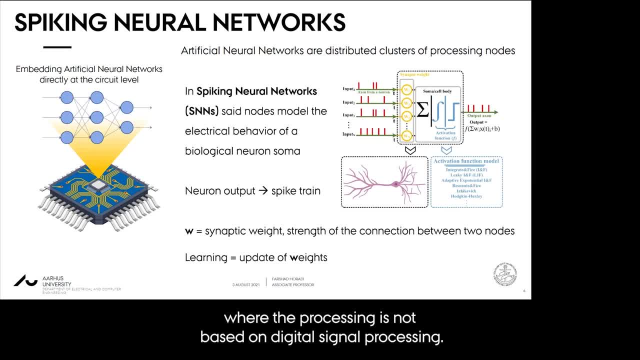 Not Like Our Brain, But There Are All These Devices Or These Neural Networks Are Working, Based On Spiking Neural Networks, So Similar To The 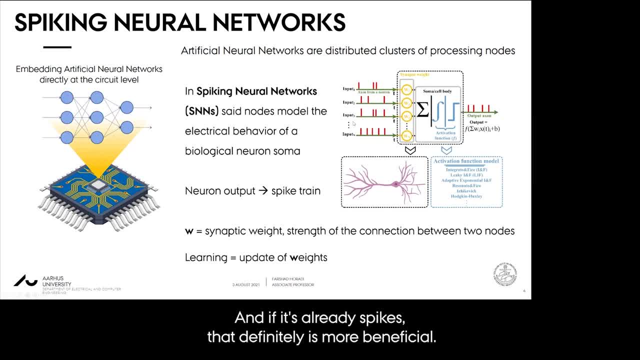 Brain, Where The Data Is Communicated Through Spikes, And So When We Have, We Have Different Activation Function Or Different Types Of Neural Implementation. So 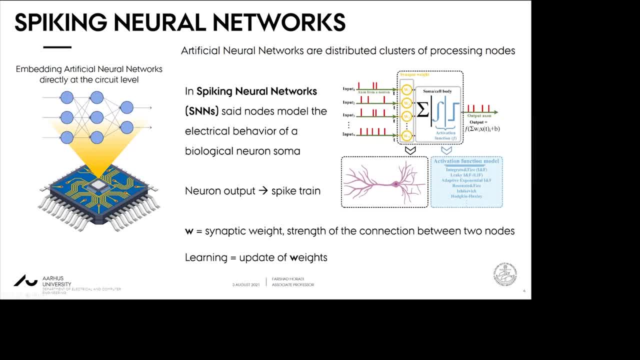 Which Can Be Leaky, Integrated Fire, Leaky Fire And Other Types Of Neurons, And Then They. So What Is Another Thing As Important Here? 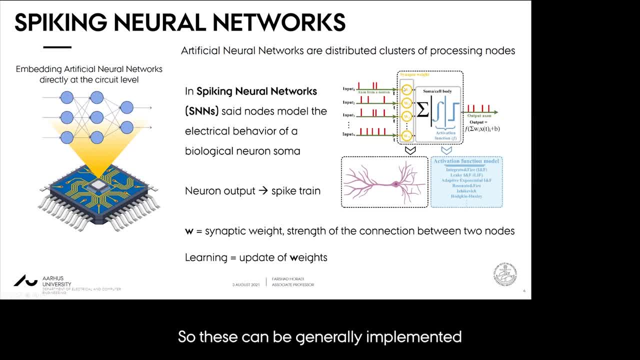 Is That Synoptic Weight, So This Can Be Generally Implemented Using Digital Kind Of Way Or Analog Way Or Other Types Of Neurons, And Then 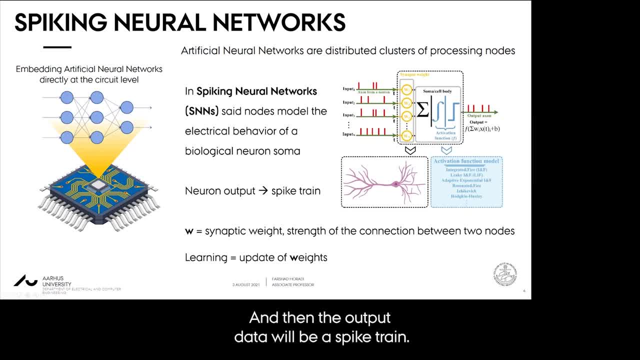 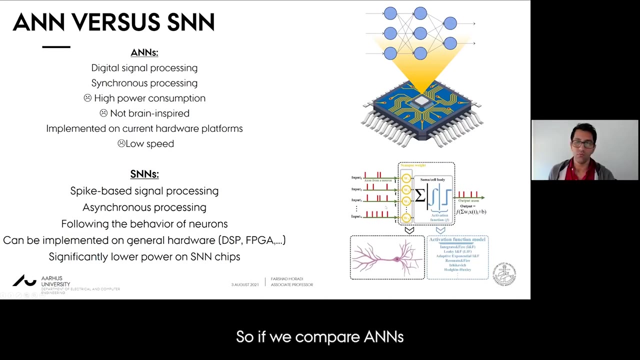 Given To A Neuron, Based On Whatever Complexity That We Have In The Network, And Then- And The Output Data Will Be A Spike Trains. 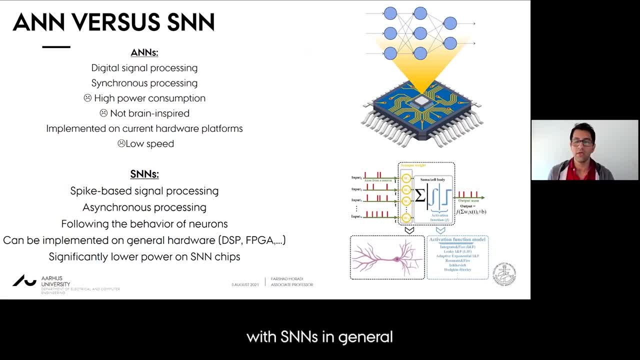 What Is The Main Problem With N? They Have A Very High Power Consumption So They Are Not Biologically Plus, So They're Not Like Brain. 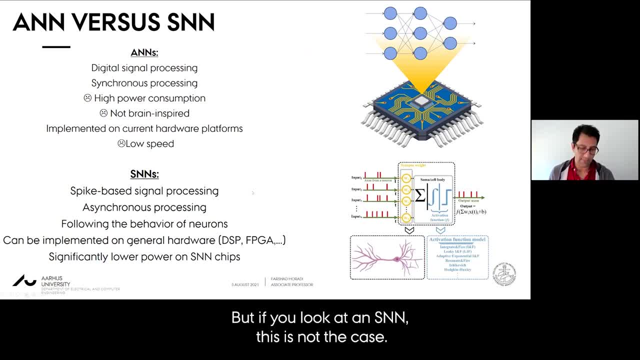 Inspired, And So They Are Not The Case. So We Are A Spike Base Signal Processing, Their Synchronous Kind Of Processing, And So We What? 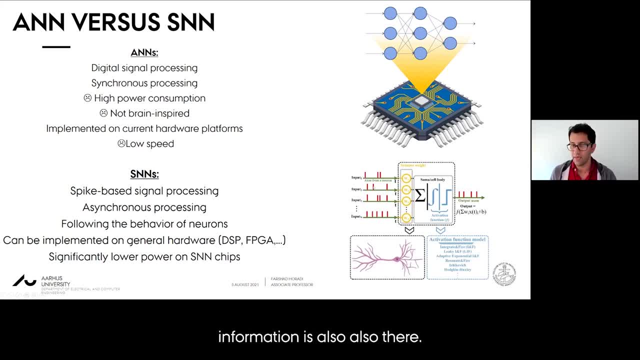 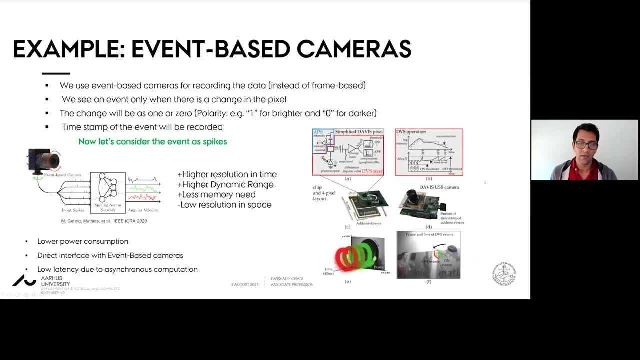 We Can Have There. They Are Able To Implement On The Frame. So This Is Just An Example: Event Base Camera. So The Way They Work, 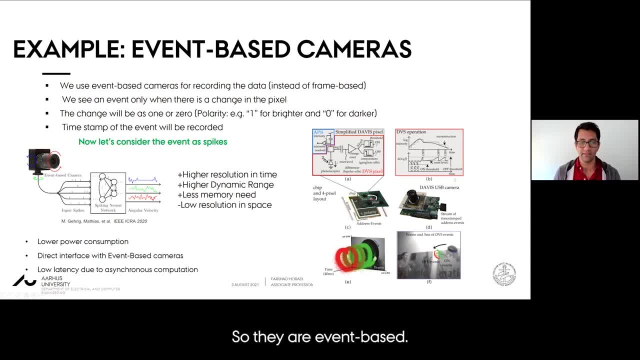 They Don't. They Don't Work Based On The Frame. Instead, They They Assuming That The Frame Can Be Interfaced Directly With This Spike. 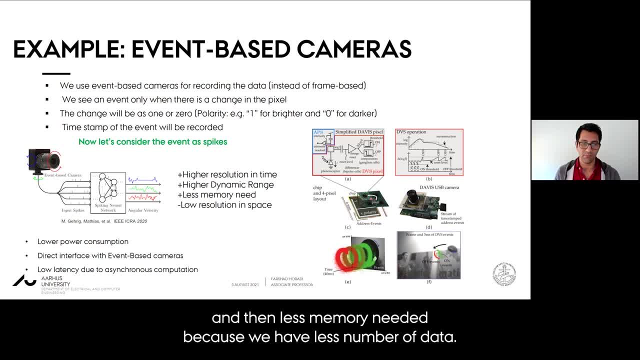 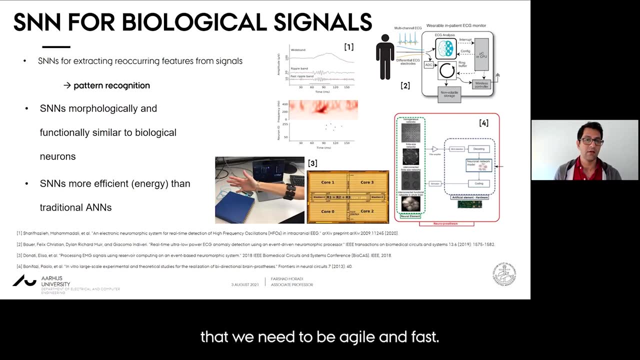 Train That We Are Getting, Meaning That We Can Make A Sense Of The Data. They Have A Very Important, But We Are Looking At Other. 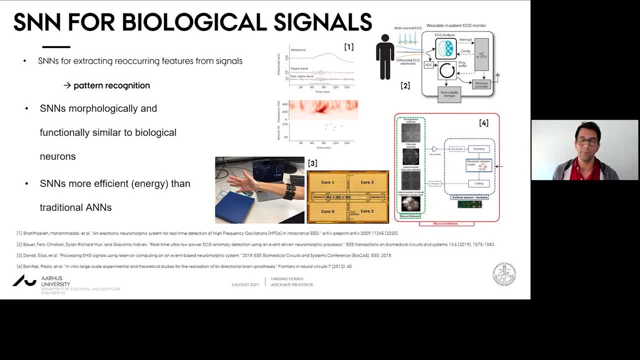 Perspective Of This, Where We Like To Interface These Types Of Spiking Neural Network That We Are Developing With Sensors Like Body Sensors That Can 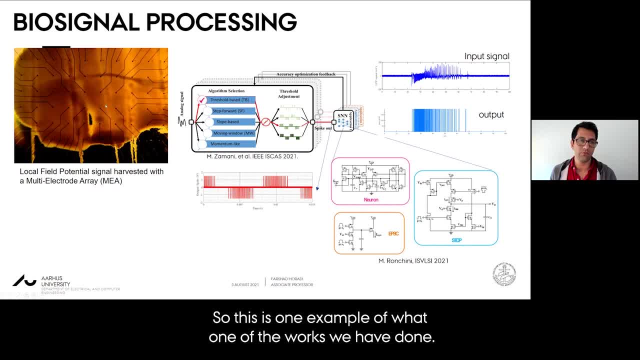 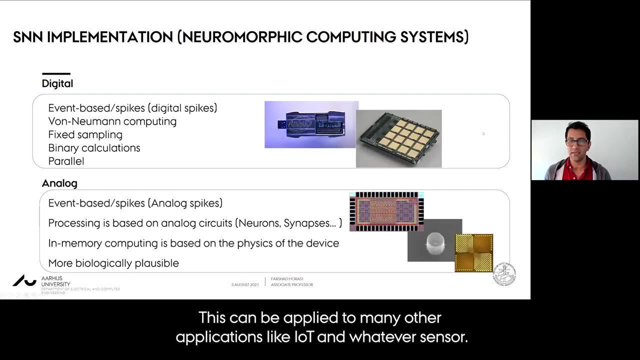 Be A Spiking Neural Network. So This Is A Brain Slice. So We Have Recorded Data Here And Then We Have Given To A Kind. 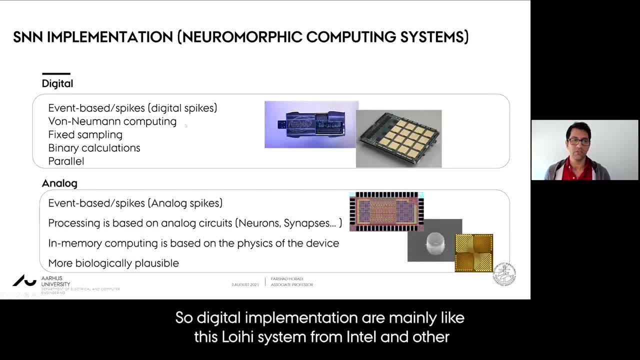 Of A Multi Log, So Digital Implementation, Are Mainly Like This Loy He System From Intel And Other, Let's Say, Companies Are Working On This. 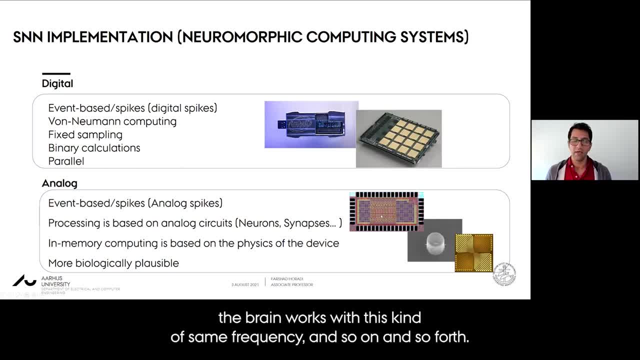 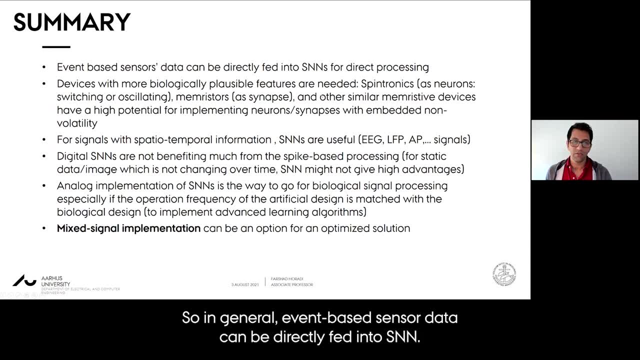 But It Can Be Also Analog, So Make Better Sense Of The Data That We Are Receiving. So, In General, Even Base Sensors Data Can 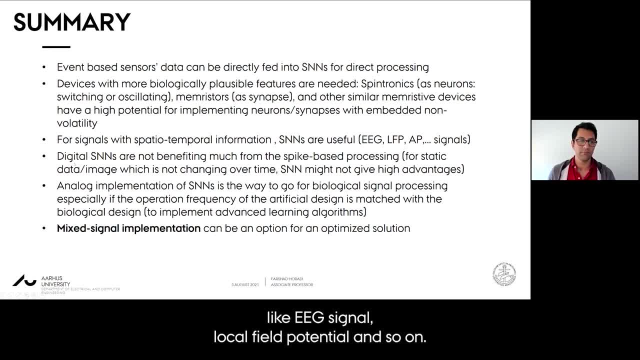 Be Directly Fed Into SNN. So This Is A Very Good Implementation Of SNN Is Way To Go For Biological Approach Mix Signal Implementation. 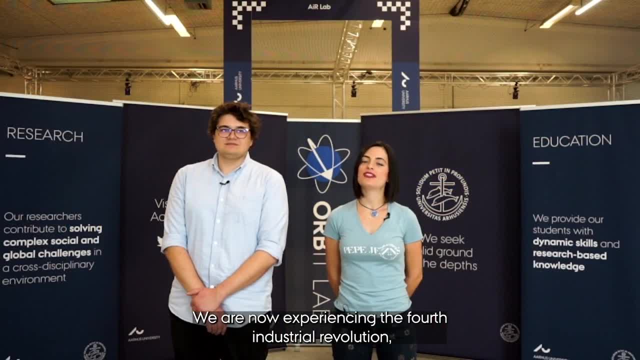 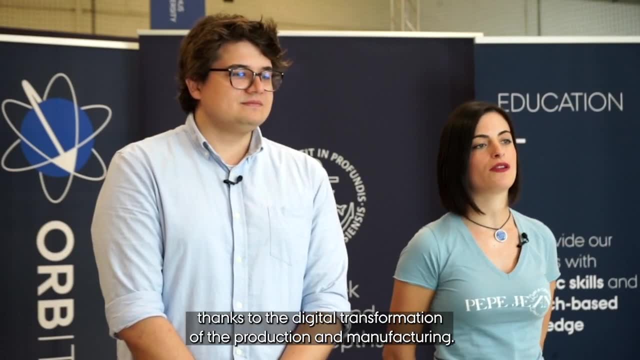 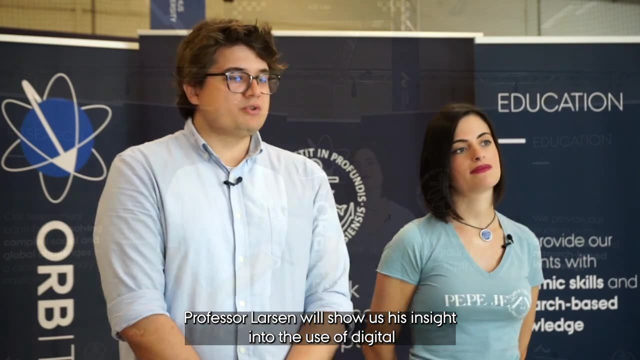 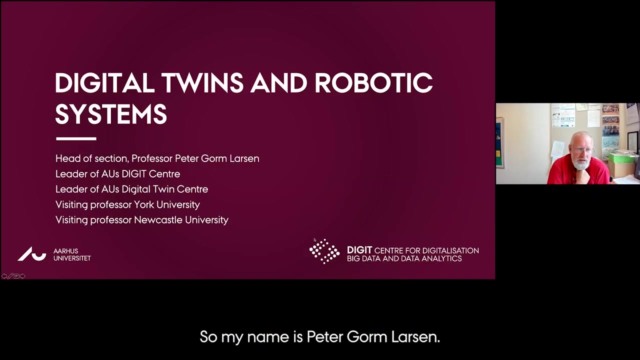 Can Be An Option For An Optimized Solution. So We Have Several Busy Positions. If You Are In This Talk, Professor Larson Will Show Us. 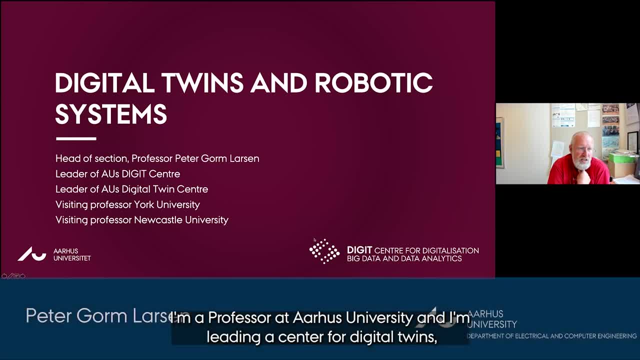 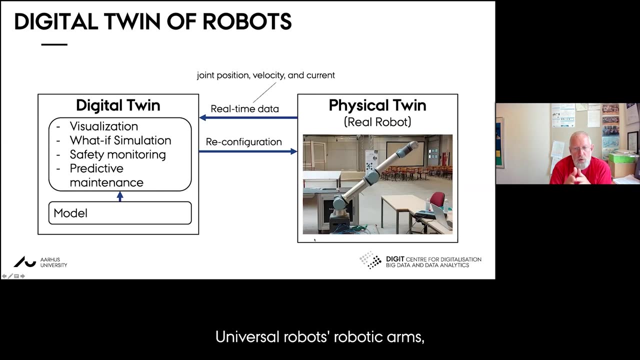 His Insight Into The Use Of Digital Twins With Robotic Systems. So My Name Is Peter Gorm Larson. I'm A Digital Twin Rather Than 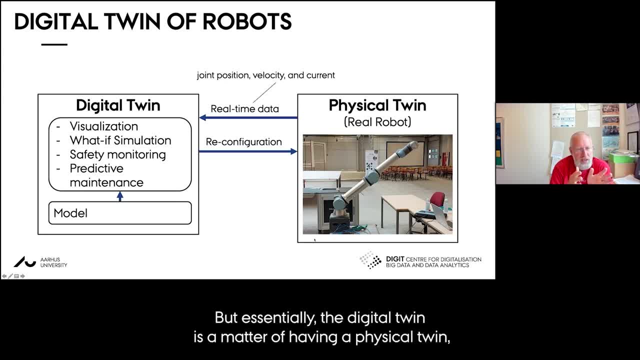 Archeological Robots, Which We Also Working With. But Essentially, A Digital Twin Is A Matter Of Having A Physical Twin, A Real Robot And A 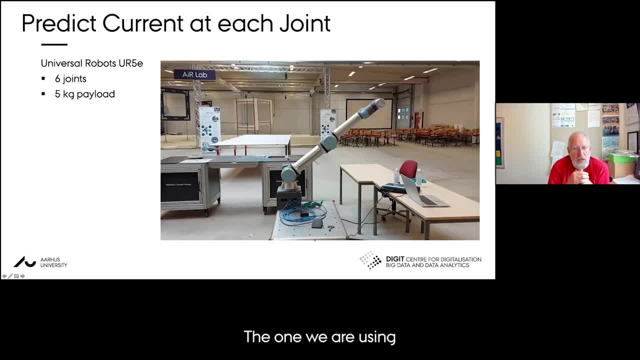 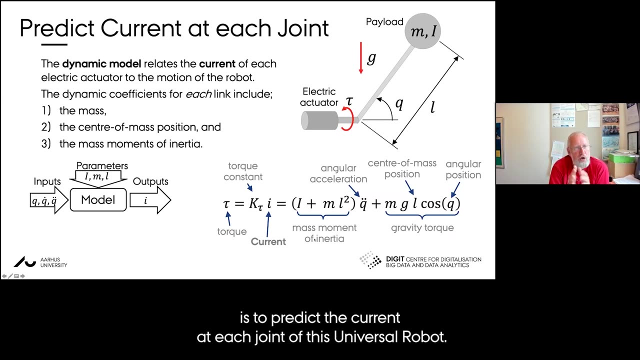 Model- The One We Are Using- Is Standing And Having Six Joints. It Can Take Five, Five Kilos Payload And Standing Physically In Sky. 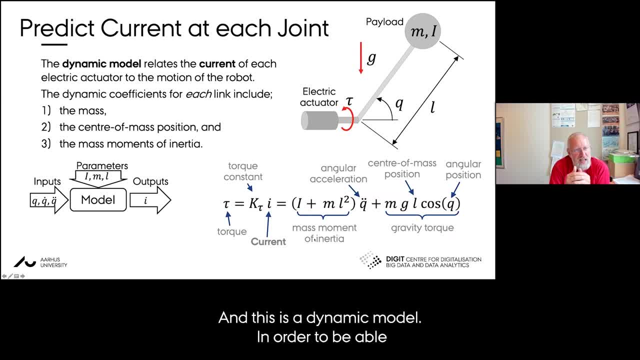 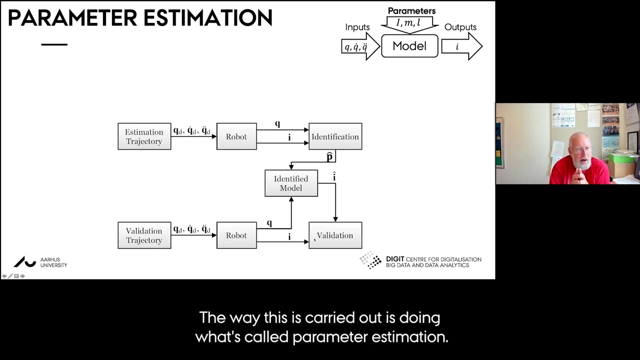 Now, What We Would Like To Do Is The Power At Each Joint And- And This Depends Upon The Mass That We Have- The Center Of 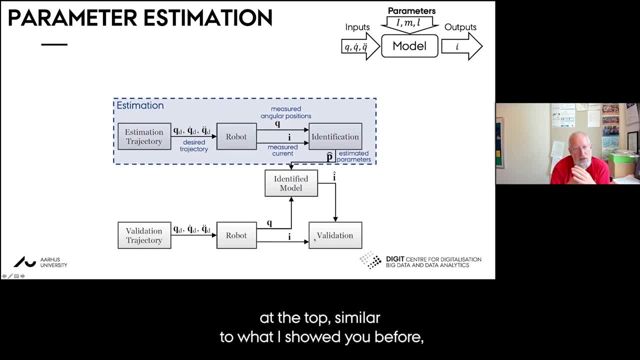 Mass Position And All Of This. So Some Rather As A Validation Component, Where You Try To Take The Identified Model And Try To Validate Against. 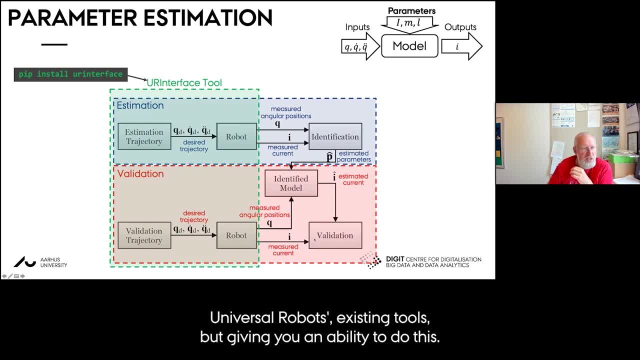 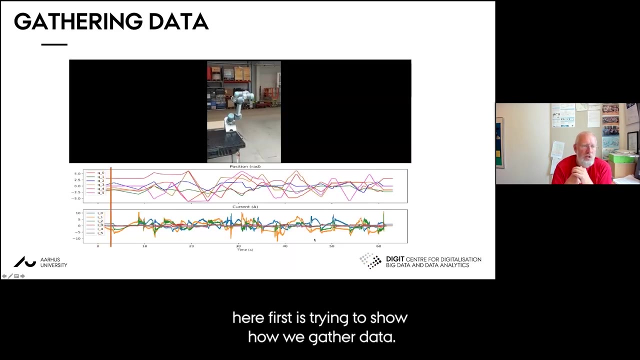 What You Actually Have Measured For Each Of The Joint. We Have This Data And This Is A Real Time Estimation Of Things And Calibration. 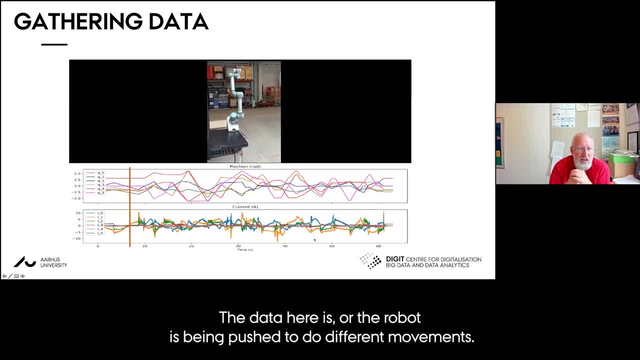 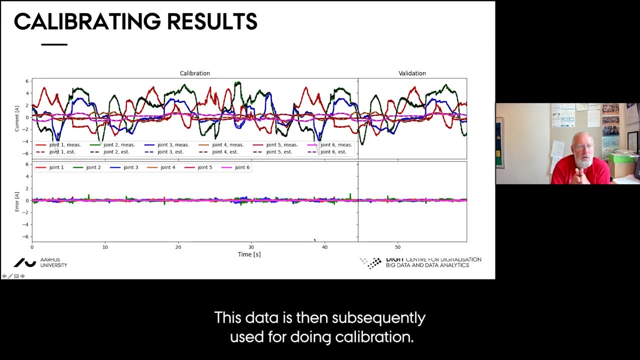 Possibilities. So What We Are Doing Here First Is Trying To Show How We Gather Data, The And Subsequent Used For Doing Calibration. So Essentially, 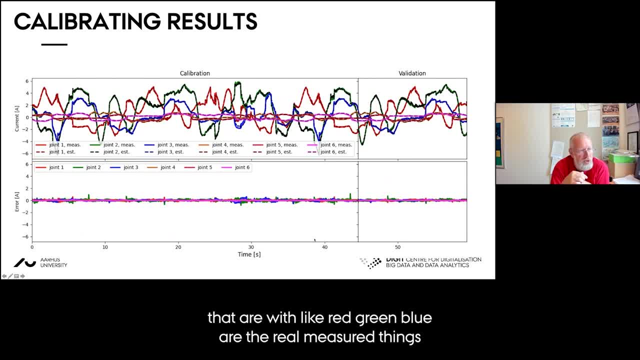 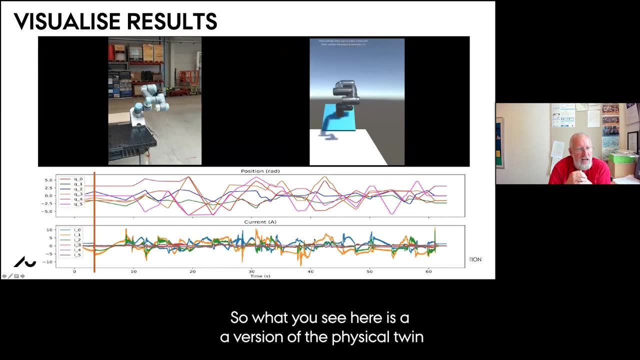 We Have The Curves That Are With Like Red, Green, Blue Kind Of Things Are The Real Measured Things And The Dot Inside Digital Twin. 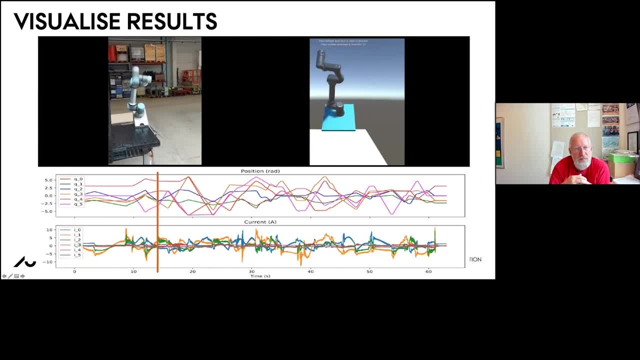 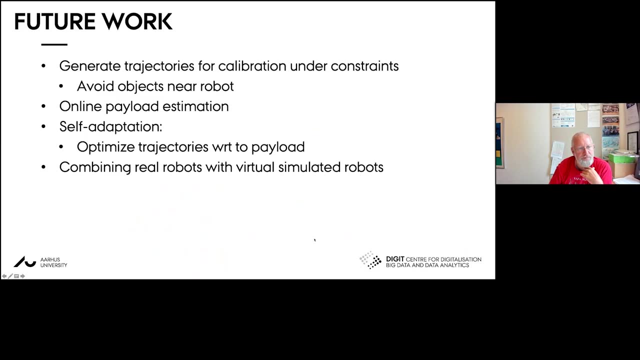 Where We Are Using The Estimations That Are Have Been Predicted In The Past, So This Is Used To To Be Able To Actually Also. 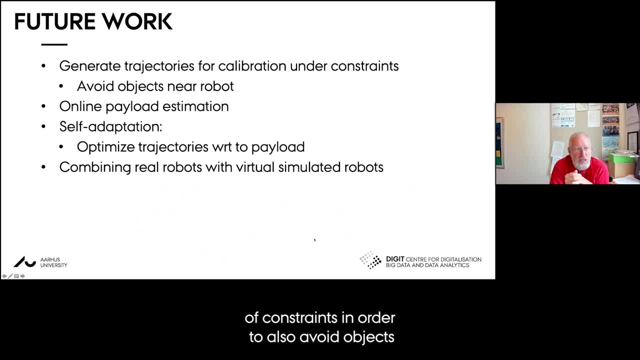 Take Into On A Different Kind Of Constraints In Order To Also Avoid Objects Coming Near To The Robot So They Can Be Giving Conditions, And 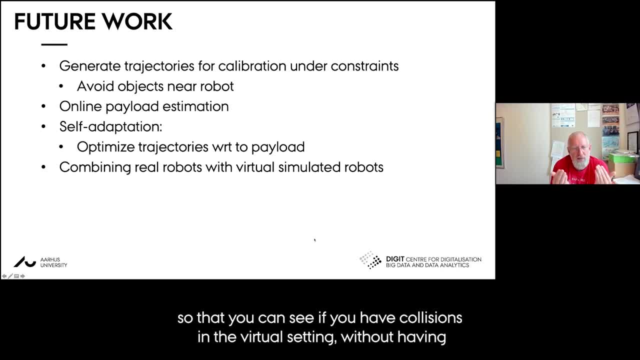 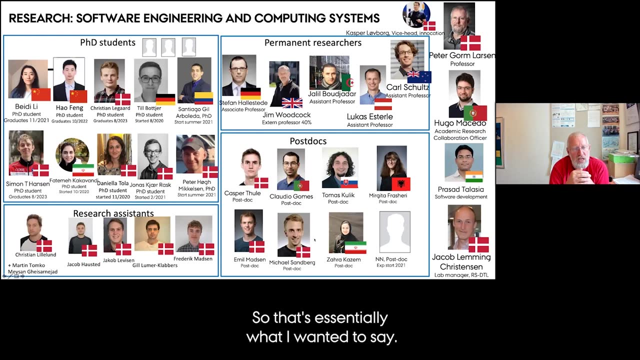 Then Do Online, Online Payload, Virtual Setting Without Having To Risk That They Really Have Conditions And Do Any Kind Of Damage To Each Other. So 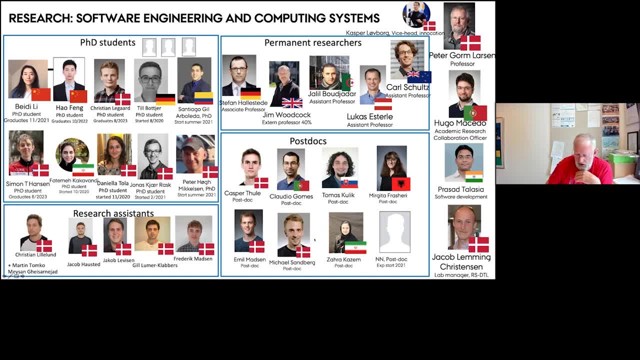 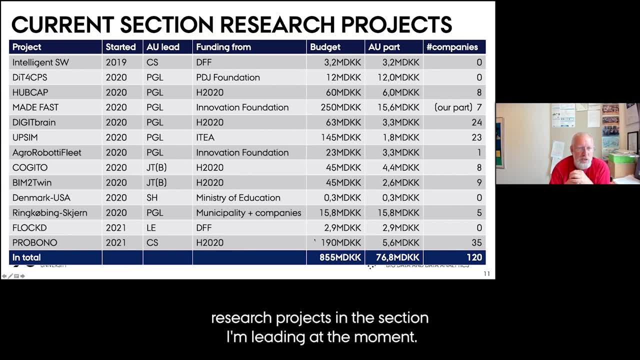 That's Essentially What I Wanted To Say. This: These Are The Current Projects, Research Projects In The Section I'm Leading At The Moment, And A 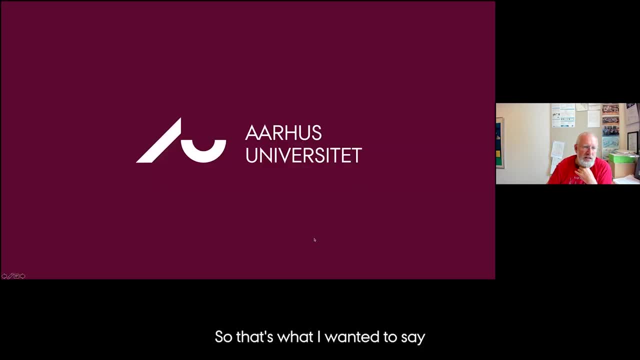 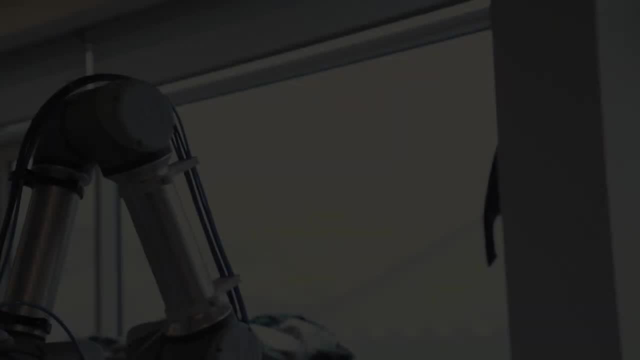 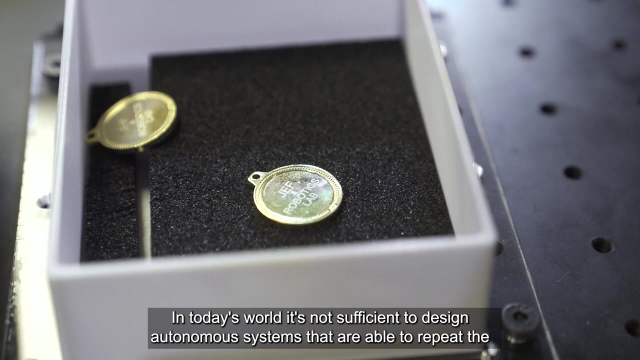 Lot Of Those Are Related To Digital Twins, Not All To Robotics. In Today's World, It's Not Sufficient To Design Autonomous Systems That Are 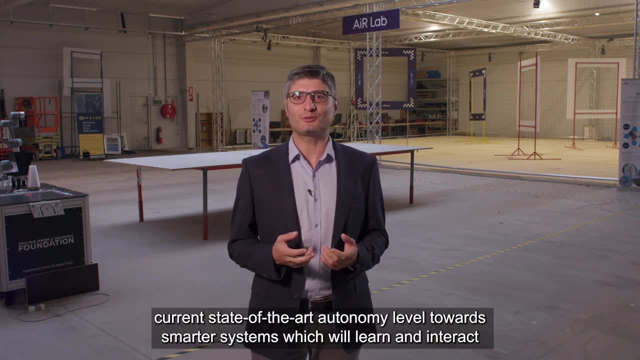 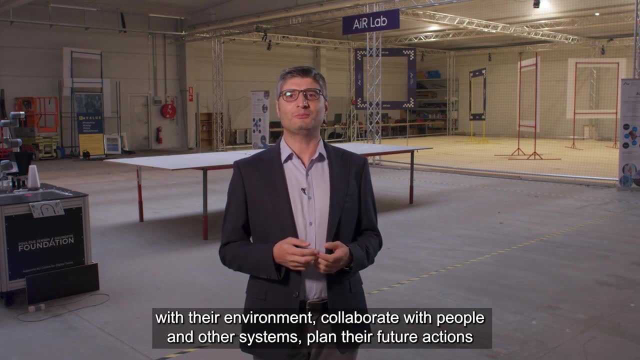 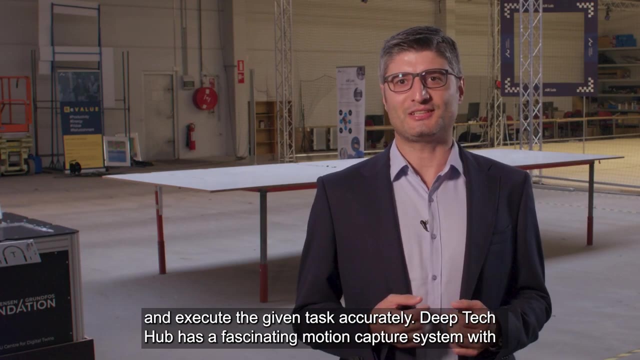 Able To Repeat The Given Tasks In Repetitive Manner. We Must Be Ready To Push The Boundaries Given Task Accurately. Deep Tech Hub. 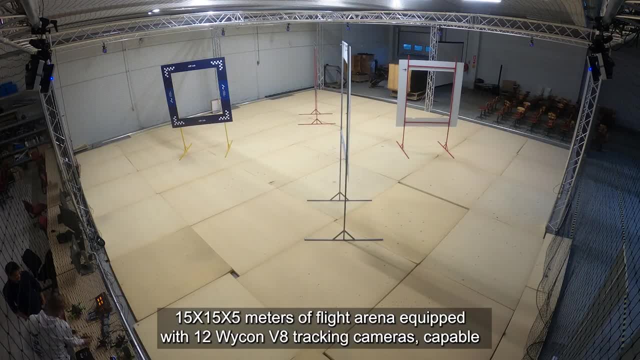 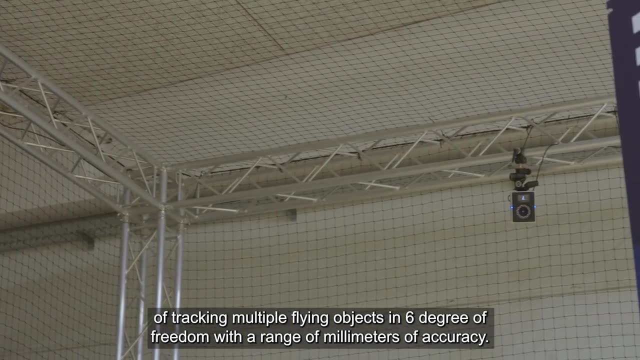 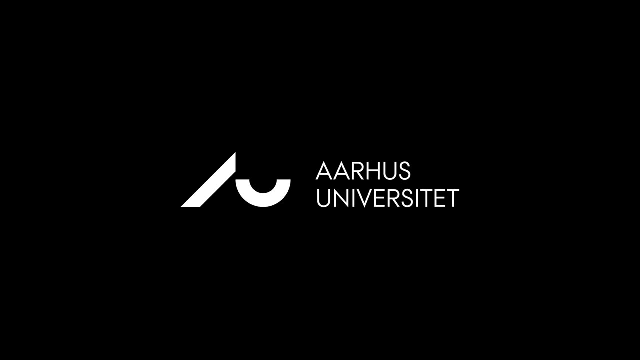 Has A Fascinating Motion Capture System. With Fifteen By Fifteen By Five Meters Of Flight Arena, Equipped With Twelve Wycombe, We A Tracking. 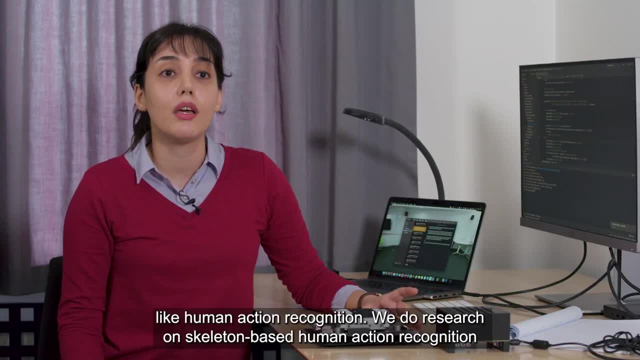 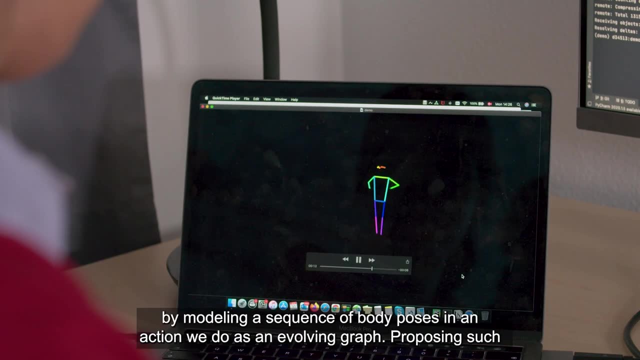 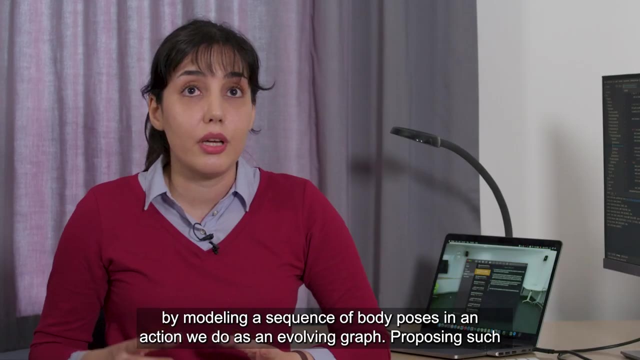 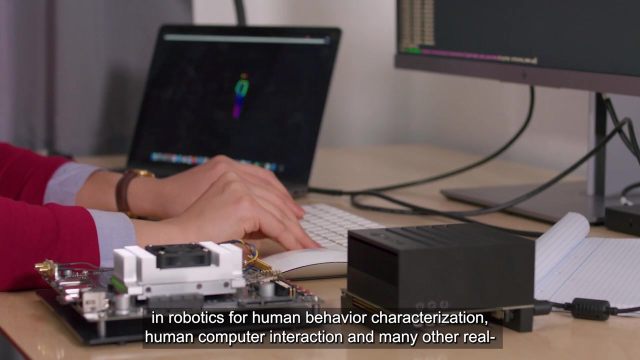 Cameras For Computer Vision Applications Like Human Action Recognition. We Do Research On Skeleton Based Human Action Recognition By Modeling A Sequence Of Body Poses. 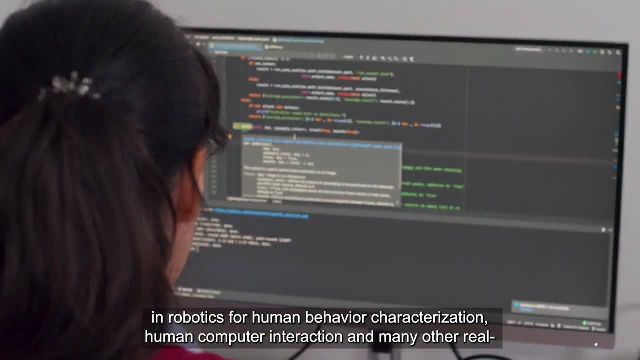 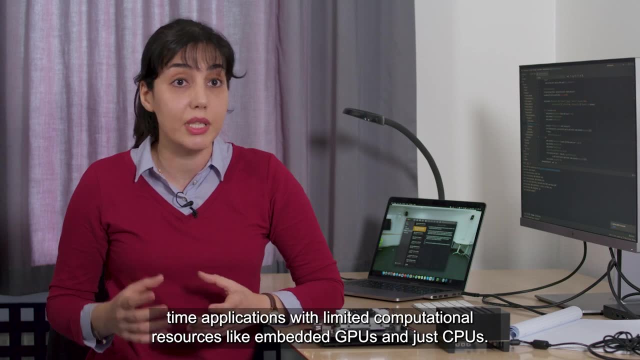 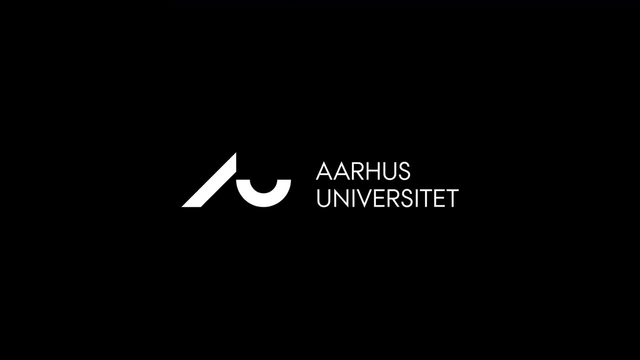 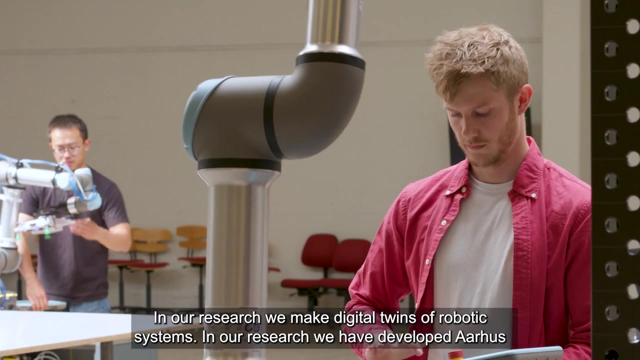 In An Action, We Do Action And Many Other Real, Real Time Applications With Limited Computational Resources, Like Embedded G, P, Us And Just C P. 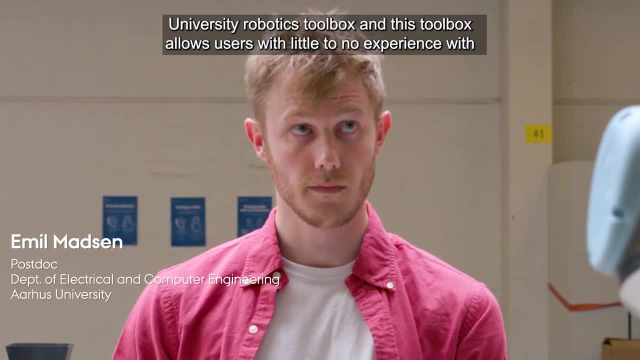 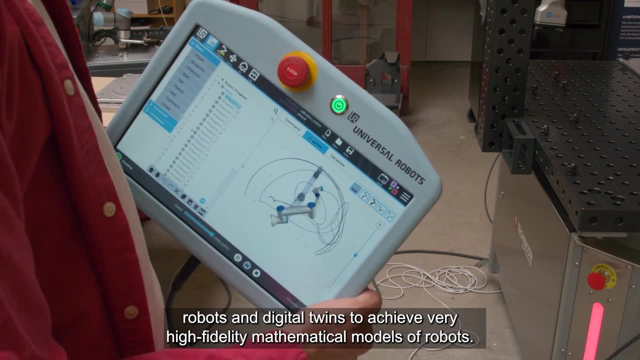 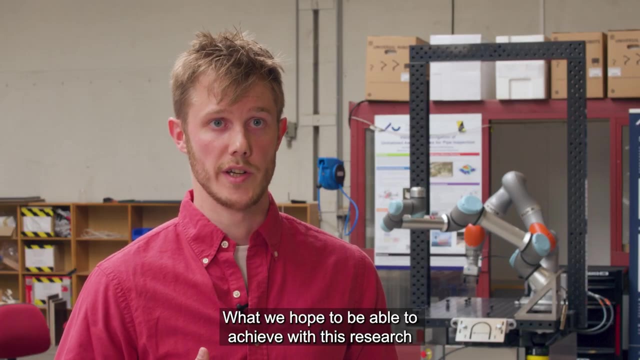 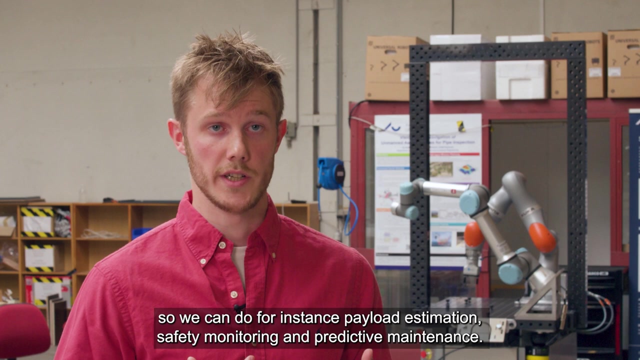 Us Now Research: We Make Digital Twins Of Robots And Digital Twins To Achieve Very High Fidelity Mathematical Models Of Robots. What We Hope To: 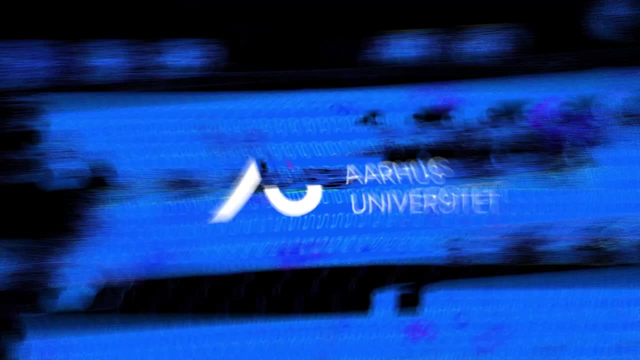 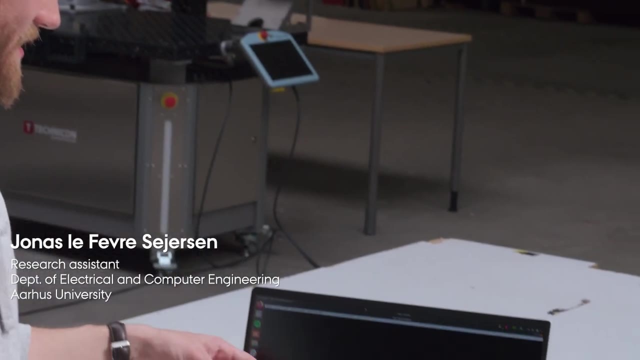 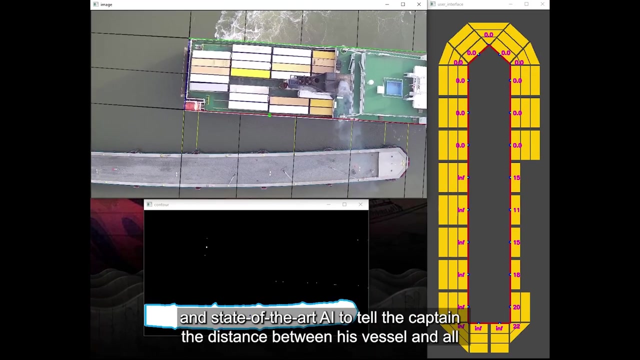 Be Able To Achieve With This Research Is Very High Fidelity Digital Waterways, We Utilizing Autonomous Drones And State Of Yard A. I. 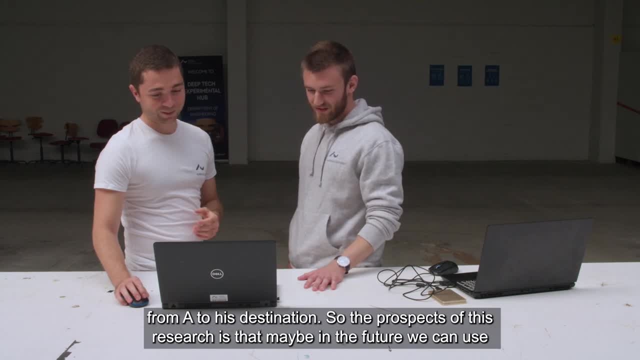 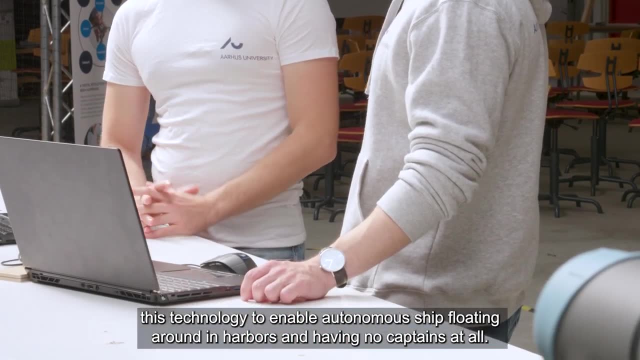 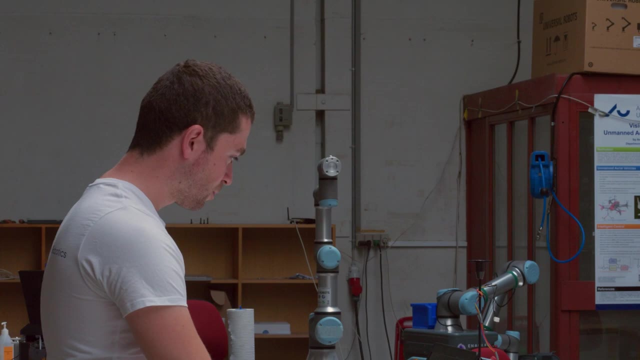 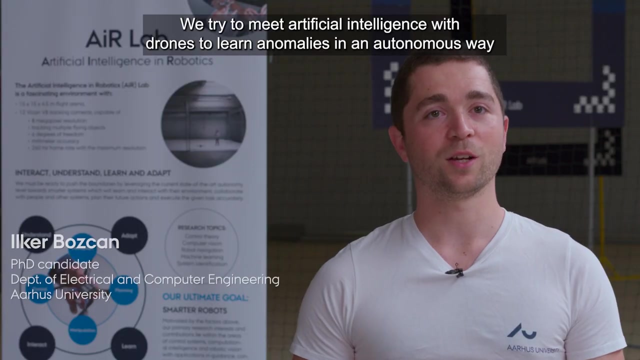 To Tell The Captain The Distance Between His Vessel And All The Surrounding Solid Objects. This Will Enable- In Air Lab We Design The Autonomous 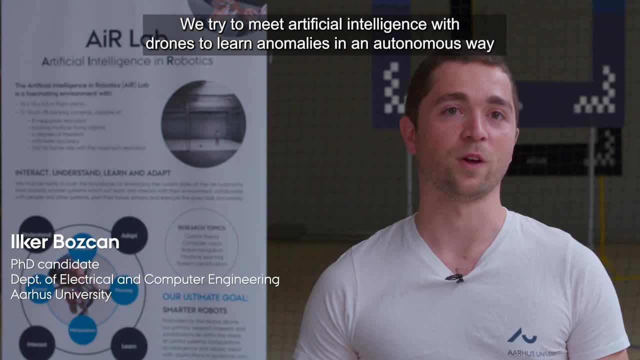 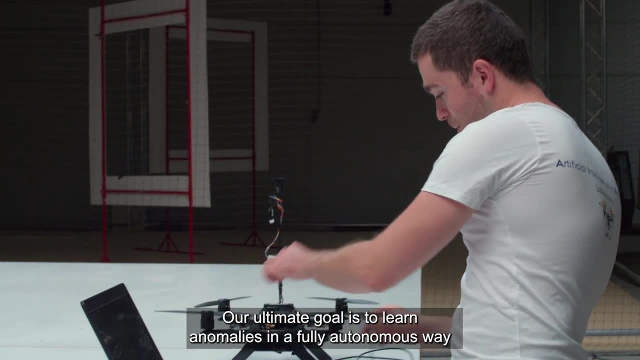 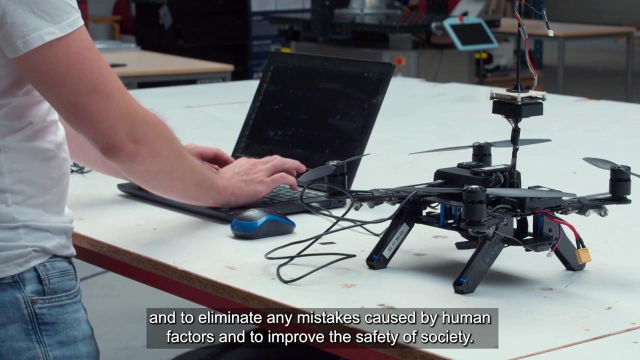 Surveillance Systems For The Monitoring Of Traffic Patterns. We Try To Meet Artificial Intelligence With Drones To Learn Anomalies In An Autonomous Research Here. 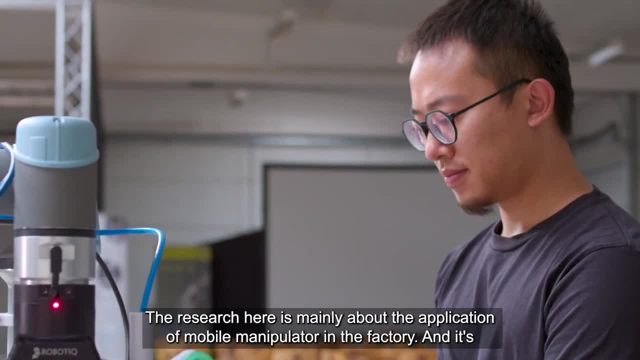 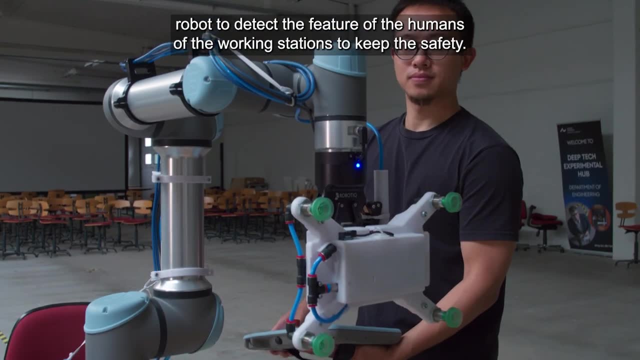 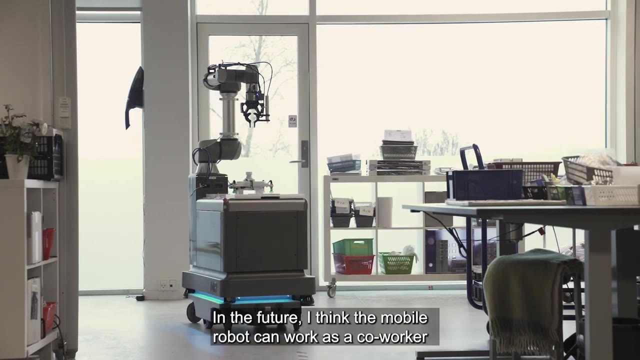 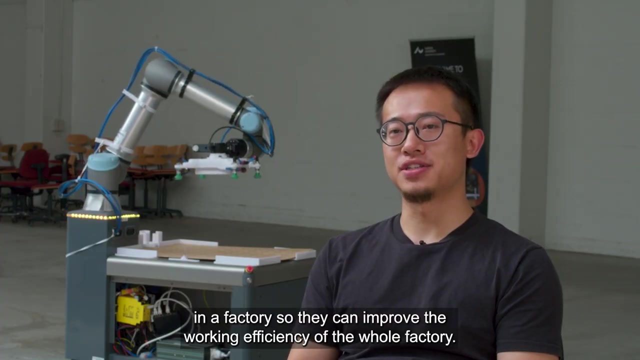 Is Million About The Application Of Mobile Metabolite In The Factory And Is Million About The Force Control And The Computer Vision Part. For Now, 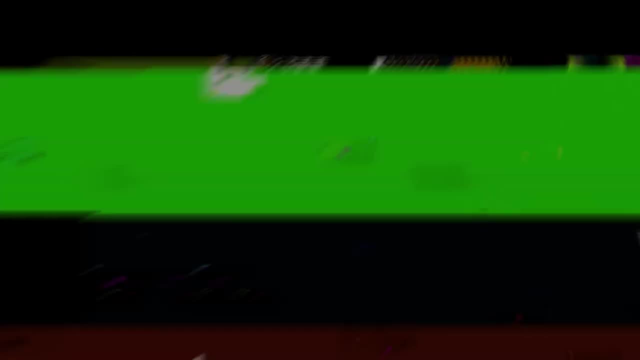 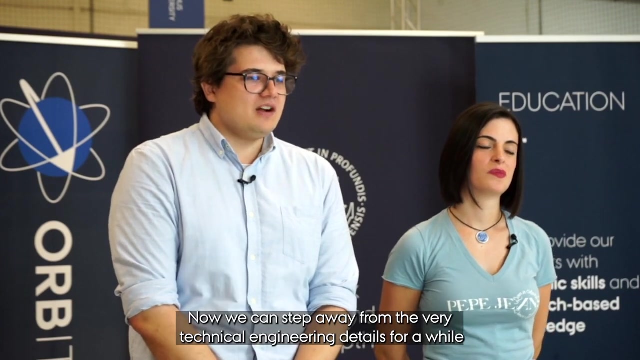 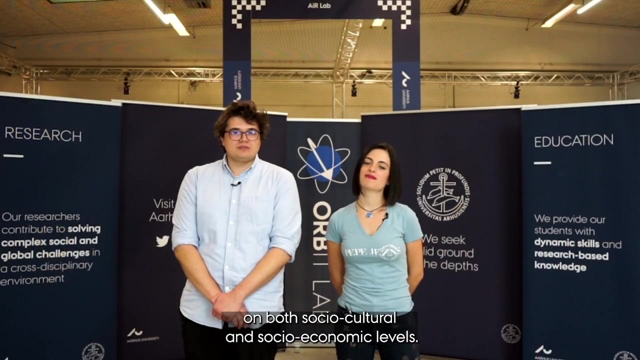 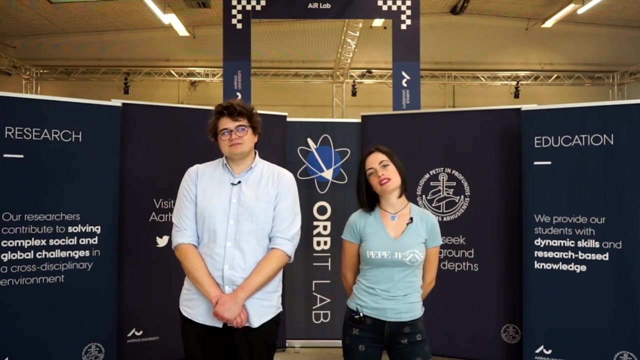 We Apply The Design To The Future, Of Our Future. Is It Fascinating To Imagine Robots With Social Skills Or Even Social Intelligence? Now We 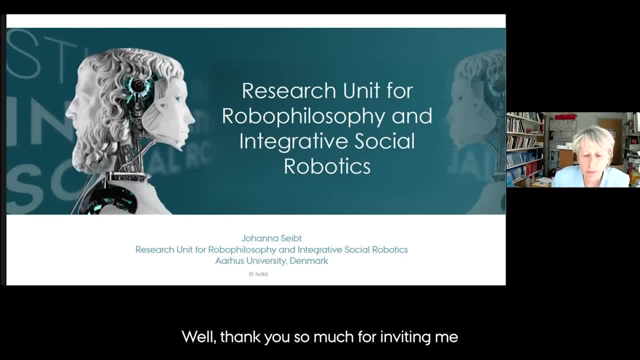 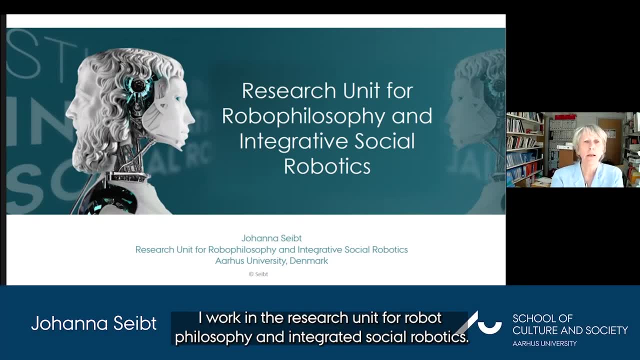 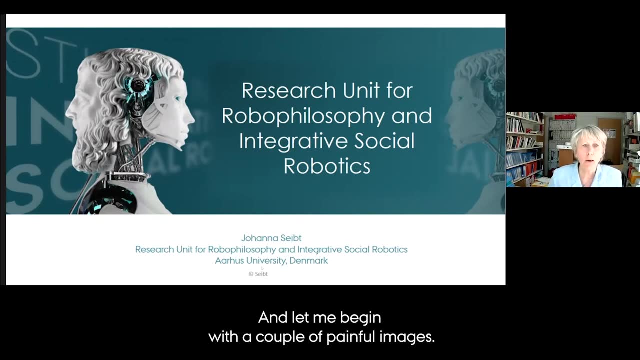 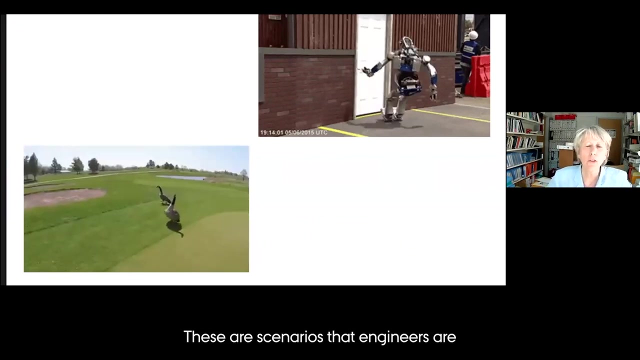 Can Step Away From The Very Important Event Here. My Name Is Johanna Sight. I Work In The Research Unit For Robo Philosophy And Integrated 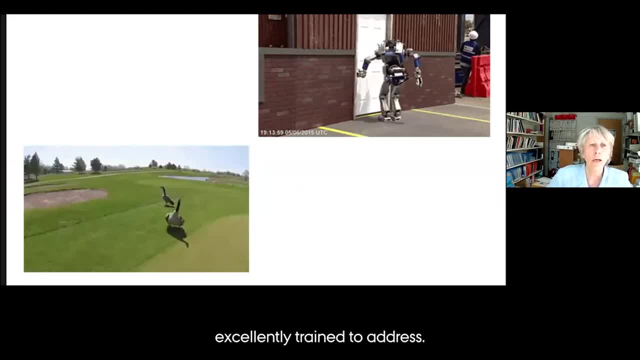 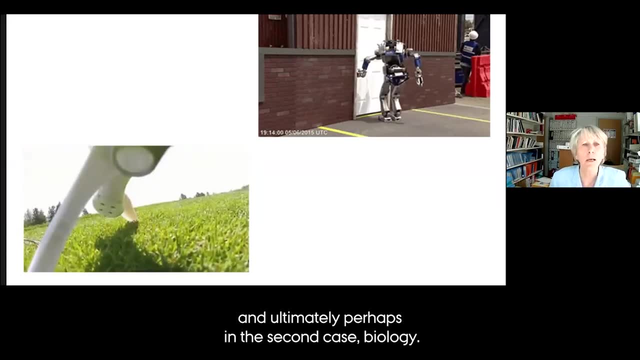 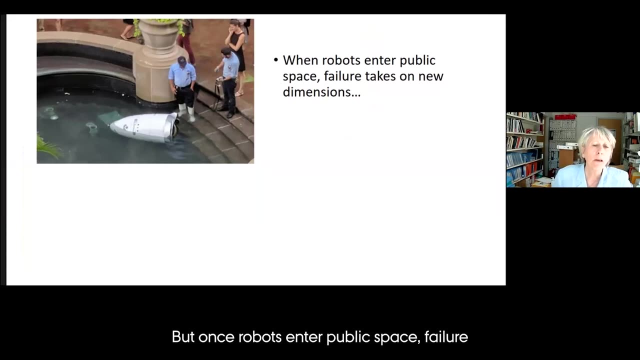 Robotics, And Let Me Begin With A Couple Of Painful And Perhaps In The Second Case, Biology. But Once Robots Enter Public Space, Failure Takes. 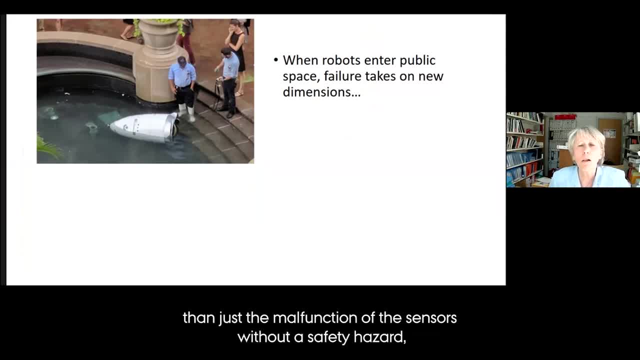 On The Dimension In Fact Increases By Several Degrees Of Magnitude- That The Robot Appear To Be Clumsy Or Out Like Stupid We 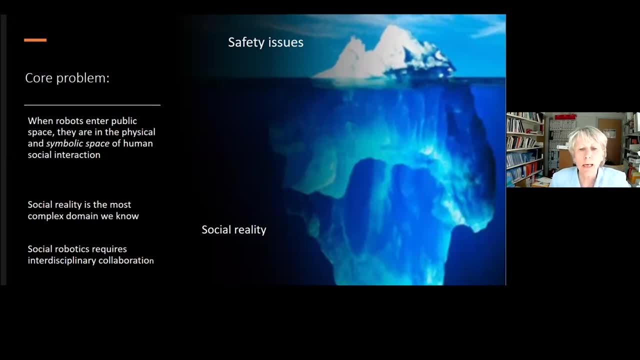 Addressing, Have Been For The Last Ten Years In Observing The Development In Social Robotics As Philosophers, Anthropologists, Psycho Psychologists, Neuroscientists In 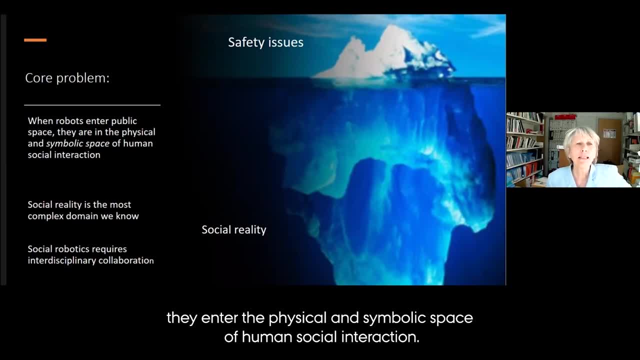 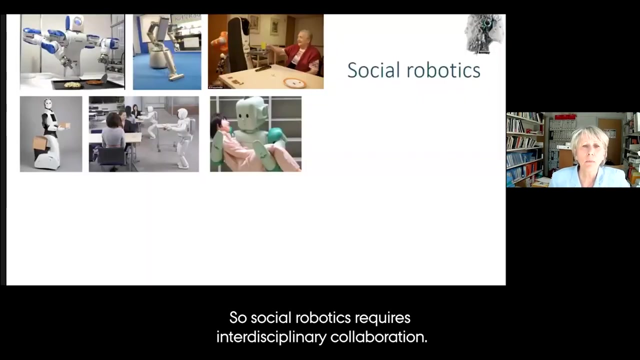 Public Space, They Enter The Physical And Symbolic Space Of Human Social Interaction. Safety Issues Are Just The Tip Of The Iceberg. Social Reality, The 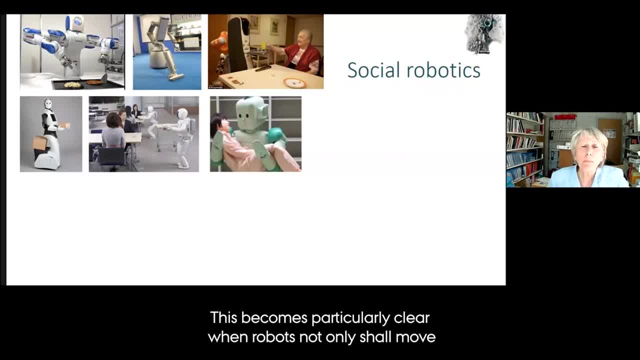 Symbolic Space Of This Becomes Particularly Clear When Robots Not Only Shall Move In Public Space, But Shall Perform More Complex Social Interactions. Fortunately, 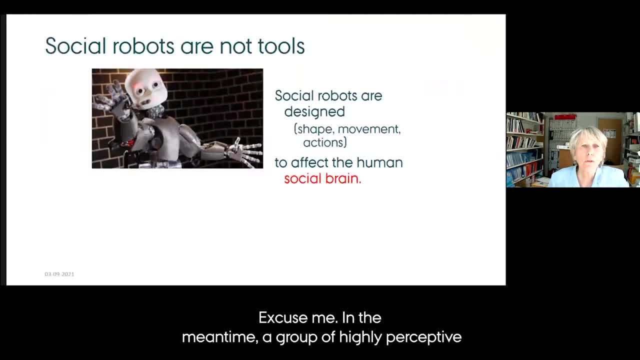 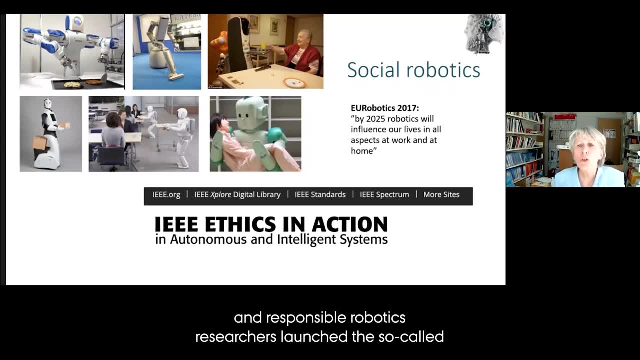 The Predictions Of Your Robotics In 2017.. Were The So Called I Global Initiative On Ethics Of Autonomous And Intelligent Systems, And That's A. 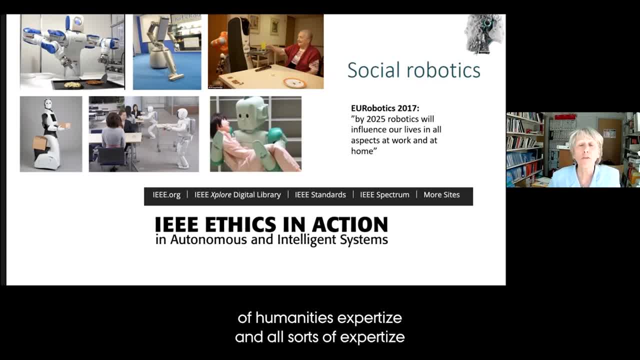 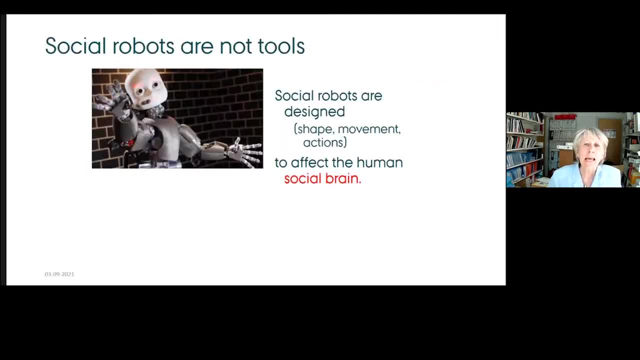 Group Of Researchers, Interdisciplinary Researchers, Working Towards New Standards For The Inclusion Of Humanities. The Human Robot Interaction Research Have Shown Social Robots Are 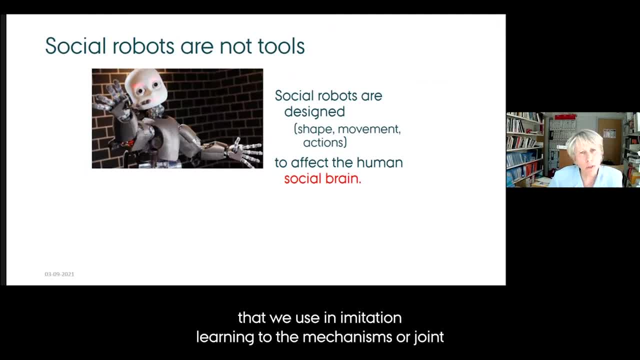 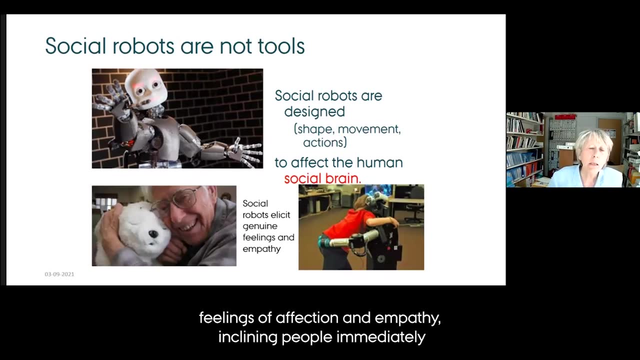 No Longer Tools. They Are Designed To Affect The Human Social Brain, Pre-Conscious Mechanisms Of Social Cognition From Motor, To Treat Them As. 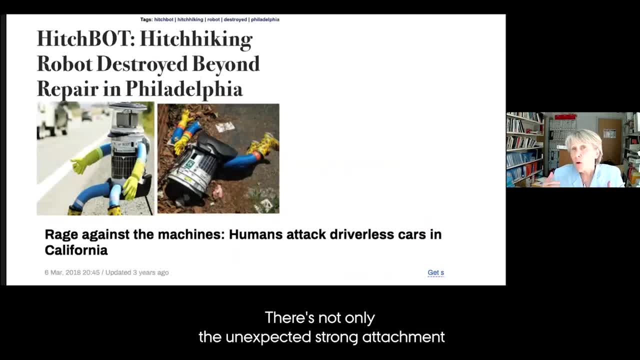 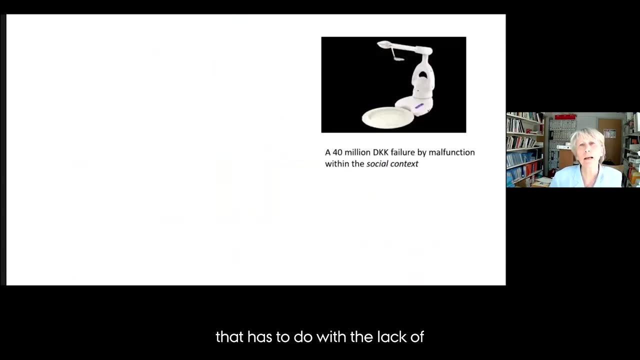 Social, Others With Certain Moral Rights. There's Not Only The Unexpected Strong Attachment That We See In Human Robot Interaction, But Also Unexpected Aggression Or 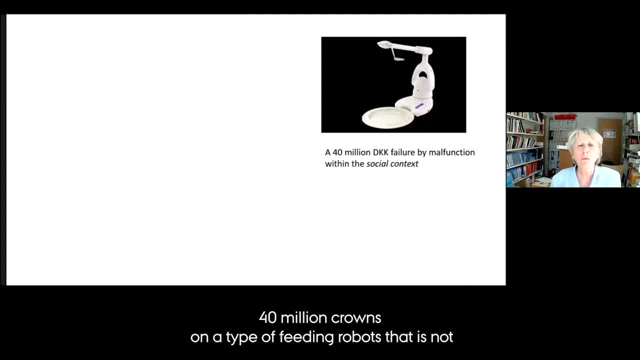 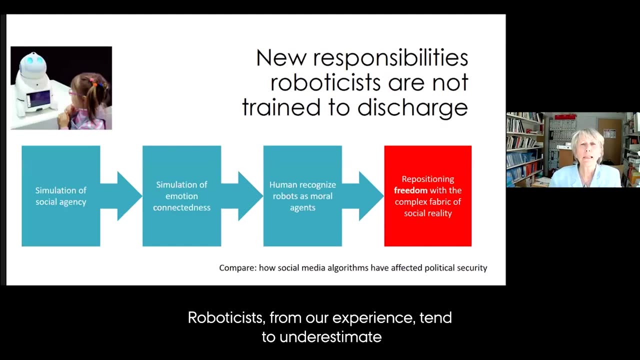 Unrest In 40. Million Crowns On A Type Of Feeding Robot That Is Not Used In Any Of The Danish Communion. According To 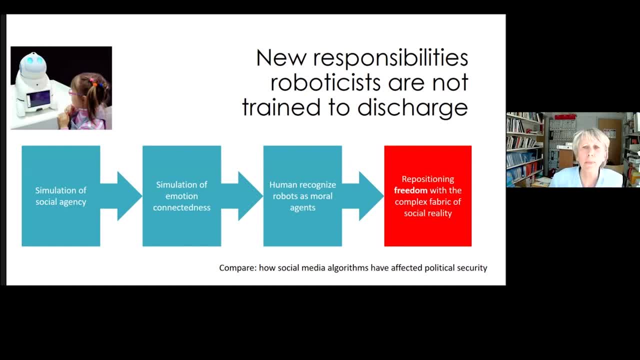 My Latest Information, Simply Because Social Reality Requires The Simulation Of Emotional Connectedness, Which In Turn Inclines People To Recognize Robots As More Patients. 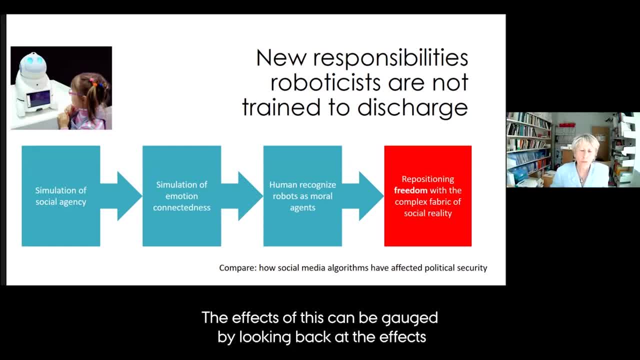 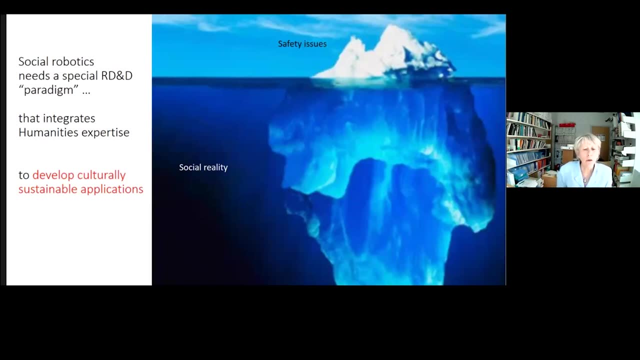 Or Even As More Agents, And That Repositions The Notion Of The Security. So Social Robotics, We Claim Needs A Special RDND Paradigm. 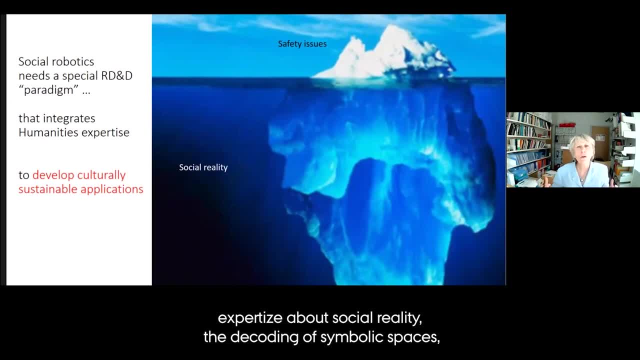 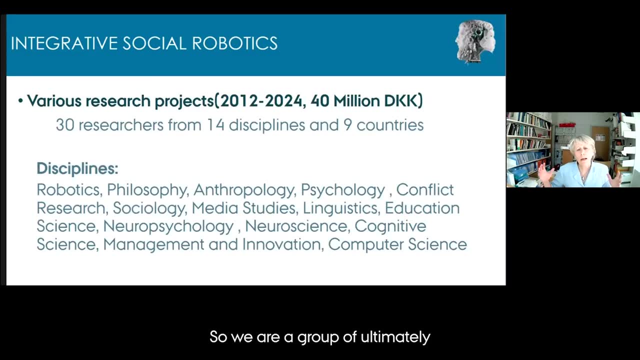 One That Integrates, Among Others, Humanities, Expertise About Social Reality, The Decoding Of Symbolic Spaces In Projects. We Have Been Working Together For The 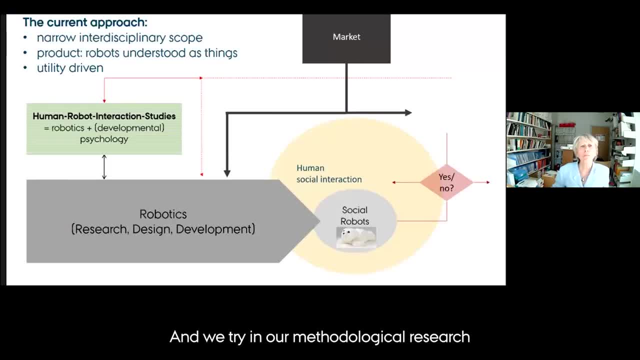 Last Ten Years And, As You Can See, There's A Wide Variety Of Disciplines Involved And We Try In Our Methodological Social Robotics. 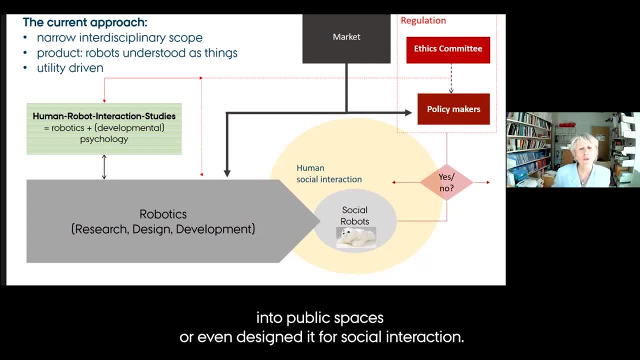 So Putting Robots- Those Of You Who Put Robots Into Public Spaces, Or Even Designed For Social Interaction. What Happens So Far Is That The 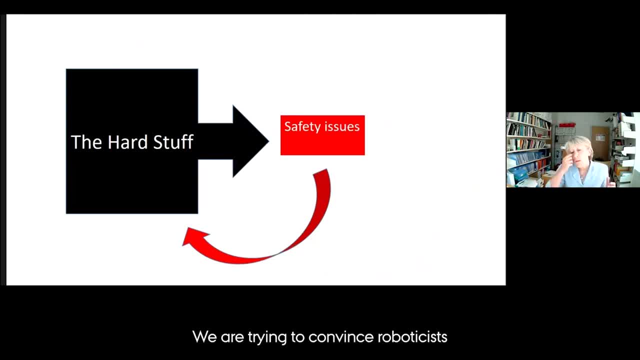 Robotics Develop. We Are Trying To Convince Roboticists To Finally Leave Behind A Simple Picture That Says We Are Doing The Hard Stuff Here. 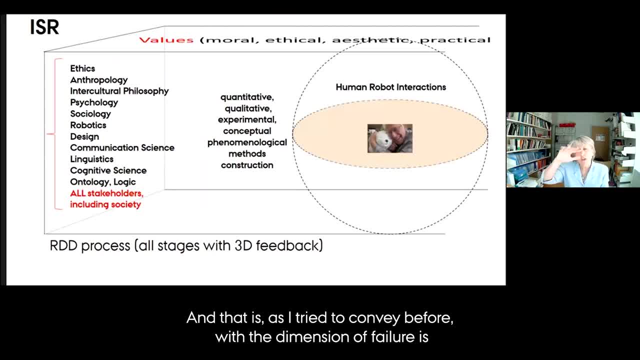 Yes, We Care About Safety Issues, But The Better Approach We Claim Is To Begin With A Multi Disciplinary And Multi Methodological Approach Where Value 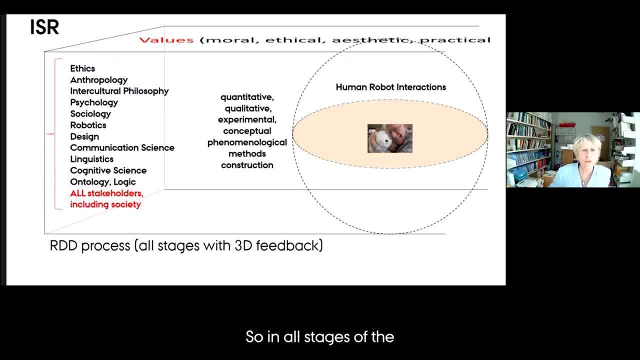 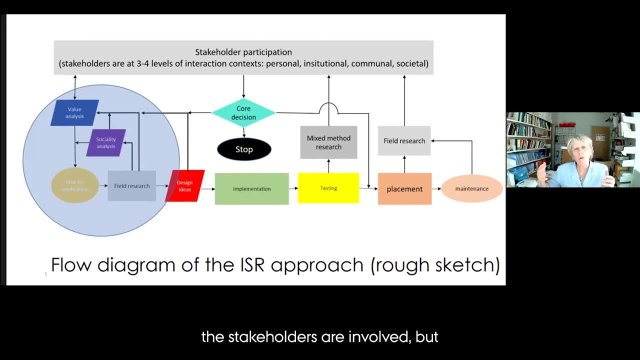 Inquiry And A Careful Investigation Of Conceptions Of Values And Practices Of The Humanities In Understanding This. Abotic Space Is Immediately Engaged From The 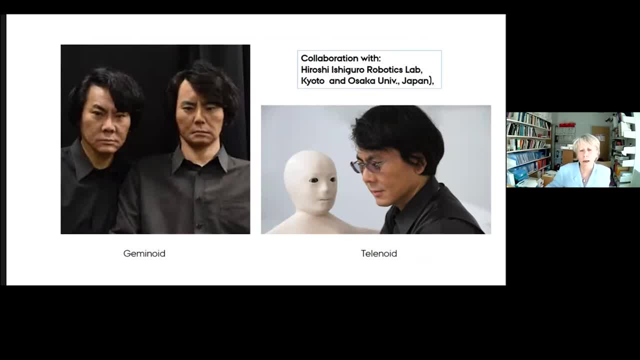 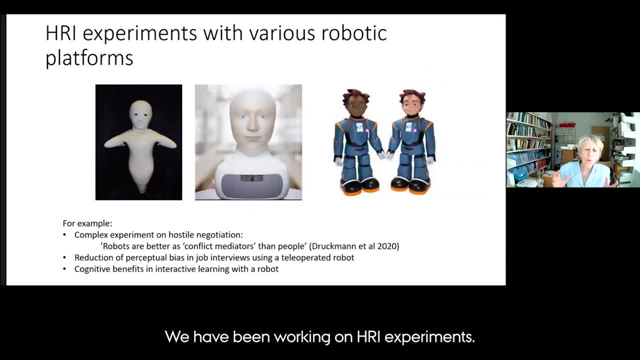 Very Beginning To The End We Work With In Collaboration With Hiroshi Ishiguro. He Has Provided Much Inspiration Where We, For Instance, Could Show. 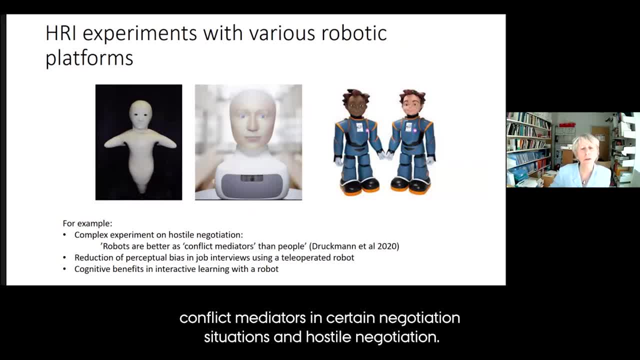 That Robots Are In Fact Better Conflict Mediators In Certain Negotiations Situations In Hostile Negotiations. We Have Investigated Whether Robots Can Reduce Perceptual 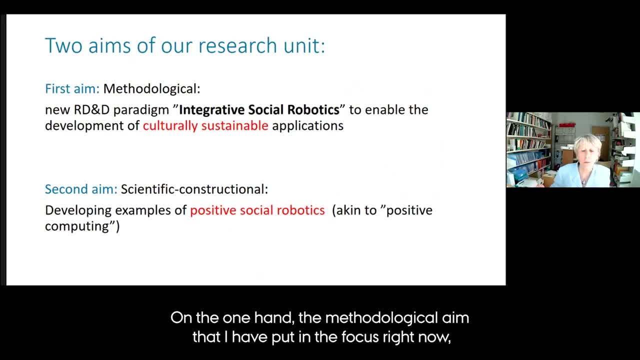 On The One Hand, The Methodological Aim That I Have Put In The Focus Right Now. We're Trying To Communicate And Invite People, And 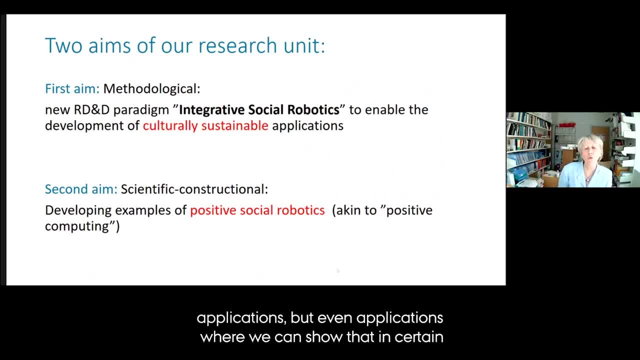 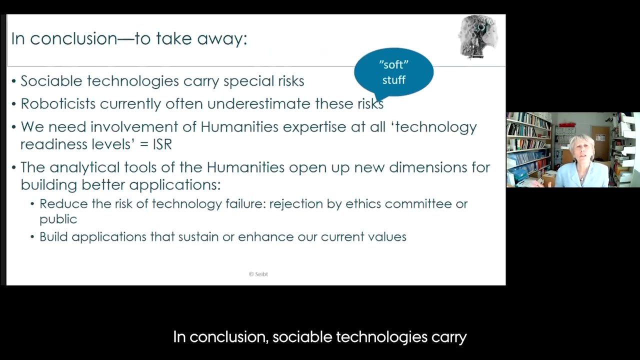 Convince People To Explore With. In Certain Cases, Robots Can Do Something That Humans Cannot Do, So That Is Positive. So Robotics Where The Robots 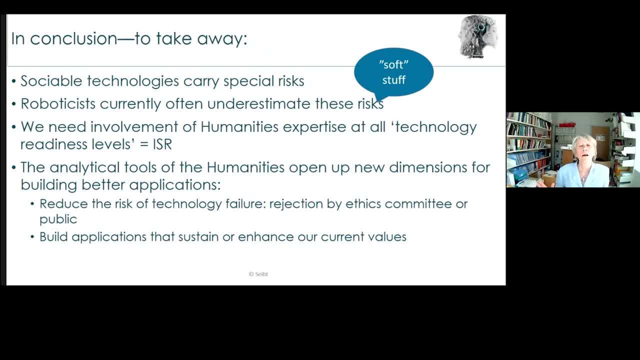 Actually Not Only Sustained, But Even Enhanced A Cultural Value Kind Of Responsibilities They Carry. Roboticists Are Not Trained To Discharge These New. 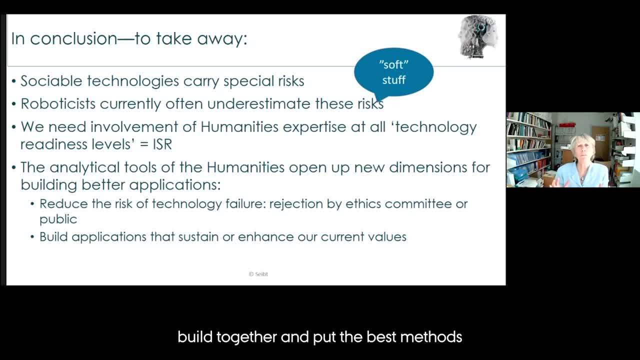 Responsibilities. We Need To Collaborate In Order To Build Together That The Best Methods Together Put The Model In The Core Of The Symbolic Spaces. 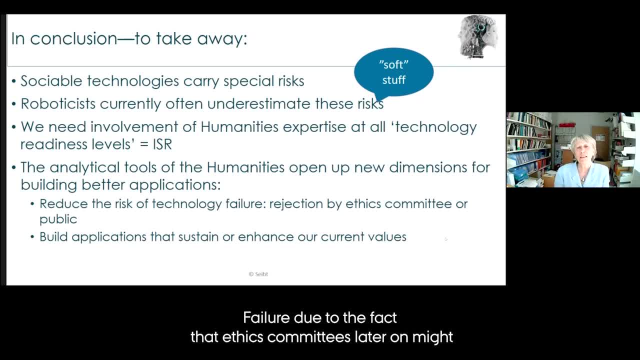 The Social Cultural Complex. Failure Due To The Fact That Ethics Committees Later On My Find Some Reason To Reject The Application. Let Us Join Our 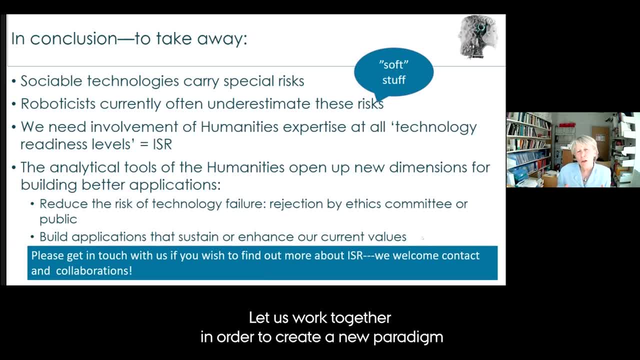 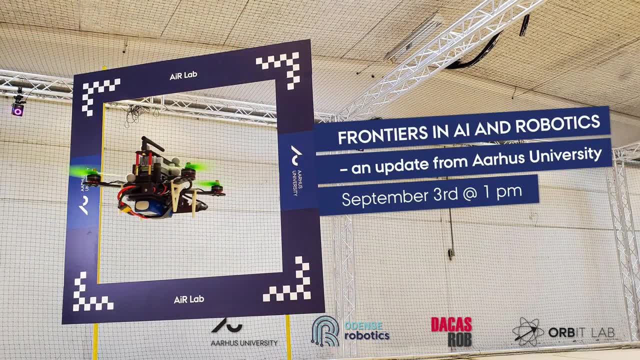 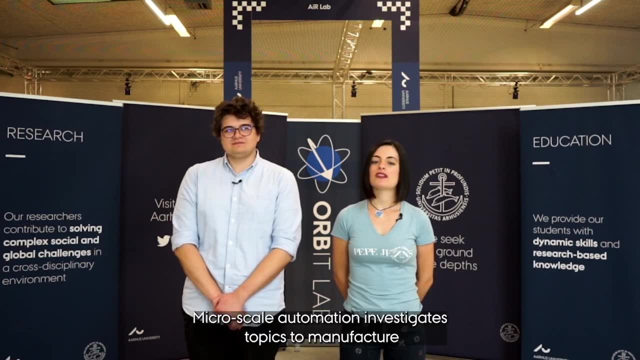 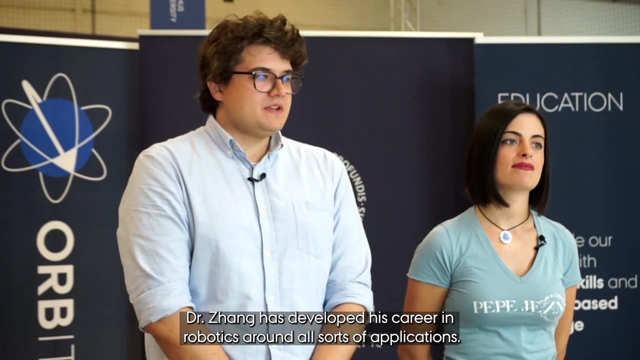 Forces. Let Us Work Together In Order To Create A New Paradigm For The Development Of Robotics Applications. Thank You Very Much. Despite Fascinating Developments, 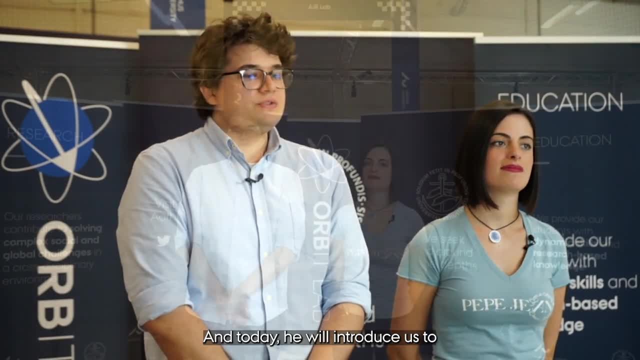 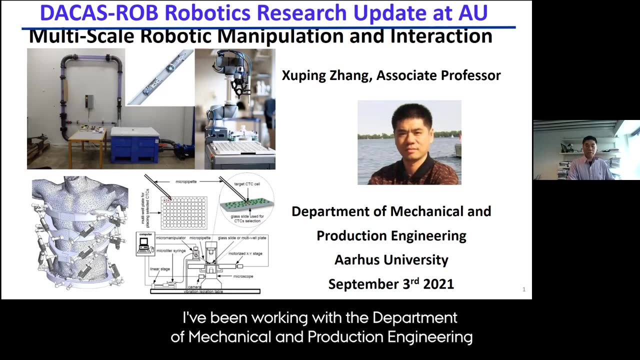 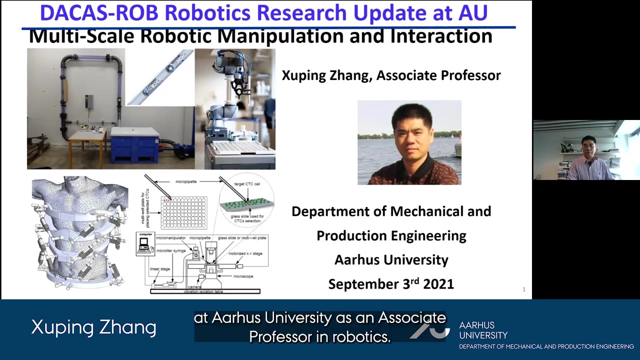 Robotics Around All Sorts Of Applications, And Today He Will Introduce Us To His Research In Biomedical And Manufacturing Engineering. So My Name Is. 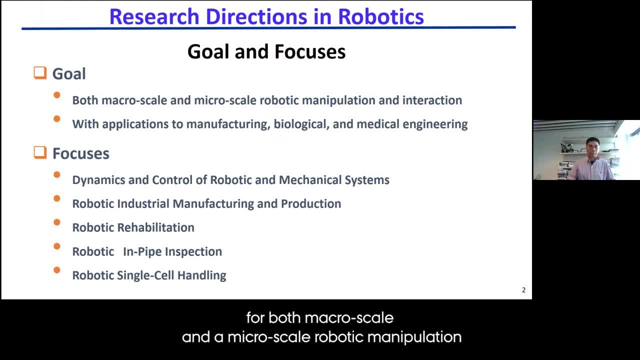 Shu Pinzang. I'm Working With A Robotics And The Interaction With Application To Manufacturing, Biological And Medical Engineering. My Research Efforts Consists Of: 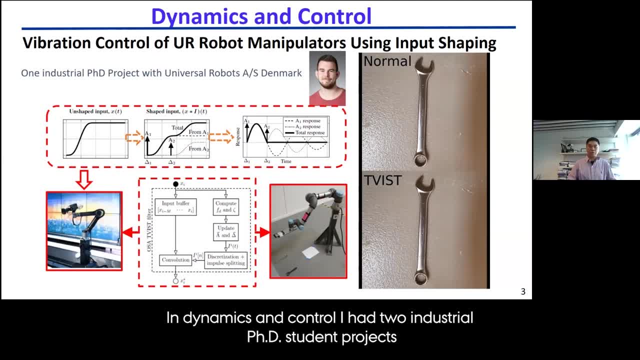 Five Research Directions As Below. In Nam Is Control. I Had Two, So First Project With Universal Boss Is A Vibrating Control Of You Are. 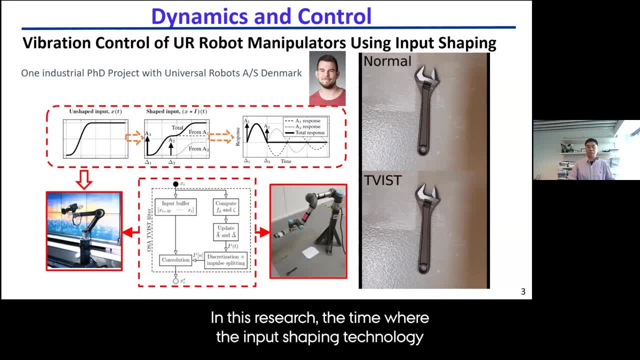 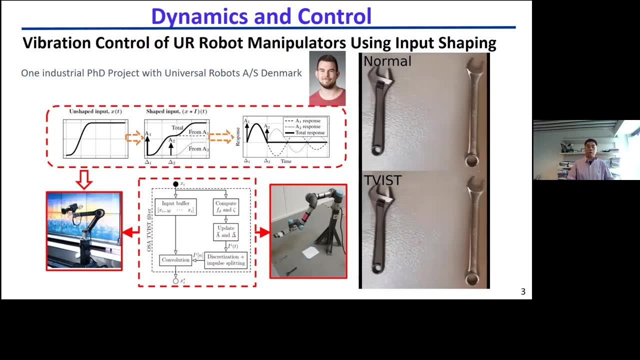 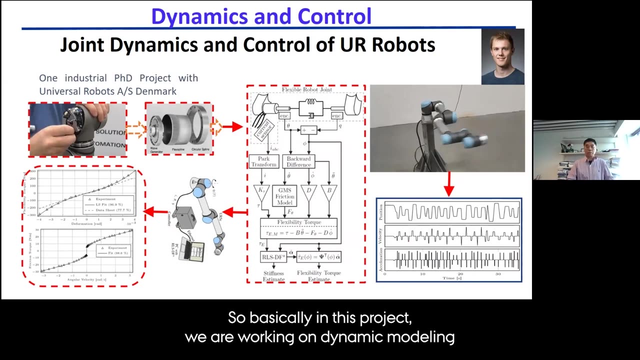 Robots, Manipulators Using A Input Shipping Technology In This Research, The Time Where The Input Shipping Technology Vibrations Of You Are Robots And Showing These. 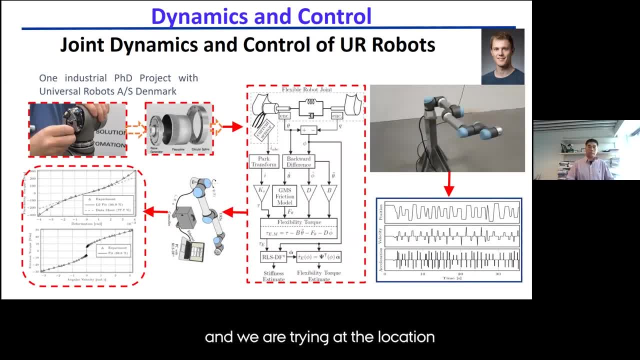 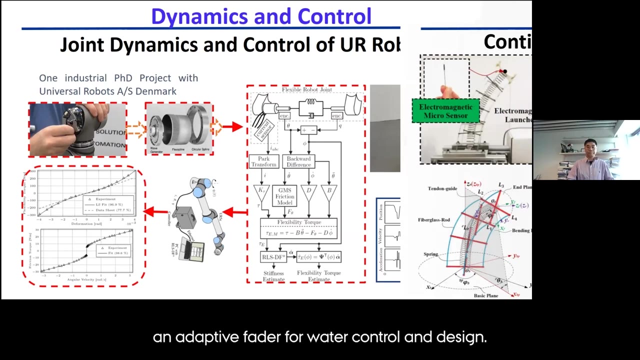 Videos. So Basically In This Project We Work On Dynamic Modeling And Real Time At The Location Of The Stiffness And Adaptive Fit For Water. 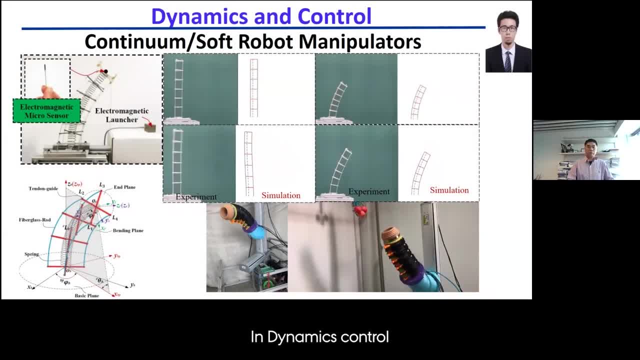 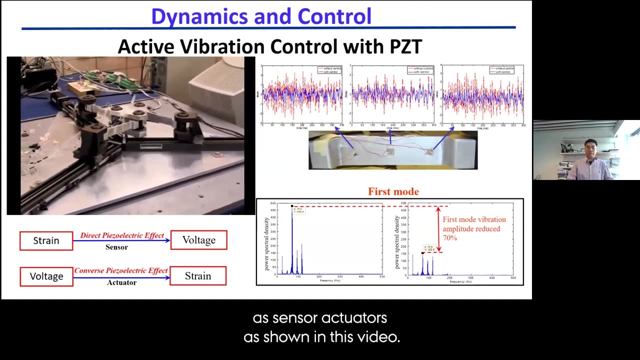 Controller Design In Dynamics Control. We Are Also Working On Soft Robot Manipulators And Showing The Video Slide. Active Vibrating Control Using Piezo Electrical. 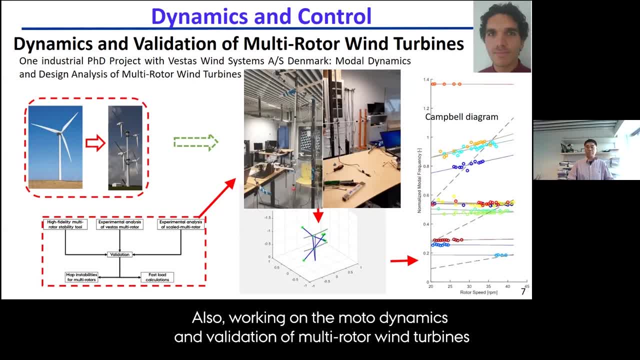 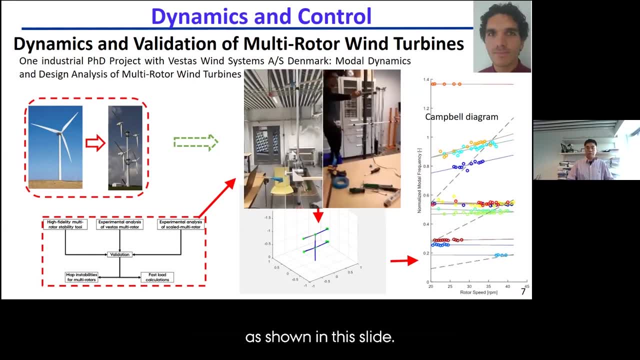 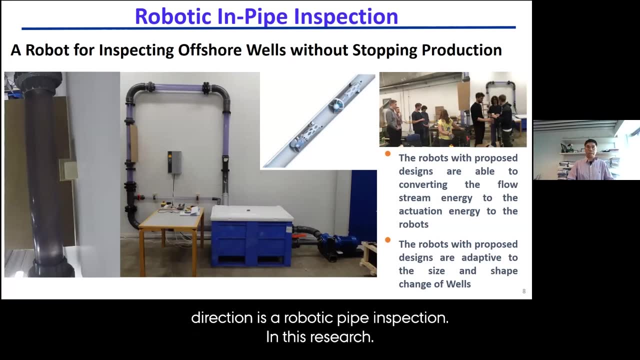 Material. We Are Working At The Location Of Multi Route Of Turbines Cooperating With Western Winter Systems, At Show In This Slide. My Second- 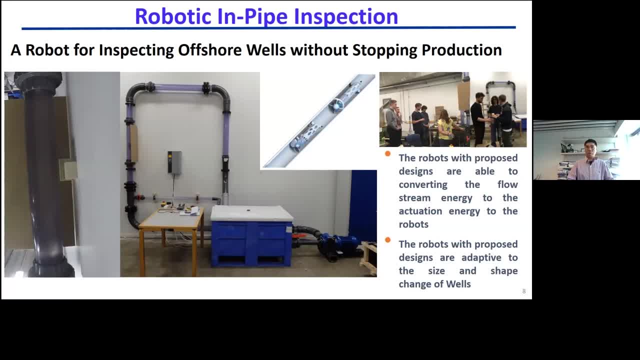 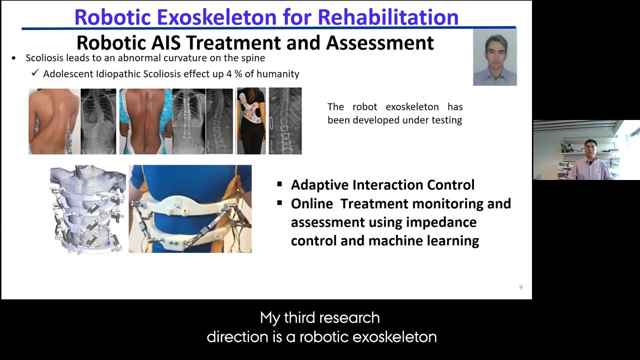 Research Direction Is A Robot In. The Robot Is A Waterproof And Is Able To Convert The Flow String Energy To Activation Energy, So That Robots 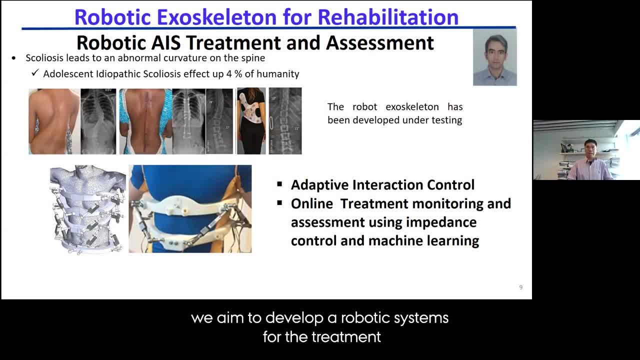 Can Move Against The Flow String, As Showing This Slide Is A Kind Of For Spine Psychosis, So We Focus On The Adaptive Interaction Control. 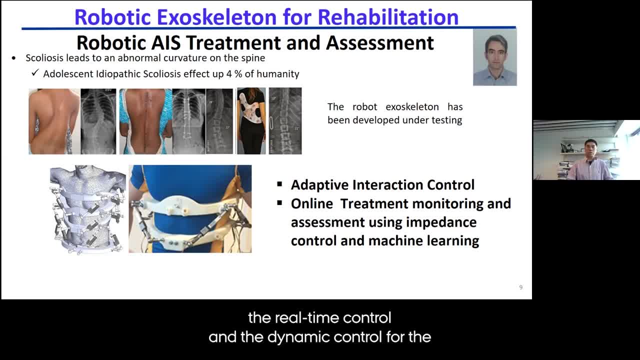 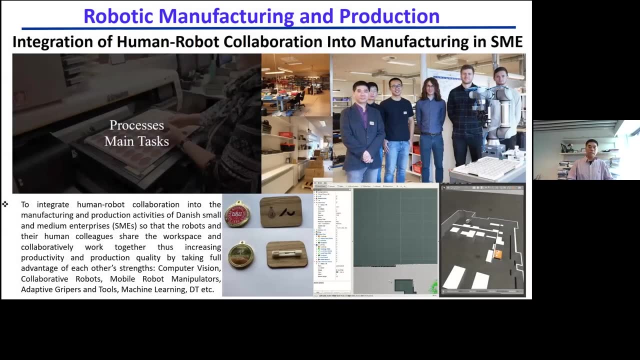 Between The Robotic Exoskeleton And The Patient And So That We Can Achieve The Realtime, And My Research Efforts Mainly Focus On 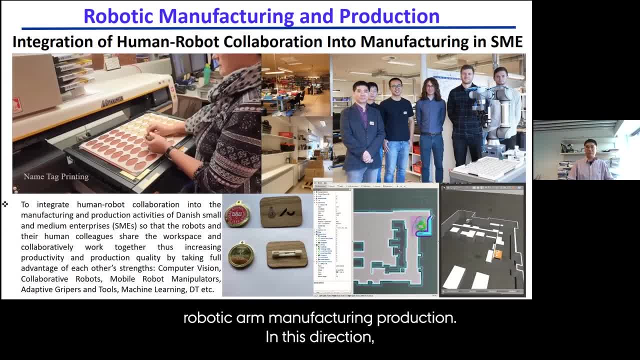 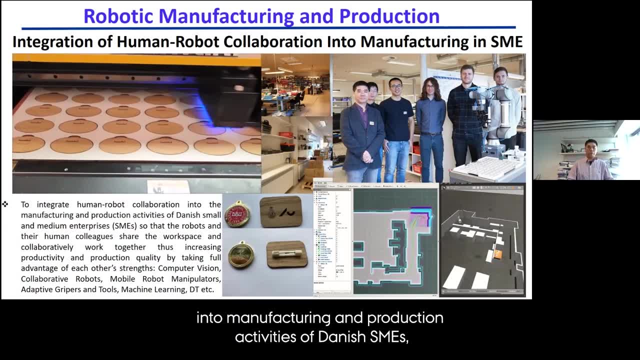 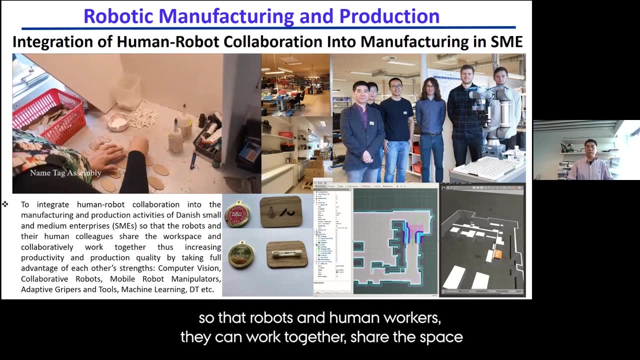 The Fourth Direction: Robotic Manufacturing Production. In This Direction, We Aim To Integrate Human Robotic Collaboration Into Manufacturing And Production Activities Of The Productivity. 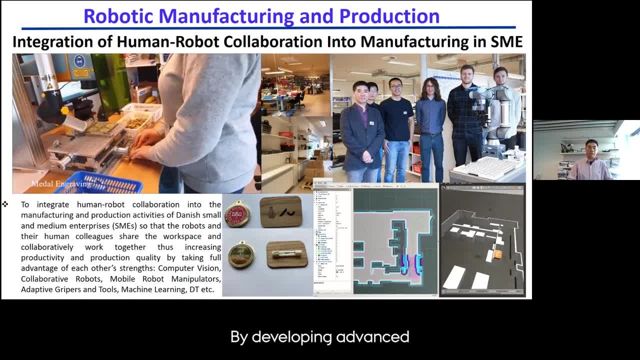 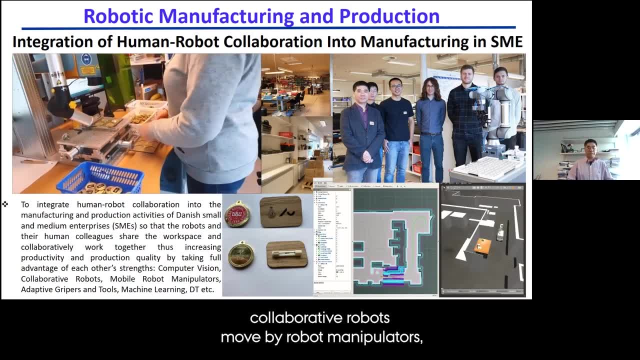 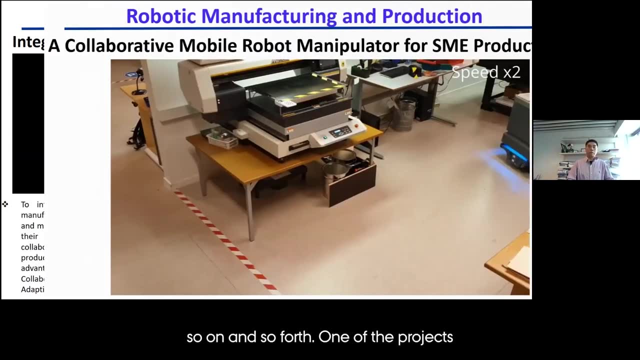 And Production Quality By Developing Advanced Technologies In Computer Vision: Correcting Robots Moved By Robot, Manipulators, Adaptive Reapers And Tools, Machine Learning And Determining. 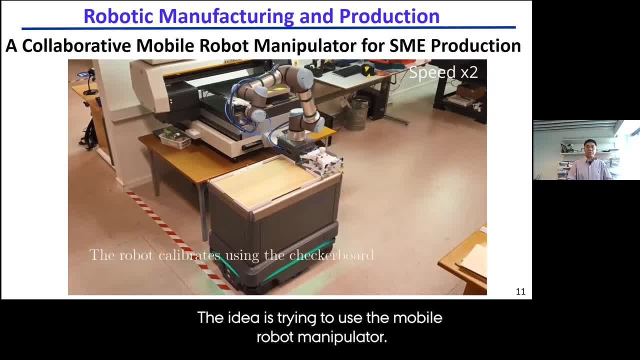 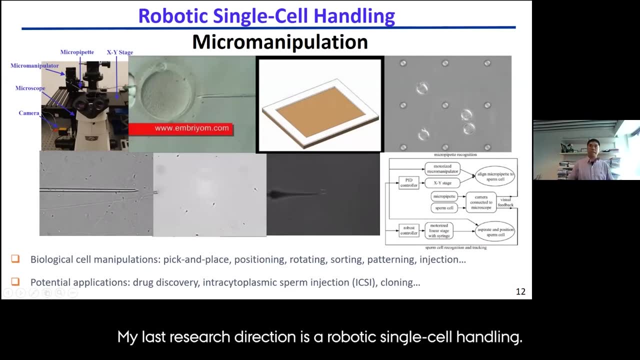 So Not So Is Trying To Use The Mobile Robot Manipulator To Automate The Process Of The Production In This Company. My Last Research Direction. 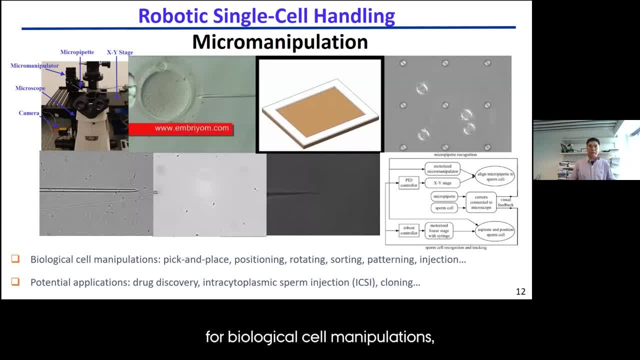 Is A Robotic Single Cell Handling The Machine, Rotating, Sorting, Patterning And Injection, With The Application To Drug Discovery, Clothing And Ecstasy. So 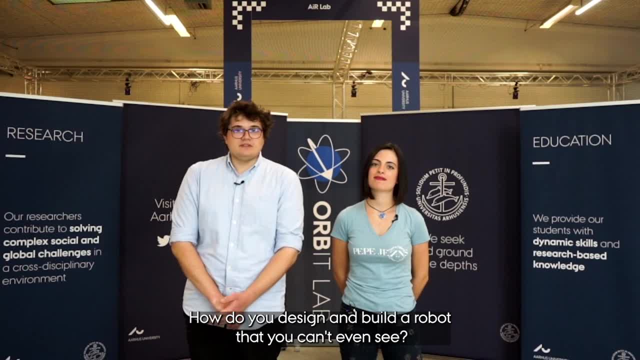 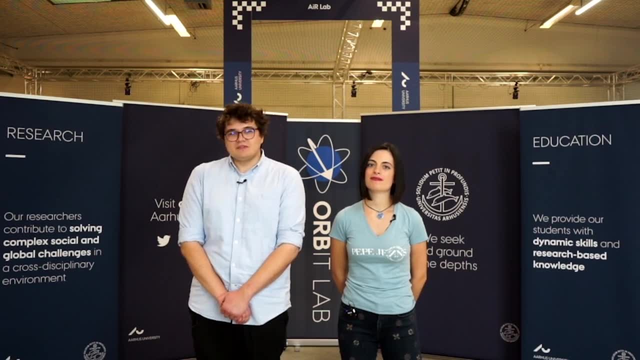 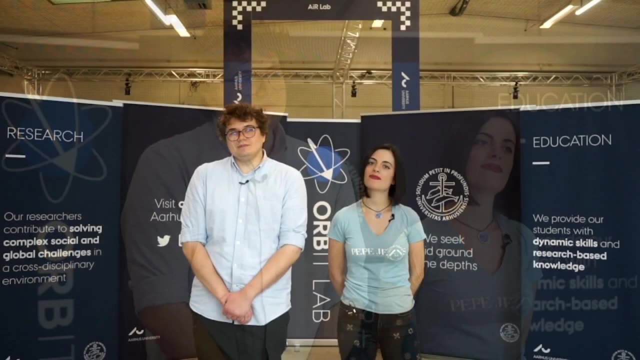 And With That Thank You Very Much Your Attention. How Do You Design A Robot Capable Of Transporting Payloads And Targeting Cancer Cells Specifically? 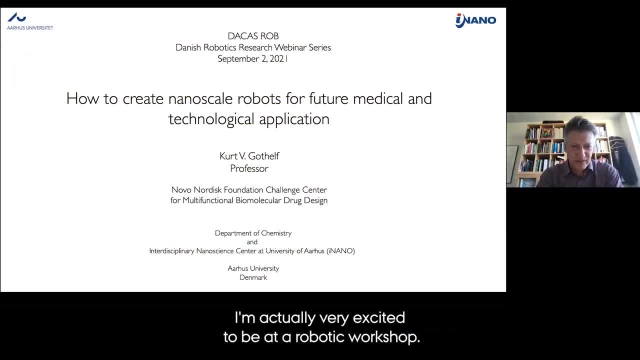 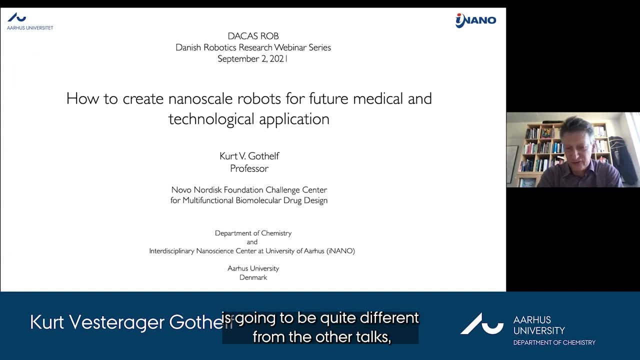 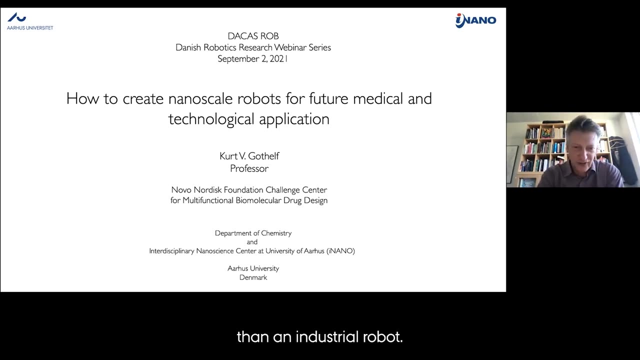 Professor Gold Health Will Introduce Nanoscale Robotics And The Recent Progress. Thank You Very Much For The Introduction Robot. So I'm A Professor At. 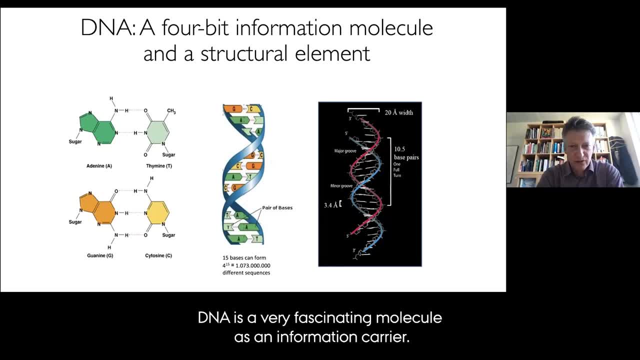 I Nano And I Have A Background In Chemistry And We Work With Dna. Dna Is A Very Fascinating Molecule As An Information That 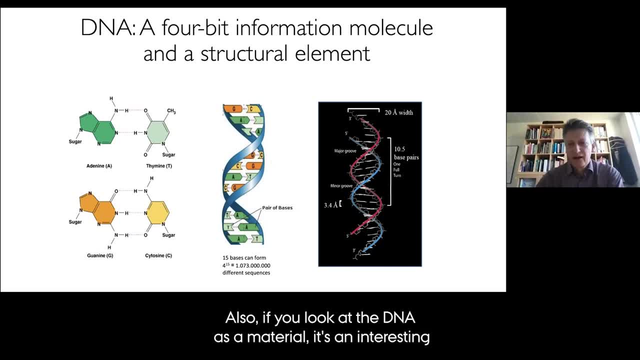 Sequences, So You Can Store A Lot Of Information In Dna. Also, If You Look At Dna As A Material, It's An Interesting Nano. 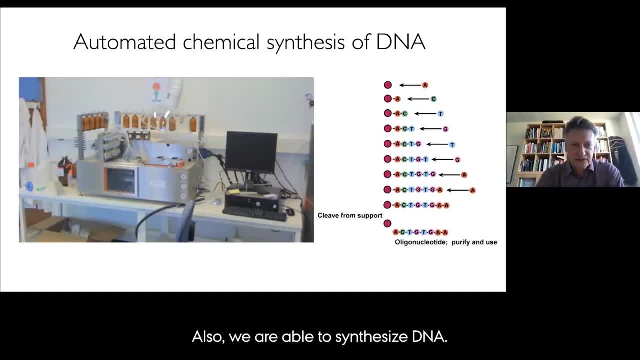 Material That Is Both Dna. This Is Actually A Synthesizing Robot From My Laboratory Where You Can Just Code In The Sequence On A. 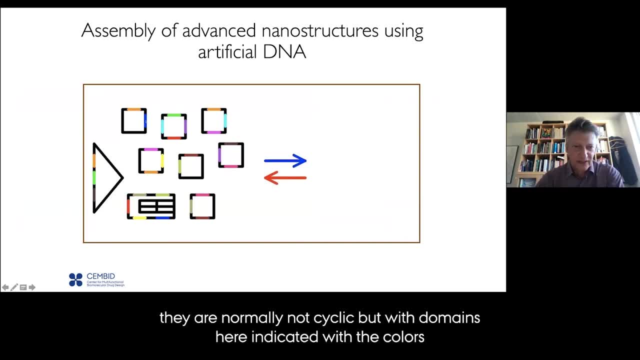 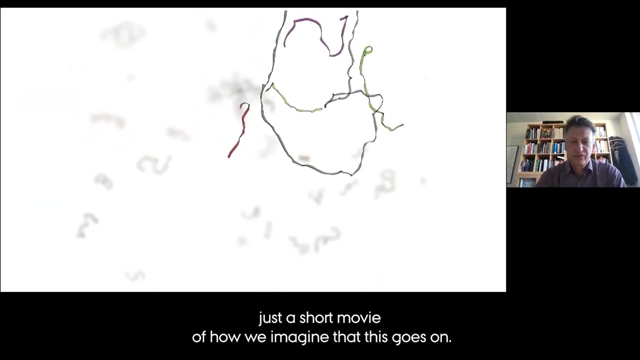 Computer, And Then The Instrument Will Make The Desired That They Fit Together And Can Pair Up, And Then You Can Program Different Dna Molecules. 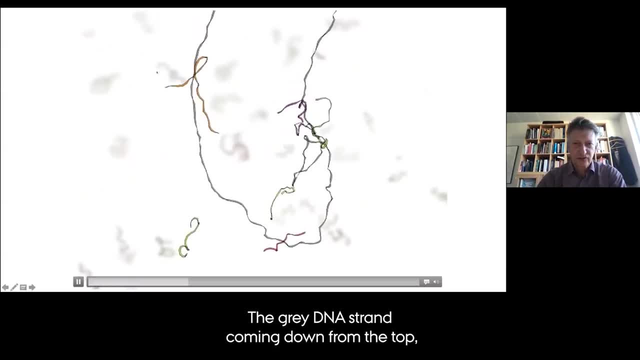 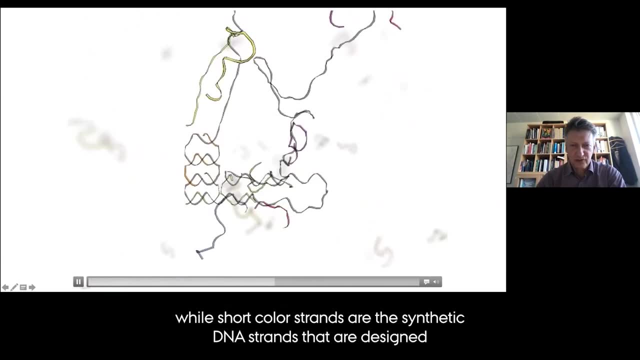 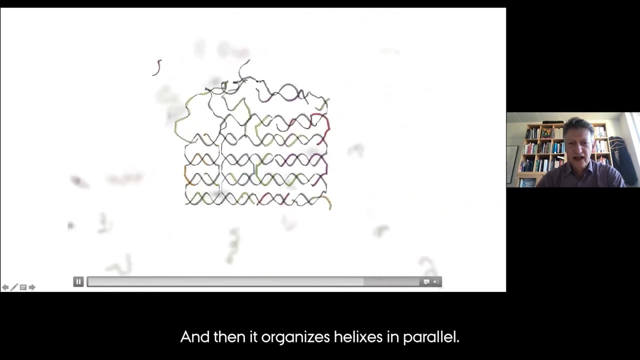 To Assemble Here, Shown By House, But To A Lot Of Different Structures Designed To Match The Sequence Of The Long Dna Sequence Here. 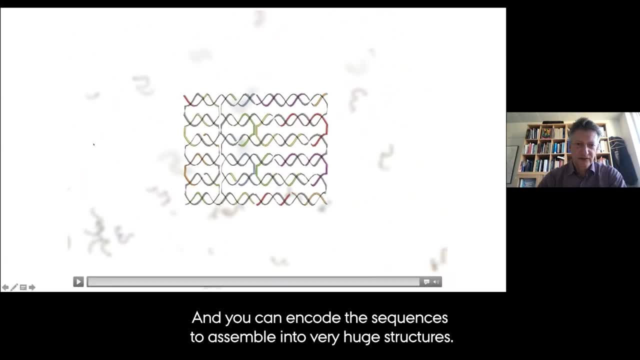 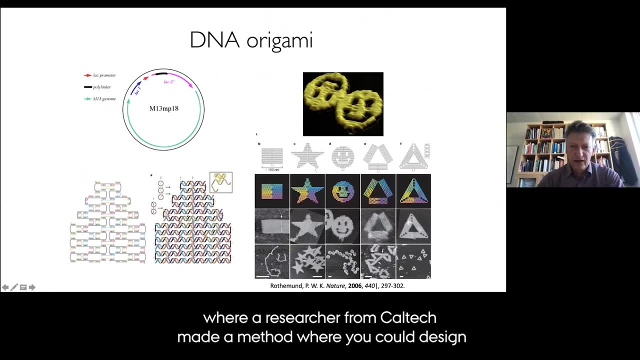 And Then It Organized Helices In Parallel, And They Are Kept Together By These Crossovers Between The Helices And Below Here In The 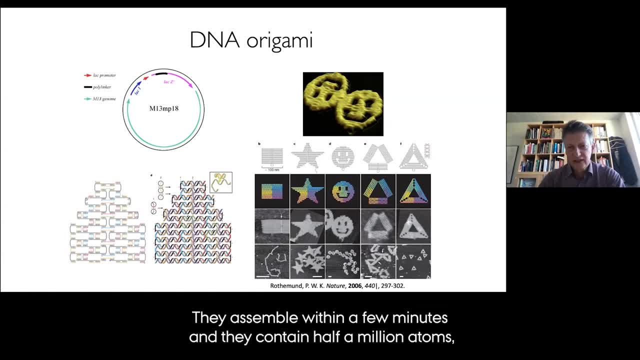 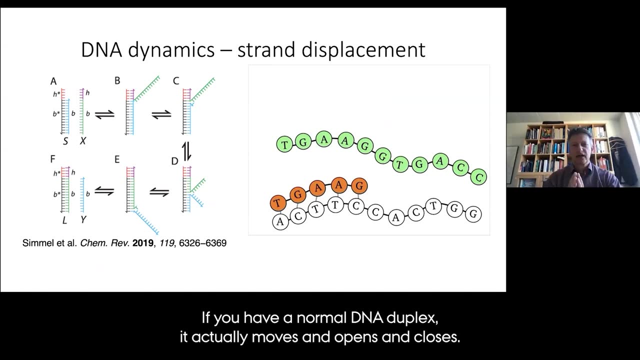 Second Room You See Actual Images Of These Structures That Are Self Assembled. They Assemble Within A Few Minutes And They Contain Half A. 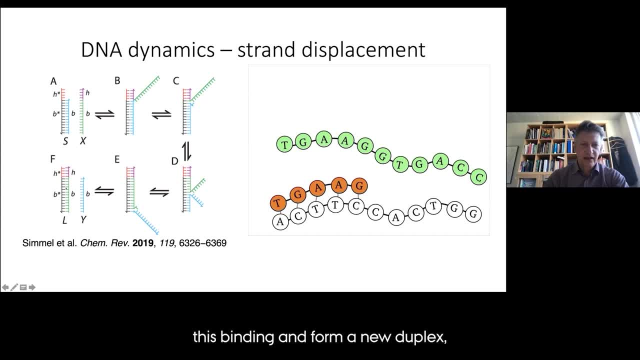 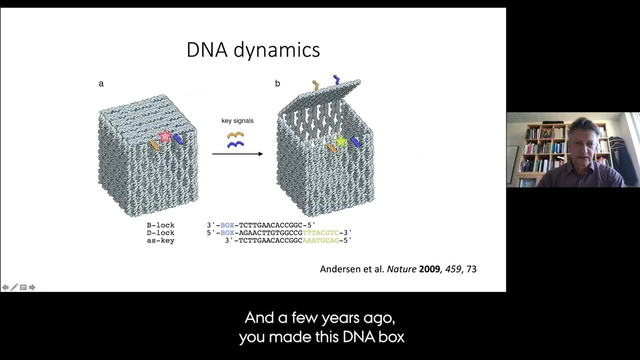 Whole Here. It Can Actually Out, Compete This Binding And Form A New Duplex, As Showed In This Primitive Video Here, Where You Can. 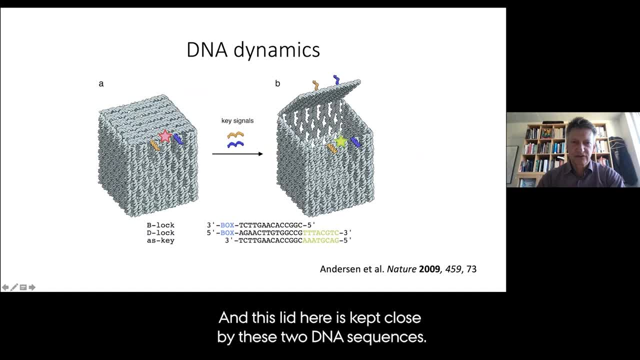 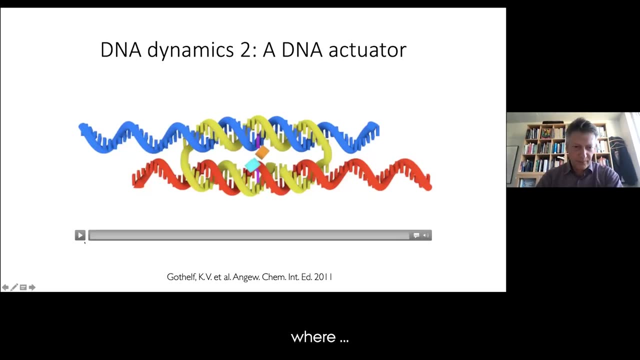 Out Compete And This Allows That To Keys. This Will Make This Strand Displacement And In This Way, Open The Box. Here's Another Design. 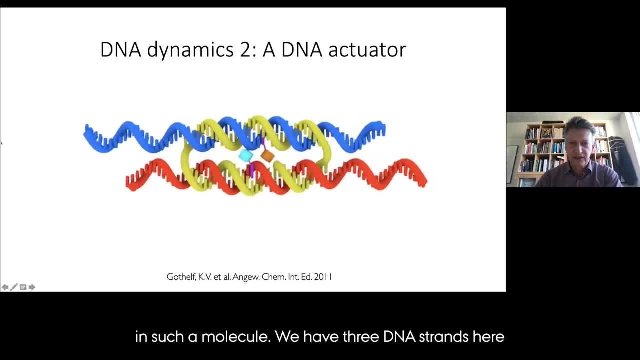 We Made Also Some Years Ago, Where We Can Have, As Mentioned, 11. Different Stages And You Can Control Exactly Each Of These Stages. 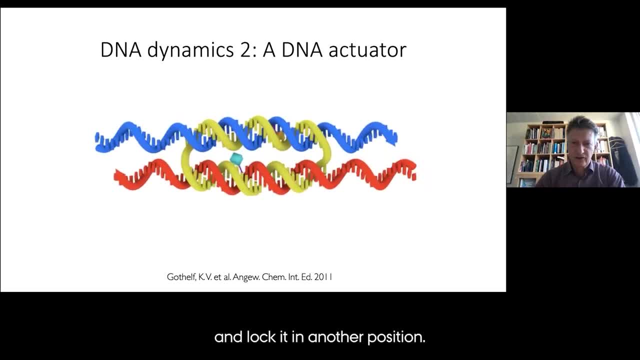 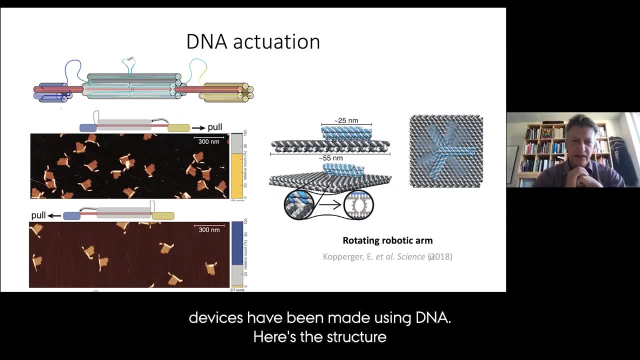 In This Type Of Actuator By Inserting Lock Strands And They'll Come Flying In The. It's Not Published Yet, But This Is What. 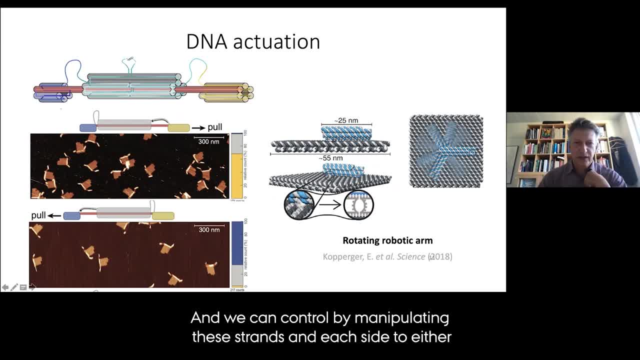 Is Called A Bowden Cable, Like The Cable You Have In A Handbrake On A Bike, Where You Have A Hosing And Where They 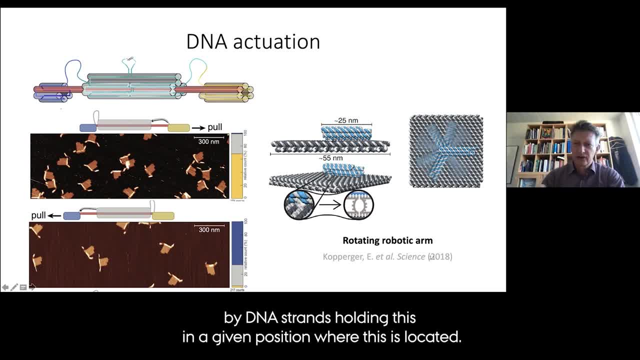 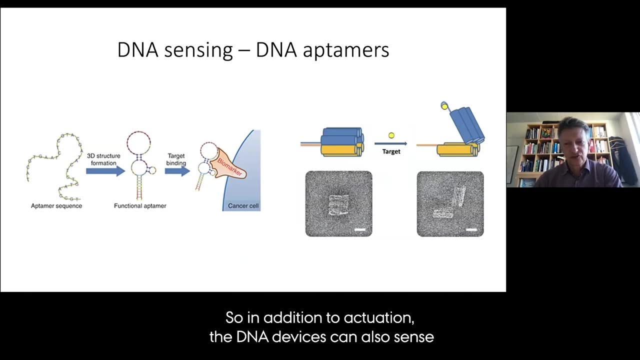 Can Control By DNA Strands Holding This In A Given Position Where This Is Located, But They Can Also Control This Robotic Arm From An 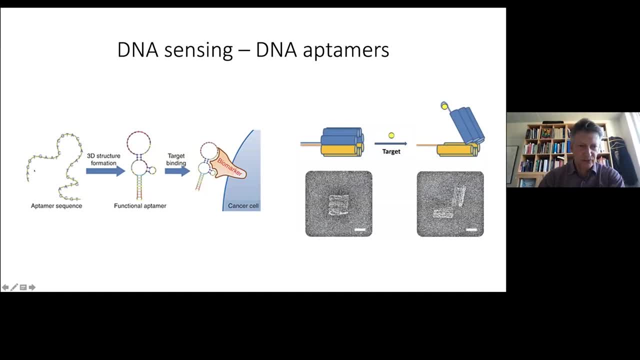 External Electrical Fields, And This Is DNA Or RNA Structures That Can Fold Into Specific Folding Structures And This Can Bind To Specific Targets. Actually, They 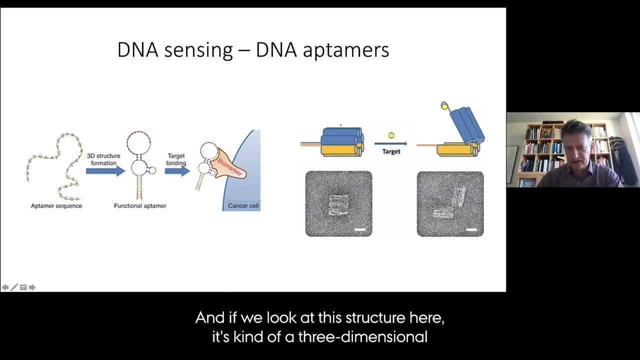 Are Selected For Specific Targets. So This Is Part Of These Six Helices That Is Parted Into The Blue Part And The Yellow Part. There's 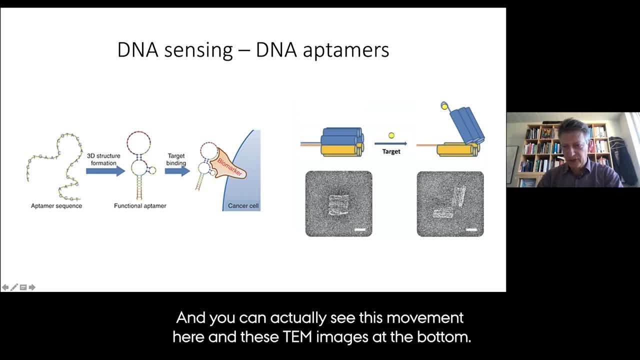 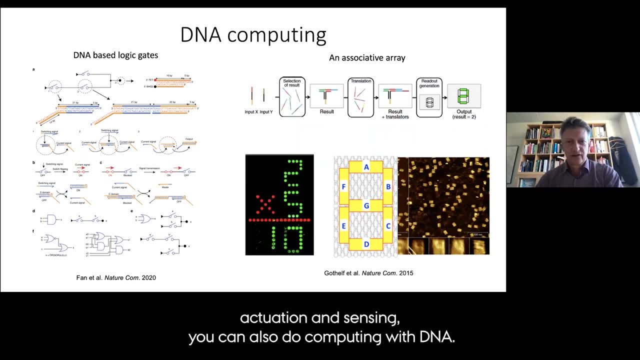 A Hinge Over Here And It's Held Together By These Placing. You Can Also Do Computing With Dna. Actually, There's A Whole Research. 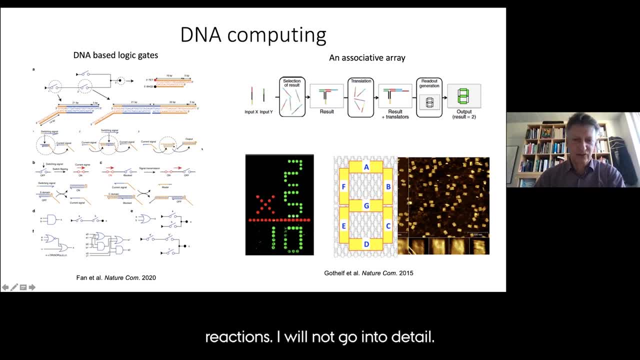 Field Called Dna Computing And In This Strand, Displacement Reactions. I Showed You You Can Actually. Yes, Gates, Org And Gates, Org, Gates And. 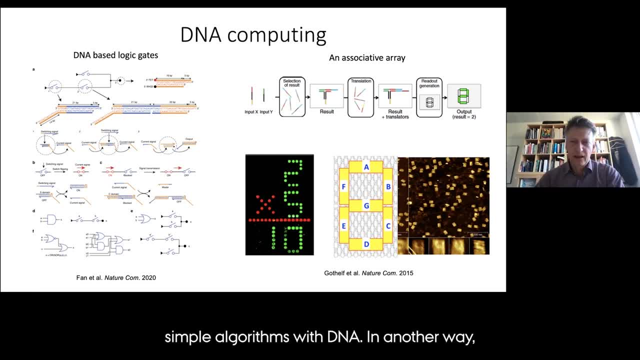 No Gates, Not Gates And So Forth, And You Can Combine Them Into Make Simple Algorithms With Dna In Another Way To Do This Result. 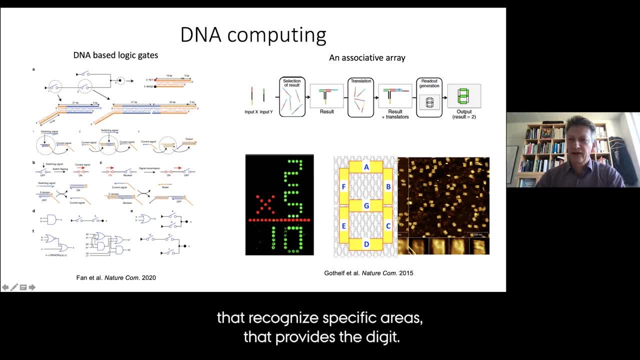 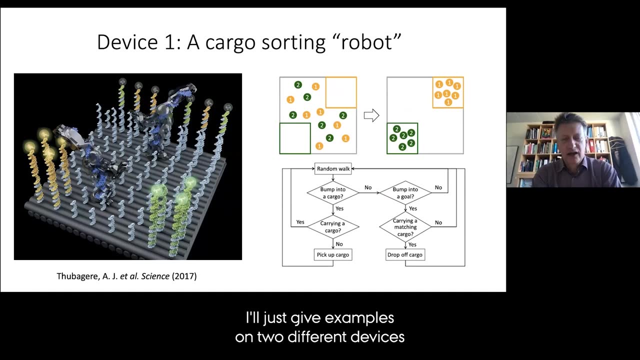 Can Then Be Translated Into Something That Can Give An Output That Recognize Specific Areas. That Provides A Digit. In This Way, We Can Select. 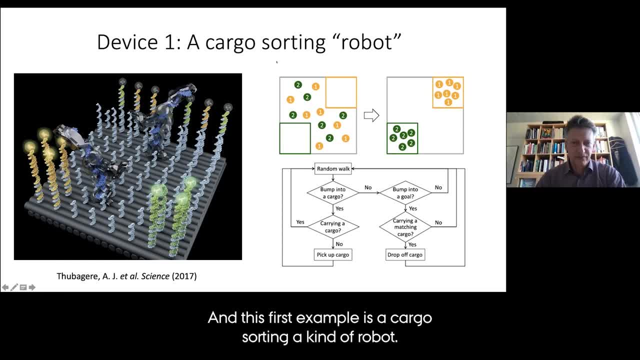 This First Example Is: Is A Cargo Sorting Kind Of Robot. Here Again The Gray Structure, Here Is An Origami Structure, And Then You Can. 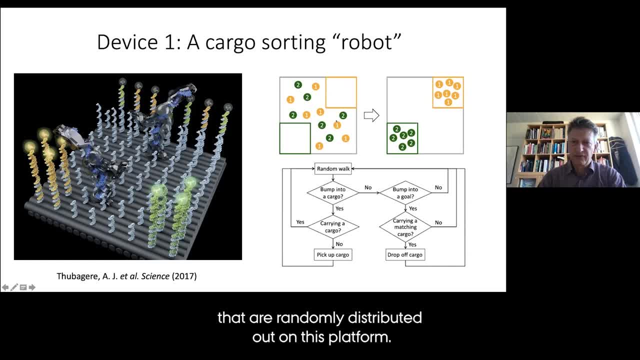 See There Are Lots. Then We Have The Robots That Do Random Walks And By A Simple Logic Scheme Here Of Operations, It Can The 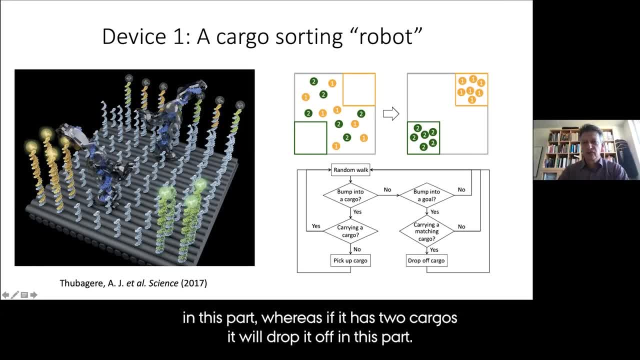 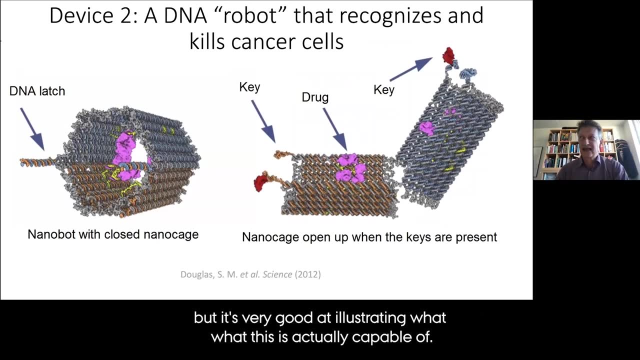 Logic Random Walk. If It Bombs Into A Barrel, Then We Can See The Barrel Inside The Barrel, And Here We Can See A Robot. 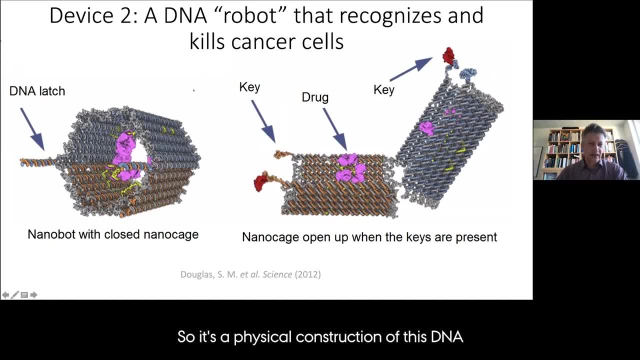 That Can Recognize And Kill A Cancer Cell. So It's A Physical Constructed, This Barrel. We Have A Protein And Antibody, A Drug And 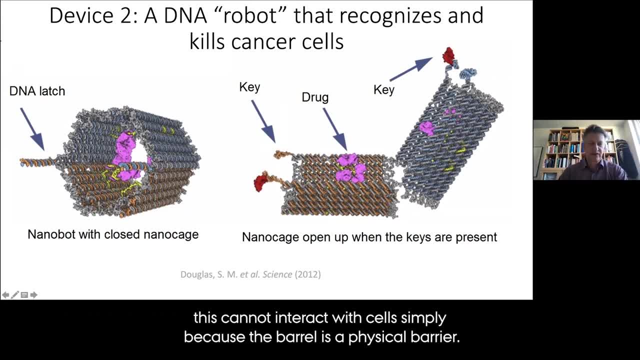 This Has The Ability To Recognize What Is Called A Death Receptor On Cells. So If This Interacts With Cells, They'll Unlock And In. 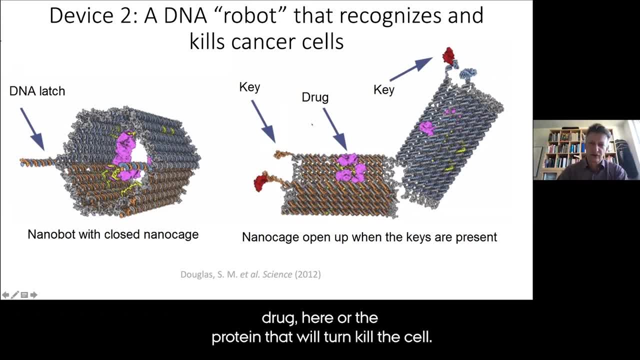 This Way Give Access To The Drug Here, The Protein That Will In Turn Kill The Cell. So This Has Been Done On Just A Area. 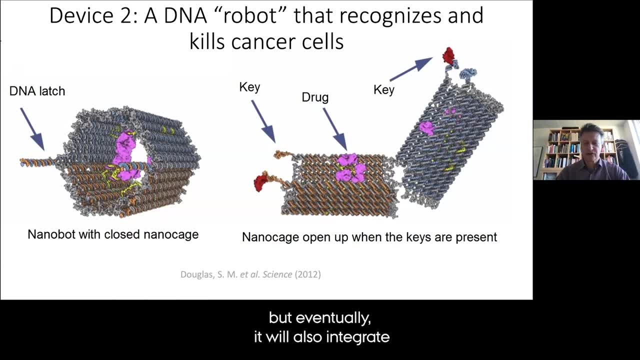 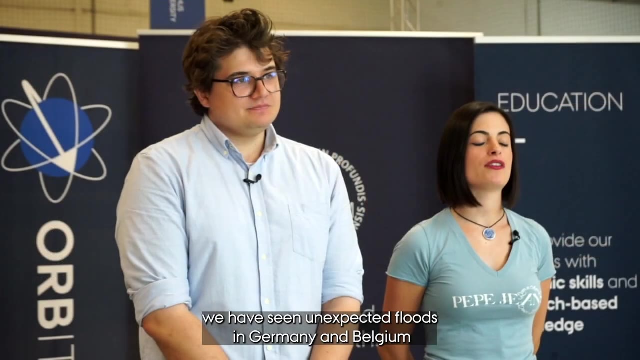 Where More And More Smart Drugs Are Made- Not As Smart As This, But But But. Eventually It Will Also Integrate Small Algorithms And Fields. 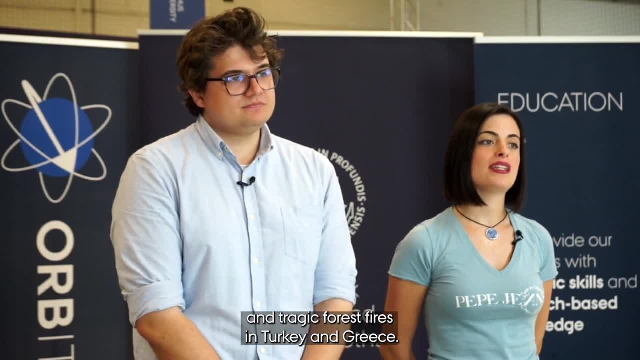 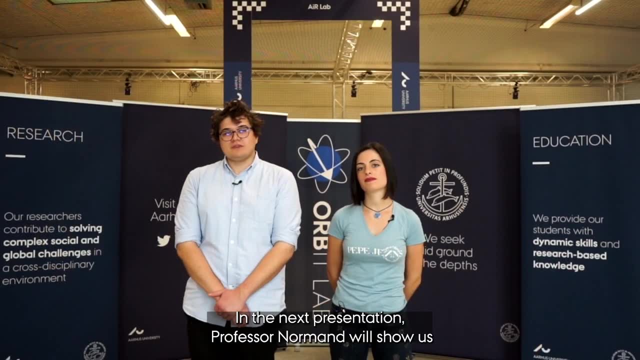 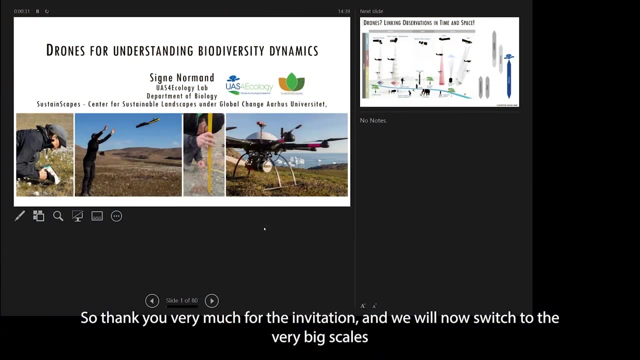 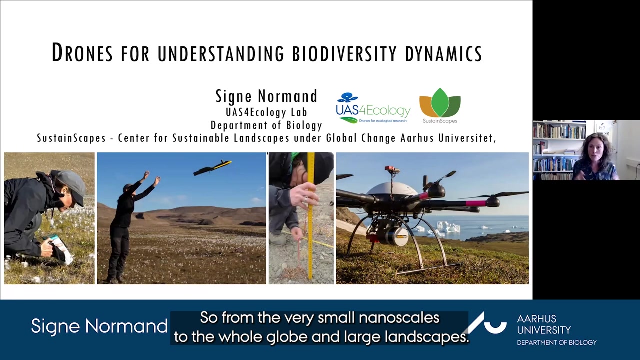 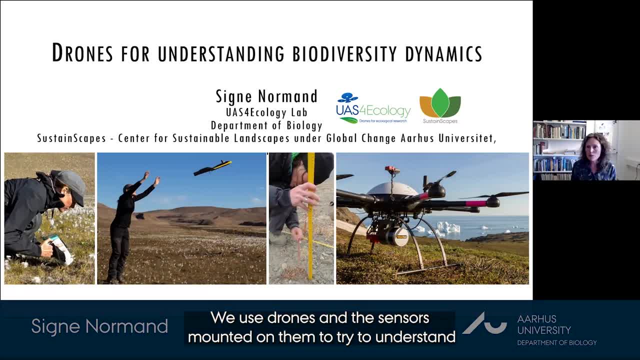 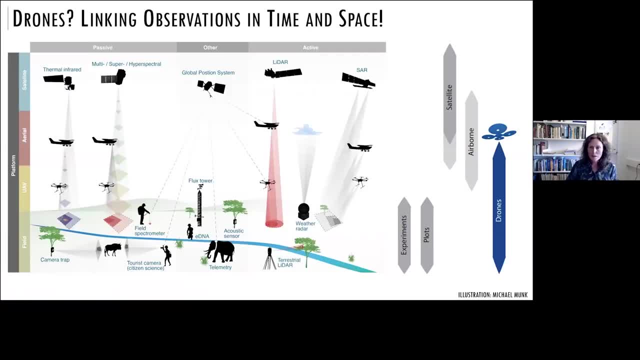 To To To To To diversity, dynamics, So the dynamics of life on Earth, And we use drones because they provide a link between the field-based observations we do as ecologists and biologists with information gathered from satellite sensors, But it's basically the essential for us, are not the 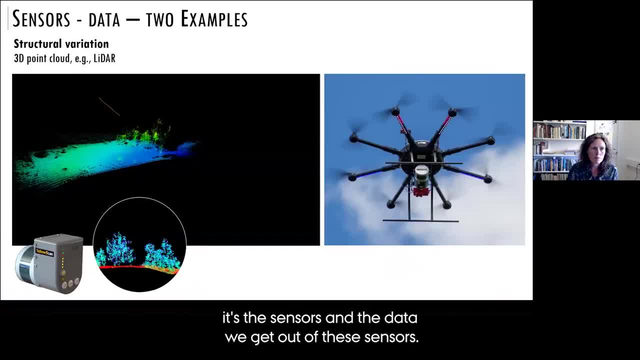 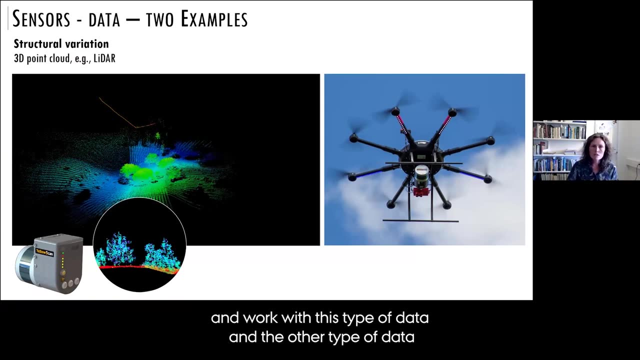 drones. it's the sensors and the data we get out of these sensors And overall we just use two different types of sensors, So LiDAR or point cloud data. So, as you see an example here, we mount the LiDAR sensor on the drone and work with this type of data And the other. 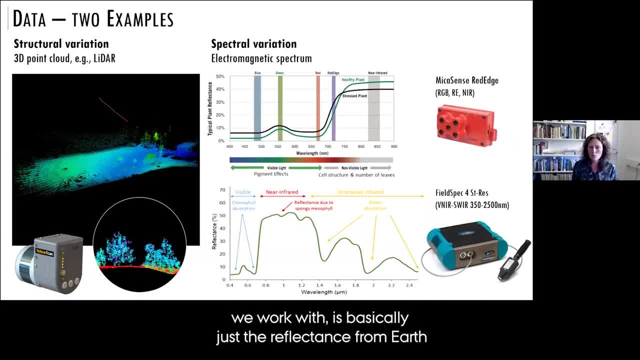 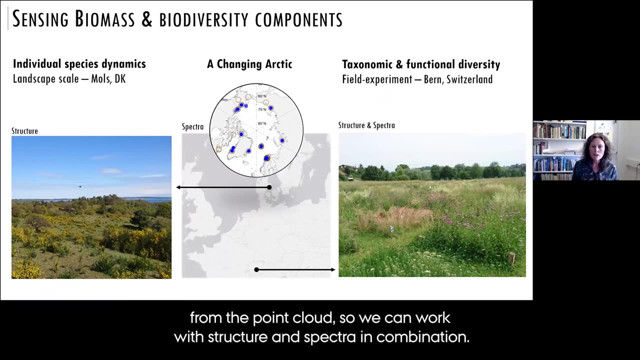 type of data we work with is basically just the reflectance from Earth and in the electromagnetic spectrum. We use different sensors to gain this information. And this type of information we can either combine or we can work. So we can work solely with the structure gathered from the point cloud. So we can work with 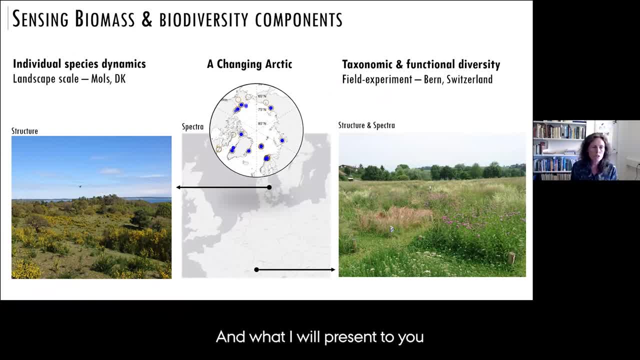 structural spectra and combination, And what I will present to you today is just three small case studies where we have used this data. So one from Denmark, out in the malls landscape, one from a changing Arctic- so the whole Arctic area- and from a field experiment. 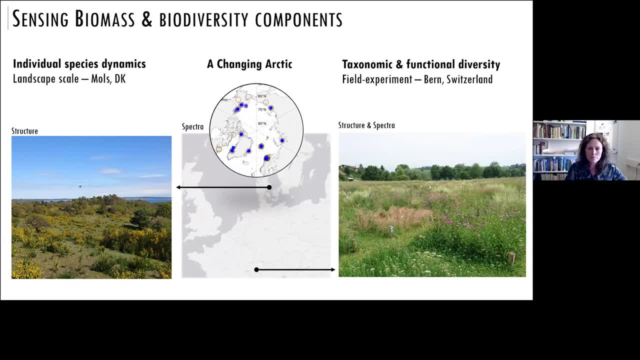 where we try to understand and map biodiversity in Switzerland. So out at MOLS, we have a very long view of the Earth, and then we have a little view on the planet. So the And now we'll take a look at the images that we've seen and put it out there. So the first one, 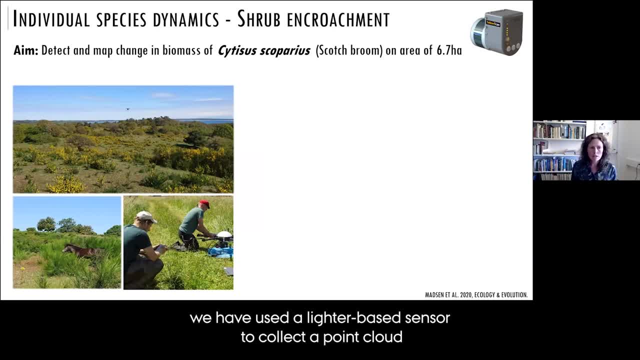 here. This is another example of the geological analysis of the Earth. This is a model that we're using in the Columna Nulation. This is a data of the Earth, So the example used a LiDAR-based sensor to collect a point cloud across the landscape of this species. 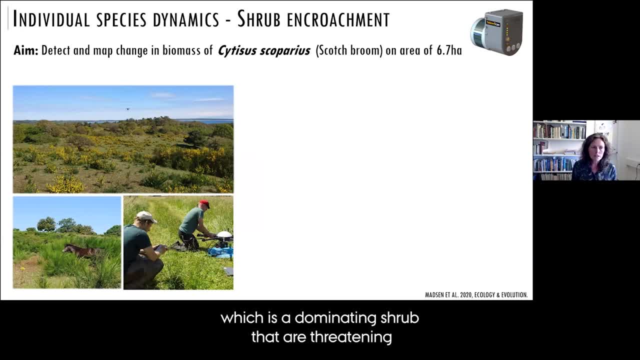 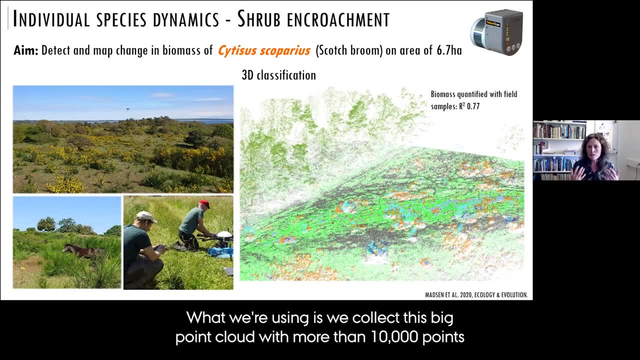 Hytisus that you see here in yellow, which is a dominating shrub that are threatening biodiversity in the area. What we're using is we collect this big point cloud with more than 10,000 points per square meter, and then we use machine learning to recognize the individuals of. 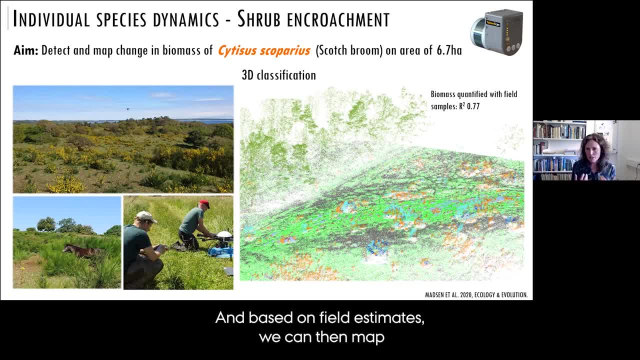 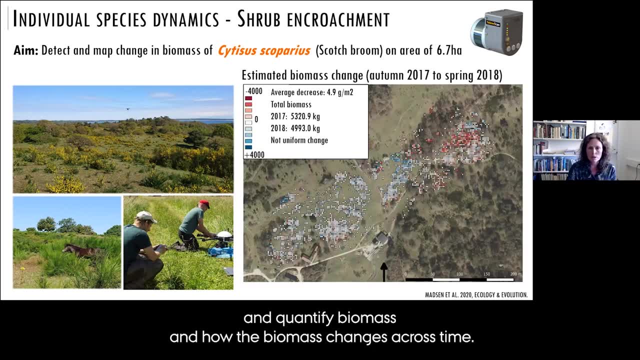 these shrub species in the point cloud and based on field estimates we can then map and quantify biomass and how the biomass changes across time. So that provides us with the possibility of estimating which areas are increasing in biomass and which areas are decreasing in biomass. 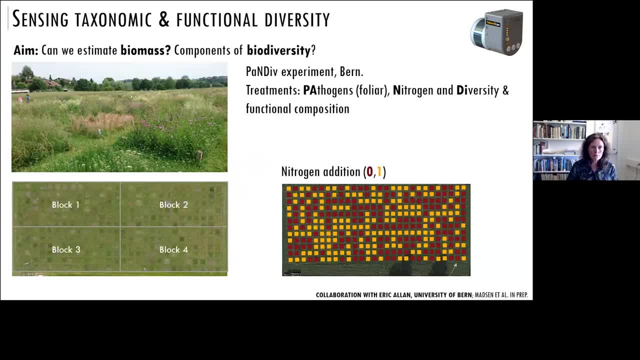 in this area. So that was the first example. The second example: we use the same type of tracking, перемафل data- in a biodiversity experiment, So trying to see if we can quantify how many different species- in this case plant species- we find in this experiment And also quantify the 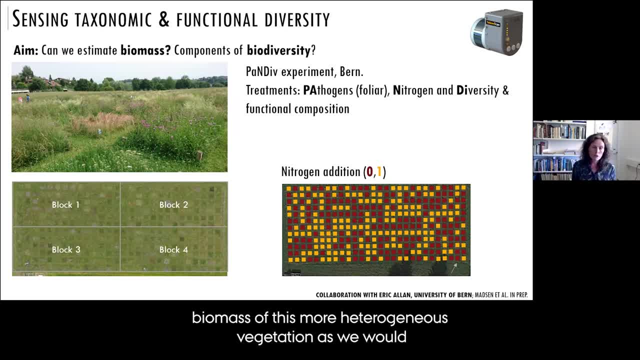 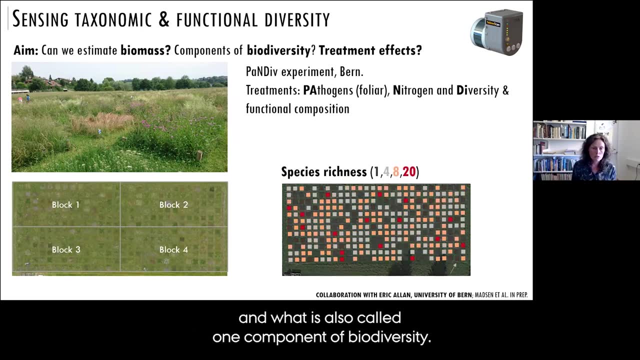 biomass, of this more heterogeneous vegetation, as we normally and as we would normally see in agricultural fields. So this experiment have three different treatments: There's a treatment of nitrogen, there's a treatment of species richness and what is also called one component of biodiversity, And there's a treatment of functional composition, which 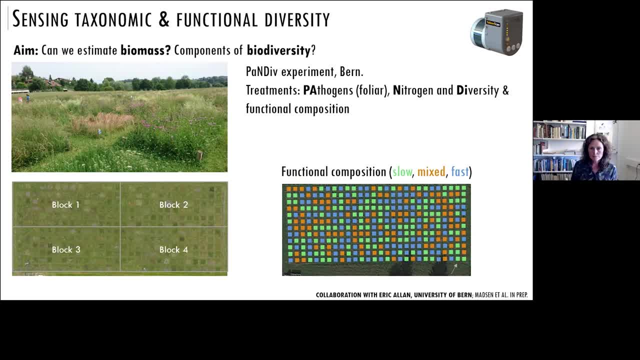 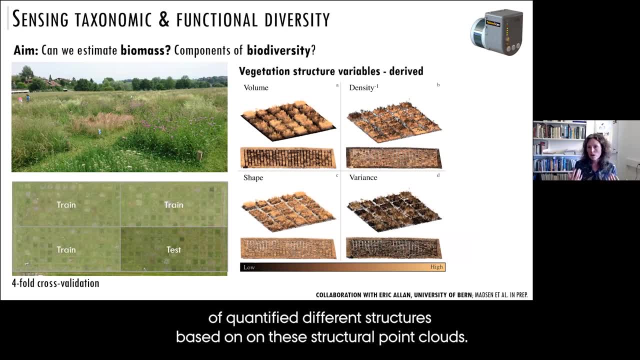 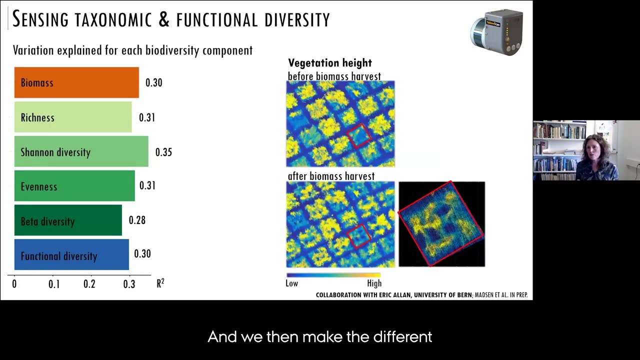 can tell us something about the ecosystem functioning. We have flown over this experiment several times, have quantified different structures based on these structural point clouds, And we then make the different measurements With machine learning methods. we can then quantify biomass and the richness and other. 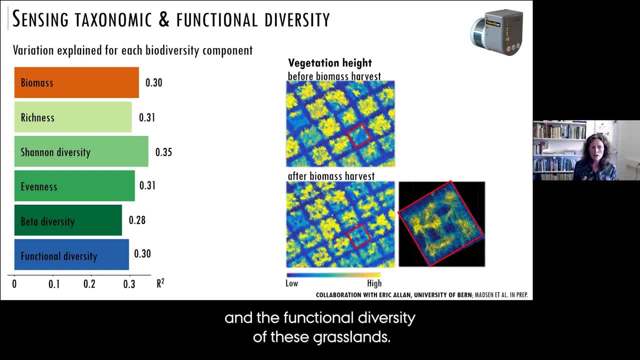 in here in green other estimates of biodiversity and the functional diversity of these grasslands, And what you see here is basically that explanatory power ranges from about 0.3 to 0.5.. So for many of you this is very low explanatory power, But actually in ecology and in biology, 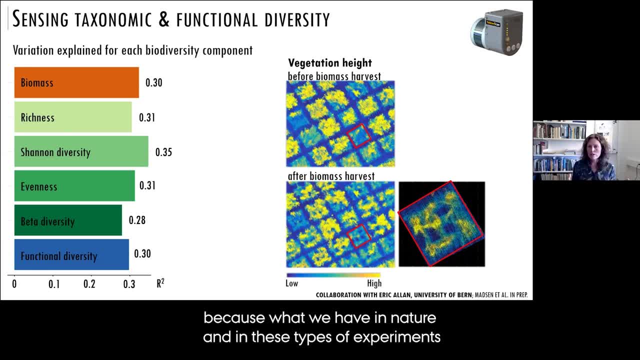 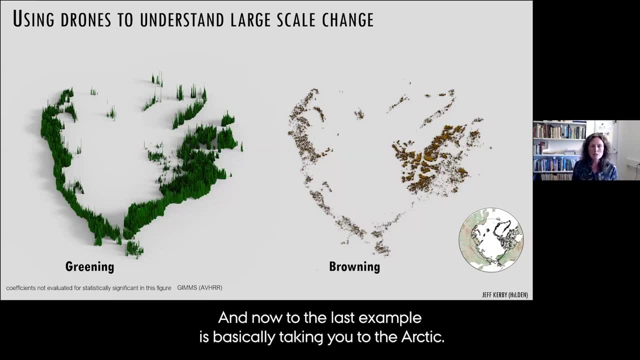 this is rather good because what we have in nature and in these types of experiments- there's a huge amount of variation that is really difficult to capture And we manage reasonable here, But there's still work to do to improve this further. And now to the last example- is basically taking you to the Arctic. The Arctic is changing. 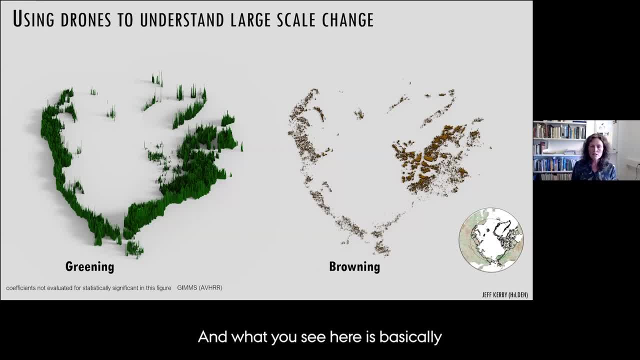 rapidly, as you all know, And what you see here is basically at the top. here it's Greenland, just to orientate yourself. And then the greening of the Arctic is an increased response and change in the NDVI over the last few decades. 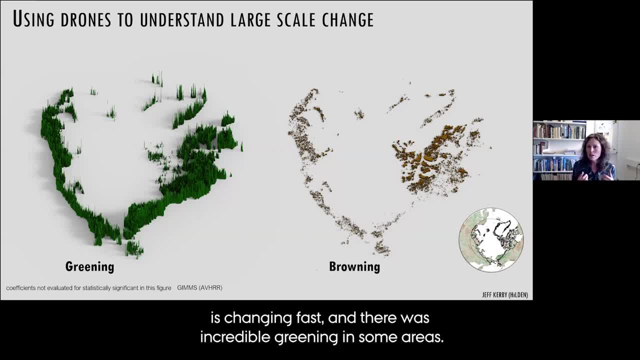 But on the one hand, the Arctic is changing fast and is incredibly greening in some areas. We also have a browning and decrease in vegetation productivity in other areas, And we want to try to understand what is causing these differences so that we can better understand the future. 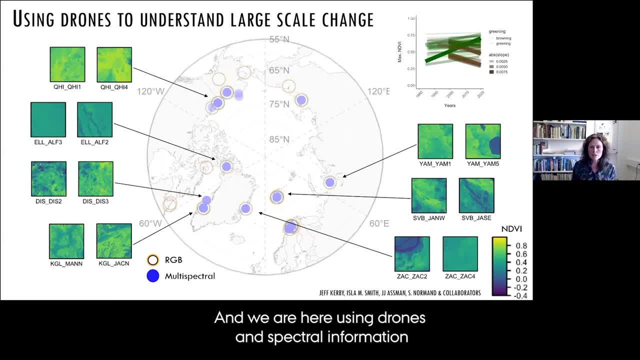 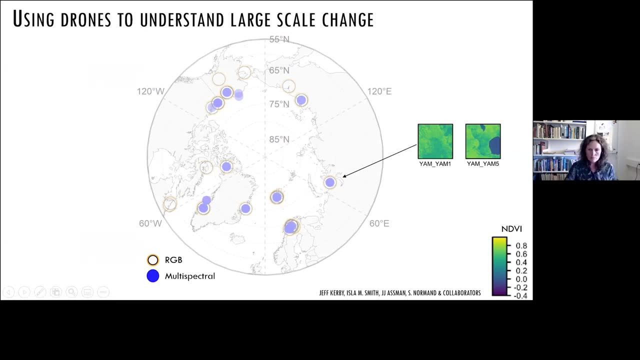 And we are here using drones and spectral information captured with multispectral sensors across the Arctic to try to understand the underlying causes of these dynamics. So here, what you see is just areas across the Arctic where we have this type of data from, And now we just zoom into one of these areas, from Yamal. 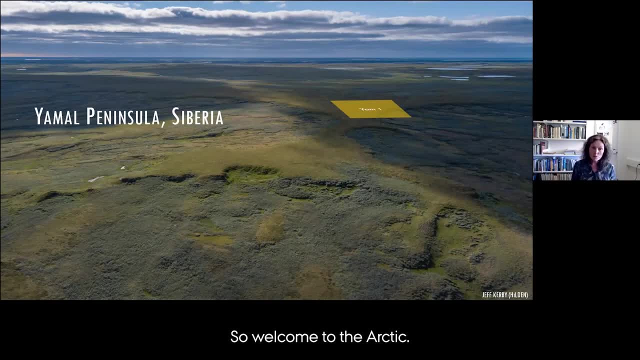 And in Yamal the landscape looks like that. So welcome to the Arctic. It's a very raced and really fascinating landscape. It's where we have these shrub-dominated patches, as you see in this gray-bluish color, And the very yellow-green is top of the plateaus. 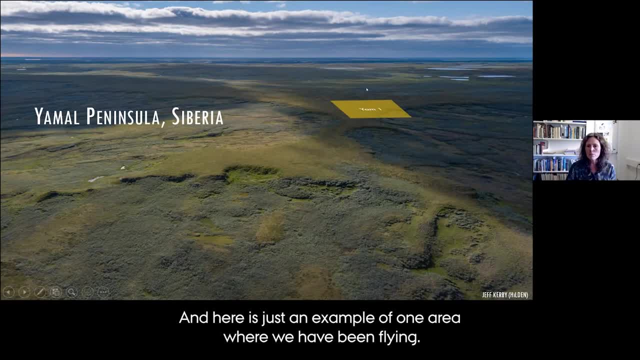 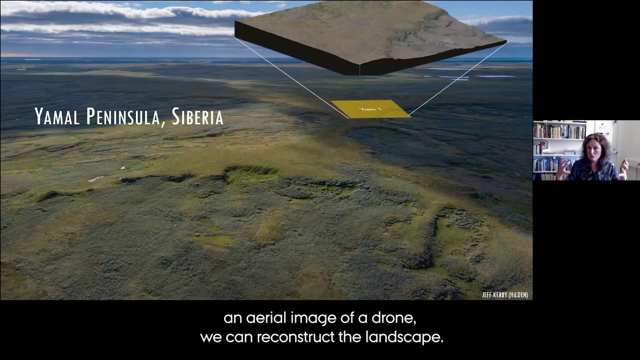 It's more dominated by grasslands And here's just an example of one area where we have been flying: Jeff Kirby, which is a postdoc in my group, have been flying the drones And from this area of such an aerial image of a drone, we can reconstruct the landscape. 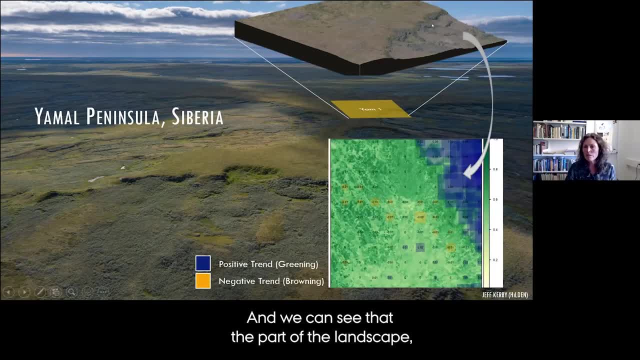 How does it look like? And we can see that the part of the landscape which is then actually greening is basically where we had rough dynamics and degradation of the landscape, And this is where we in blue here see the increase and the change in greening over the last decades. 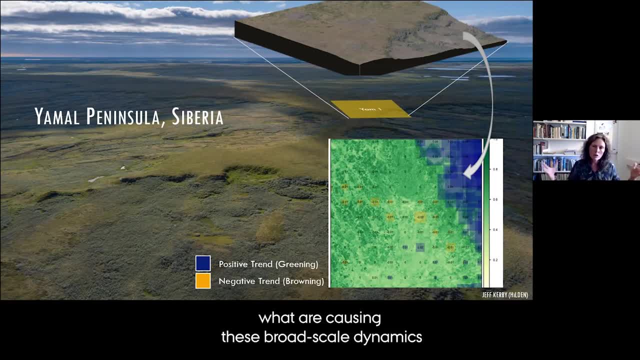 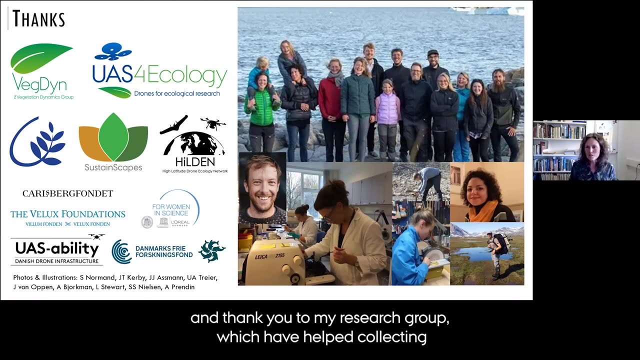 So here we are, using the drones to really try to understand what are causing these broad-scale dynamics at the very local site. So with that, actually just thank you for listening And thank you to my research groups which have helped collecting all these types of data across the Arctic and the European landscapes. 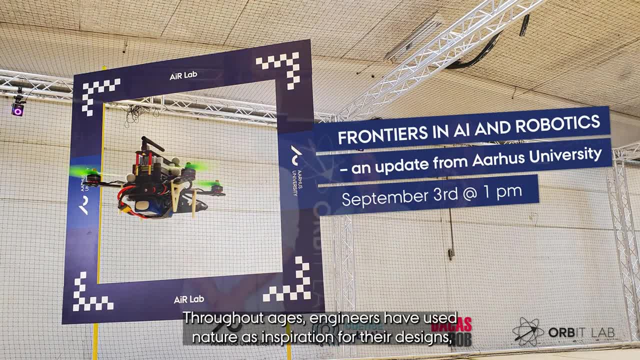 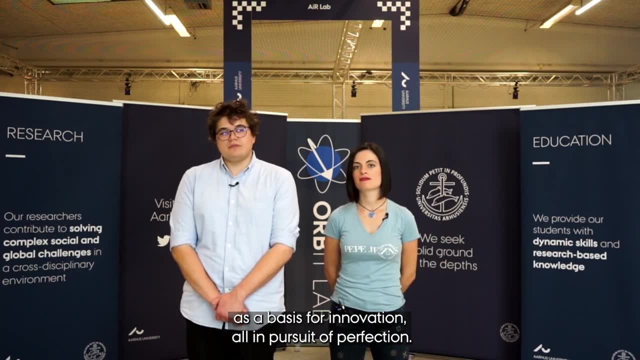 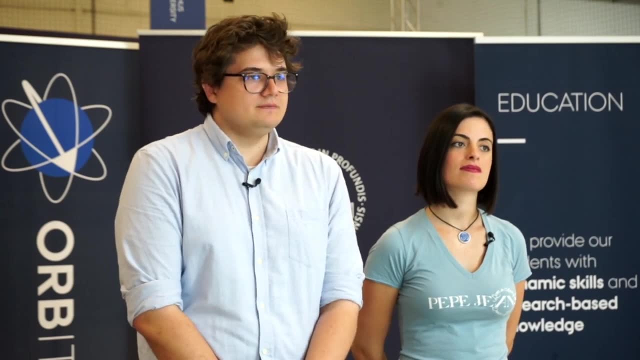 Thank you. Throughout ages, engineers have used nature as inspiration for their designs, as basis for innovation, all in pursuit of perfection. However, the gap between nature and our technology is small. It's still significant and we still need to reach very far. 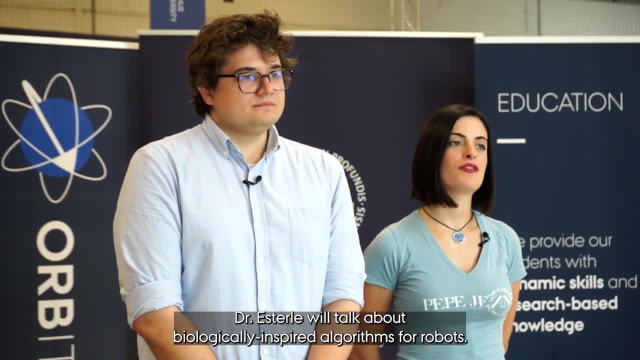 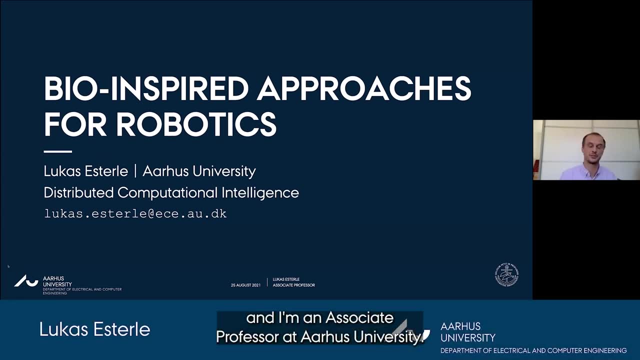 Dr Esterle will talk about biologically inspired algorithms for robots. My name is Lucas Esterle, I'm the head of the Distributed Computational Intelligence Group and I'm an associate professor at Aarhus University. Today I'm talking about bio-inspired approaches, and we actually heard a lot about different bio-inspired approaches already. 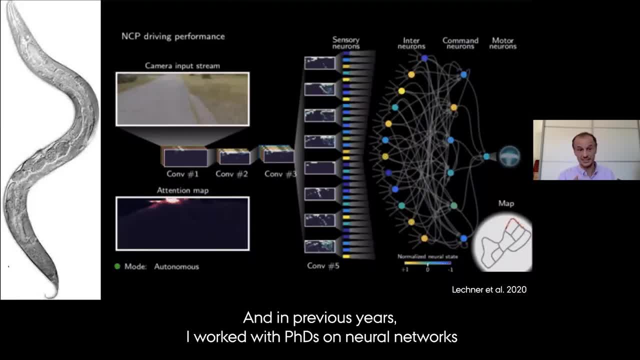 And specifically these are neural networks And in previous years I worked with PhDs on neural networks Inspired by a very small nematode called C elegans, And this nematode is very interesting because it only has 302 neurons and we can actually replicate those networks to achieve certain behavior. 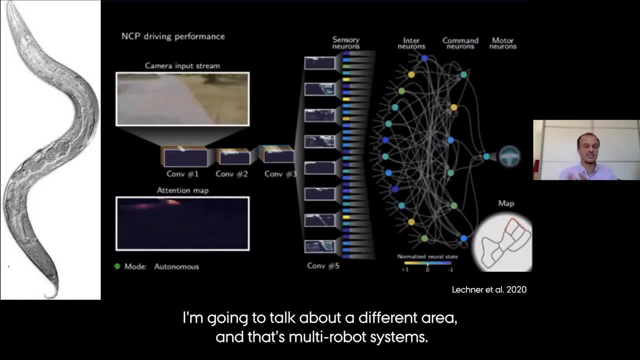 But I'm not going to talk about networks. I'm going to talk about a bit different area, and that's multi-robot systems. The reason for this are images like that. So this is a recent image from earlier this year where a young woman was. 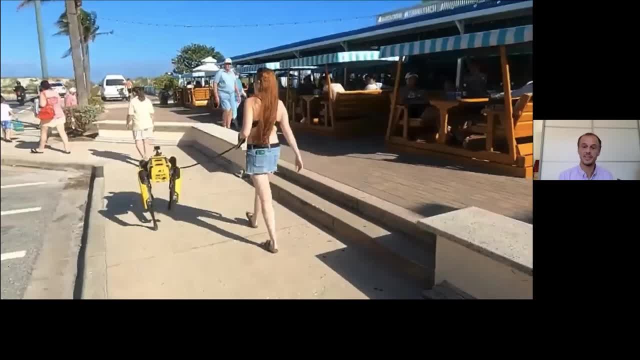 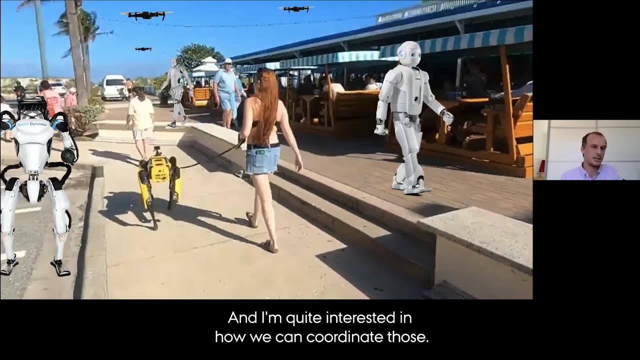 Walking her robotic dog in Florida, And I believe that this is becoming a new normal, so to say, and more a few that we're going to get used to, And I believe that there will be more and more robots in our environment and I'm quite interested in how we can coordinate those. 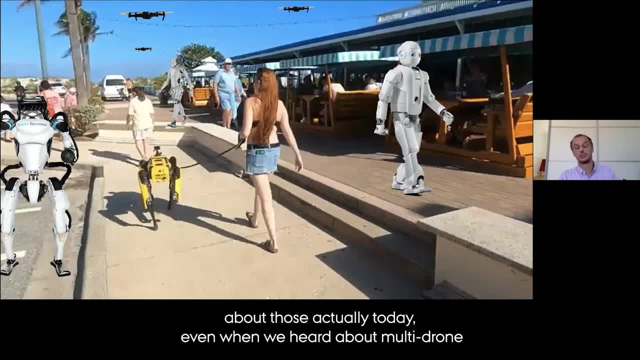 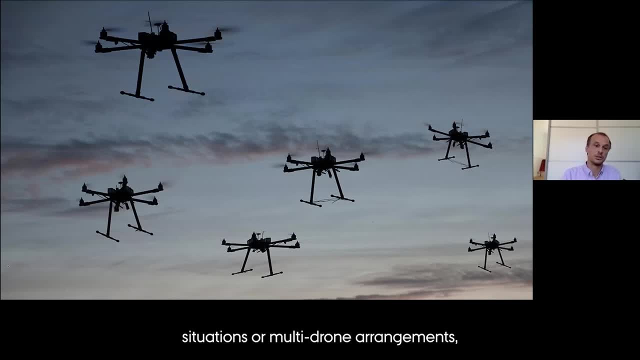 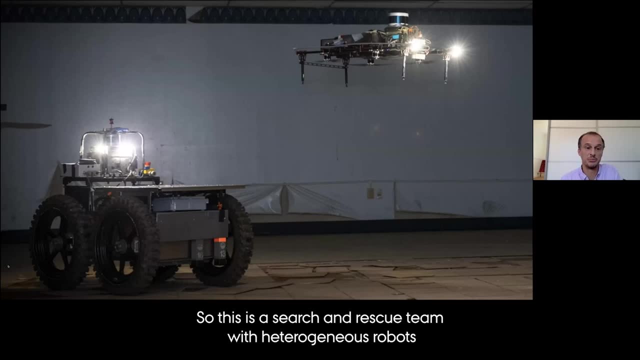 We've seen such interactions already and we've heard about those actually today, even when we heard about multi-drone Situations or multi-drone arrangements, but also when we heard about search and rescue. So this is a search and rescue team with heterogeneous robots. 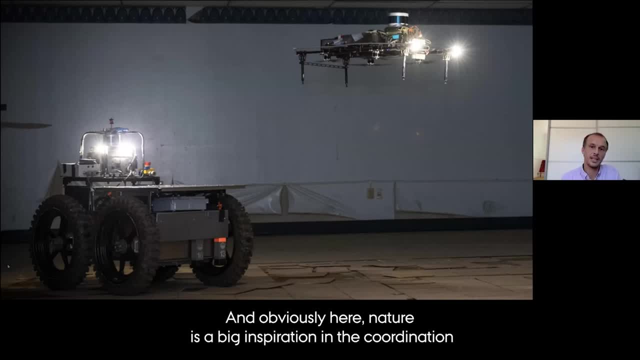 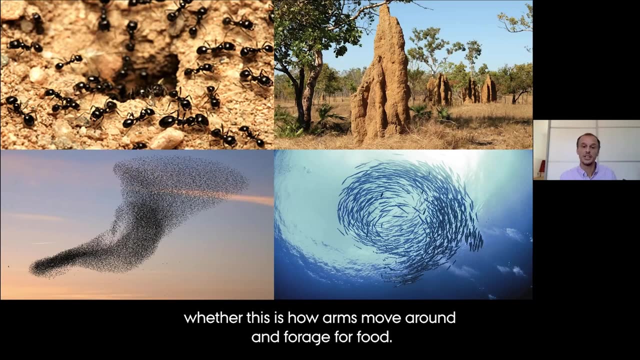 We have a ground robot and a flying robot, And obviously here nature is a big inspiration in the coordination of such things, because we can see this in nature quite often, Whether this is how ants move around and forage for food or termites build up their 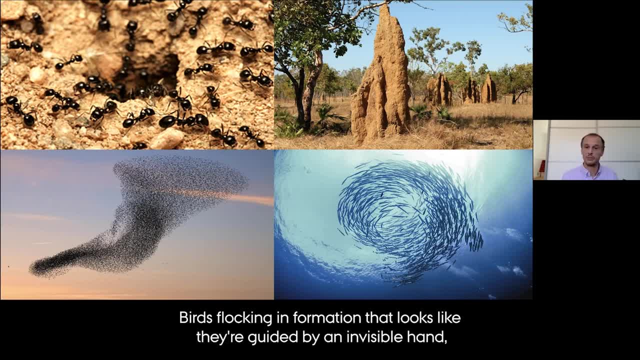 Termite hills, birds flocking in formation that looks like they are guided by an invisible hand, or schools of fish that are trying to perturb a predator. We use this as inspiration to work on coordination of tasks, as well as coordination of movement of different robots and agents. 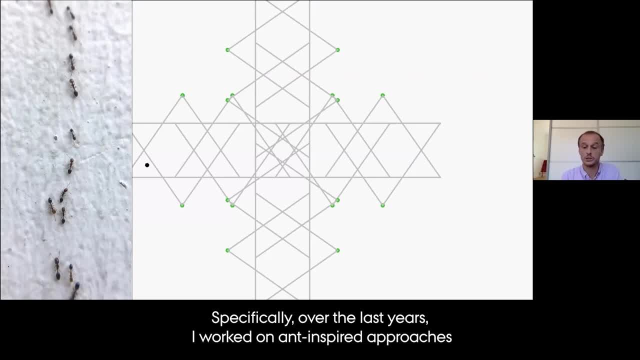 Specifically over the last years I worked on ant-inspired approaches with the idea. see that this starts With the idea that we learn neighborhood relationships among robots. Here our robots are not moving, but they are serving moving objects. the black dot. 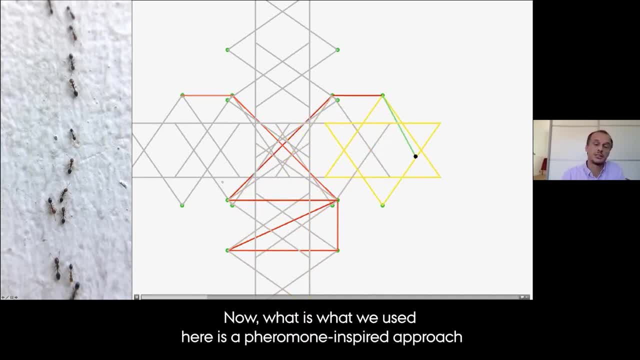 And the red line indicates their learning behavior. Now, what we used here is a pheromone-inspired approach, inspired by ants, and we learn relations as pheromones do, And we can actually unlearn this. so pheromones, our artificial pheromones, evaporate over time. 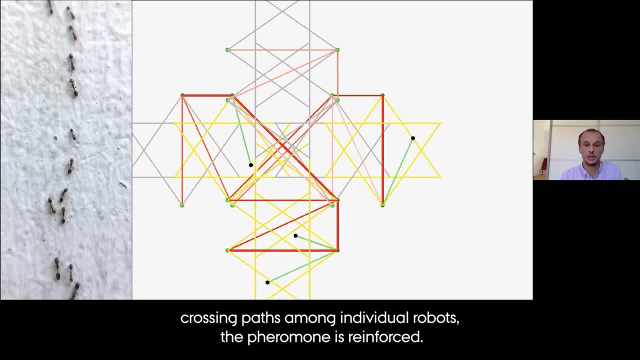 If we see more objects crossing paths among individual robots, the pheromone is reinforced. Now this can be used to greatly reduce communication efforts or assign tasks within a multi-robot setting. Another area we worked on is formation flights, So here we were inspired by the formation of geese. 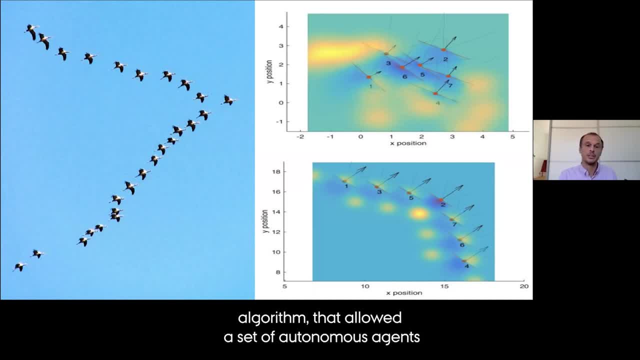 Basically what we did here is: we developed a planning algorithm that allowed a set of autonomous agents that started off in an unstructured way to find their position and create a view. with its fellow well flying drones, for example, We showed that this is quite, not only quite efficient in terms of planning, but also reduces the energy efforts in flying information. 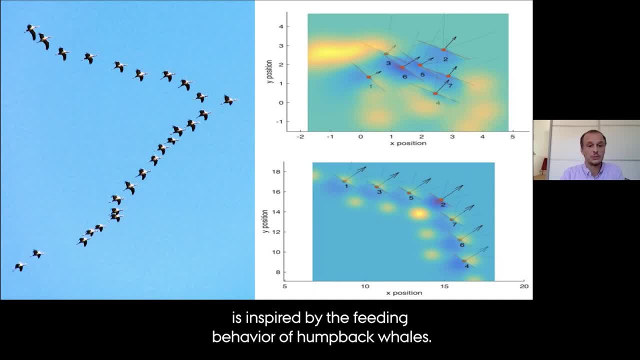 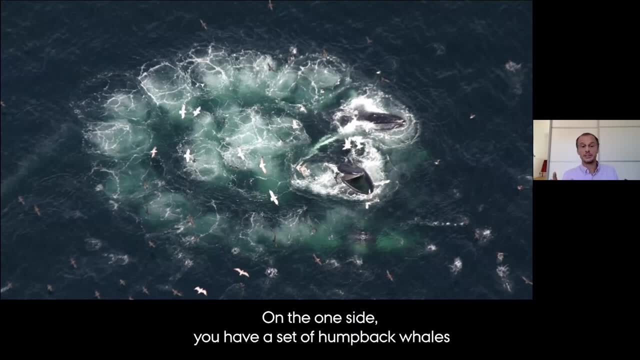 Now the last bit, that is, my most recent work is inspired by the feeding behavior of humpback whales. Now, what they do is they form different teams. On the one side, you have a set of humpback whales that swim underneath a fish or grill and blow up bubbles. 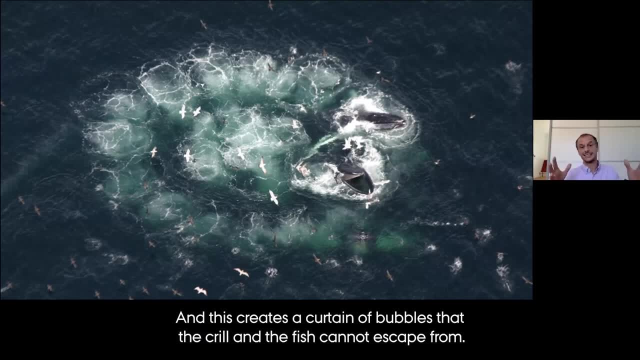 And this creates a curtain of bubbles that the grill and the fish cannot escape from. Now the second team comes in swooping from underneath and starts feeding on the grill, And that is something that looks pretty much what we have here on the left. 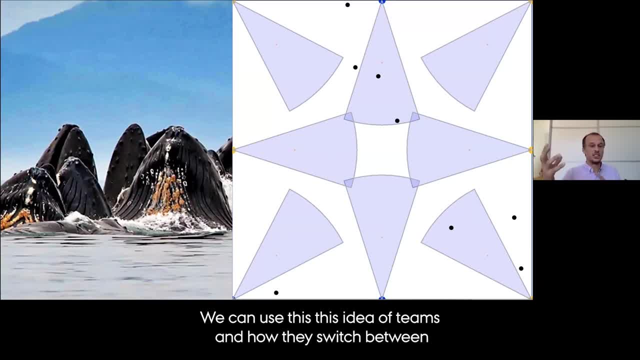 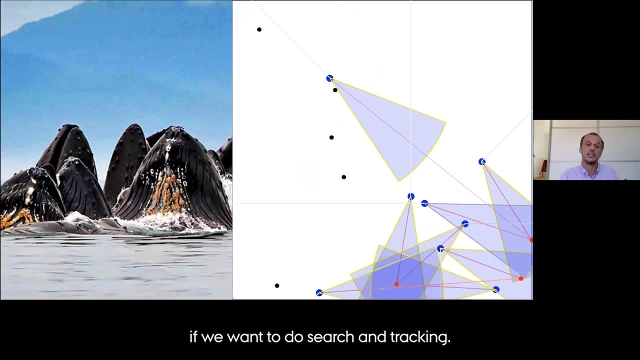 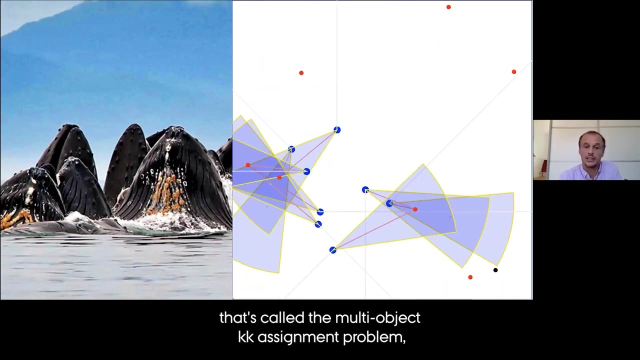 And we can use this idea of teams and how they switch between their actual team as an inspiration for our work, And we showed that such a switch- dynamic switch during operation- actually is quite helpful if we want to do search and tracking. So here, in this specific case, we have a problem that's called the multi-object K-assignment problem. 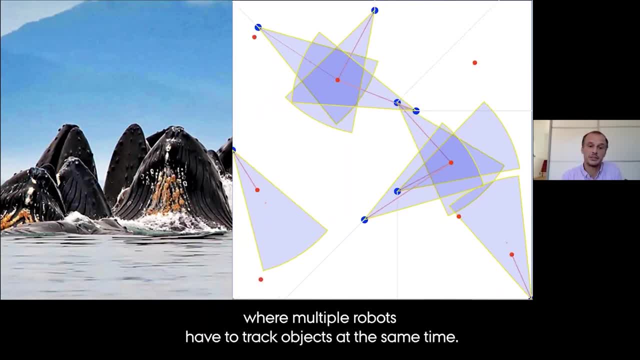 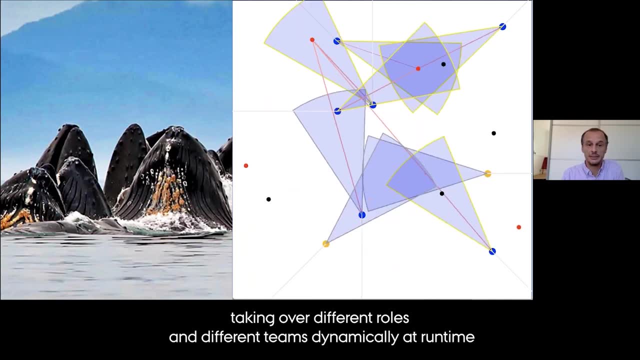 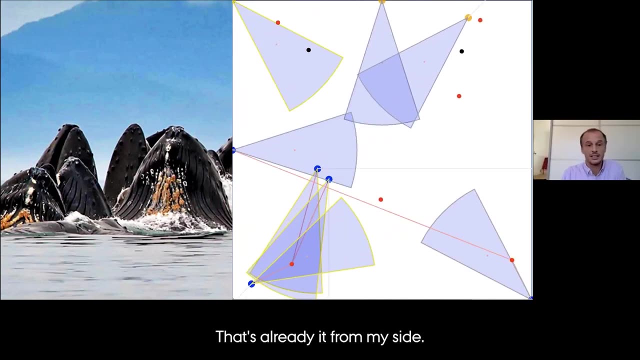 where multiple robots have to track objects at the same time, And we showed that having the robots taking over different roles and different teams dynamically at runtime has a huge impact on the performance of the entire team. That's already it from my side. That was my five minutes. 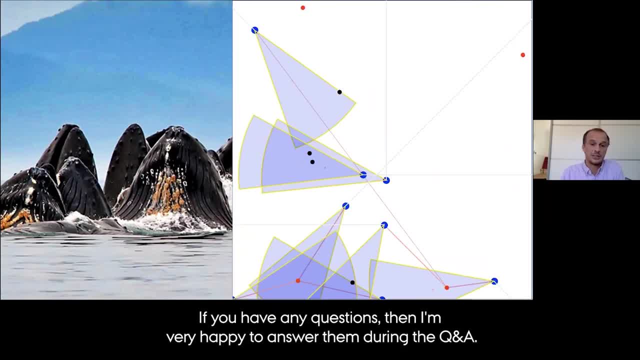 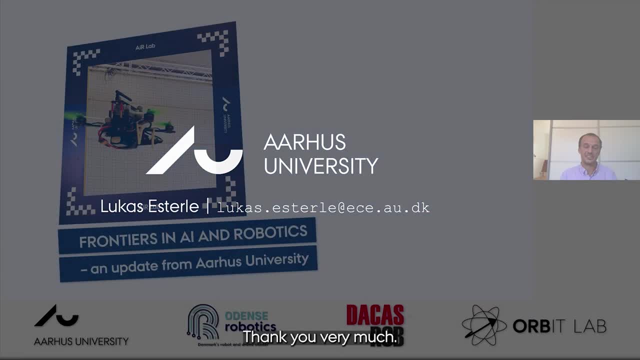 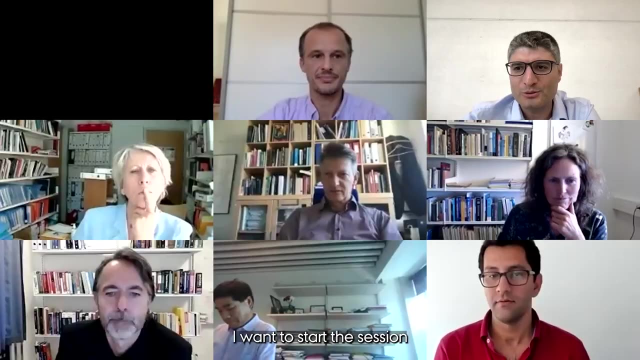 If you have any questions, then I'm very happy to answer them during the Q&A. You're also very welcome to send me an email if you have a question later on. Thank you very much. I want to start The session with a question for you. 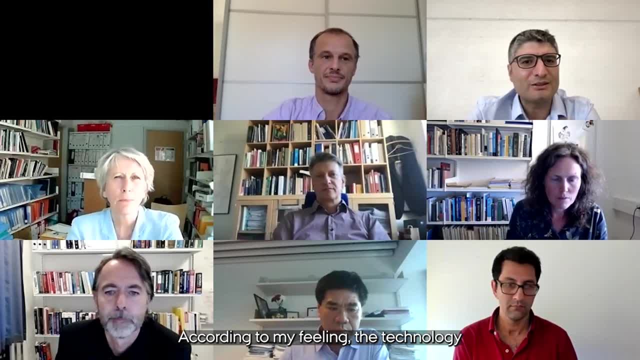 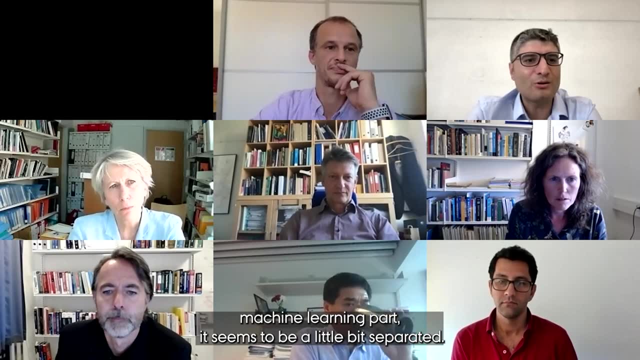 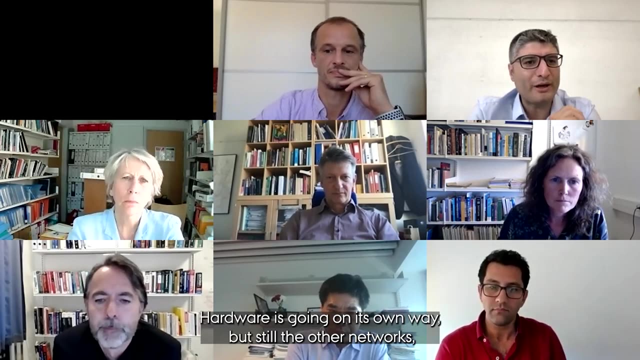 According to my feeling, the technology on the neuromorphic computing and the machine learning part. it seems to be a little bit separated. Hardware is going on its own way, but still the other networks, like deep neural networks, convolutional neural networks, 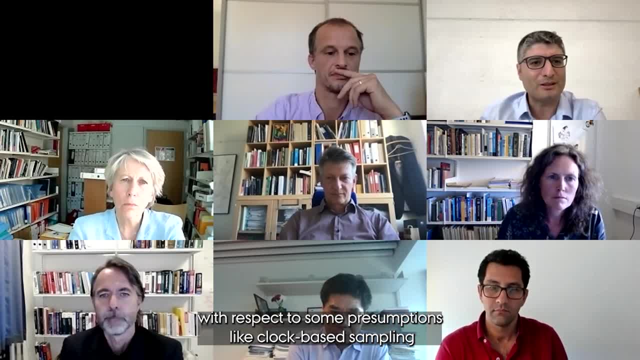 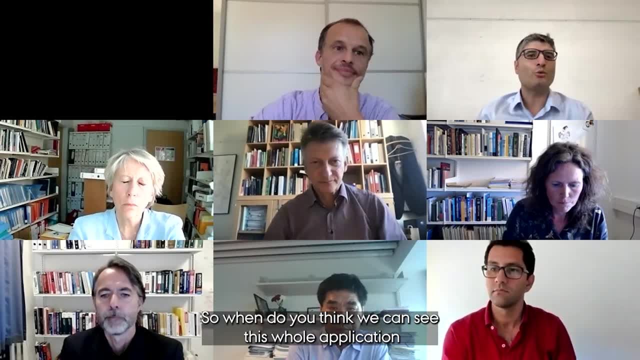 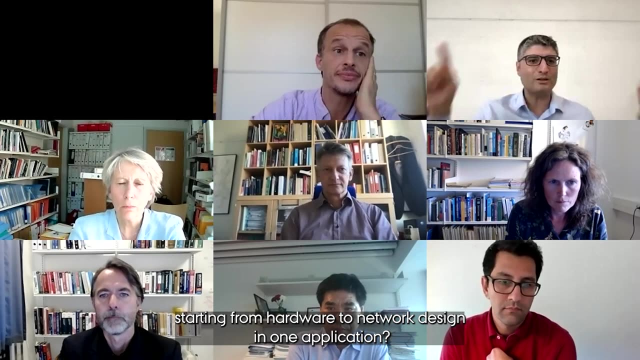 they are still done With respect to some pre-assumptions like clock-based sampling, and then event-based cameras are coming into the picture. So when do you think we can see this whole application, starting from hardware till network design, in one application? Is it going to happen in a few years time, five to ten years of time, or what? 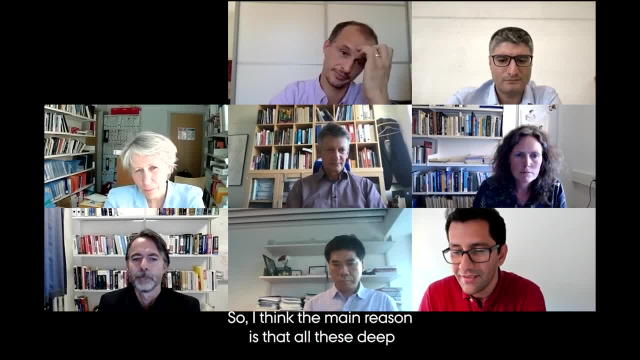 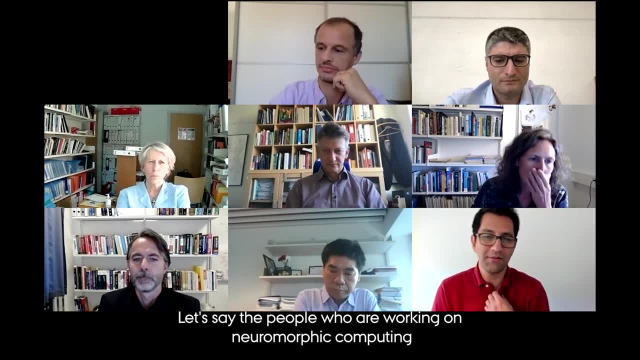 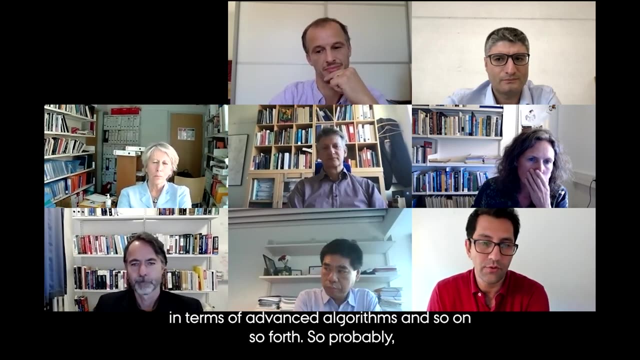 Yeah, thanks for the question. So I think the main reason is that all these deep learning algorithms and so on, they're way ahead of us, Let's say, the people who are working on neuromorphic computing in terms of advanced algorithm, and so on and so forth. 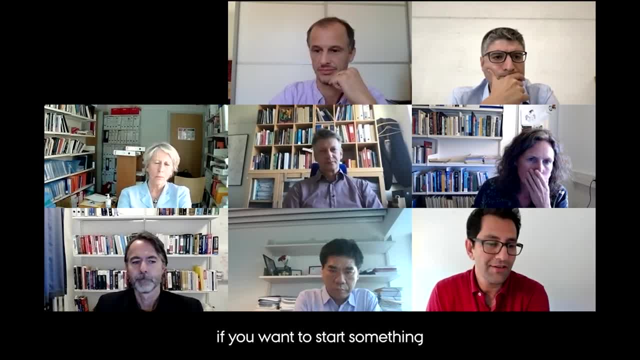 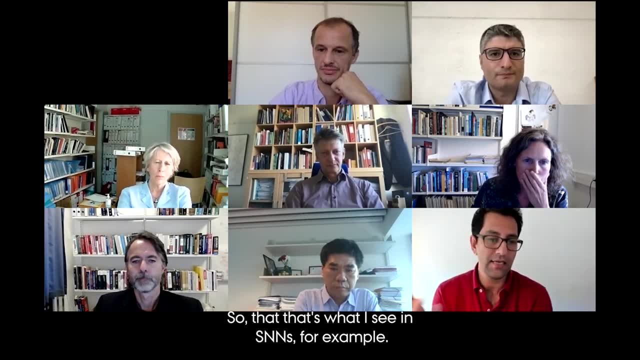 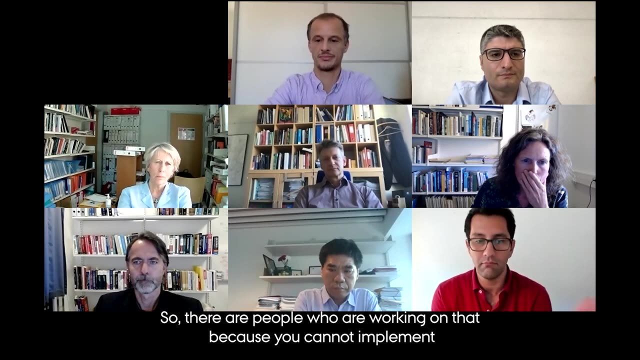 So probably, if you want something, if you want to start something from scratch, so probably it should go hand in hand. So that's what I see in SNNs, for example. So the algorithms are still not mature. So there are people are working on that because you cannot implement many of them. 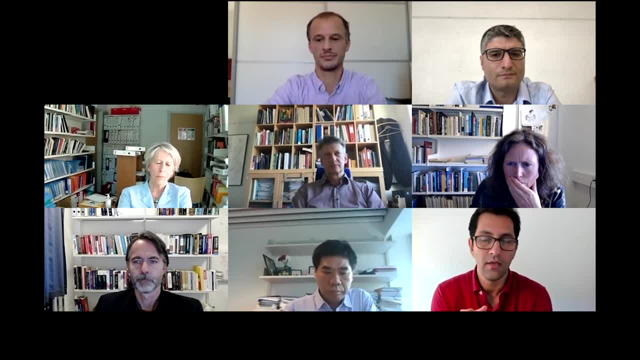 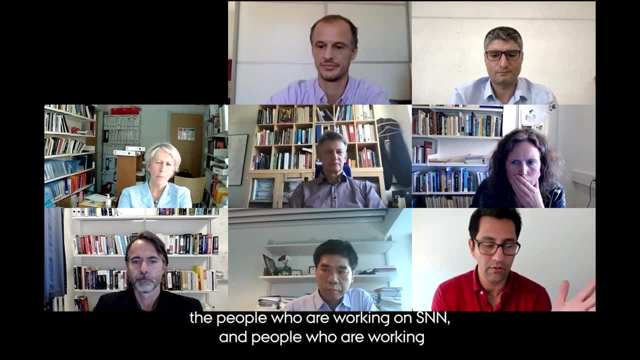 Kind of learning the algorithm on this SNNs. So that's why people are talking to each other a lot within the community, The people who are working on SNN, people who are working with from the soft side, from the hard side. 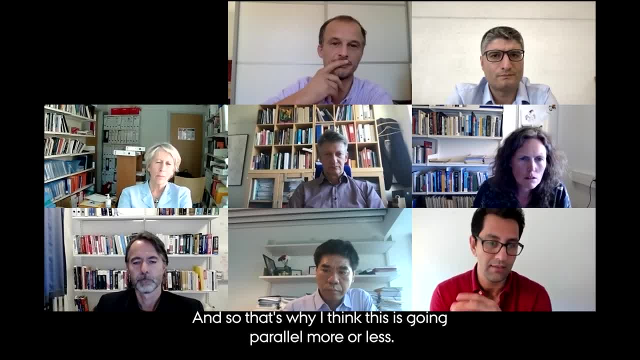 So they are talking to each other, And so that's why I think this is going parallel more or less. But when you look at the deep learning, I mean OK, the GPUs have been there, and so on and so forth, for a long time. 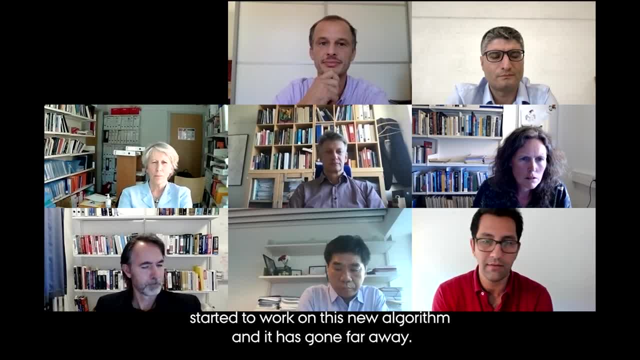 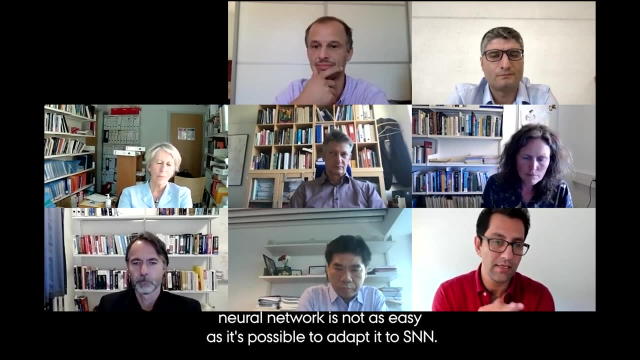 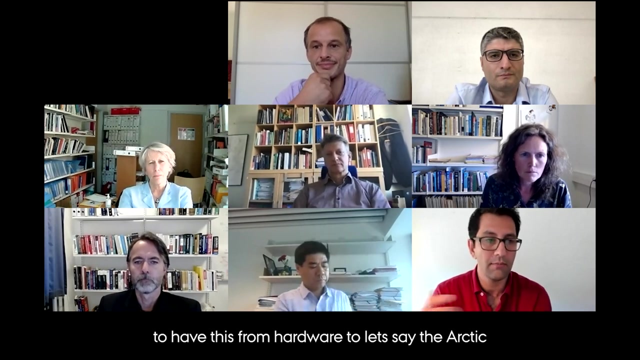 And then people have started to work on this new algorithm And it has Gone far away. So that's why probably adapting new hardware to this deep neural network is not as easy as it's possible to adapt it to SNN. So, but then I believe SNN will find a way, its footprint, to have this from hardware to, let's say, architecture and soft advanced algorithms. 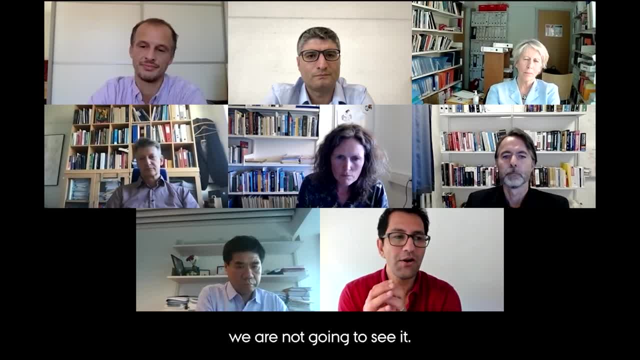 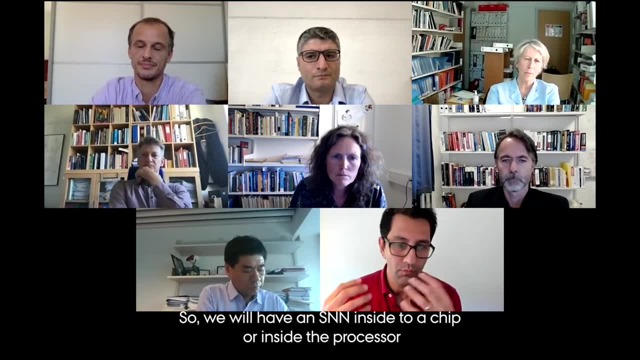 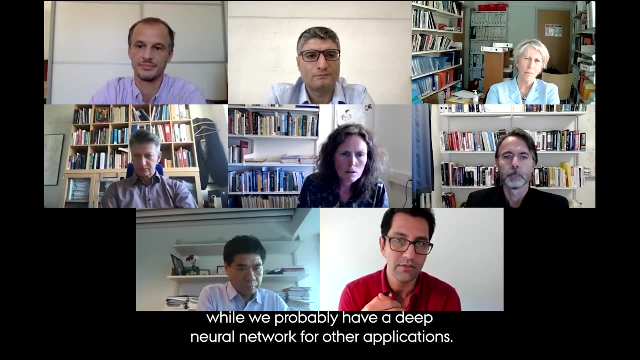 But for deep learning, I believe we are not going to Proceed, and probably it will be a combined approach at the end, of using this and this together. So we will have an SNN inside a chip or inside the processor, while we probably have a deep neural network for other applications. 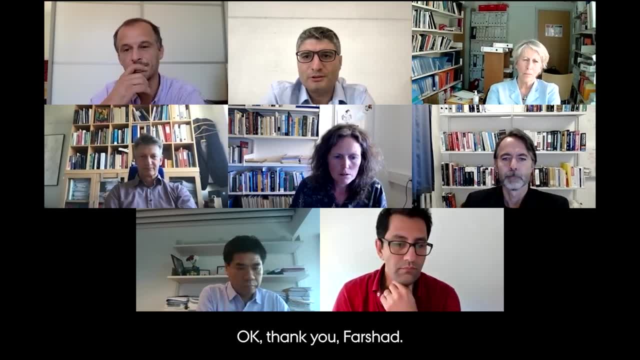 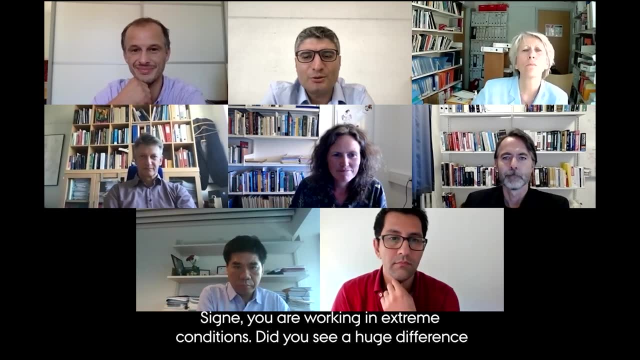 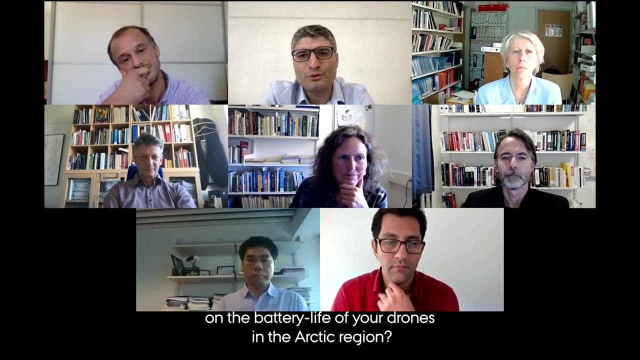 OK, thank you, Farshad. Since there is no question from the audience, I have one question for Sine. Sine, you are working in extreme Conditions. Did you see a huge difference on the battery life of your drones in Arctic? 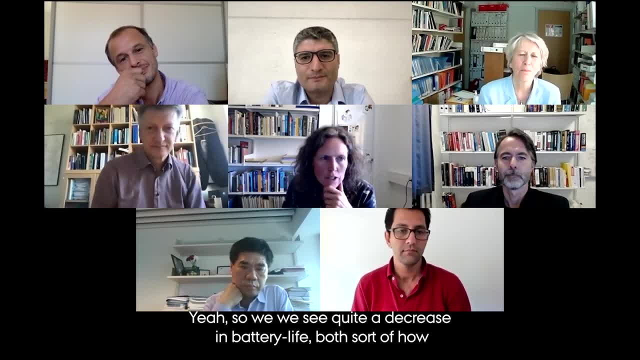 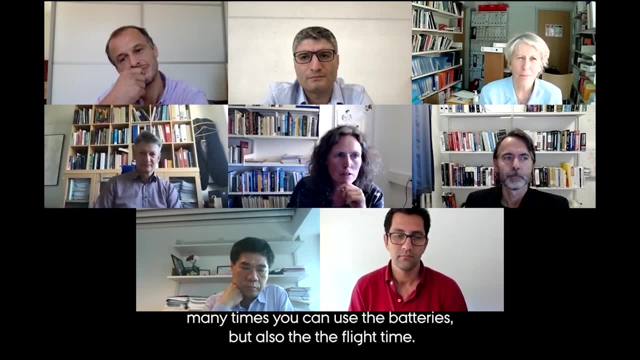 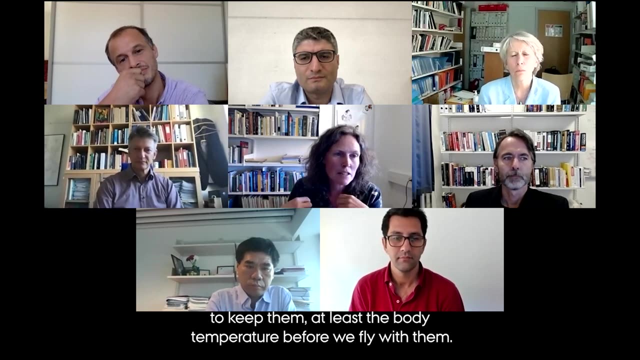 Region. Yeah, so we see quite a decrease in battery life, both sort of how how many times we can use the batteries, but also the flight time. It helps, helps a lot, because we put them on the body to keep them at least at body temperature before we fly to them. 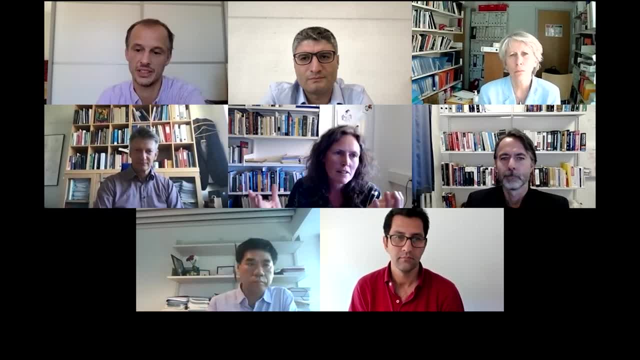 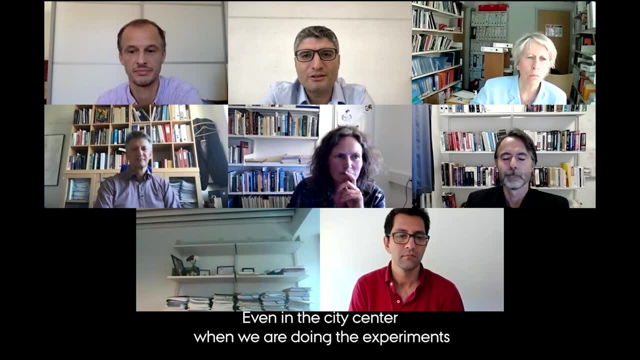 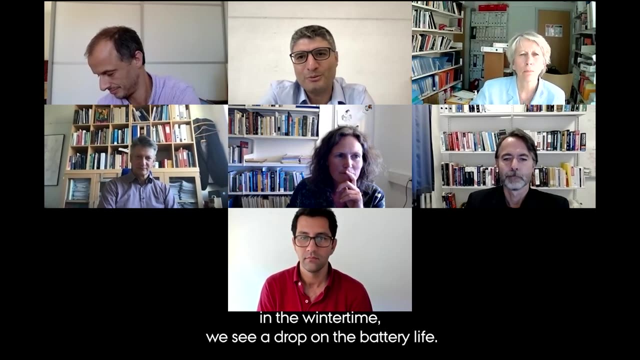 That gives us two to three minutes. It's additional, But but yeah, we have less flight time in overall. Yes, that's a bit unfortunate. even in the city center When we are doing the experiments in the wintertime, we see a drop on the battery life. 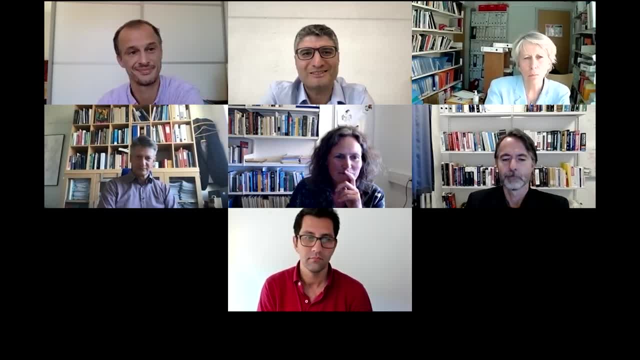 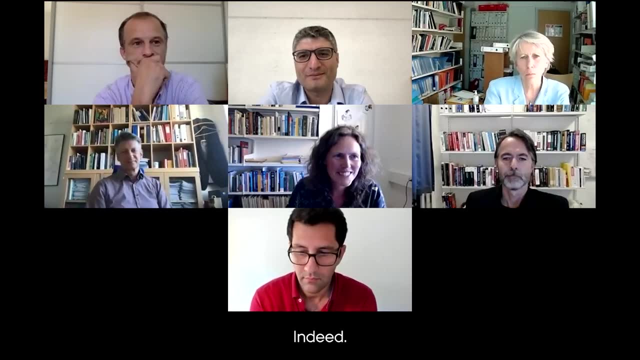 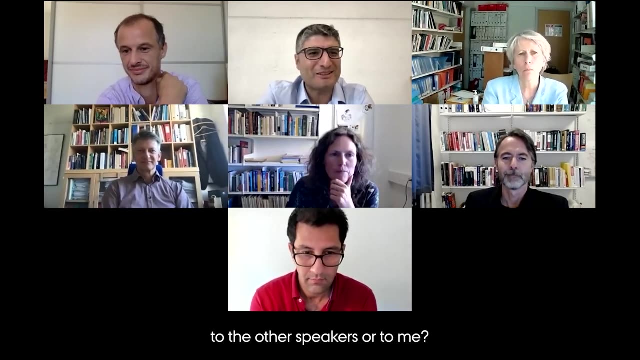 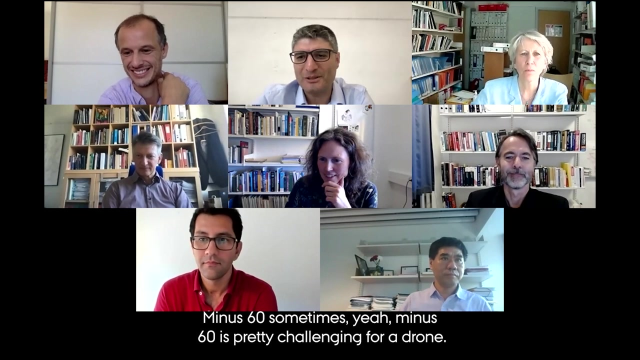 So I can't imagine how it goes when you have minus degrees in the in the Arctic area. So I can imagine it's pretty challenging, Indeed, OK, is there any question from my speakers to to other speakers or to me? Minus 60 sometime. 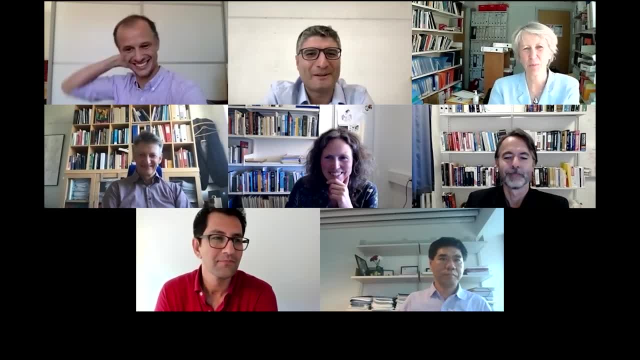 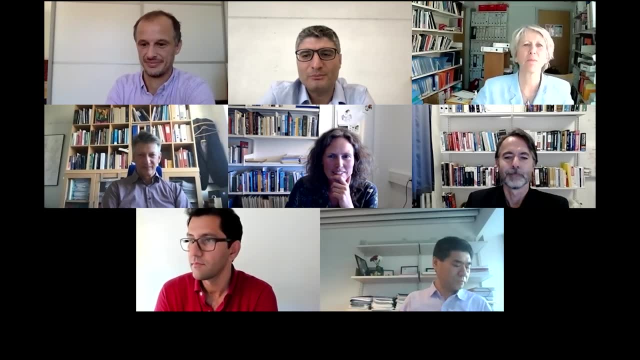 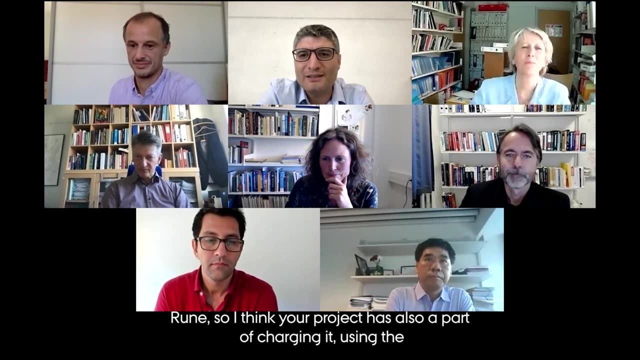 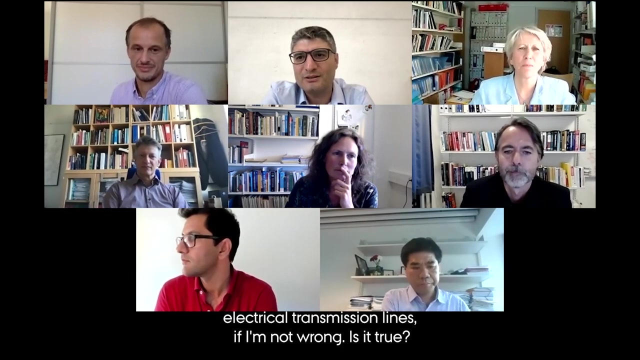 Yeah, minus six is pretty challenging for a drone. OK, my, I have maybe one last question for Rune Rune. So I think your project has also a part of charging it using the electrical transmission lines, if I'm not wrong. Is it true? 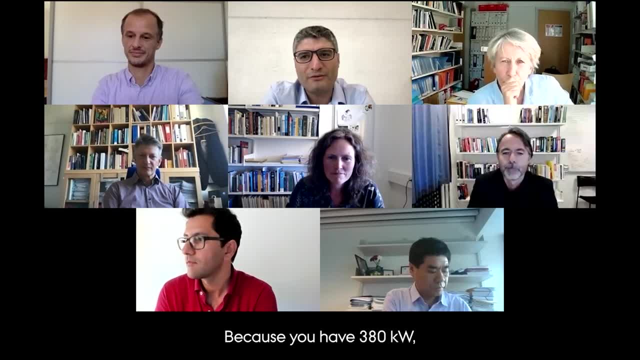 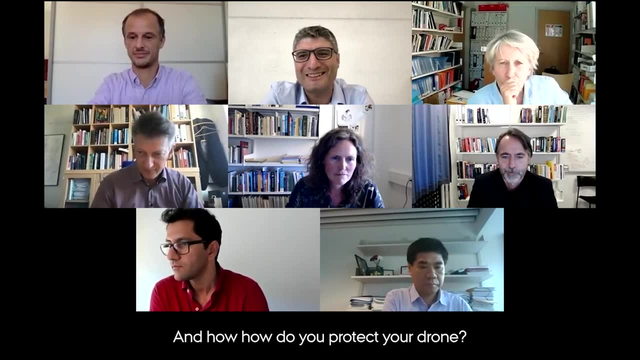 True, Yes, So how is it possible? Because you have three hundred and eighty kilowatts or kilowatts on your lines, and how do you protect your drone? Yes, So obviously, when you have such high voltage, when the drone approaches you, it's not so important. 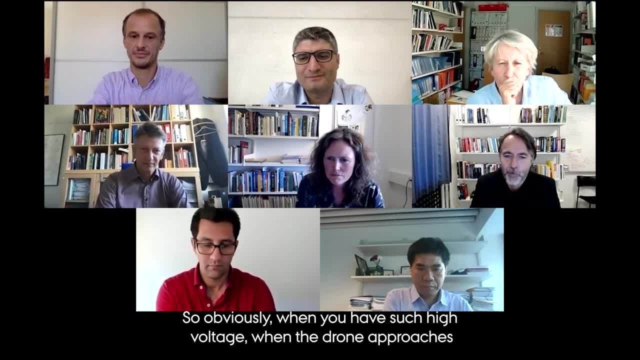 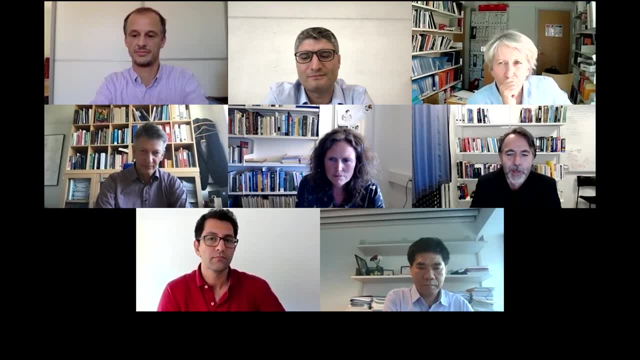 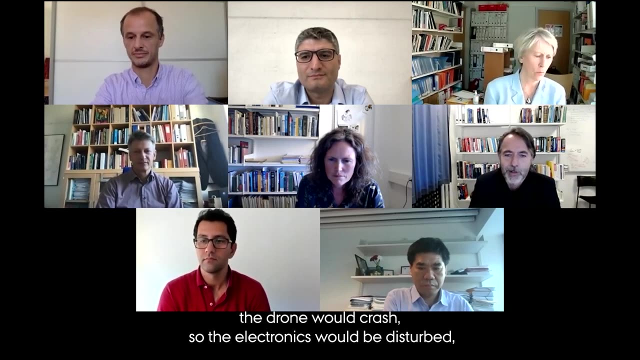 It's not so important. It's not so important for you. it's not so important for you. drone approaches the power line. there will be a spark going from the power line to the drone and in the first, first attempts to try this, the drone would crash. so the electronics would be. 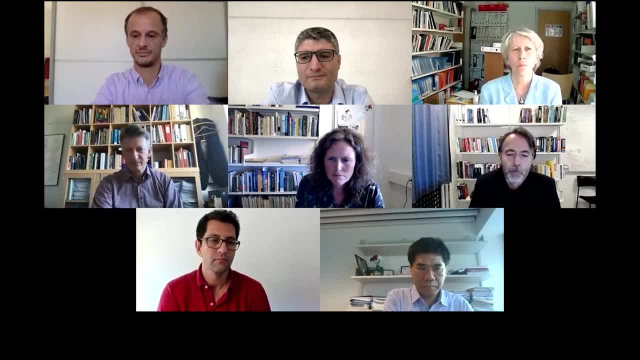 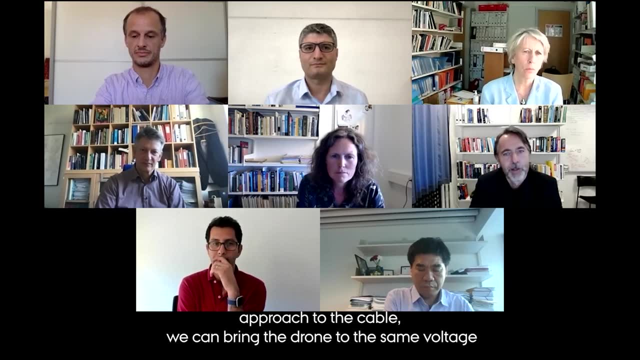 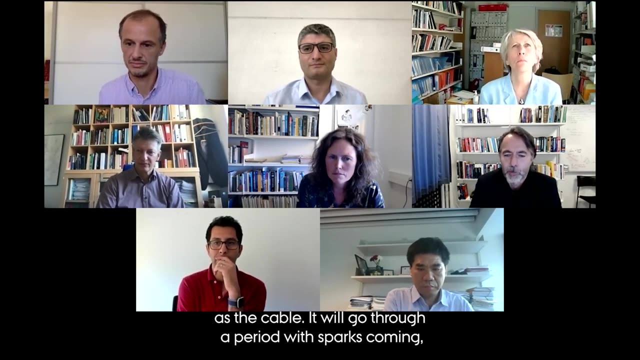 disturbed, the communication would break and it would be crash. but what is possible is to shield the electronics and then, with the soft say approach to the cable, we can bring the drone to the same voltage as the cable. it will go through a period with sparks coming, but with protecting. 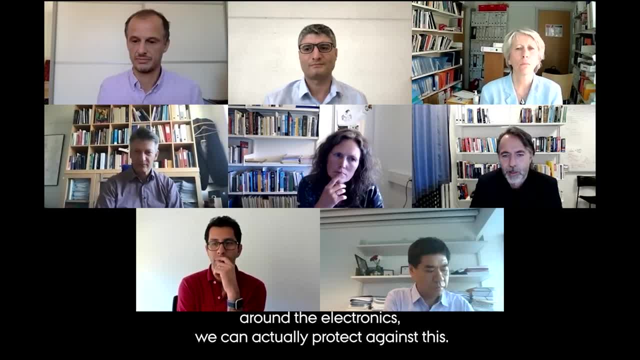 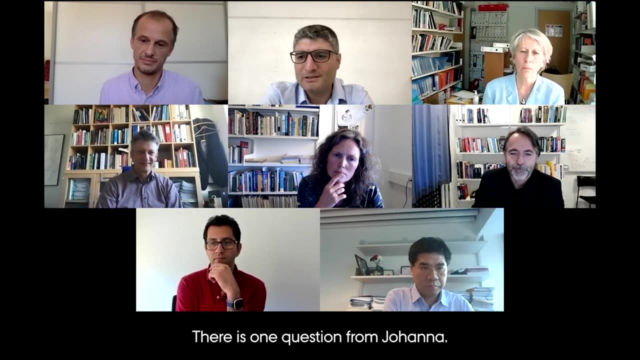 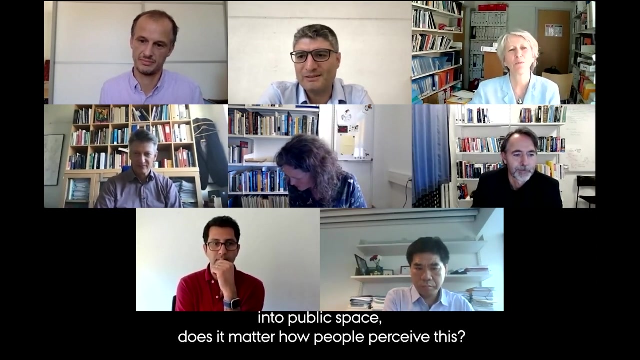 making, say, metallic cages around the electronics, we can actually protect against this. so it is possible, but of course, some engineering needs to be done to to become successful. okay, thank you, Rune. there is one question from Johanna. for those of you who put the drones into public space, does it matter how people perceive this? I think this is this. 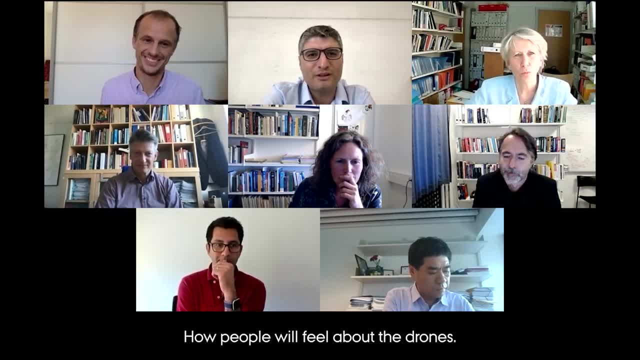 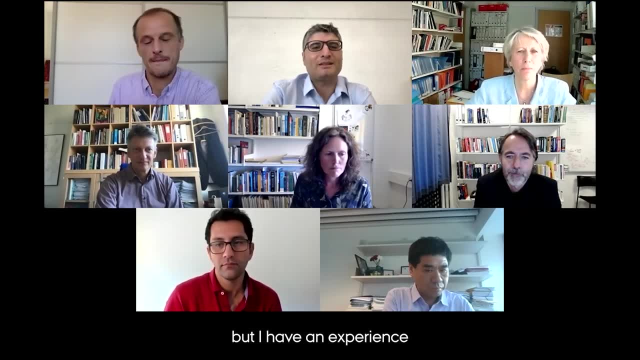 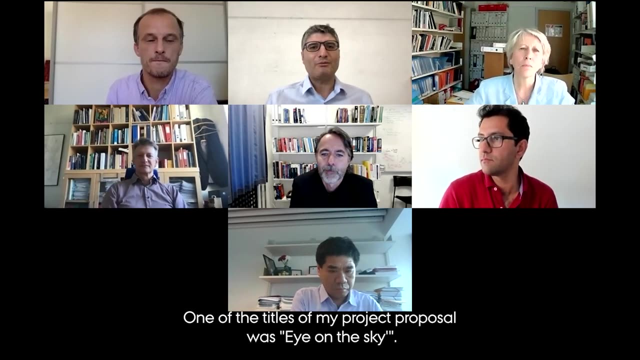 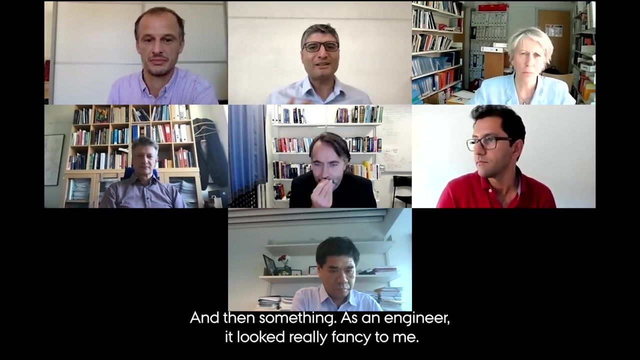 question is related to psychology, right, how people will feel about the drones. okay, um, it's not for the public space, but I have a an experience with social uh science people. one of the titles of my project proposal was eye on the sky and done something as an engineer. it looked really fancy to me. I really liked the title and, and one of my friends, 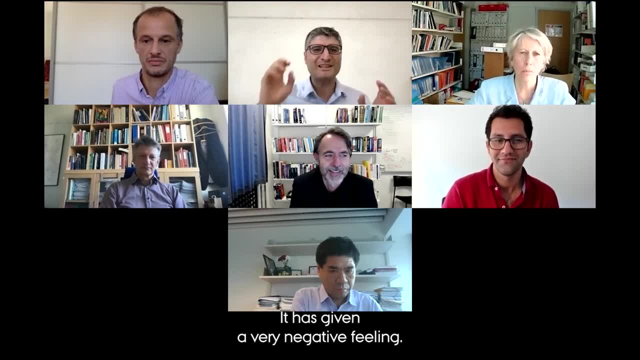 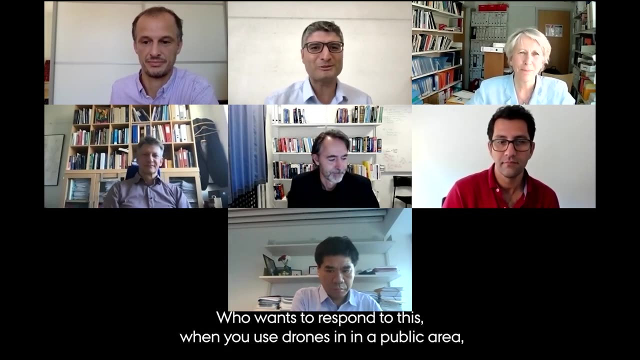 said: oh my God, it's horrible. what do you mean by eye on the sky? it's, it's. it has given a very negative feeling. so I think the drones: when I see the drones, it gives me very positive feeling, like because I'm doing research with them. but yes, your question is is interesting. who wants to respond to? 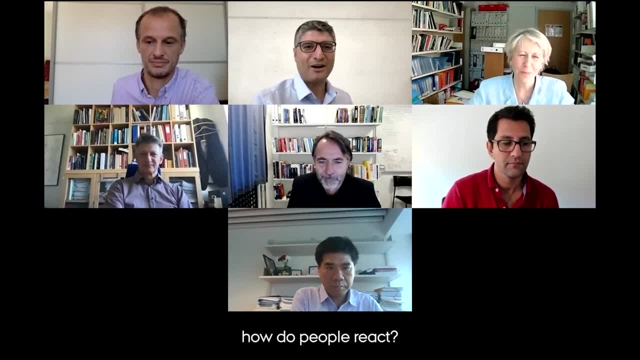 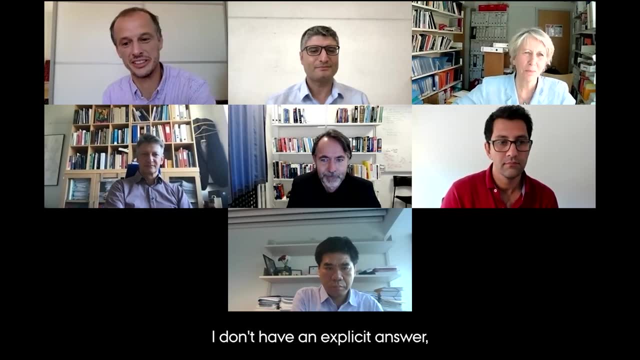 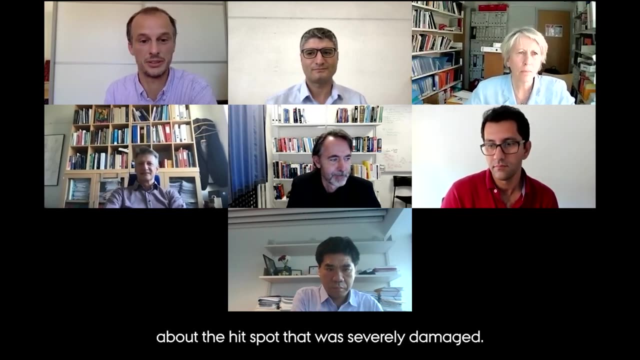 this: when you use drones in in public area, how people react. I don't. I don't have an explicit answer, but I'm going to start with with my thoughts. I mean, I've written it down, uh, Johanna herself gave a couple of interesting examples about the, the Hitchbot, that 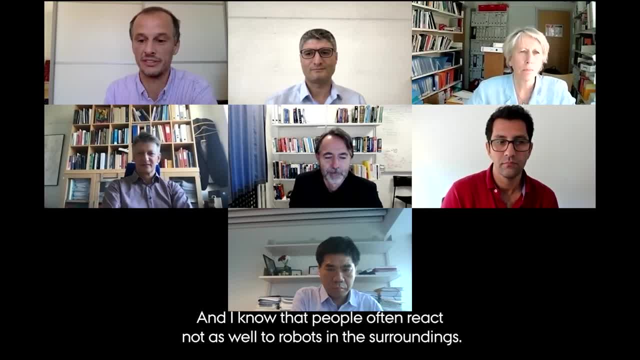 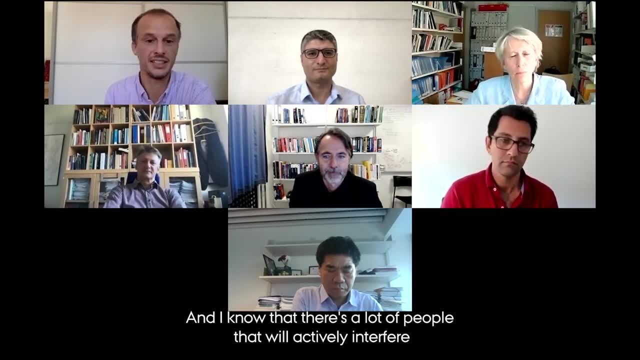 was severely damaged and and I know that people often react not as well to robots in the surroundings, and I know that there's a lot of people that will actively interfere with the robots in a way that will harm them or at least disturb their, their action patterns, and so I think it's important to 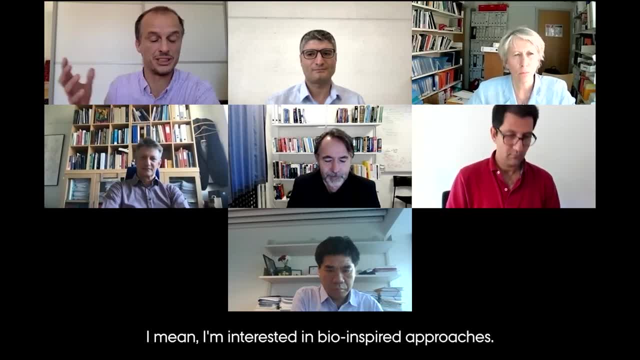 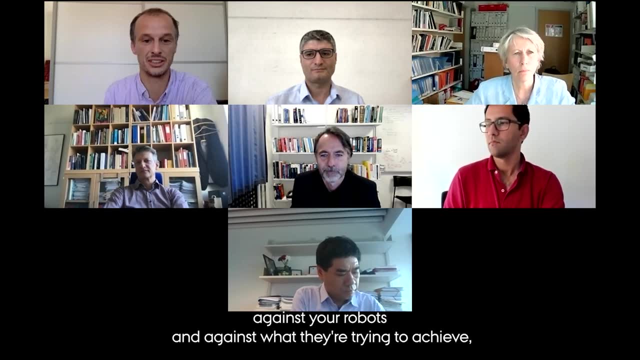 experience, and that's from bio-inspired I mean. I'm interested in bio-inspired approaches. I know this can be a real problem when people actively trying to work against your robots and against what they're trying to achieve, even though it does not interfere with them in any way. 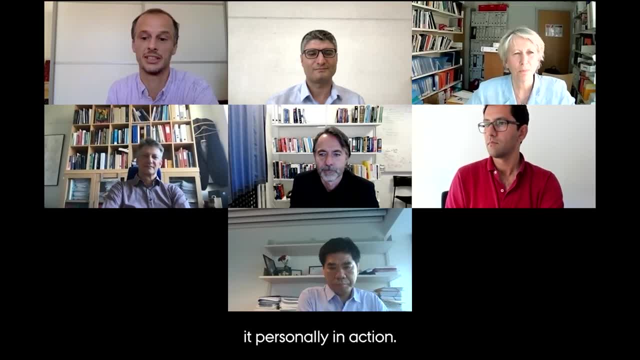 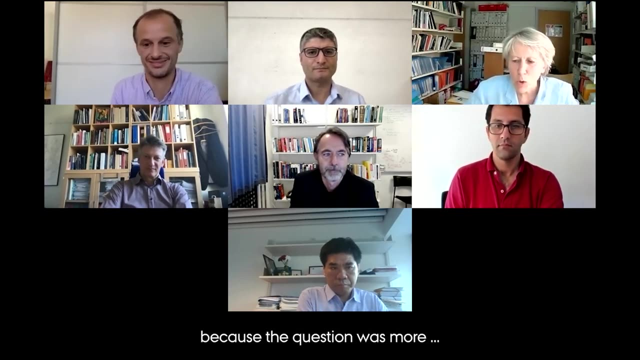 um, so yeah, I believe I haven't done it and I haven't seen it personally, uh, in action, um, but I do believe this is a this is a huge problem to us in the future until they are fully accepted. yes, Johanna, do you want to say something? add something, because the question was more. I mean. 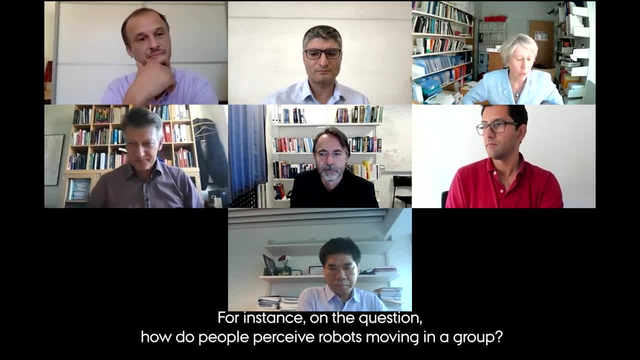 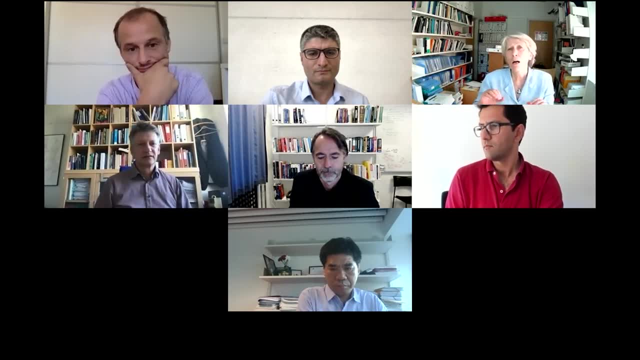 there's quite a bit of HRI research precisely on that. for instance, on the question: how do people perceive, uh, robots moving in in a group? um, different kinds of swarm movements, how they perceive the friendly cooperative, and so on. lots of research on it. so, um, and also, how do they perceive? 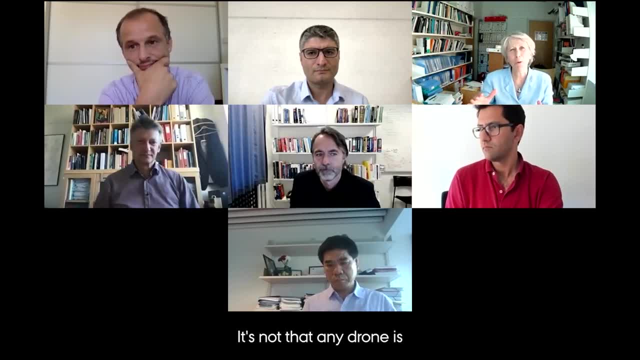 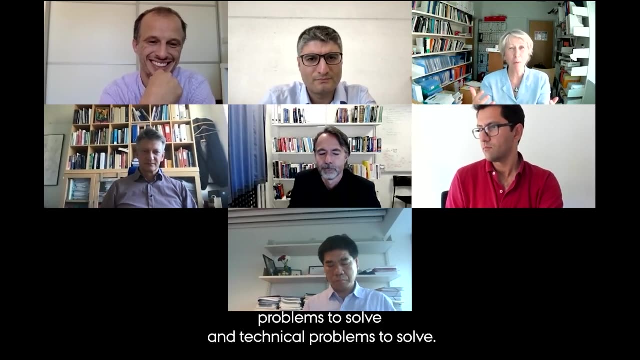 fly patterns of the drone. right, it's not that any drone is the eye in the sky, but it depends very much on how it moves. so there's lots of research out there. now my question to you is: does that matter? I mean, obviously you have so many practical uh uh problems to solve and technical problems to 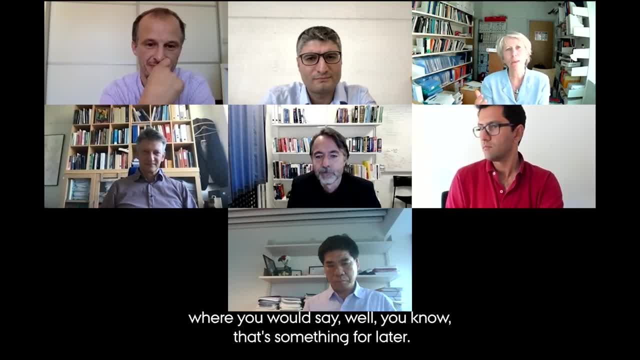 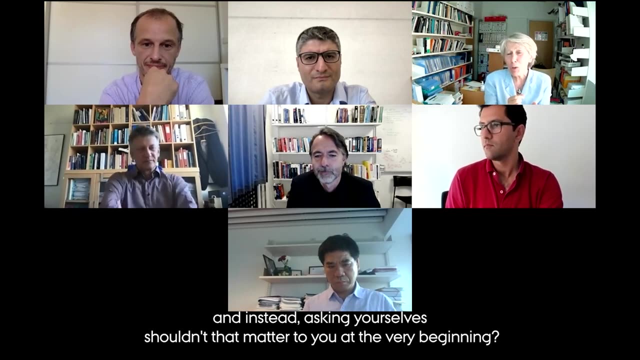 solve. I could perfectly understand that it doesn't matter where. you would say, well, you know, that's something for later. but I I want to invite you to think about starting on the other end, and and, and, and. so asking yourself: shouldn't that matter to you at the very beginning? the more you put your technology into society, the more it becomes. 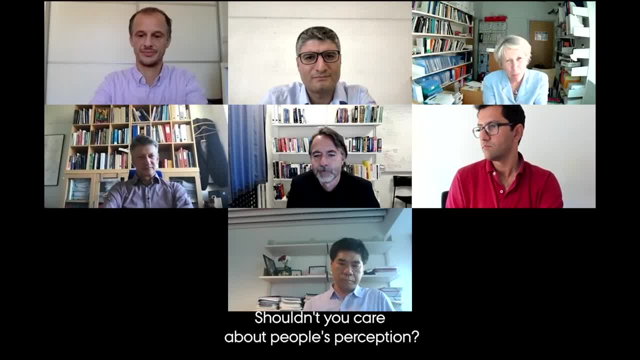 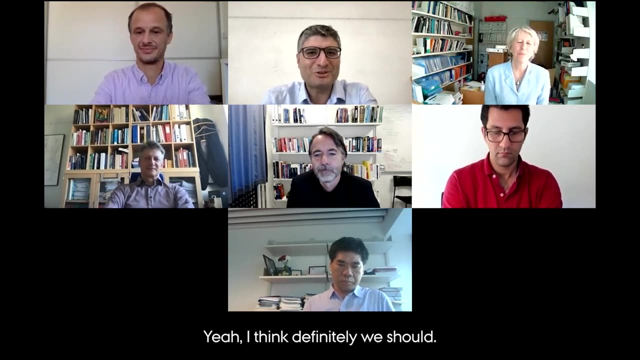 interactive. shouldn't you care about people's perception? and, given that, of course, you cannot do everything alone, um, wouldn't it be good if we collaborate more? that's the idea. yeah, I think uh definitely we should uh, but personally, I haven't uh spent time for this part of the picture. 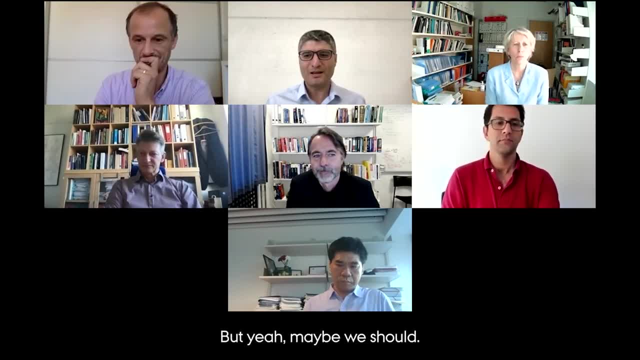 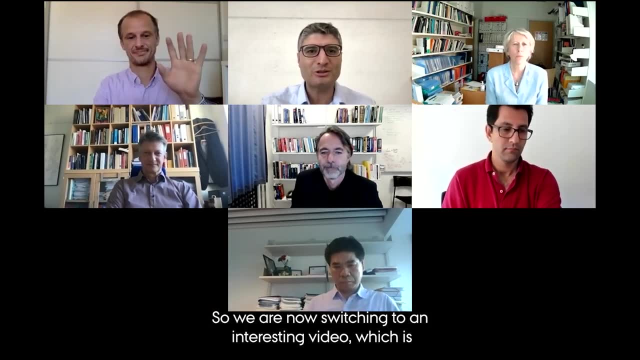 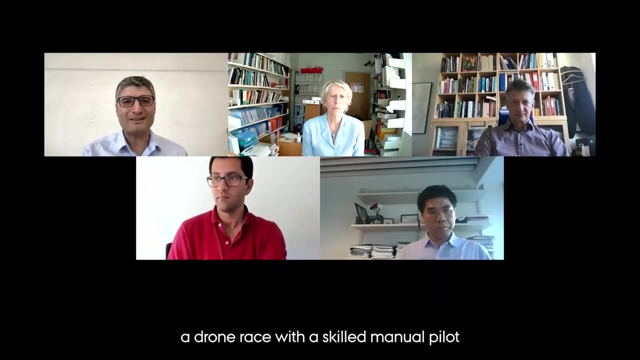 um, but, yeah, maybe, yeah, we should. um, okay, so I think the time is up. um, there's no more question from the audience. so, um, we are now switching to an interesting video, which is um at drone race with a skilled manual pilot and with our sophisticated AI algorithms. 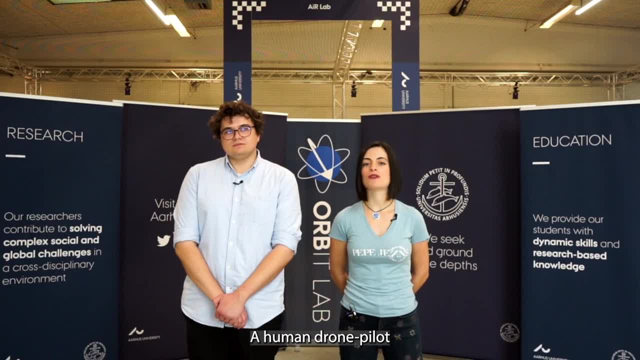 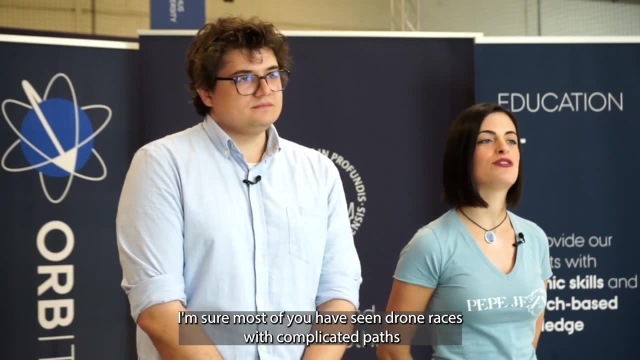 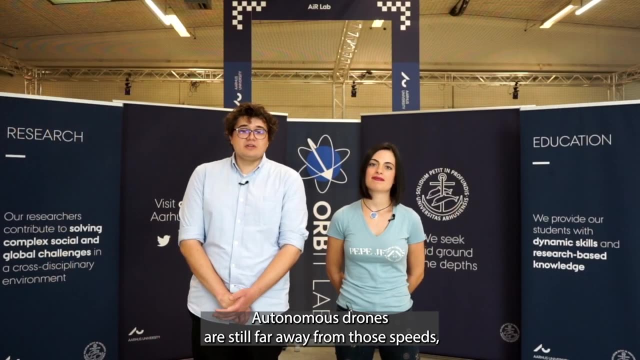 the human body has mind-blowing skills. a human drone pilot can fly on ultra high speeds without having any crash with environment. I'm sure most of you have seen drone races, with the complicated paths and crazy speeds that the human pilots can achieve with their drones. autonomous drones are 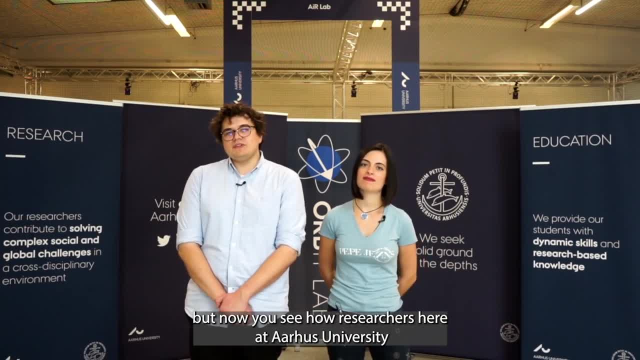 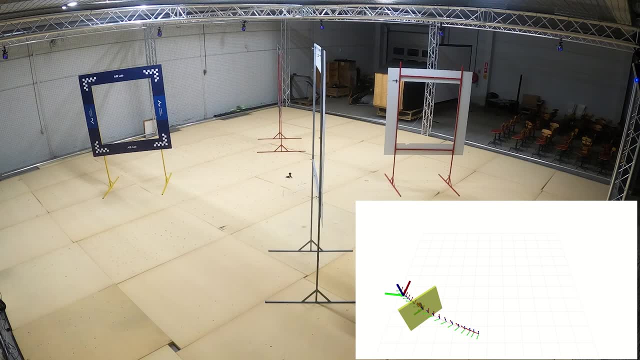 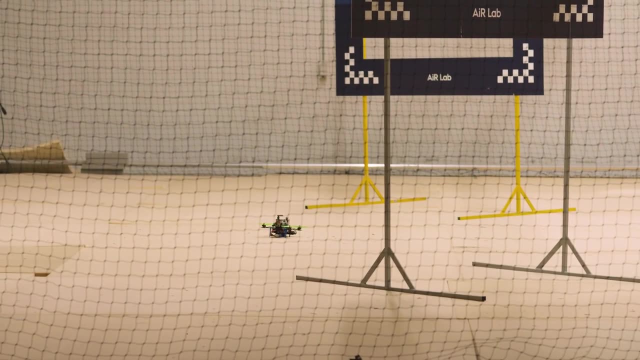 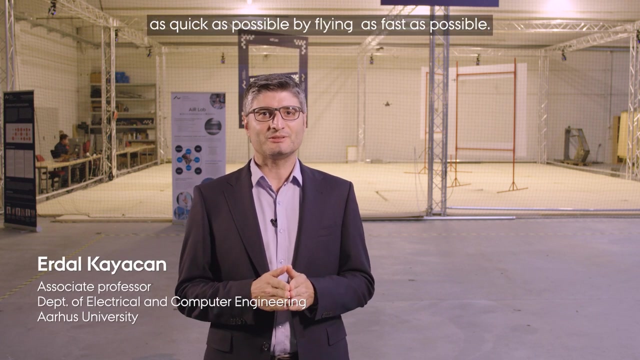 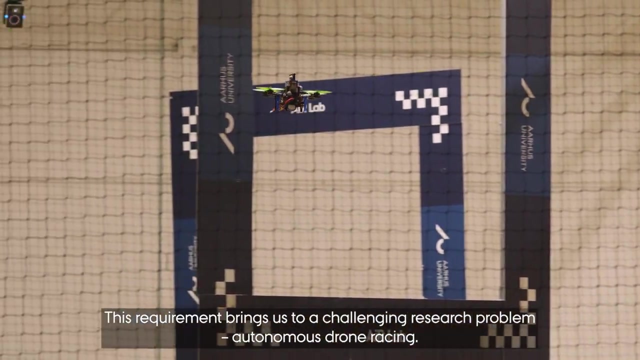 still far away from those speeds, but now you will see how researchers here at Aarhus University are working on minimizing this gap. since drones have limited battery life, they have to complete their tasks as quick as possible by flying as fast as possible. this requirement brings us to a challenging research problem: autonomous. 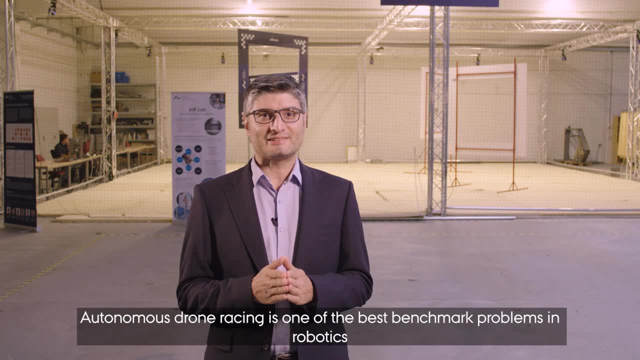 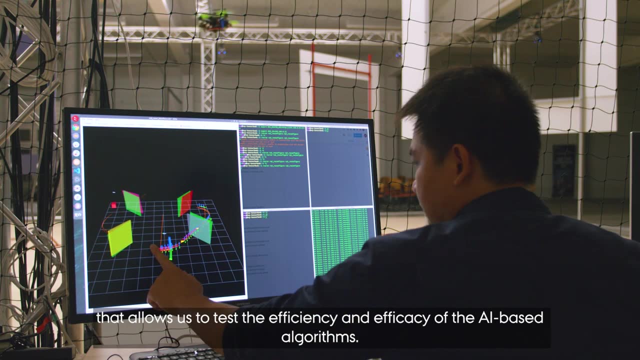 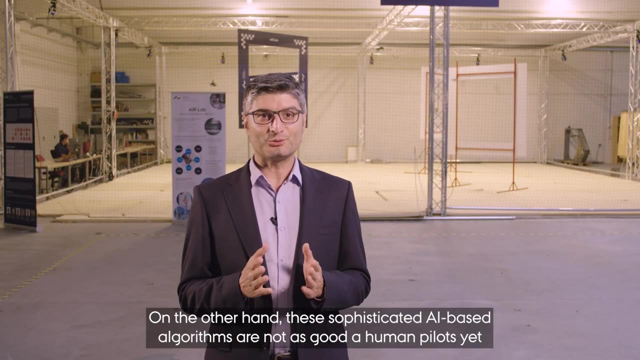 drone racing. autonomous drone racing is one of the best benchmark problems in robotics that allows us to test the efficiency and efficacy of the AI based algorithms. on the other hand, these sophisticated AI based algorithms are not as good as human pilots yet in most of the real-time scenarios, this is because 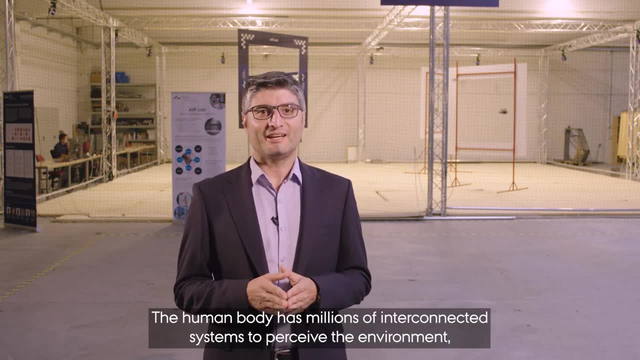 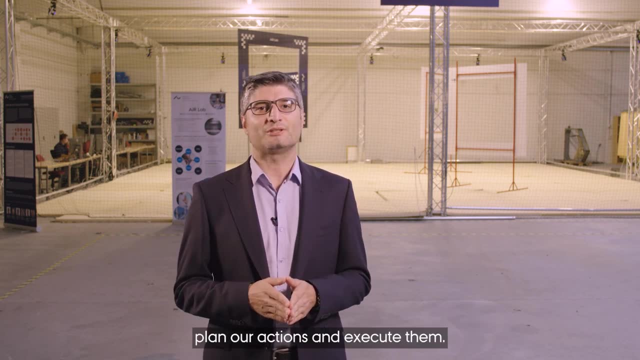 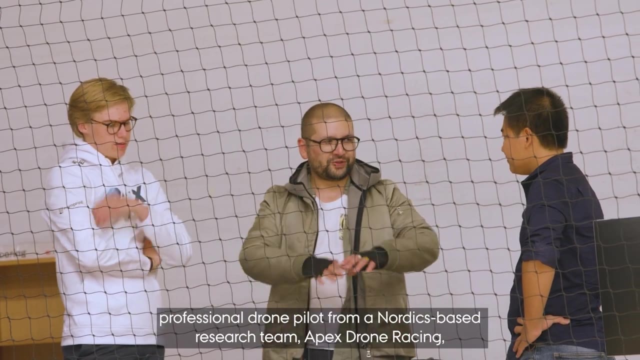 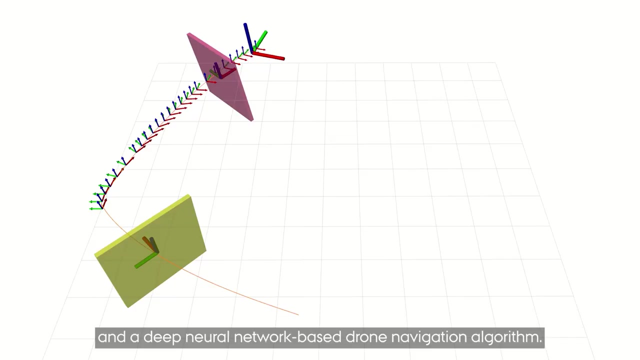 human body is amazing. the human body has millions of interconnected systems to perceive the environment, plan our actions and execute them. in this video we will try to show the performance comparison of a skilled human professional drone pilot from a Nordic based research team, Apex drone racing, and the deep neural network based drone navigation algorithm. 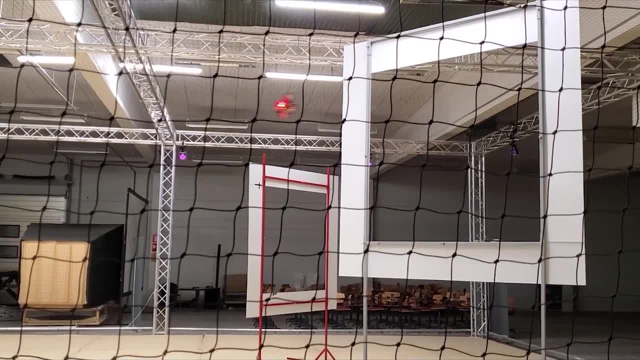 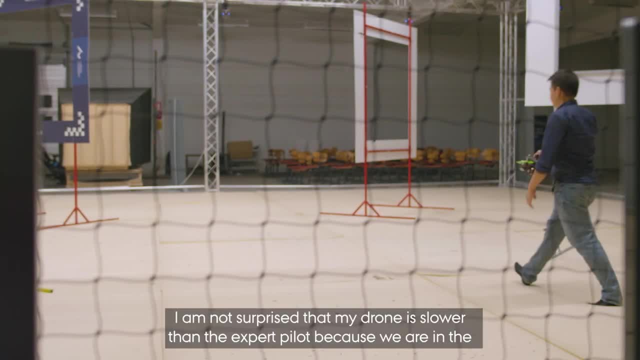 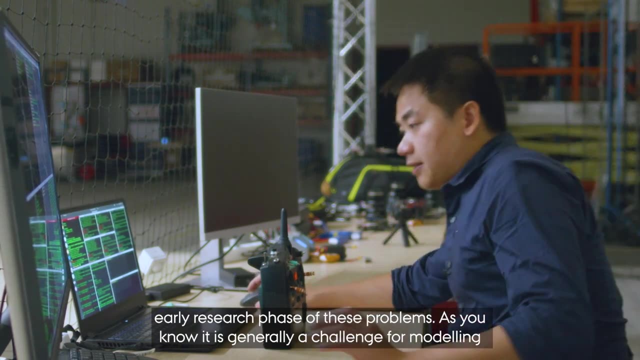 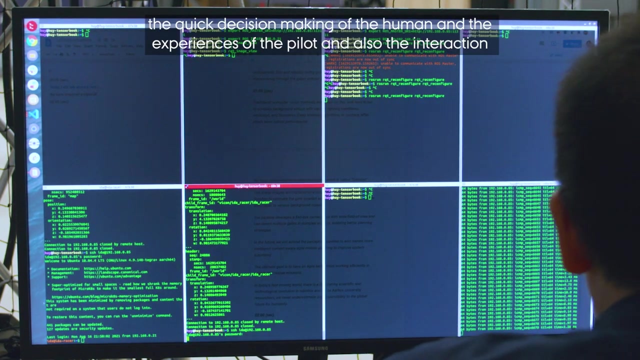 I'm not surprised that my drone is slower than the. the expert pilot- because we are in the early research phase of these problems, as you know, is generally challenged for mordor's the quick decision making of the human and the experiences of the pilot, and also the interactions between 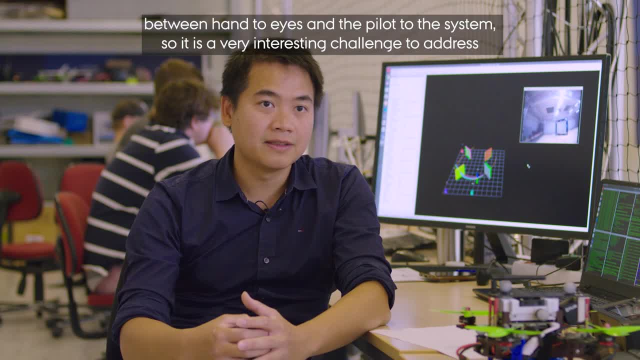 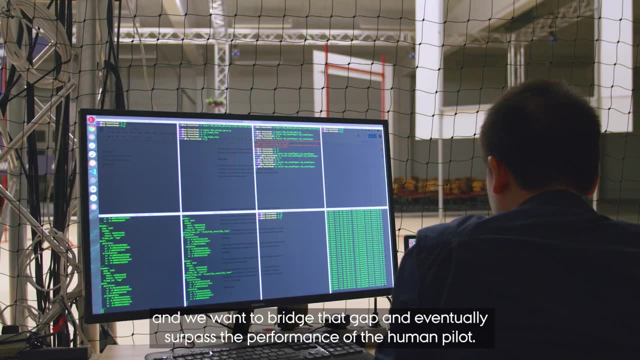 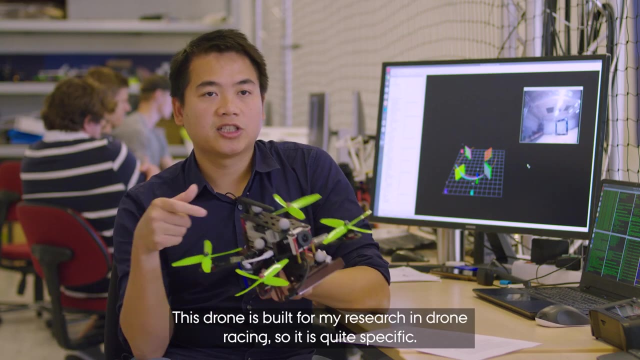 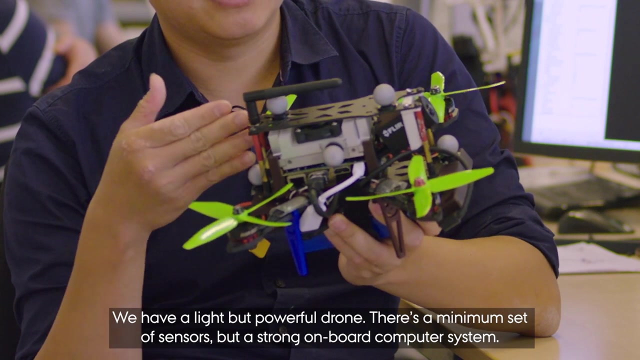 hand-to-eyes interactions of the pilot to the system. so it's a very interesting challenge to address and we want to bridge that gap and eventually surpass the performance of the human pilot. this drone is built for my research in drone racing, so it's quite specific. we have a light but powerful drones and there's a minimal. 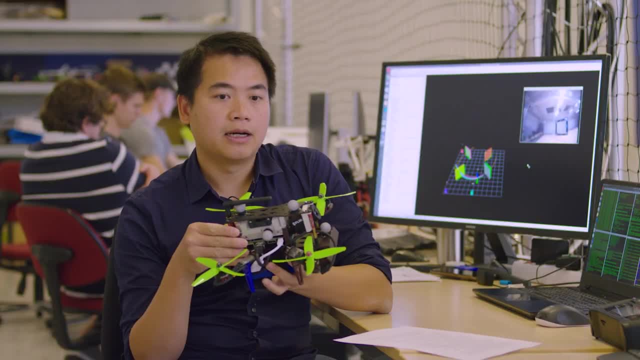 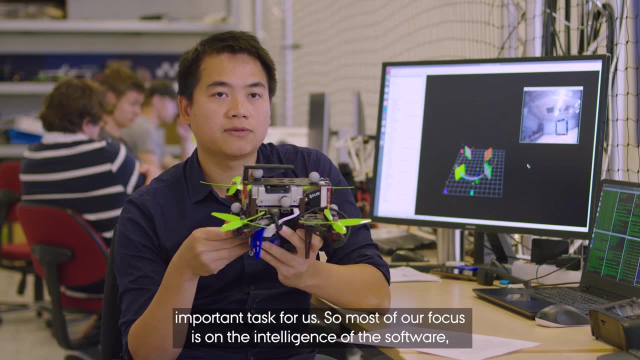 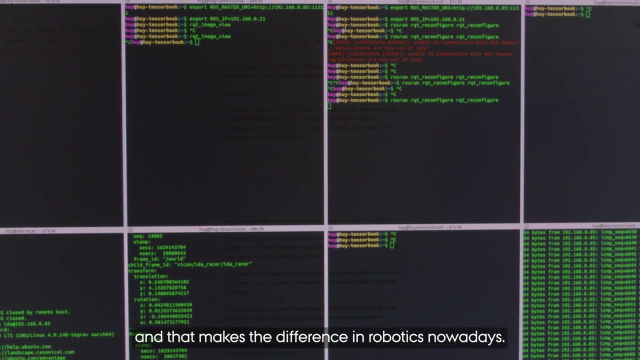 set of sensor but a strong onboard computer system. the challenge is to quickly understand the environment, so perception is a very important task for us. so most of our focus is on the intelligence of the software, and that's make the difference in robotics. nowadays, I think the biggest challenge is in. 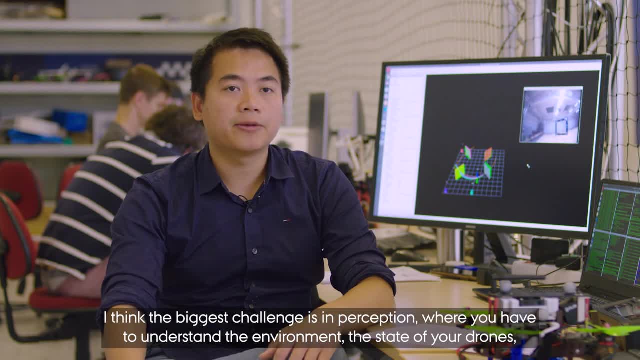 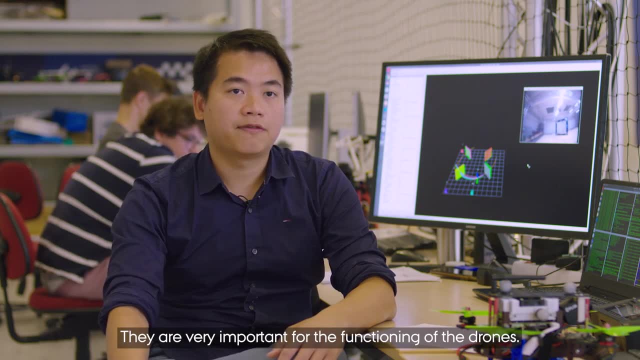 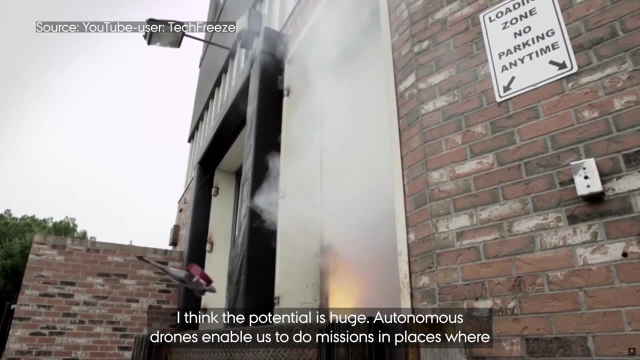 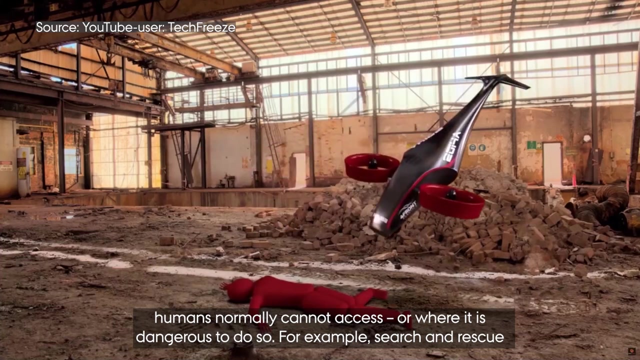 perceptions, where you have to understand the environment, the state of your drones, the context and the situations. they are very important for functioning of the drones. I think the potential is huge. autonomous drones enables to do the missions in the place where normally humans is cannot access or is dangerous to do so, for example, search and rescue. 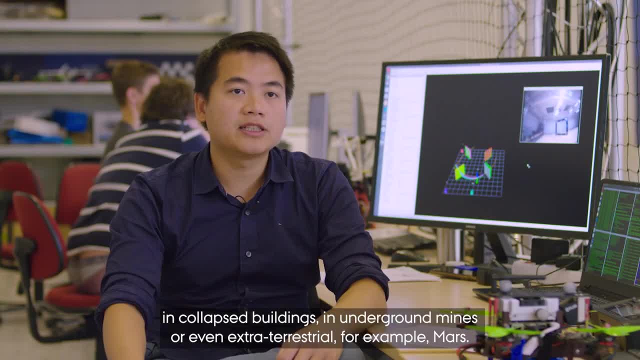 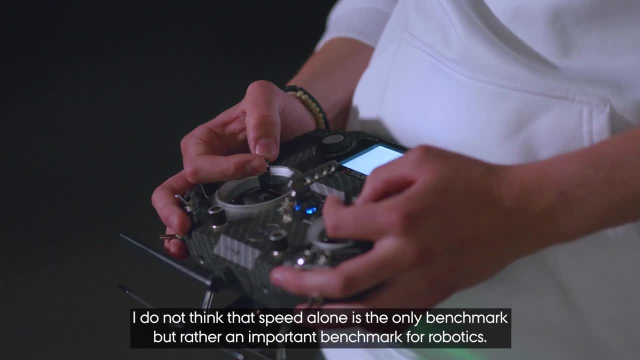 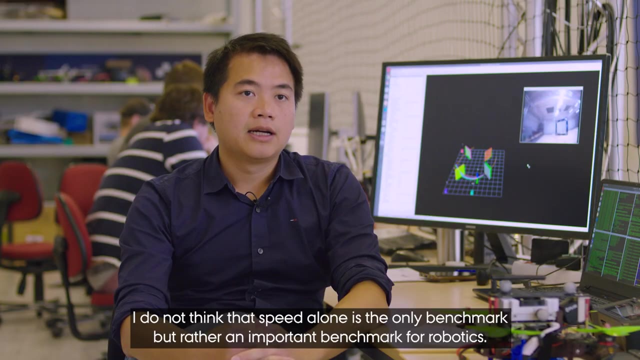 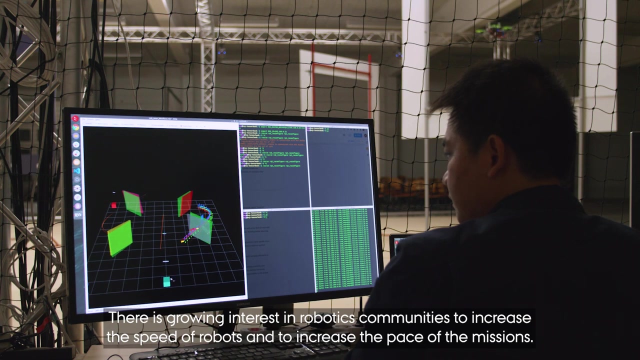 in collapsed buildings, in underground mines or even extraterrestrial, for example, Mars. wow, keep getting faster. I do not think that speed alone is only benchmark, but rather an important benchmark for robotics. there's a growing interest in robotics communities to increase the speed of robots and to 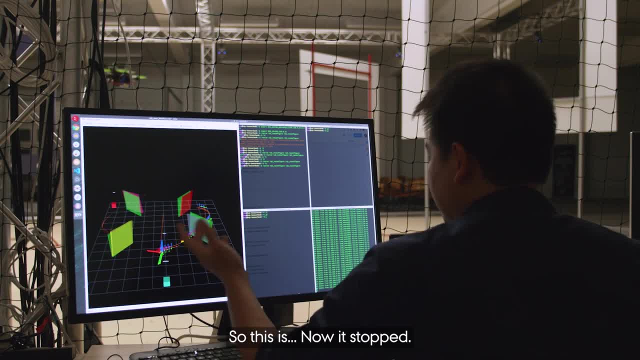 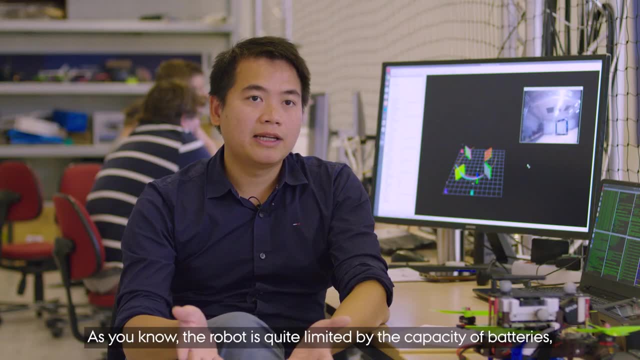 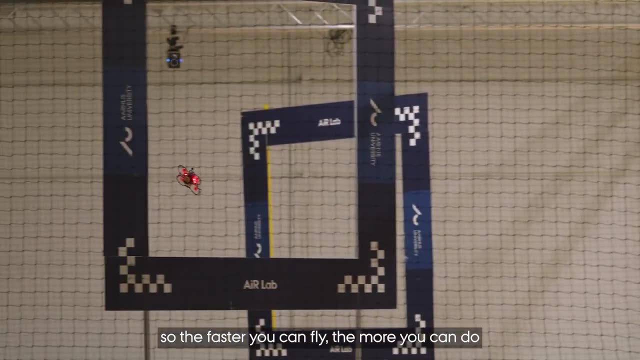 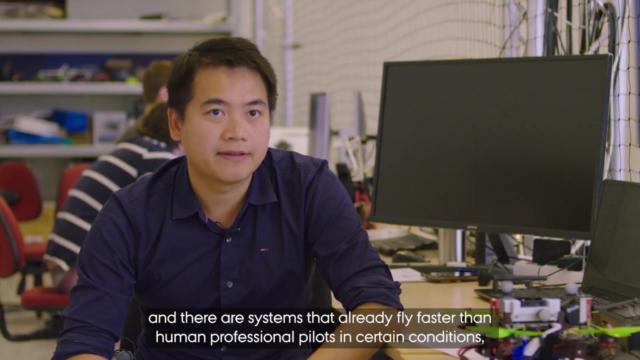 increase the pace of the missions. so should we start again? as you know, that robot is quite limited by the capacities of batteries, so the faster you can fly, the more you can do and the further you can reach. there's a lot of research and there are systems that already fly faster than human professional pilot in. 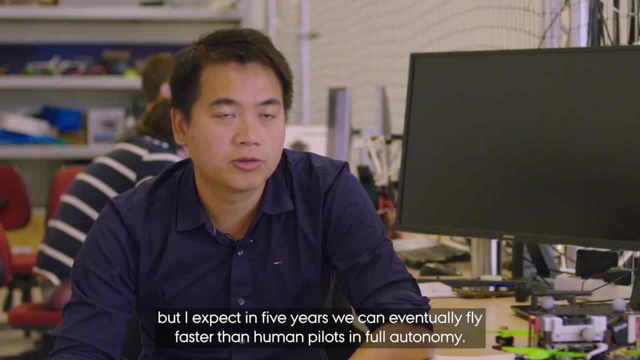 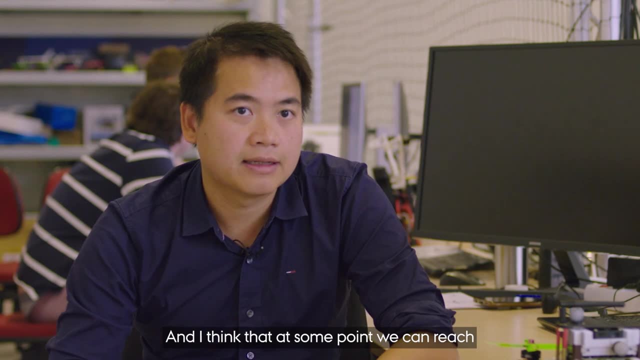 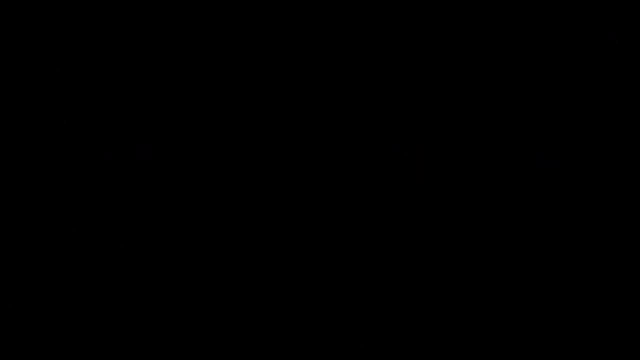 some certain conditions, but I expect in five years we can eventually can fly faster than the human pilot in full autonomy and I think at some point we can reach to the performance of a superhuman. thanks a lot for attending this online event today. I would like to 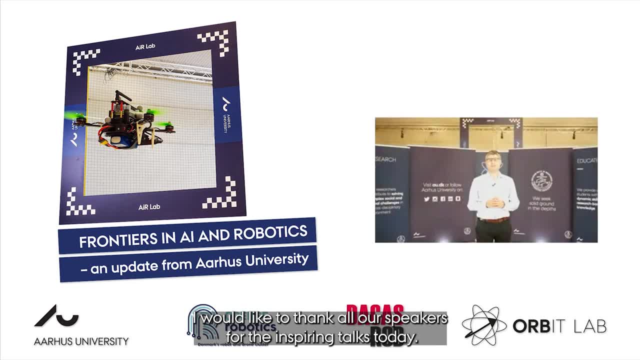 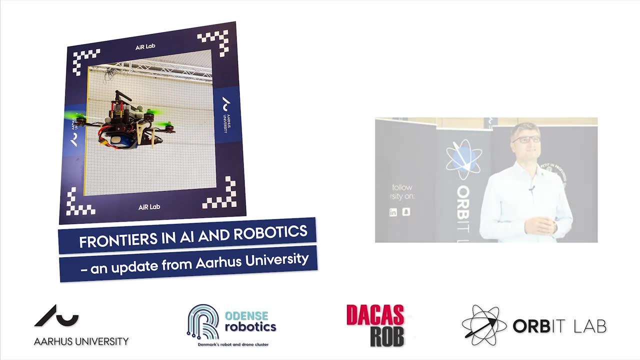 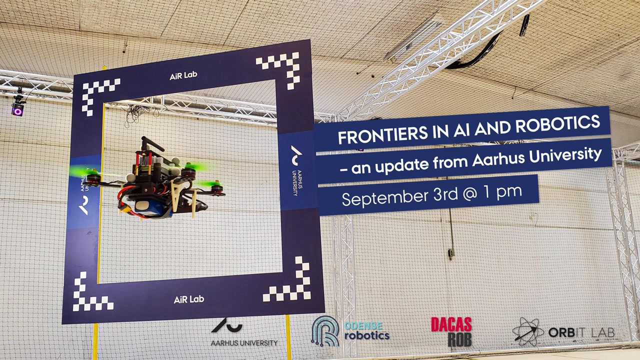 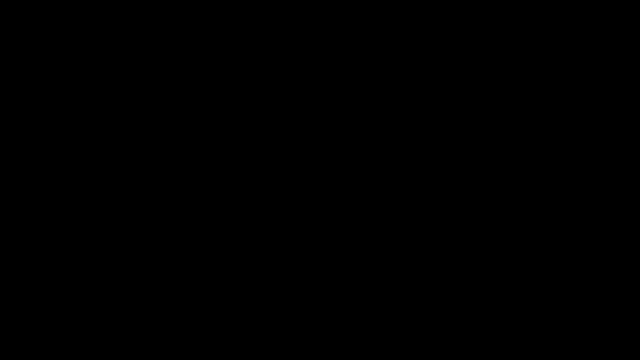 thank all our speakers for the inspiring talks today and thank you for people who have attended this online event and we like to see you in the future with with another events at Aarhus University. you.